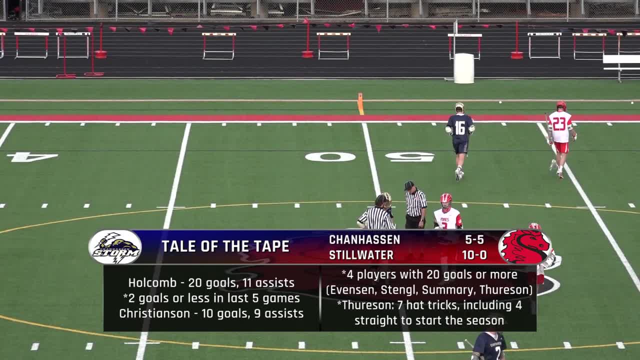 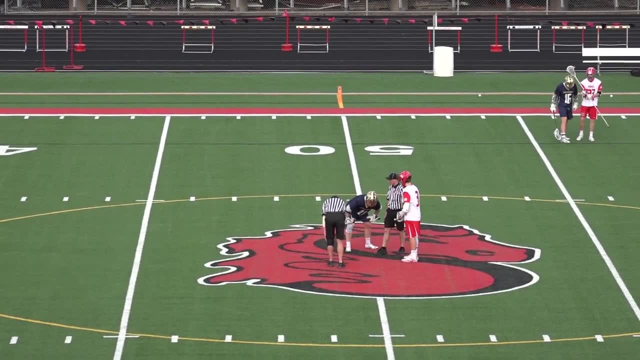 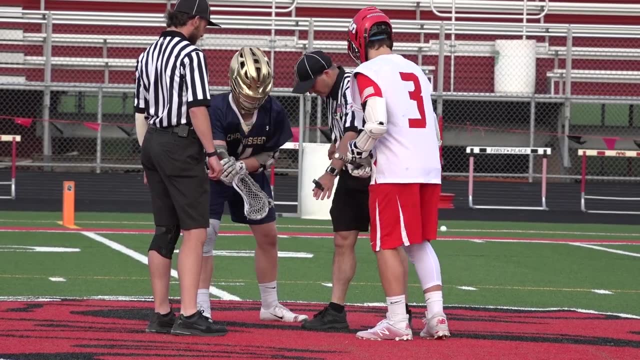 may have been the first one against Monomidai, when they had some struggles with ball control. ever since they've cleaned that up. they had a couple of miscues against White Bear Lake, but, as you said, their ball control is on point and they make it really difficult for opponents to sustain any kind of rhythm. 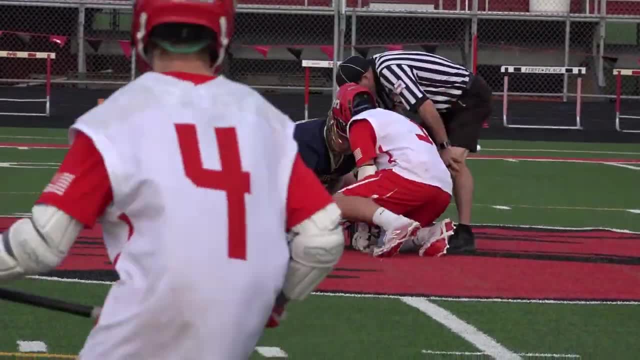 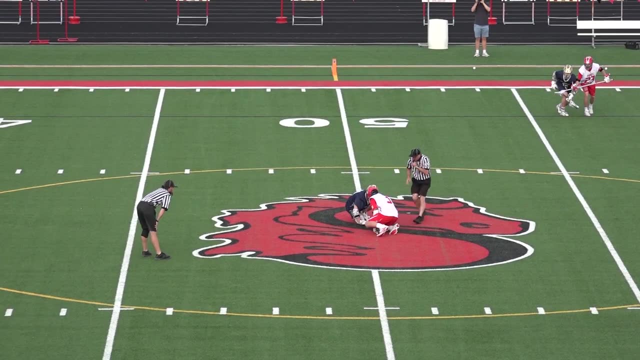 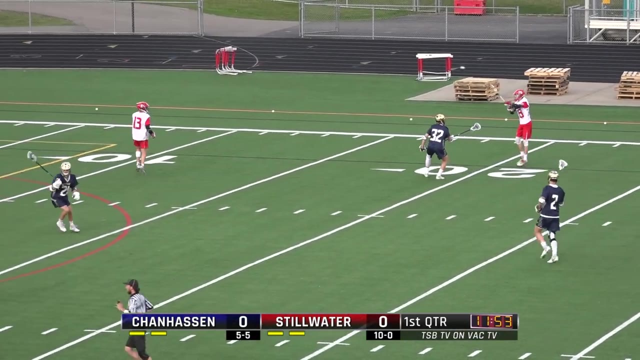 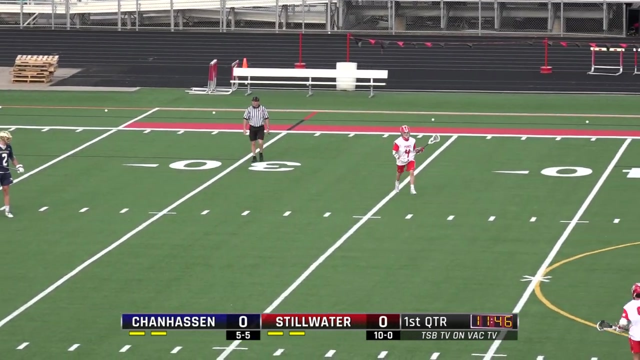 on. offense ponies have two more games after this, both winnable ones. it's a likely that they're gonna run through the tables undefeated. they have Parker Cottage Grove next week. NYZ ponies win the face-off. that's Corbin Van Dyne, the freshman. I happen to know Corbin's mother for a very strange reason. I was. 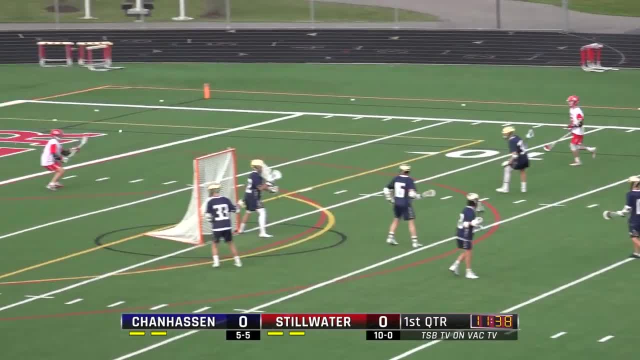 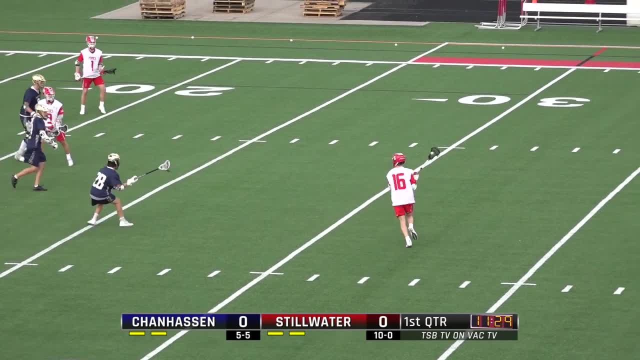 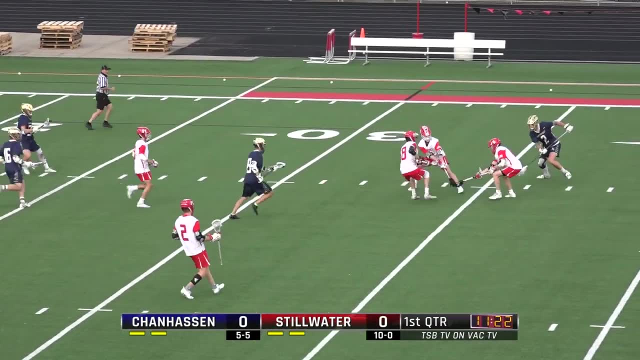 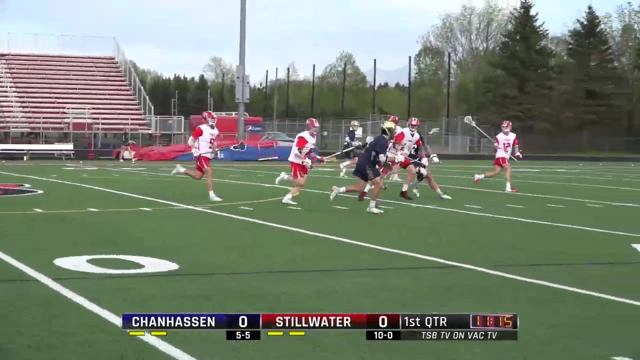 hosted. I don't remember hosting her myself is like anything else. you cover so many groups or host so many groups, it becomes a blur. but you told me they were on the struggle bus a little bit, but in a weird way Corbin's mother is the second person with Stillwater ties that I've hosted. I 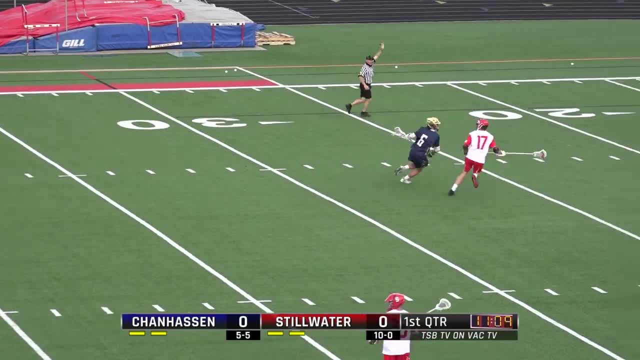 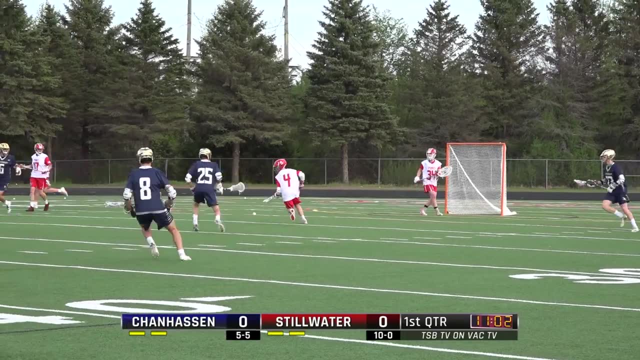 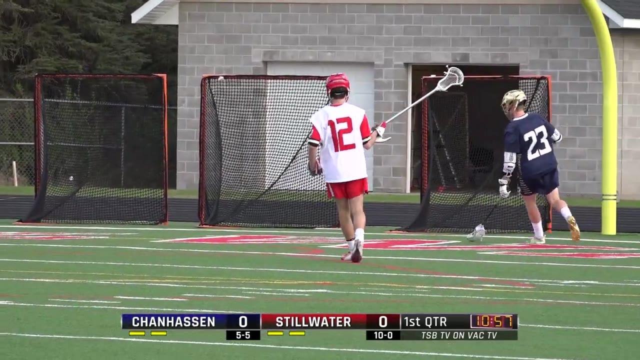 also hosted Ricky Michael and his family at an escape room last spring. Chanhassen with the ball. they tried the quick stick and that's what Chanhassen is gonna have to work on is the passing game. but Stillwater with a turnover. it's dangerous when that happens and Stillwater escapes with no damage. 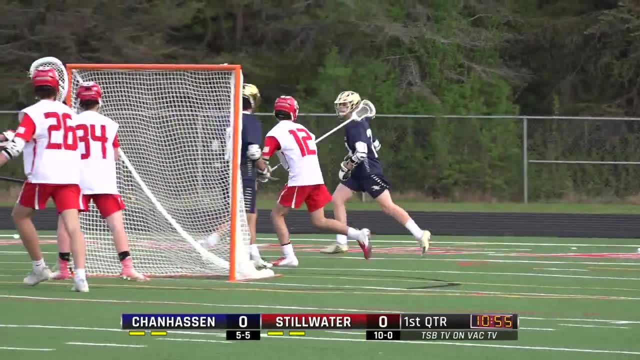 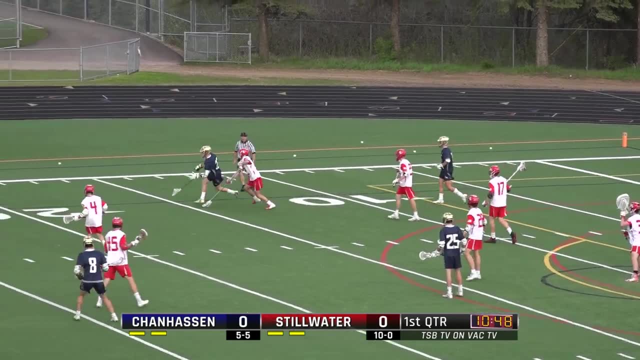 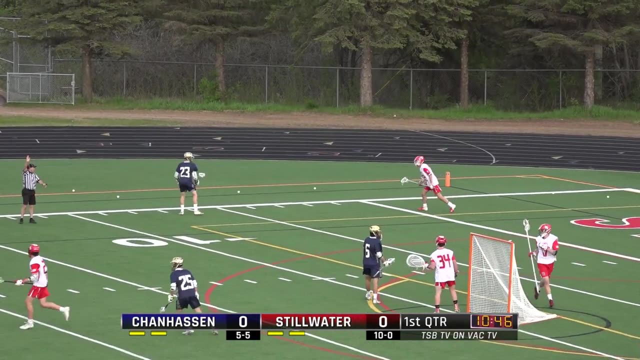 Tyre Christensen was right there and we saw this happen a couple of times. turnovers in their own side of the net can be disastrous. Gunnar saw the net so far over a couple of shots, no fear whatsoever, and Stillwater catches a break. foul called on Chanhassen. 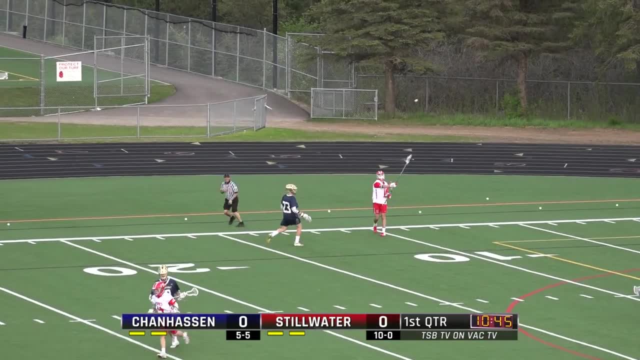 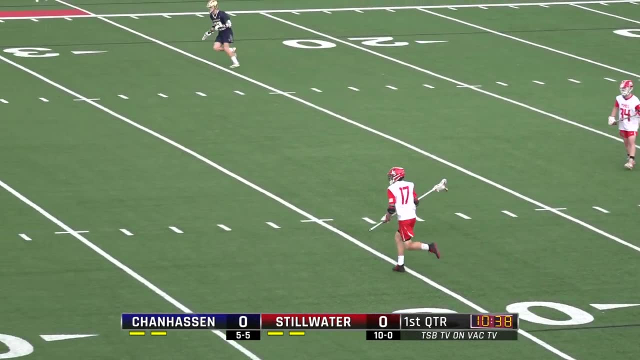 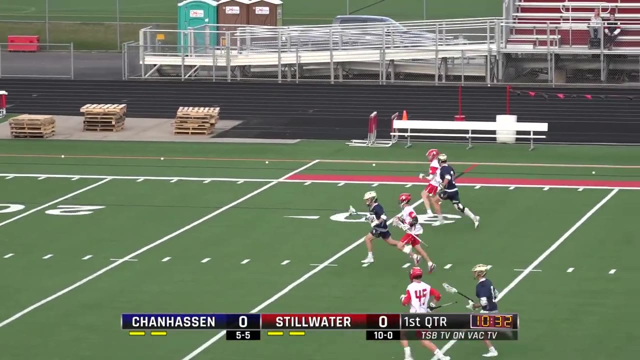 a sloppy giveaway by Stillwater in the offensive zone caused a little bit of havoc in their own end. if there's one knock for Stillwater, that is it turnovers on their own side of the field. but they can make up for it on offense, as we've. 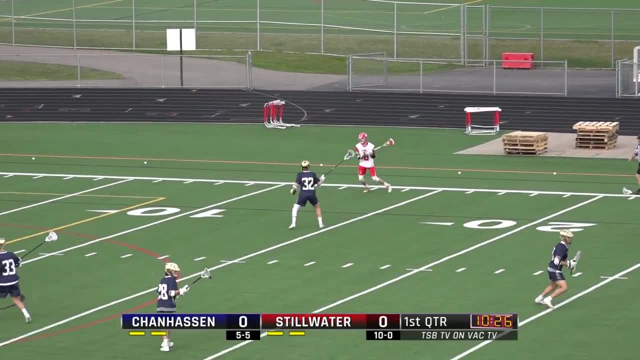 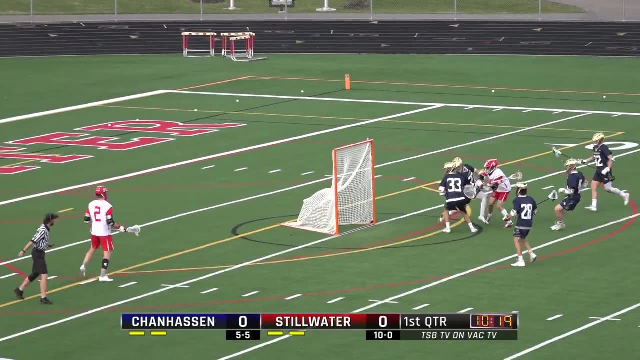 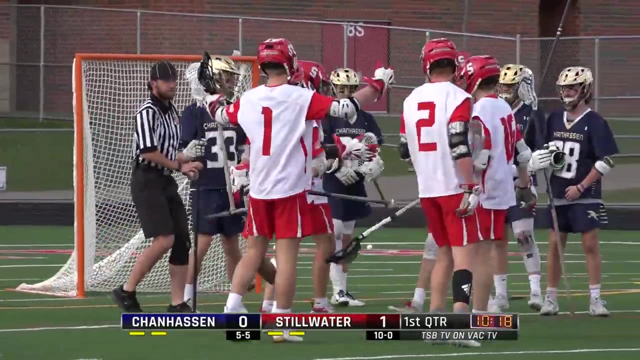 seen. as we said, the season opener may have been their toughest game. out of me, die was trailing by just one at halftime and then the ponies pulled away and the second half. and here they go again. what a great move by Quinton White. Quinton White gets the ponies on the board. we know they can score quickly and 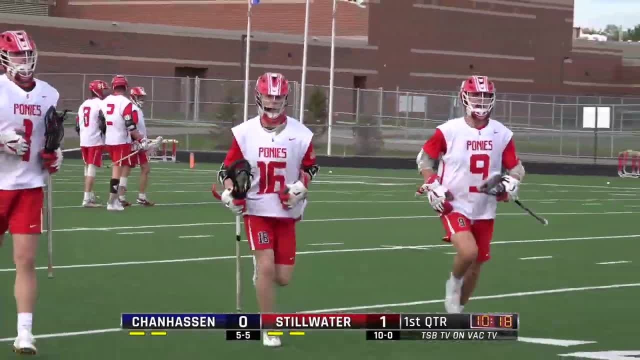 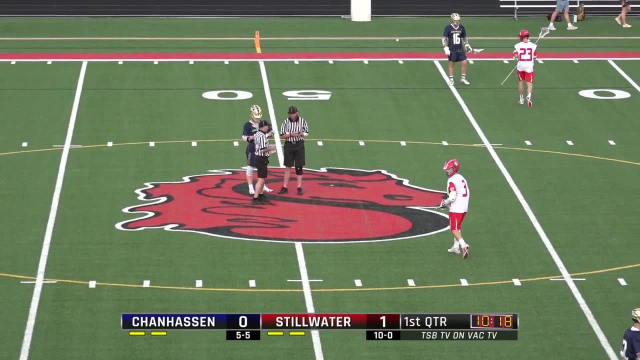 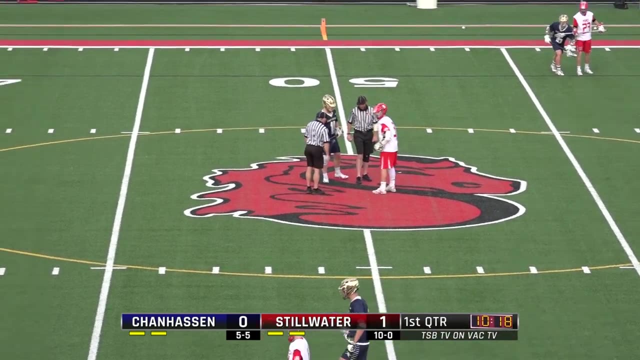 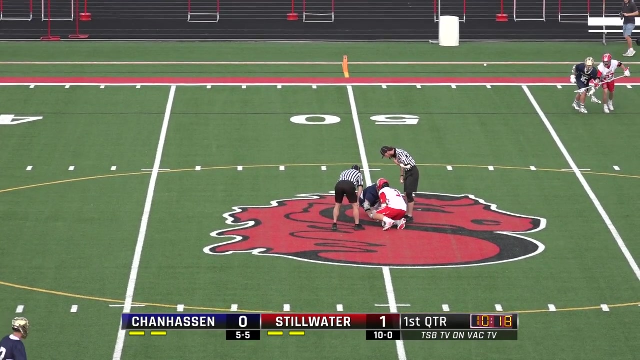 they can score big. they scored 11 goals against st Thomas Academy in the first half. they scored 10 against Eastridge. yeah, great, giving goal from Blake Evanson. he faked it to Quinton, he passed back to Evanson and then back to Quinton again, who faked up high, then went down low. with it low and 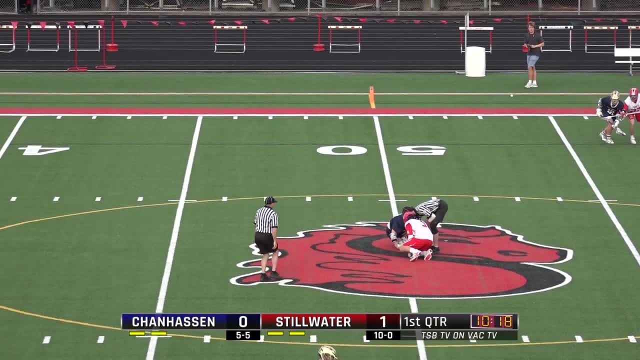 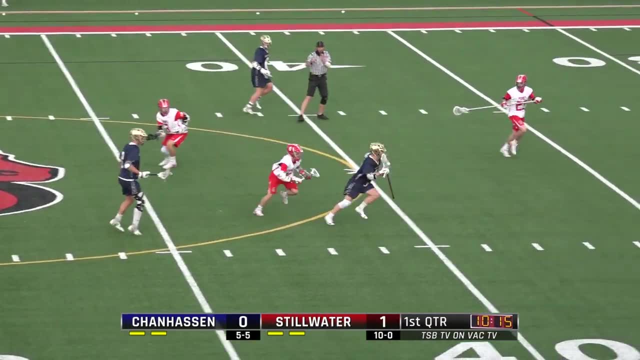 hard Blake Evanson, entering this game third in the state in assists, he just picked up his 27th of the year. Quinton White goal number 17. the ponies, they don't post stats in the hub. Chanhassen wins the face-off but that gives you an. 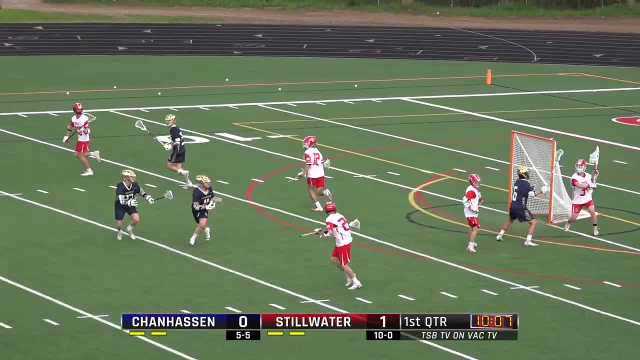 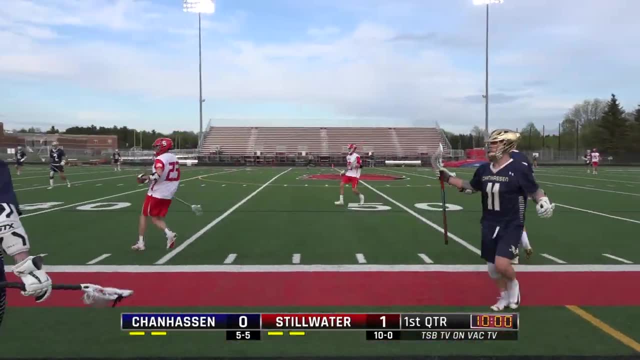 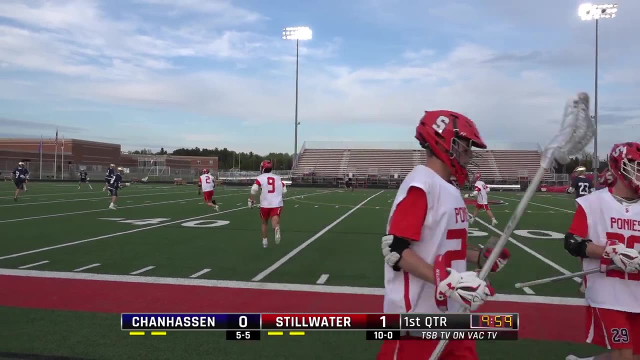 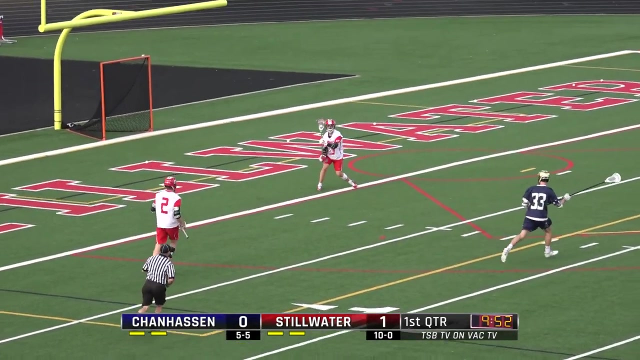 idea and the storm not wasting any time. and another big save by Gunnar Ahrens to swat away Nate Nicholson. we mentioned Chanhassen and their lone 20-goal score. that is, Hunter Holgum: 20 goals, 11 assists. Nicholson, one of the captains you. 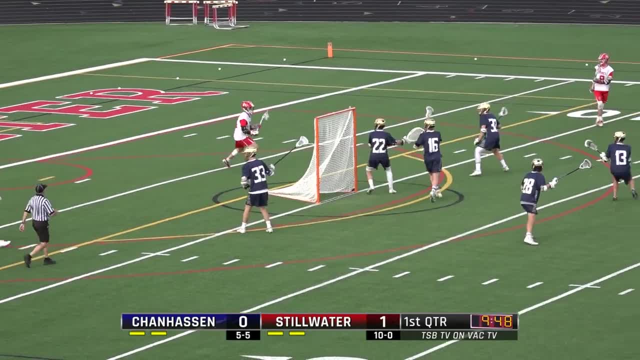 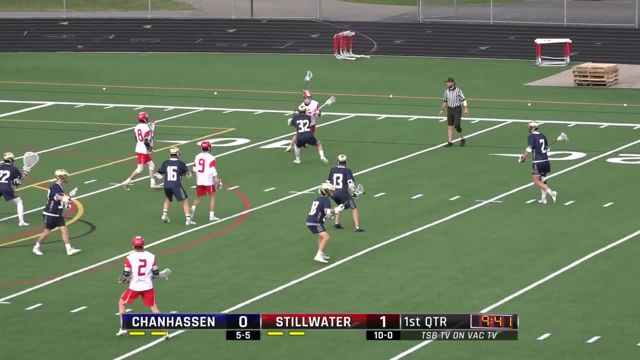 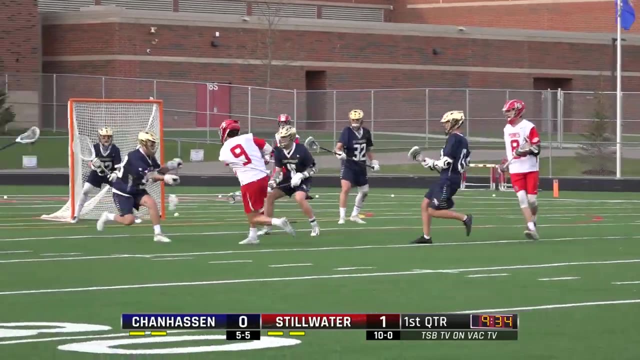 may have seen Chanhassen on school space media broadcasts. of course you definitely have seen Stillwater on Valley Access channels on a perfect spring evening. temperature hit 80 degrees for the first time this calendar year and the ponies are heating up on offense Evanson, the set up man, Joe. 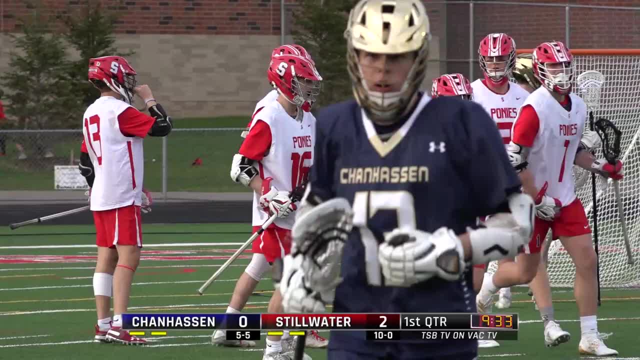 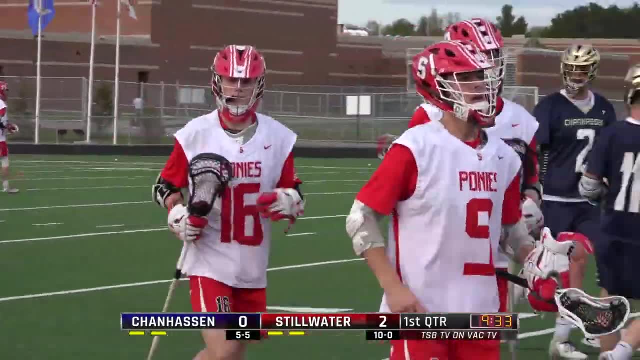 Stengel with the goal and Evanson doing what he does best: facilitate the offense and start me up as a fitting tune with the ponies starting up another potential big rally, why you've seen lots of hookups between those two this season so far. Mike Evanson, a long way to go. 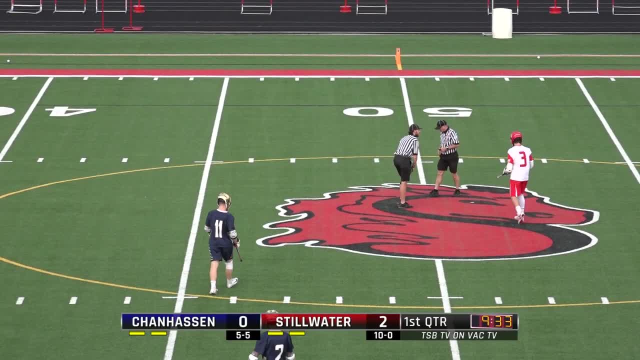 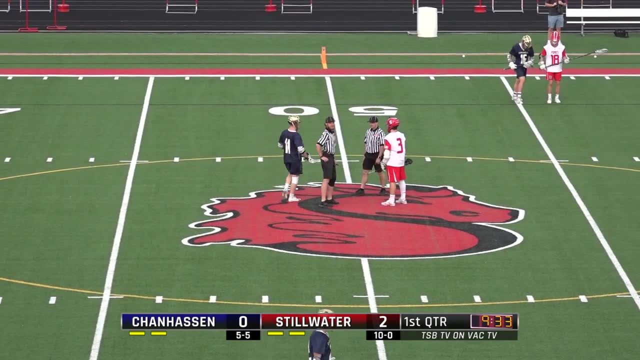 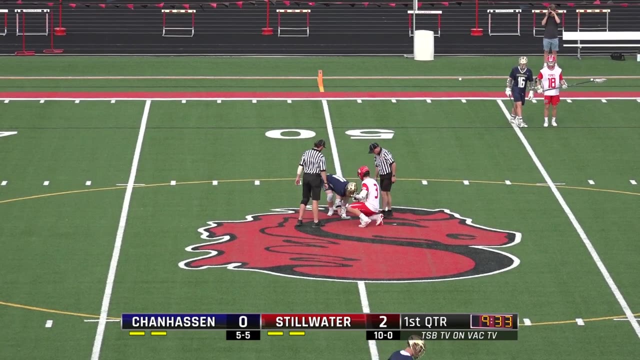 and Stengel, Just two great players that can see the field and the ball really well. Joe Stengel with his 23rd goal of the year- Well, not every public address announcer can be perfect- And Evanson with assist number 28.. 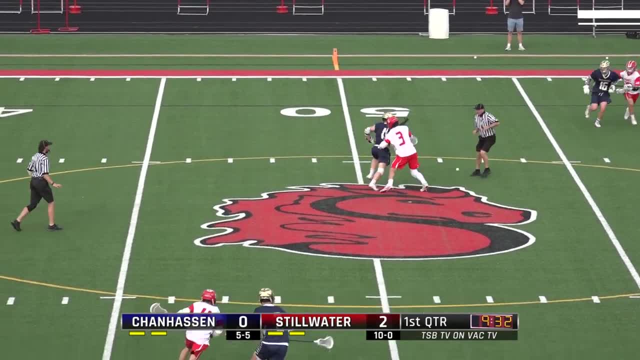 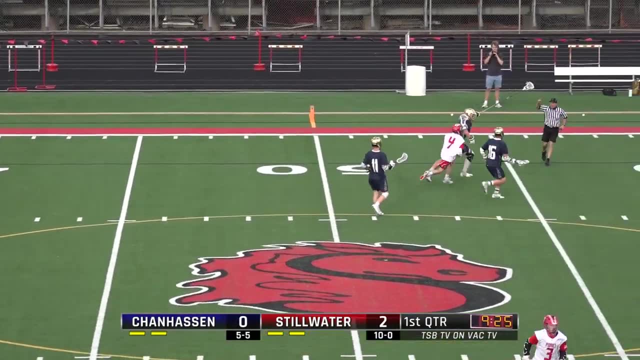 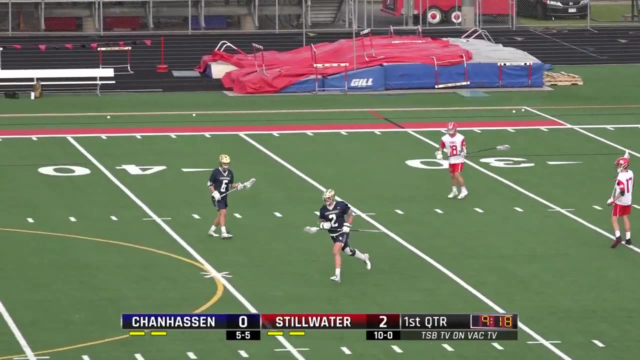 We mentioned Evanson entering this game third in the state in assists. Tyler Thorson would be tied for seventh in goals And it's crazy to think, with a team like Stillwater, that you might think they wouldn't have any players on the leaderboards because of how much they spread the ball around on offense. But 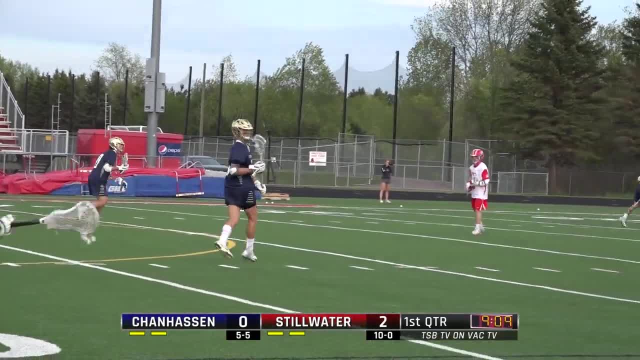 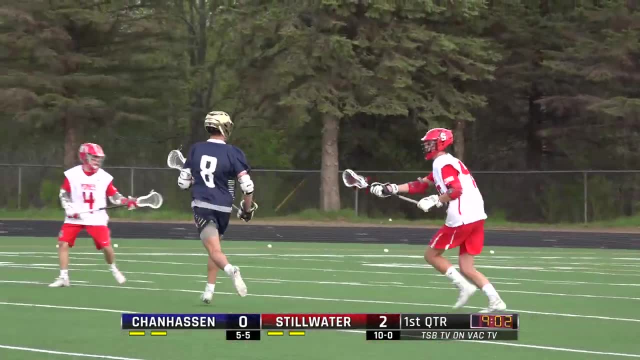 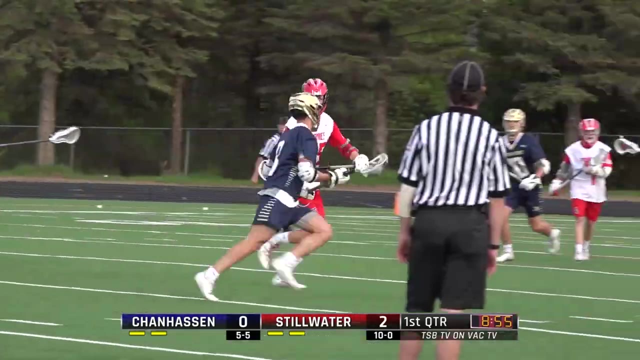 Evanson. he's got so many weapons he can go to. He can rack up assists like crazy And Thorson can rack up goals. Right now it's Chanhassen with the ball. They've had a couple of shots so, unlike some other teams that have a hard time developing an offense, 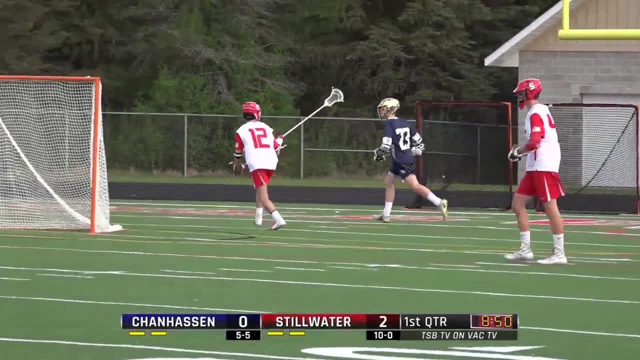 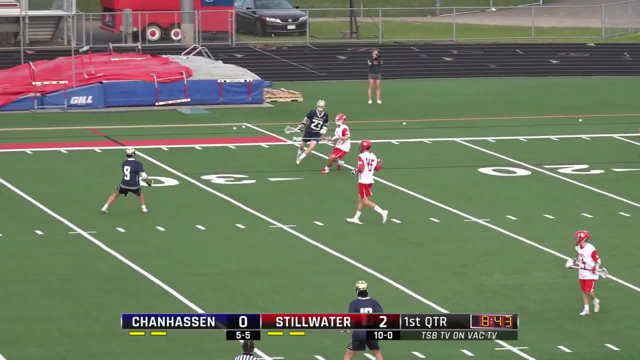 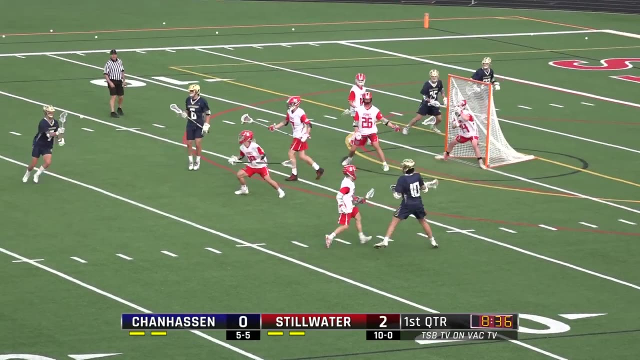 Chanhassen has put together a few quality chances here, But Gunnar Ahrens has stepped up. Ahrens, the sophomore Quite. some really stiff defense by James Stahl, midfielder for Stillwater. just watching this guy ever so closely. Alex Dua with the shot. 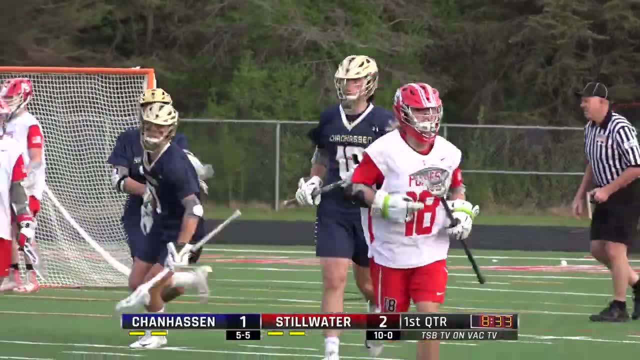 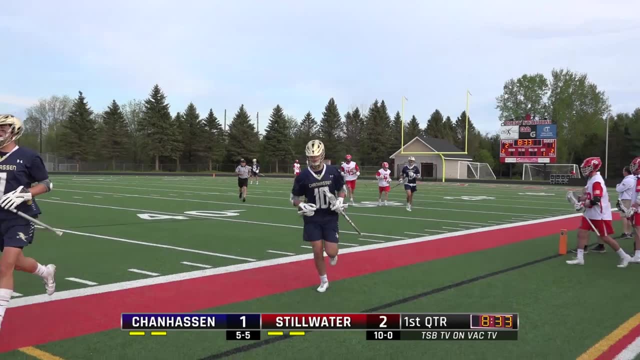 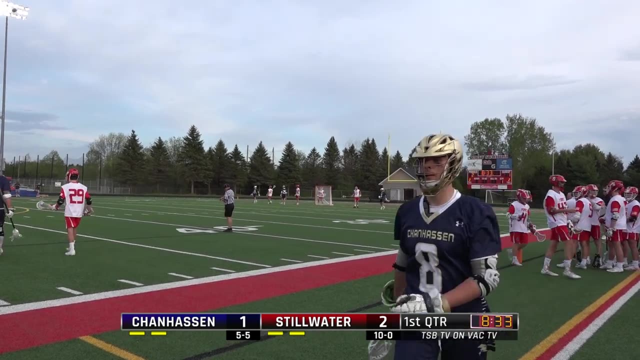 And Chanhassen gets on the board. Alex Dua with his eleventh goal of the year. Alex Dua, one of those big scorers for Chanhassen. You know they've got four guys that have got double digits in goals this year so far. 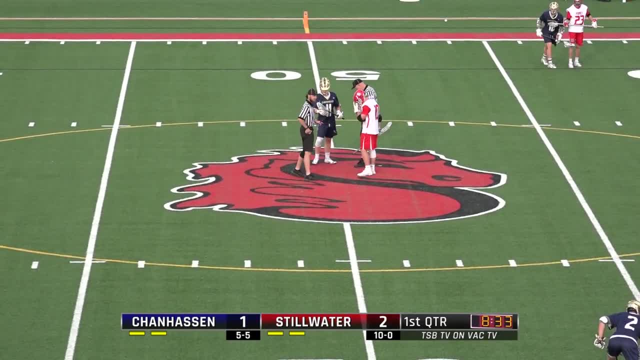 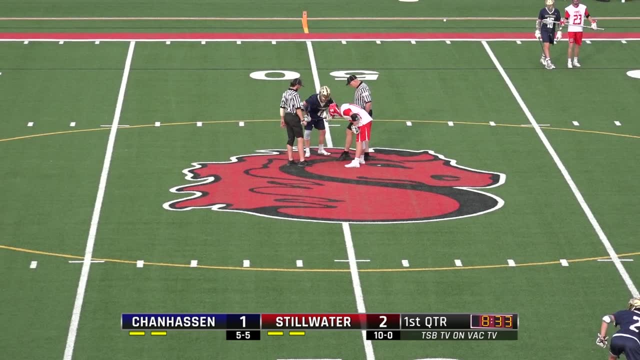 And the man between the pipes. we haven't mentioned his name yet is Zachariah Raphe. Dewey Dewey, Dewey, Dewey, Dewey, Dewey is how they pronounce it. Vincent Manuel will get credit for the assist. 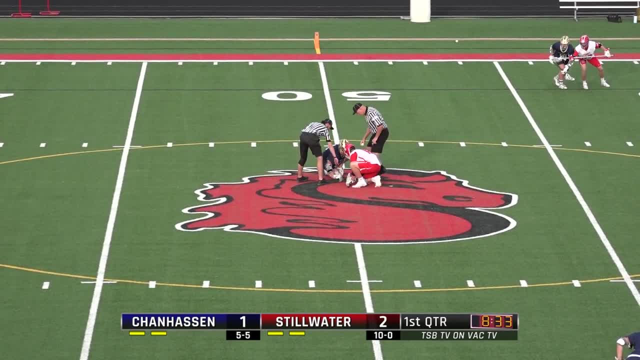 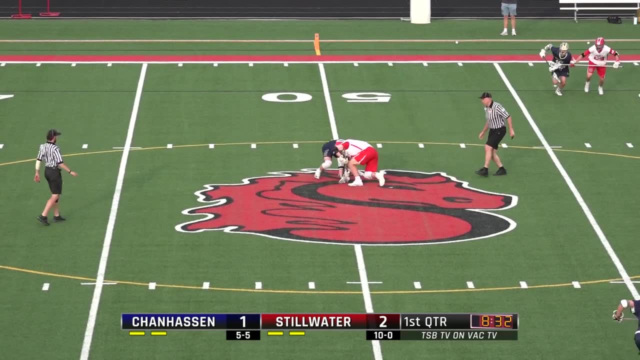 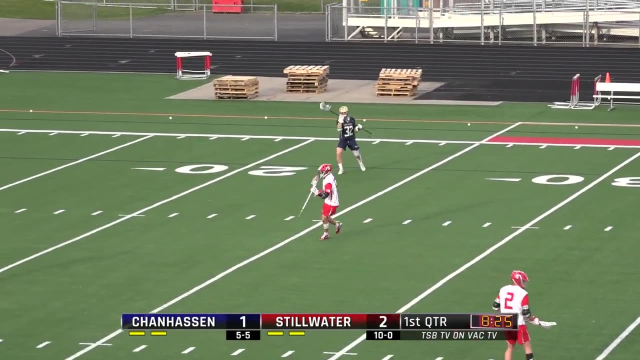 Zachariah Raphe, the Chanhassen goalie, 6.52 save percentage And, as we said, a picture-perfect spring evening. Temperatures hit 80 degrees for the first time this calendar year. We'll have a few more. 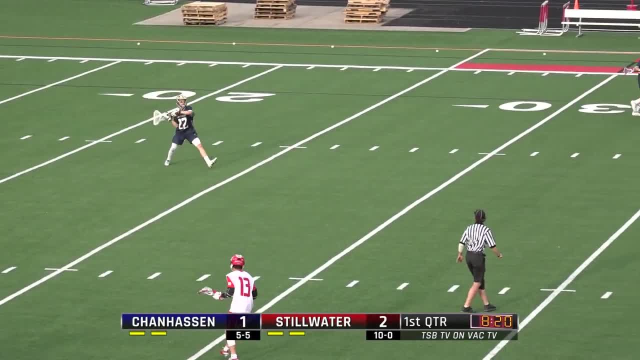 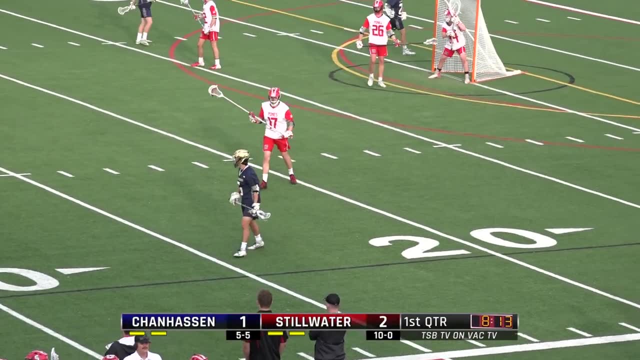 Right now it's 70 degrees. It's going to get cooler this weekend, so I hope you got out and enjoyed some sun, Robert. It'll be a little while before we get back to 80.. I did Just enough to get a little sunburnt there, Mike. 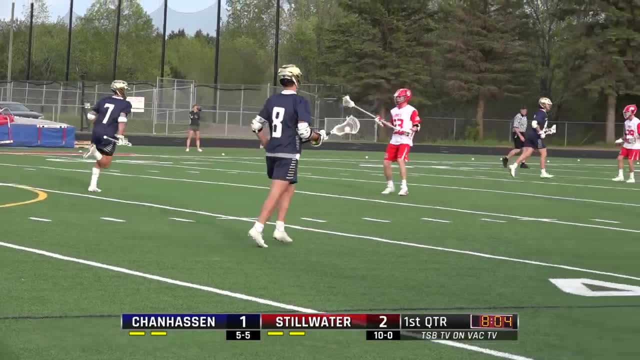 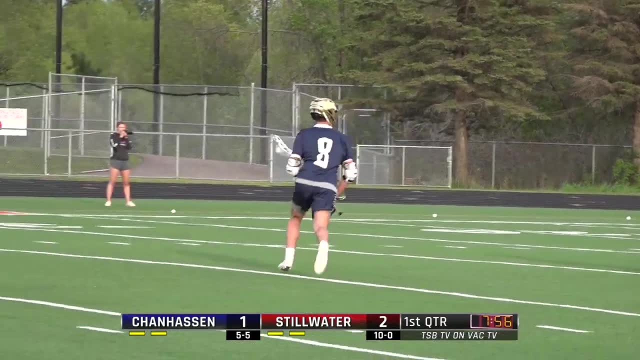 And you had a stoppage in play. No, he didn't. The clock stopped momentarily And it's Chanhassen with the ball, Jason Collins, Pressured by Jamison Stahl. That's Chanhassen with the ball, Jason Collins. 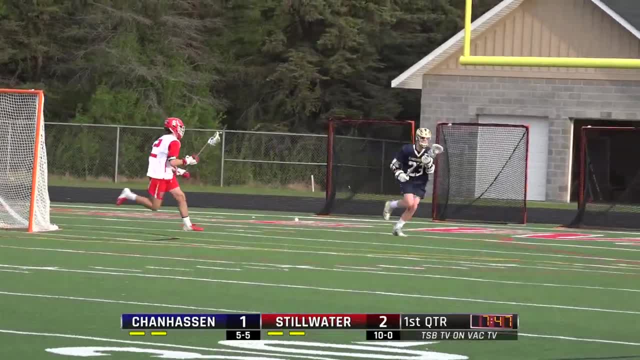 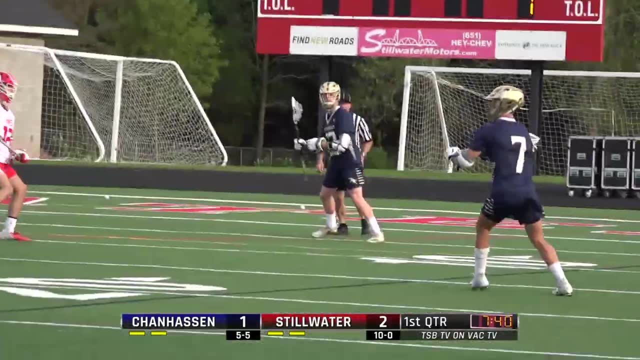 Pressured by Jamison Stahl. Two to one is the score, And there's Cal Davis, one of the players to watch for Chanhassen. One of those double-digit scores that you alluded to, The vision, to Alex Dewey. 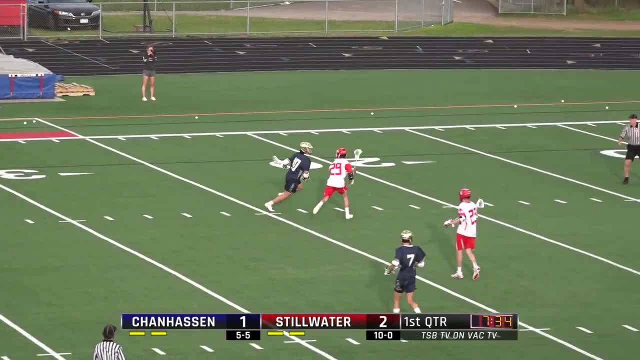 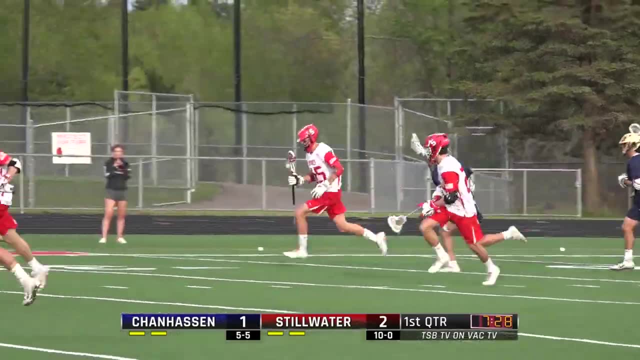 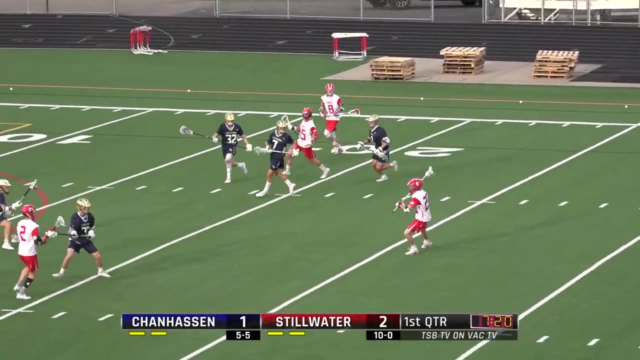 And back out to Vincent. Manuel Sees a lane Fires, Ahrens blocks it with a stick, Loose ball scooped up by the Ponies. It's Jamison Stahl And he'll trot down the field. He'll end it off to Ben Long. 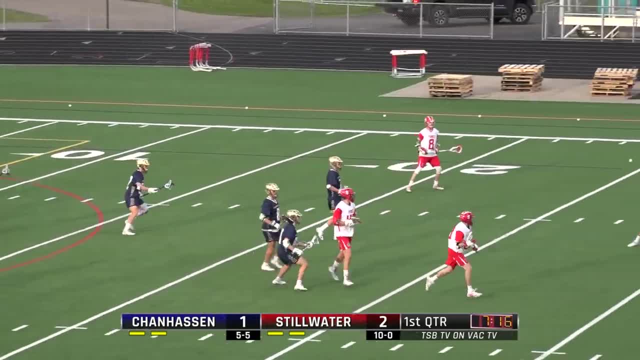 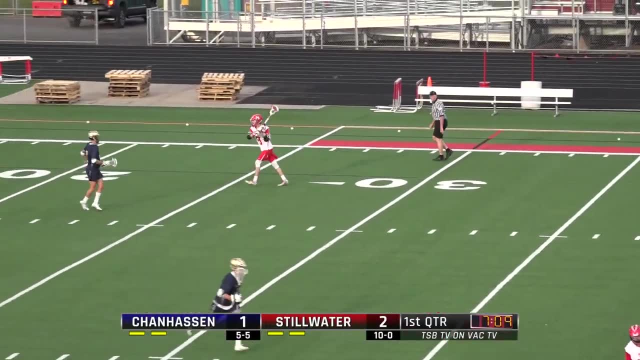 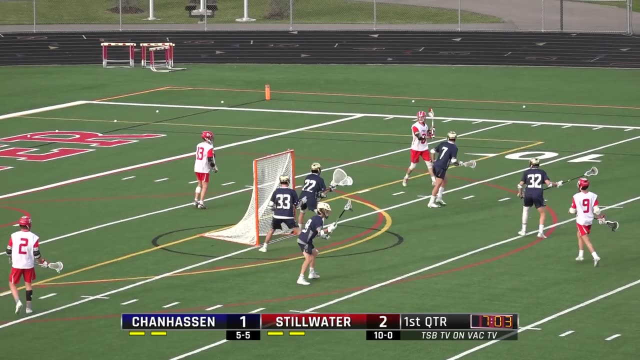 And it looks like Long will head out. Stillwater was taking a peek there, But they'll wait to get their offensive rotation in position. There's Cody Berger. Cody Berger's been playing great this season, Mike, He's one of six. 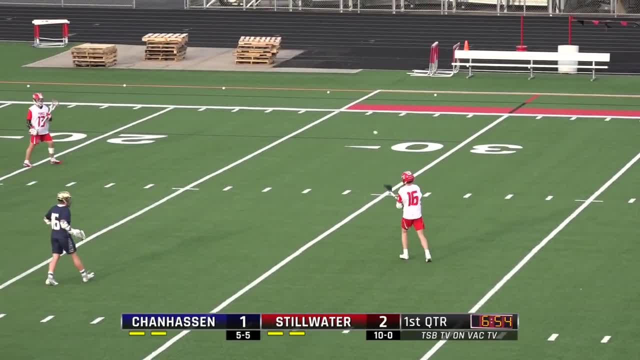 And he's going to get it, He's going to get it, He's going to get it. He's one of six Stillwater players in double digits with 13 goals- He and Quinton White, not 20-goal scorers. 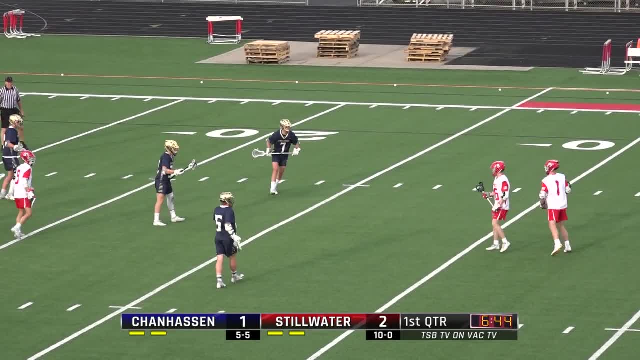 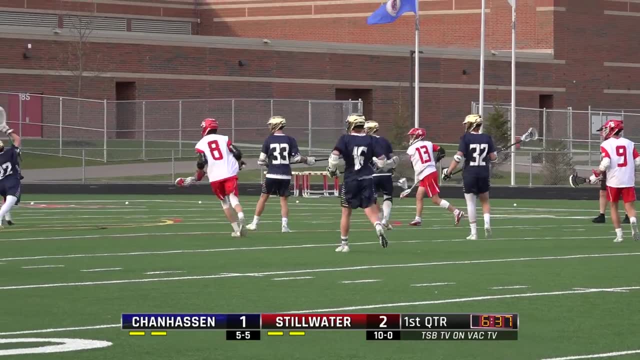 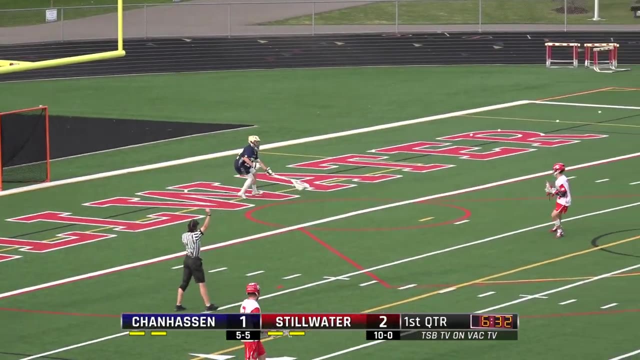 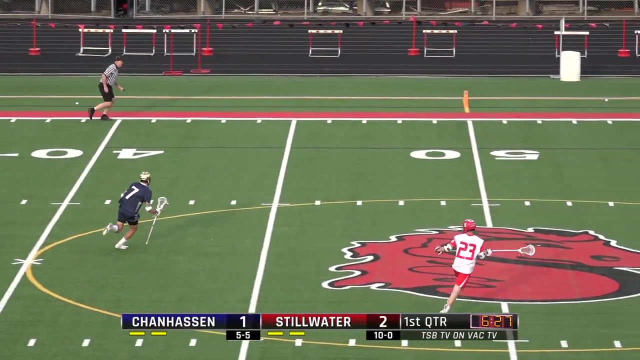 But that doesn't invalidate what they have done on offense Summary: sends it over to White And then White side-armed it. Chanhassen was closest to the ball, So the Storm will pick it up And if you're the underdog, like Chanhassen is, this is what you're looking for. 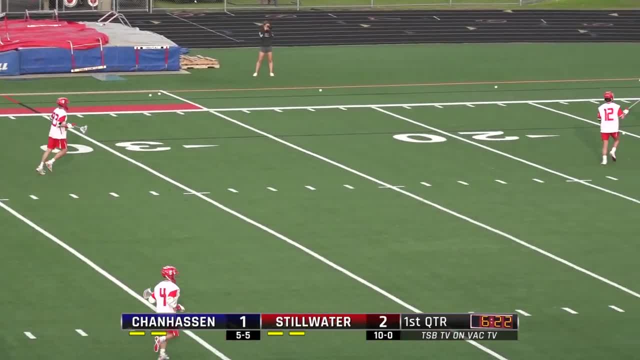 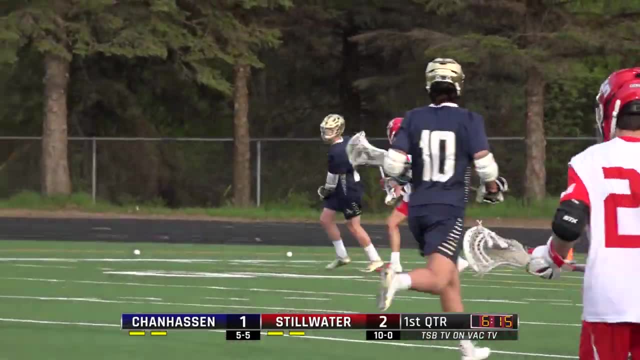 You want a good quarter, a good half, where you're hanging around, You don't want to let the Ponies go on that big run that has demoralized so many teams this season. Oh, absolutely, Mike. We sent them a rack up of double-digit scores in the first quarter. 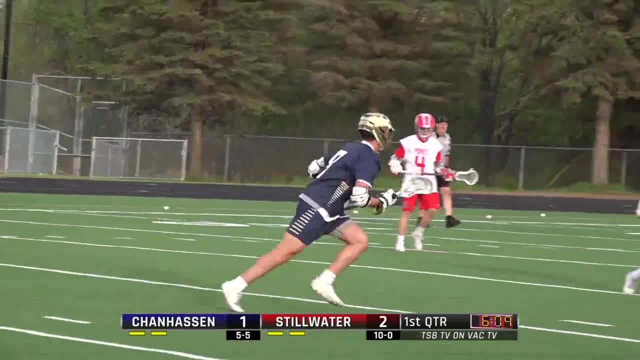 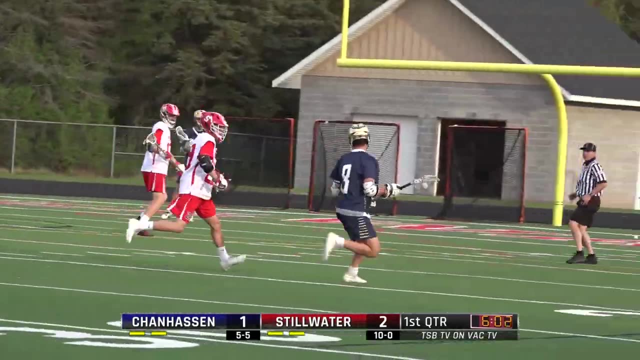 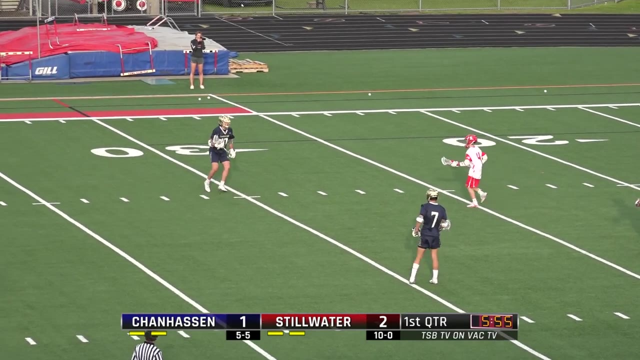 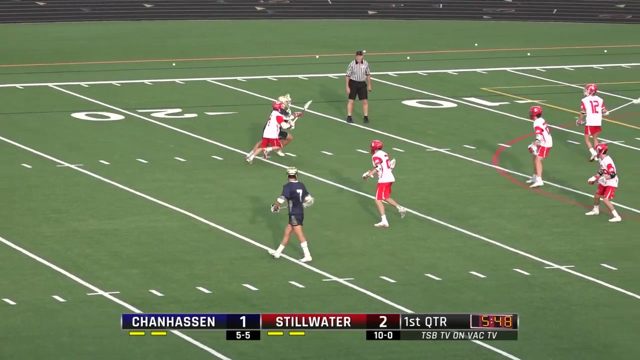 Only the other team's got to fight uphill the rest of the game And Chanhassen doesn't want to do that. Chanhassen 5-5.. It's been an interesting season for the Storm. They've won their last two games. 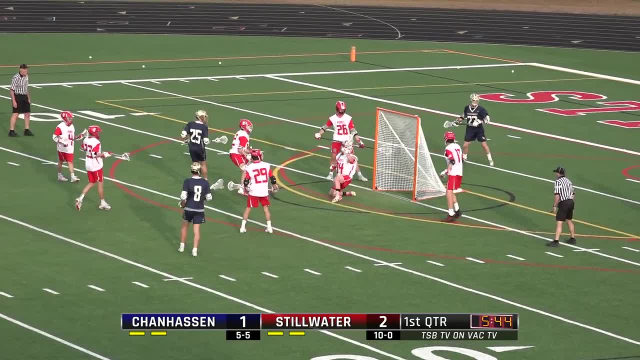 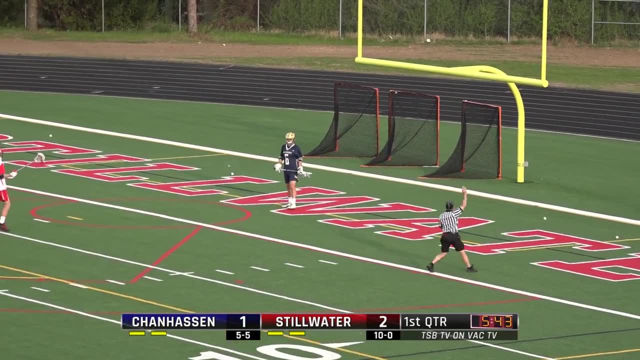 They beat Wayzata 9-4.. And then blank St Louis Park, 19-0.. They lost to Benilde St Margaret's, the number three team in the state, 9-4.. And they beat Mata Bidai by a single goal: 10-9. 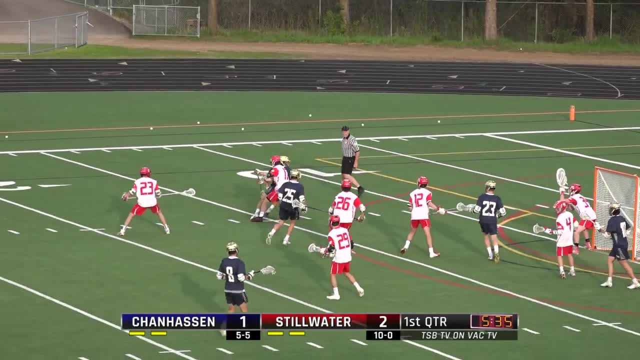 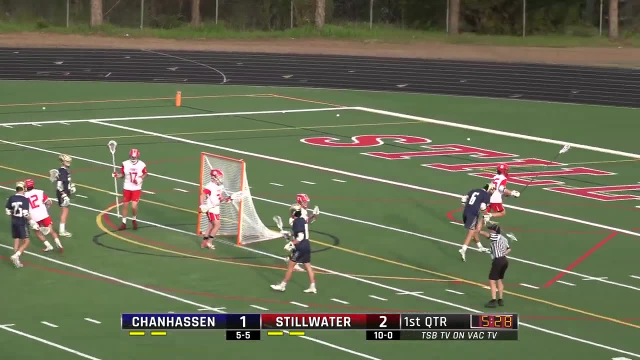 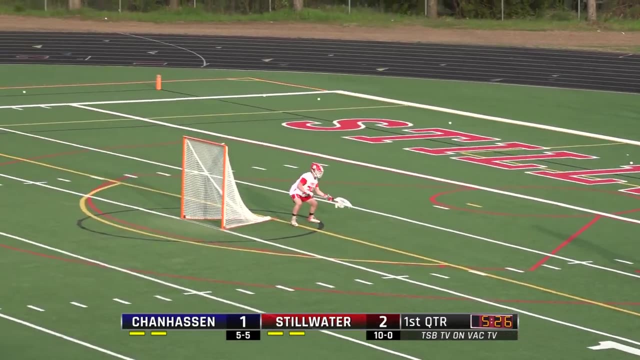 So this Chanhassen team a little unpredictable. They haven't been blown out a lot, But they haven't won as much as Stillwater has. They tried to quick-sit from behind And that's going to be Stillwater ball, with that shot by Tyre Christensen going off the mark. 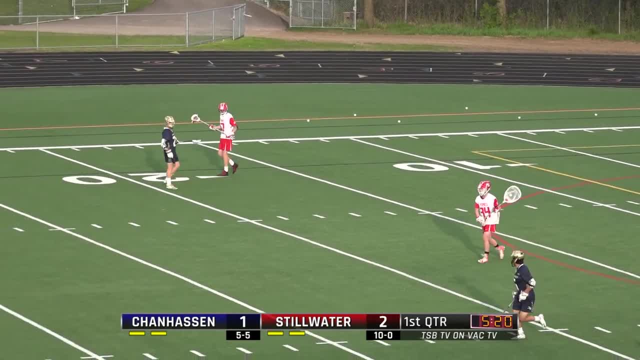 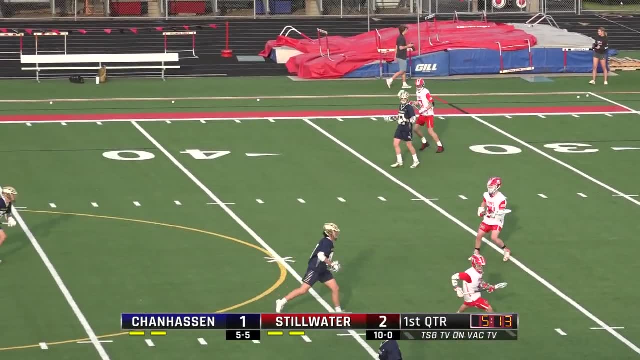 Gunnar Ehren. still, you know, keeping a tight lid on that goal. He's not letting much through at all. Chanhassen's worst loss, if you're wondering, was 19-11 against Eagan. So it's a team. 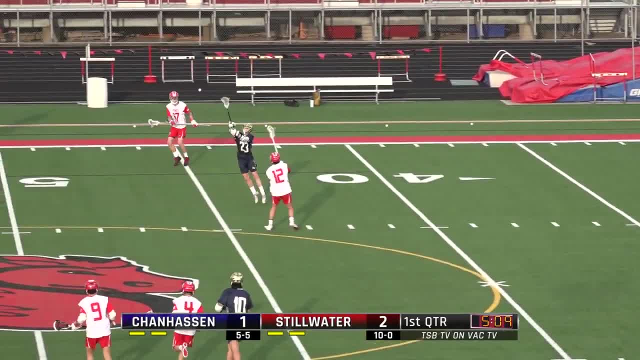 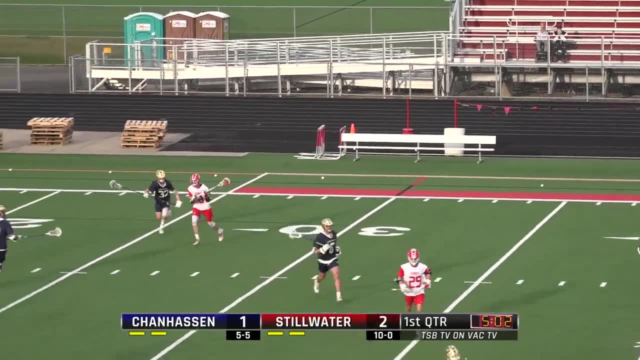 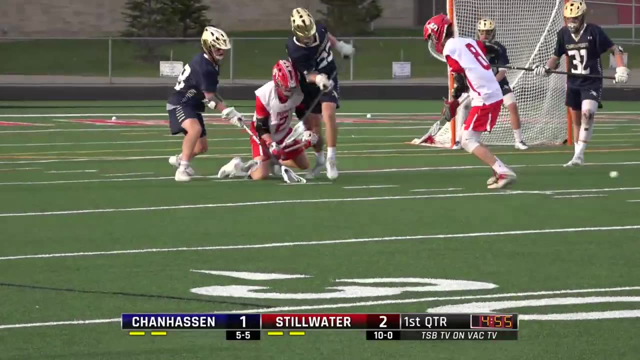 It's a team that can win by a lot, lose by a lot or fall somewhere in the middle Stillwater. all W's Here's Evanson. a big reason for that Stumbles Nothing called Chanhassen tried to strip the ball. 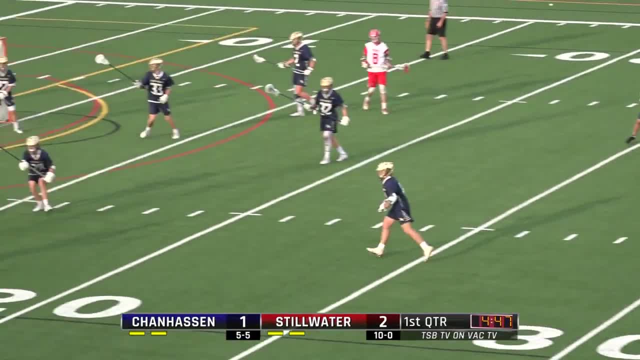 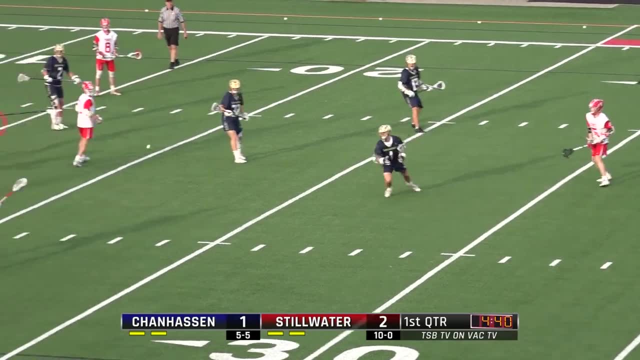 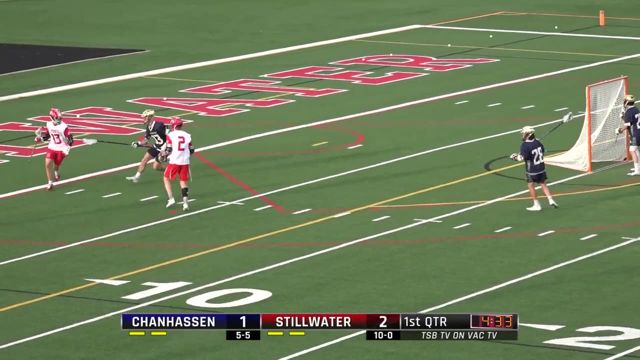 And nice recovery on the part of Joe Stengel. Here's an interesting factoid about Stillwater. They have never scored more than 17 goals in a game And they have not scored fewer than 13.. Every game this season they've averaged or they've hit the mid-teens. 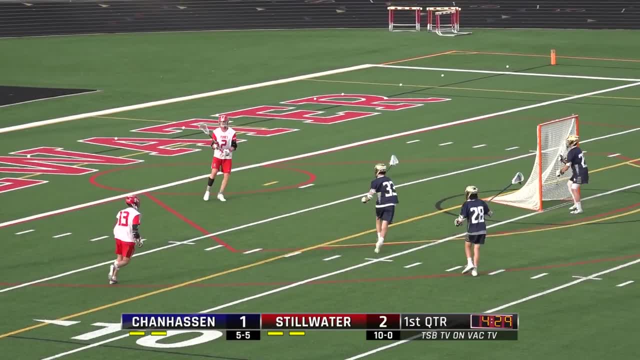 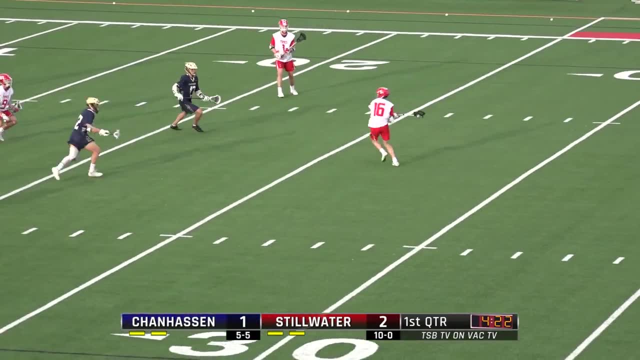 It's not surprising to see because of the amount of talent they have and how well they play together. Not when you look at this team, But that's a rarity, as Rathie gets the save. on summary, You see a lot of talent in this team. 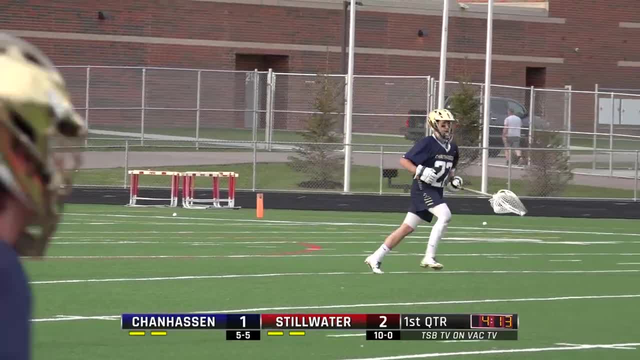 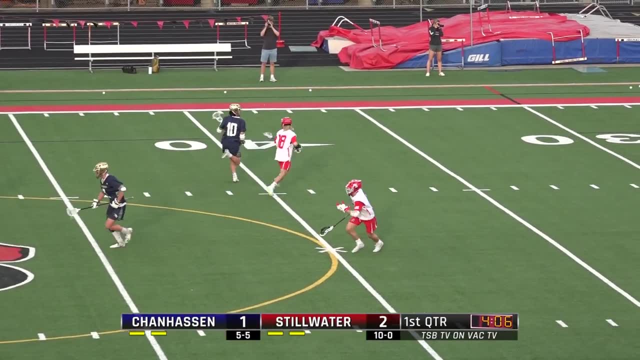 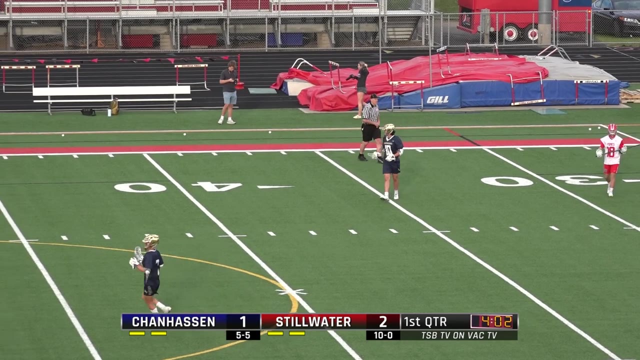 You see a lot of teams that will put up 20 goals in a lopsided game, Or they may have a single-digit performance, like Chanhassen has had a couple of times. Not Stillwater, They can score and score big. Chanhassen calls timeout. 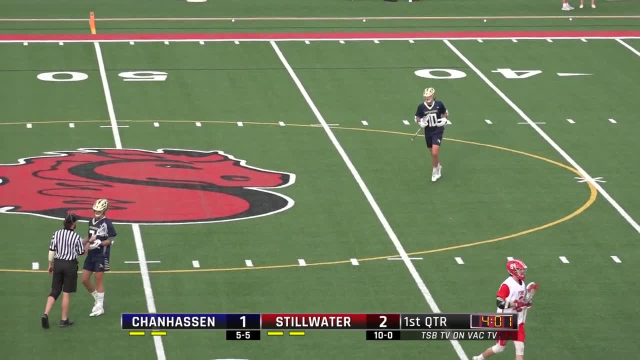 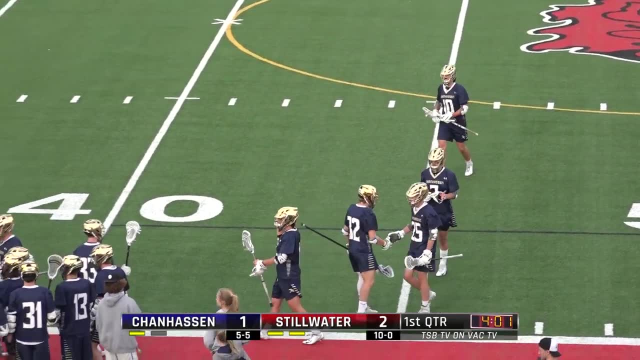 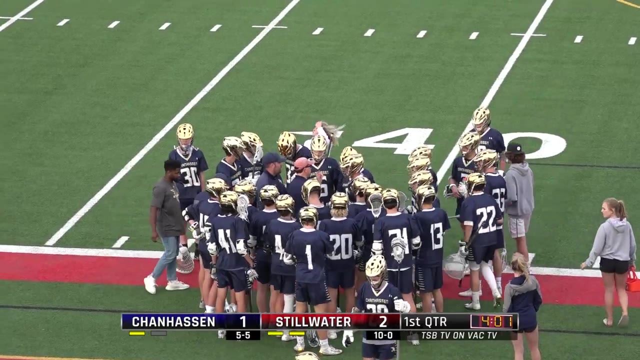 Their first of two and a half 4-0-1 left in the first quarter. What a nice close game. so far They've been giving up a lot, Both teams trying to make something out of nothing, Some really hard outside shots being fielded by the goalies. 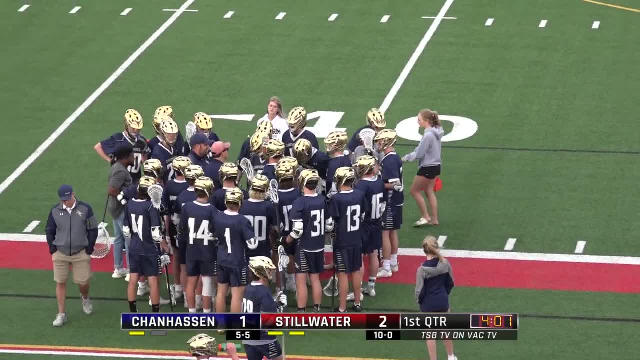 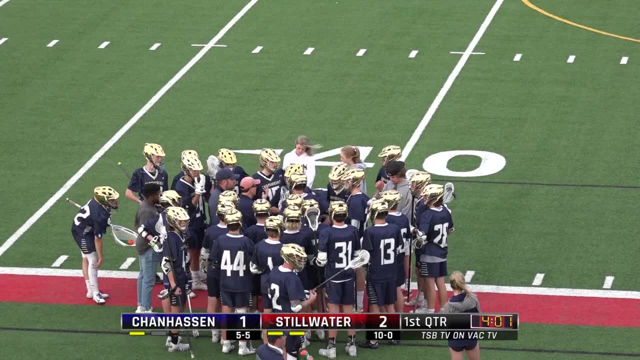 So if you're watching this on tape delay on Valley Access channels. there are no more regular season live broadcasts, But earlier today this was pretty big news for you, Robert, and I'm sure for everyone here: Valley Access channels. If Stillwater makes the section final for La Crosse. 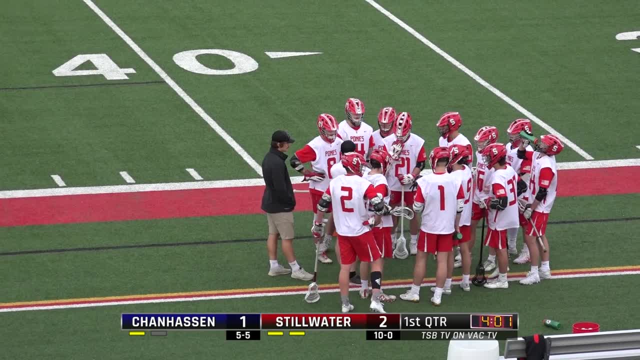 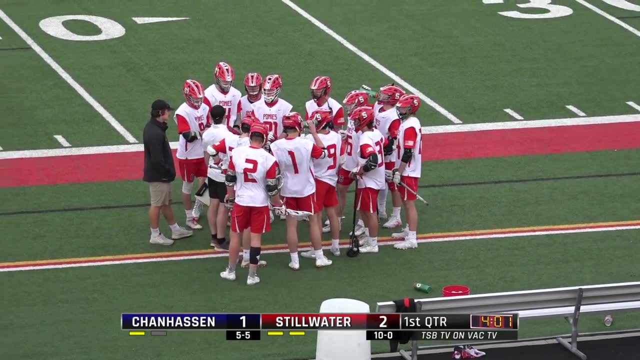 we'll have live coverage of both the boys' and girls' section championships. They will be held at White Bear Lake. I thought you'd be more excited about that. Well, I'm confused. I thought you said they were going to be held here. 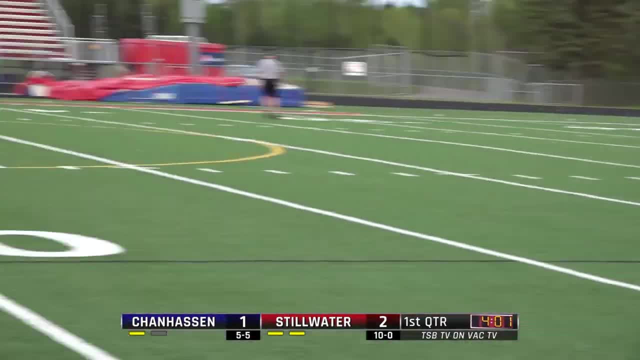 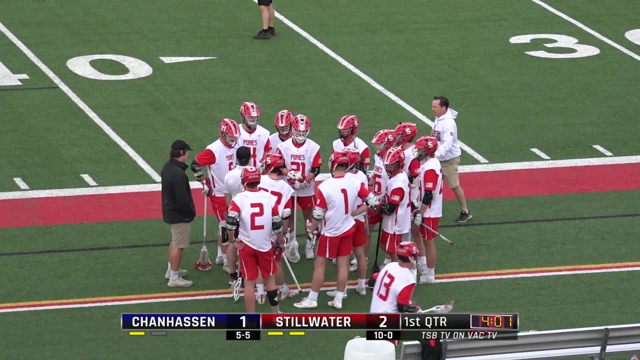 Or maybe they are. I thought they were a neutral site. But Valley Access channels, wherever it is, will be at the section final. Well, that's Valley Access channels for you everywhere, doing everything for everyone in any way possible. And that could be a busy night for the Valley Access channels. 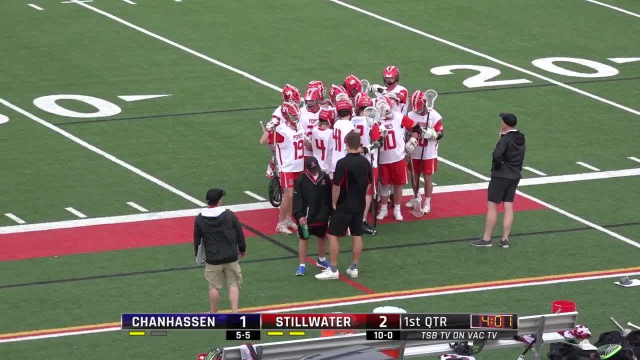 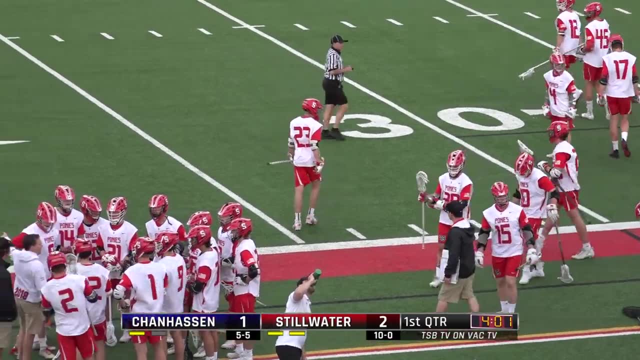 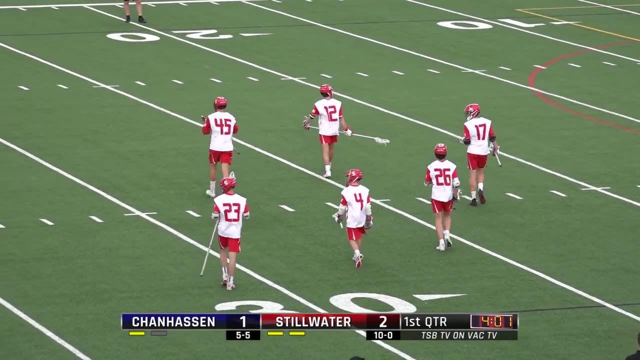 Because that same night the Stillwater baseball team could be playing for another section title over at CHS Field. Well, we'll just have to send one of the ten VAC crews over to whichever venue needs them most. Well, we've been at two places at once before. 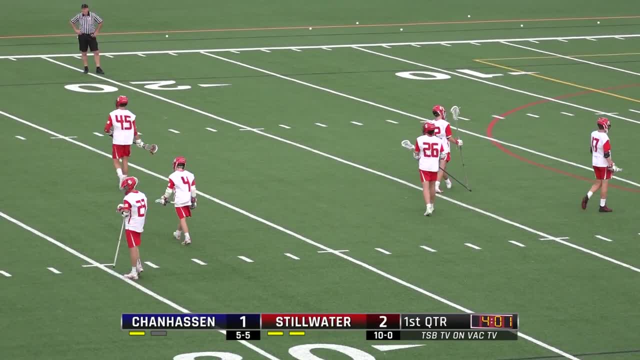 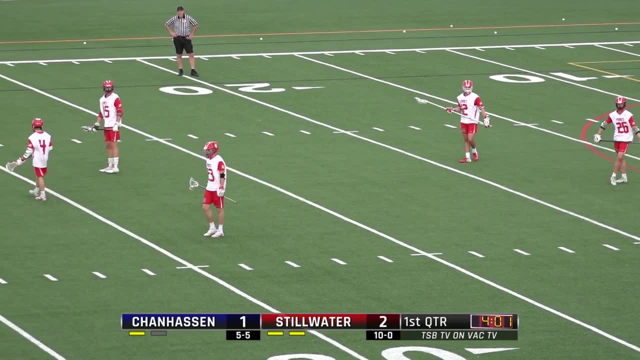 We could do it again, But an exciting opportunity. It's the first time we will cover a section final live Again, that's if the Stillwater La Crosse teams make it. The boys have a really good chance of doing so. Looking at their section, the girls have a good chance as well. 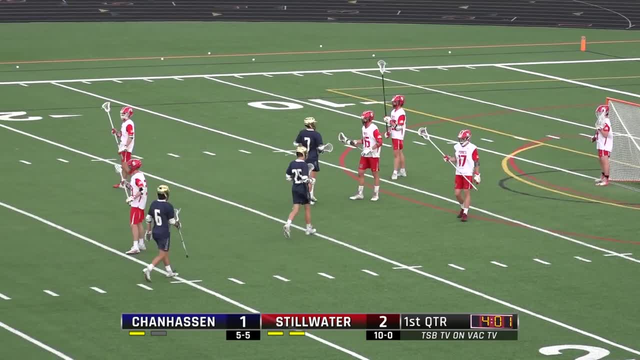 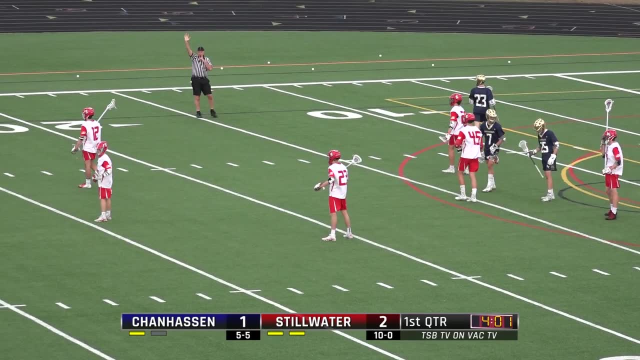 They're in the top ten in the state rankings And they've made state the last eight years in a row, So there could be a lot of ponies in spring state tournaments this year. I've been able to see a lot of winning so far on the girls' and boys' side. 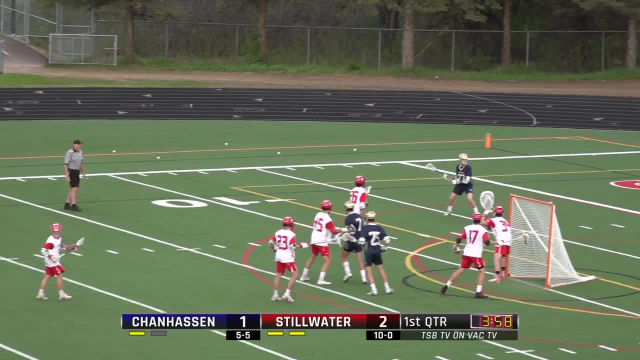 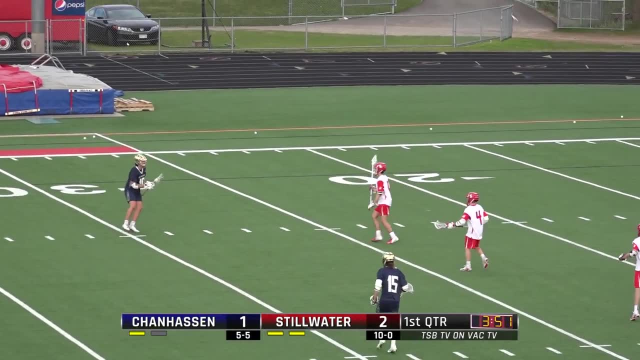 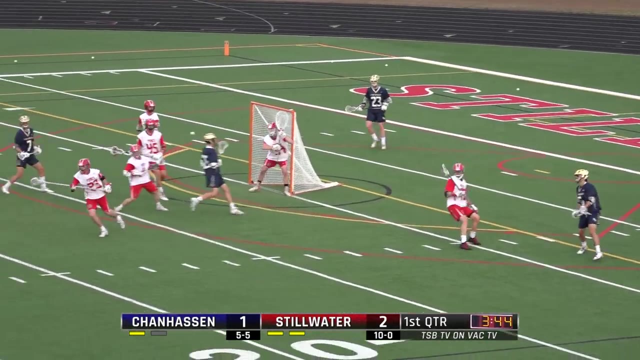 Whenever I watch them win, it makes me very hungry. Ted and I have joked about the problem we have, or the downside of all of this, is that we're often covering teams deep into the playoffs, Whether it's volleyball, soccer, La Crosse, basketball this year. 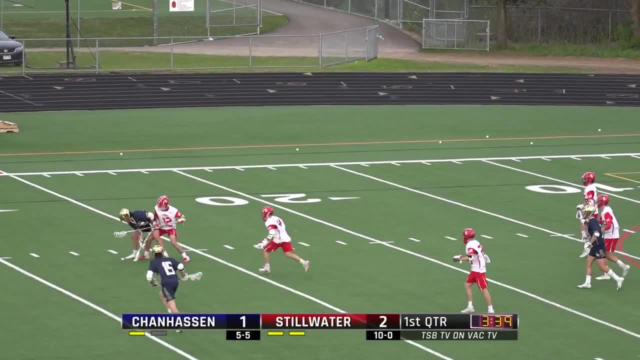 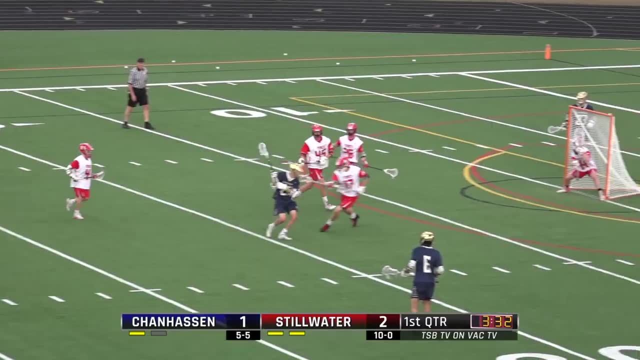 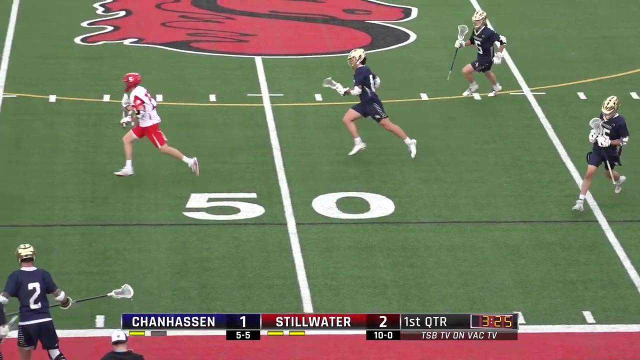 Things don't end in the regular season. You have to plan for at least one state tournament. run Chanhassen with the ball. They've been holding their own against Stillwater. An off-speed one-hopper aren't read that easily. His lead pass a little long, but recovering it is been long. 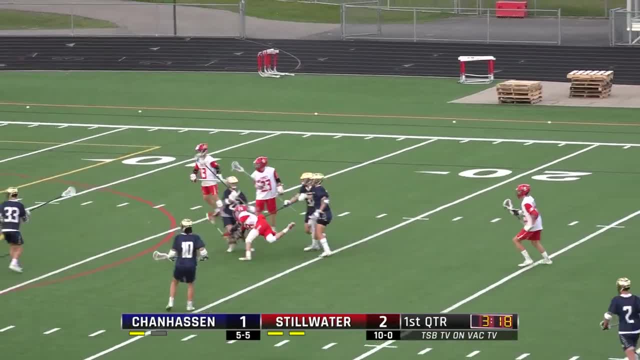 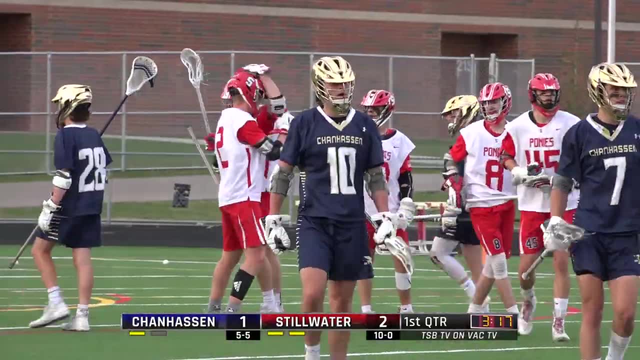 Evanson to Long Long couldn't handle it. He had an opening in the middle, But Stillwater recovers for the goal. The ponies pick each other up. Cody Berger cleans up the mess. Wow, Usually when that happens, everything unravels. 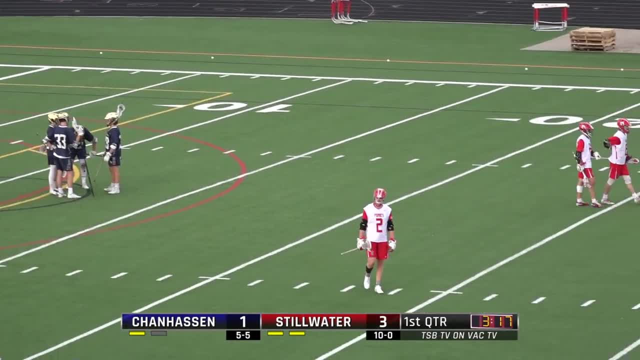 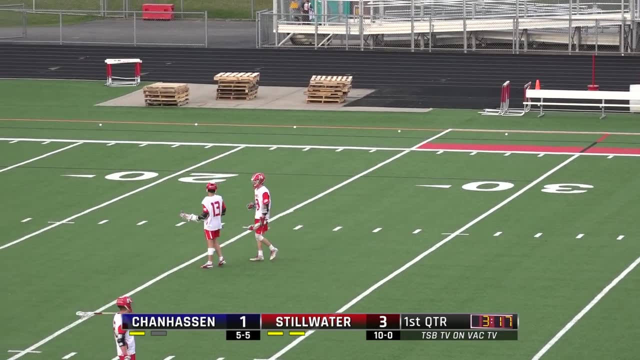 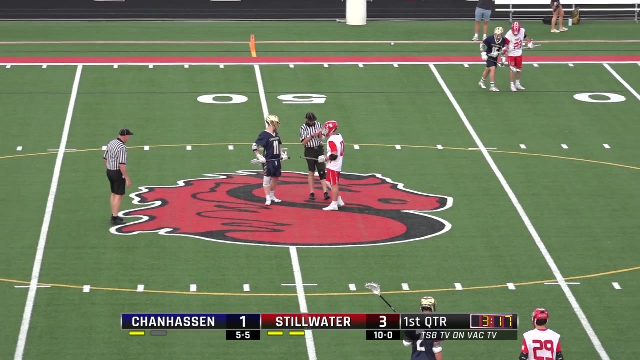 But there we saw the ponies do some cleanup work. That's not what they're known for. but Tom Ho will take it. Cody Berger with his 14th goal of the year That makes it 3-1.. Robert, that's the kind of goal that could not necessarily pick up this team. 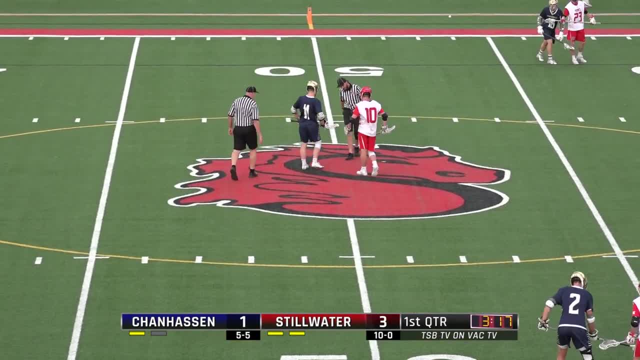 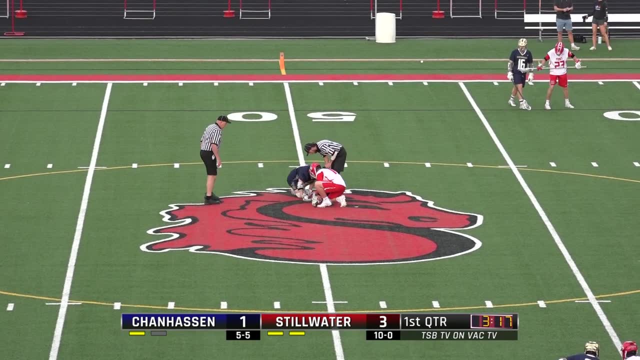 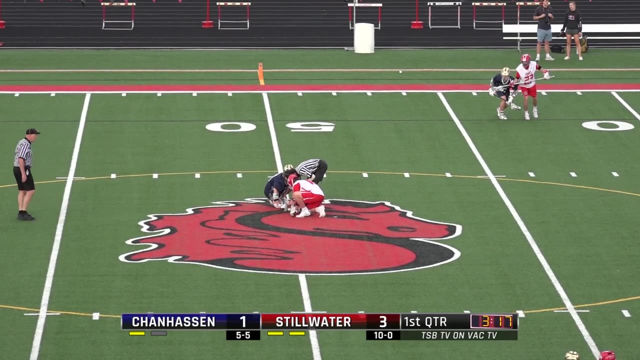 They don't really need confidence or momentum but to turn a broken play into a score that could help them build that coveted first half run. we know them for That was amazing how they gave up possession twice in one short span of time and yet recovered the ball enough to get a shot on the inside, a good, hard shot. 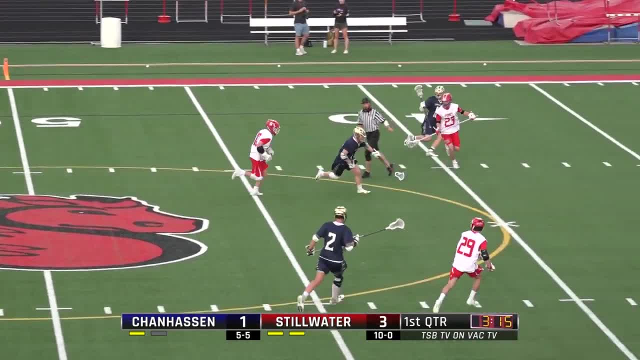 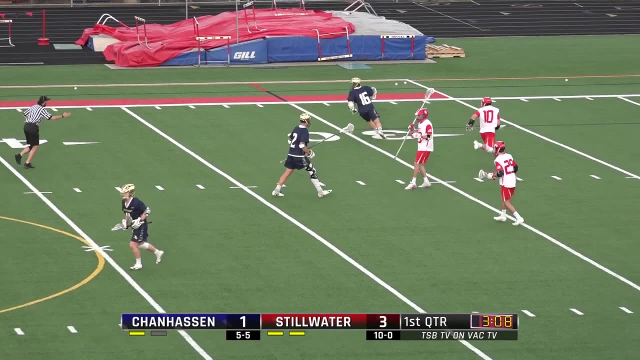 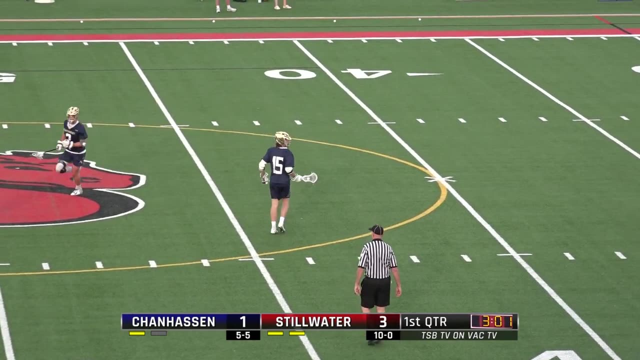 It doesn't happen where you get a second chance like that. You know Evanson Had Ben Long in his sights and the perfect one-timer opportunity. Long couldn't handle it. Cody Berger, right place, right time. Three minutes left in the first quarter. 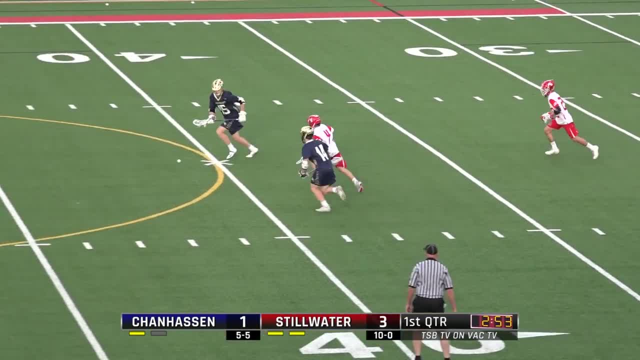 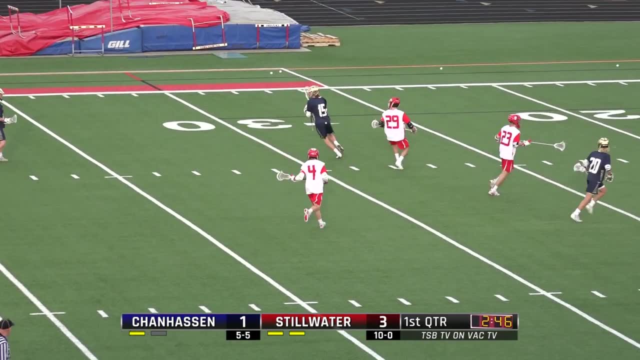 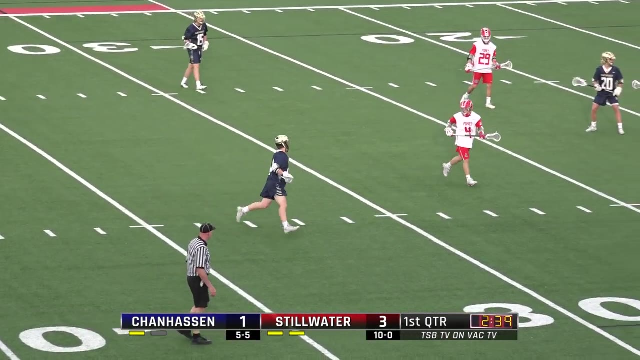 3-1 Stillwater over Chanhassen. Stillwater has never gone undefeated this long in school history And There's good reason to believe they could end the regular season undefeated. Of course, the parents don't want to think about section or state titles. 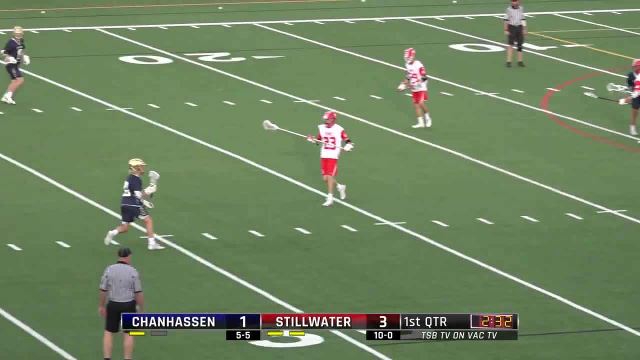 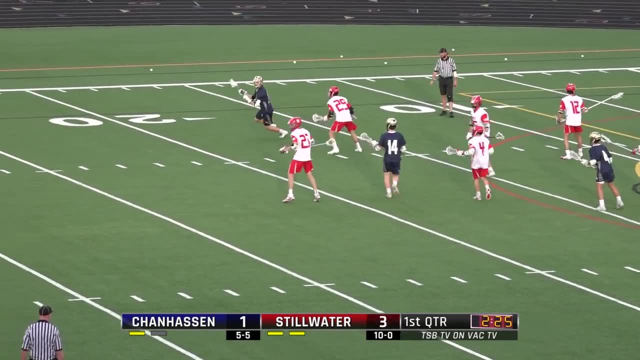 They know it's single elimination so you've got to play one at a time and that section round figures to be a little tougher than the regular season. but you have to like the wave of momentum Stillwater's on. They were good last year. 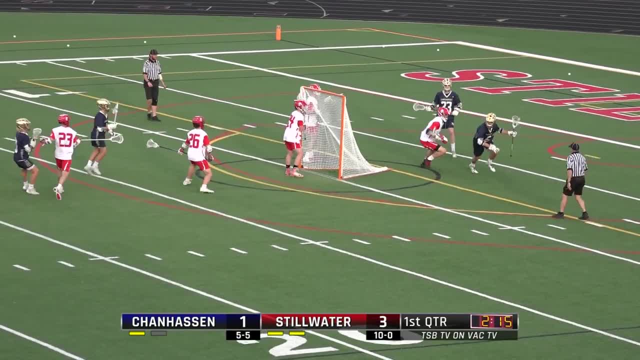 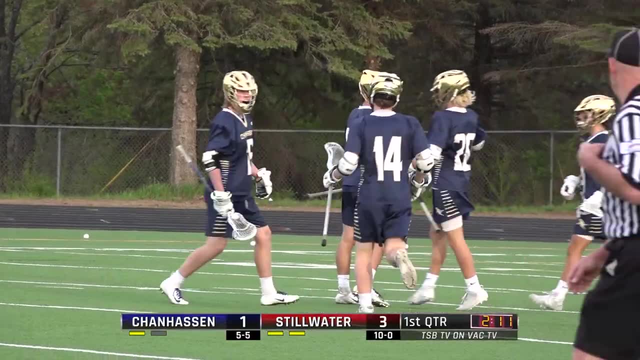 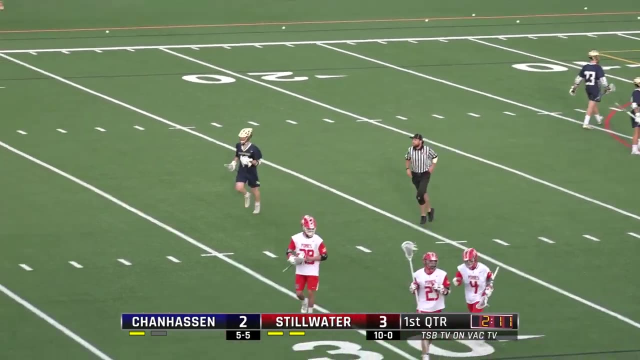 They've been ferocious this year as they have ascended in the state rankings. Nice move by Chanhassen's Hunter Holcomb With a little fadeaway move and that gets the storm within a goal once more. It just goes to show you that it doesn't have to be a hard shot. 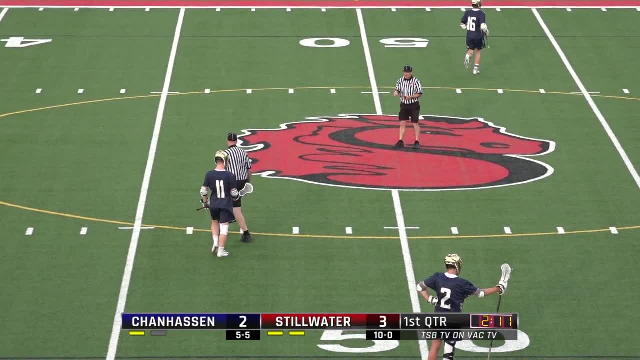 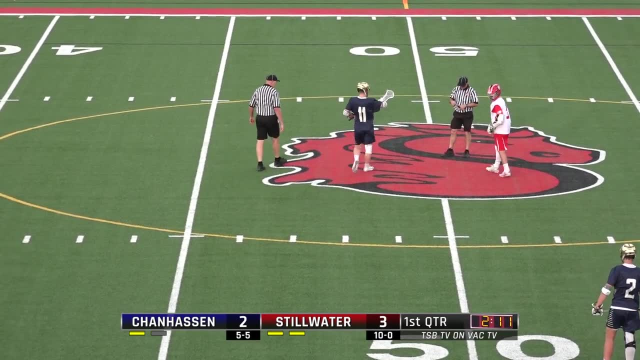 It just has to be one that fools the ball. It's not easy to fool Gunnar Ahrens, but he did not get the best of that shot. Holcomb picks up goal number 21. And he is the leader in scoring for the Storm. 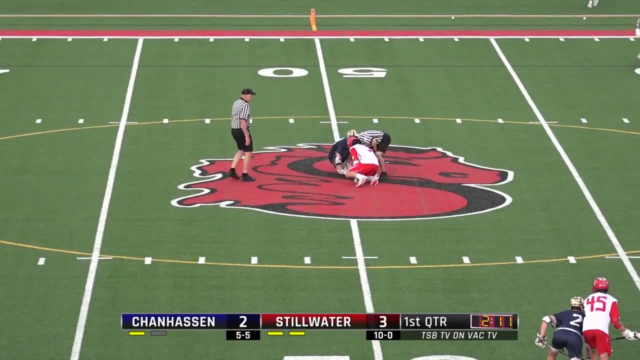 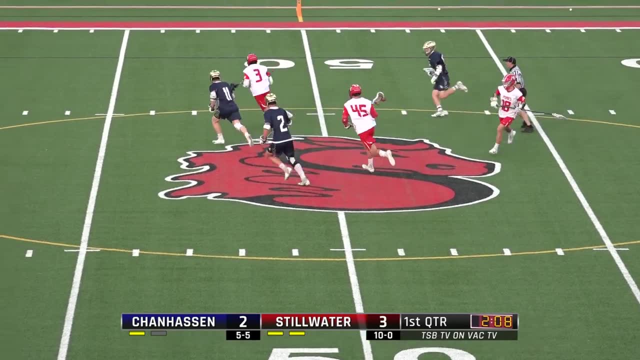 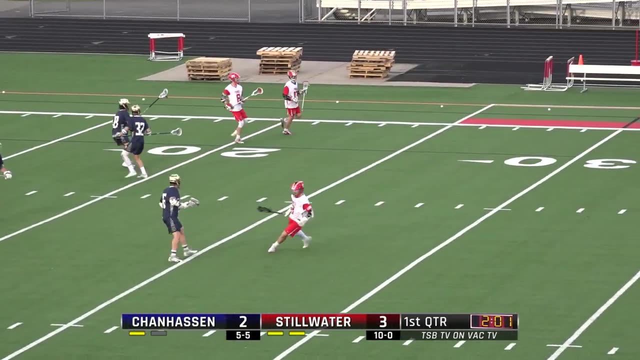 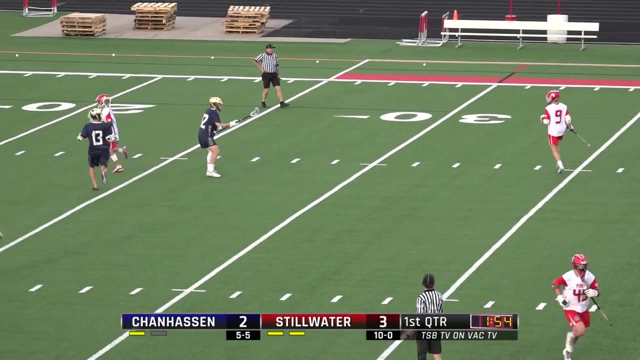 And we haven't talked about him yet. but Ty Thorsen, as we noted, seventh in the state entering this game, started the season with four straight hat-tricks. The Ponies win the face-off And we've got some noise. 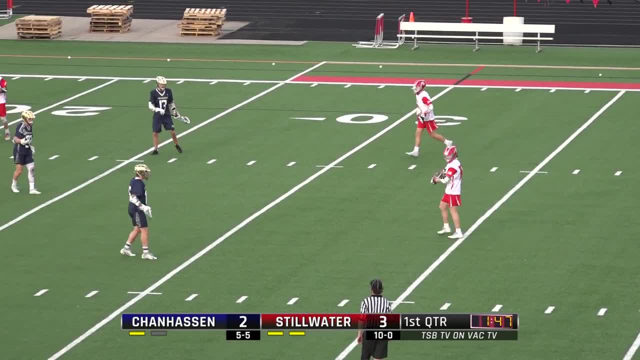 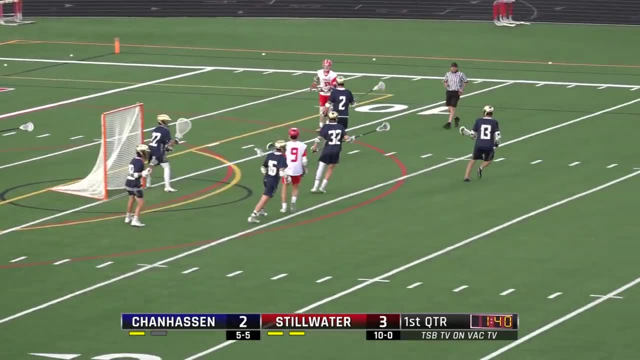 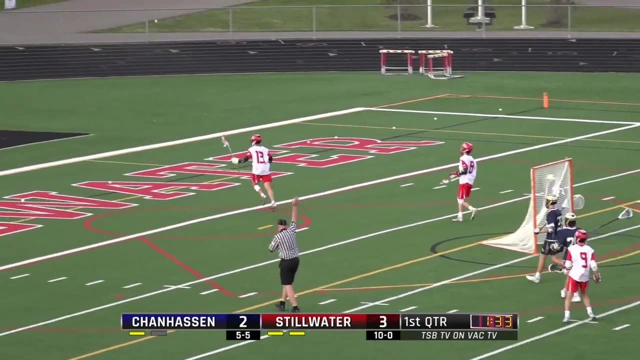 I think it's the wind and I think we've got some young fans also causing a ruckus. Evanson will dump it over to Quinton White Stillwater on the cycle play. Evanson centering pass 14!, 14!. 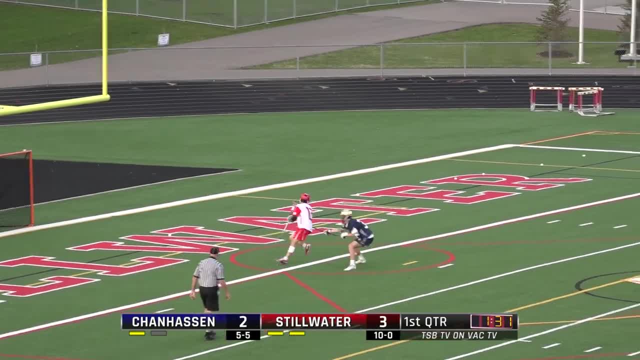 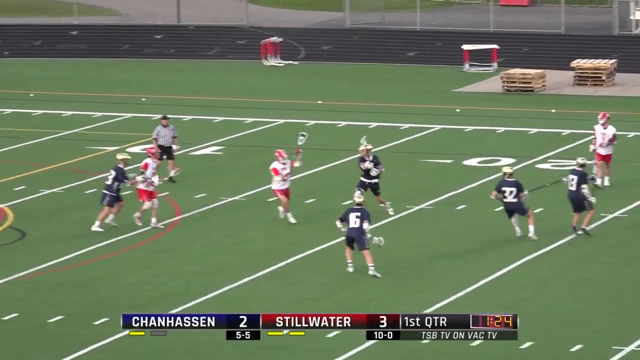 Joe Stengel the right idea. I think Rathie got a piece of it to deflect it out of bounds. Stillwater hangs onto it, White. He set up a few folks. Summery goes up the middle and Stengel can't handle it. 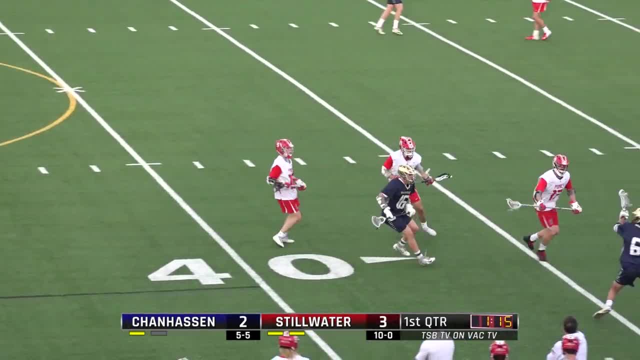 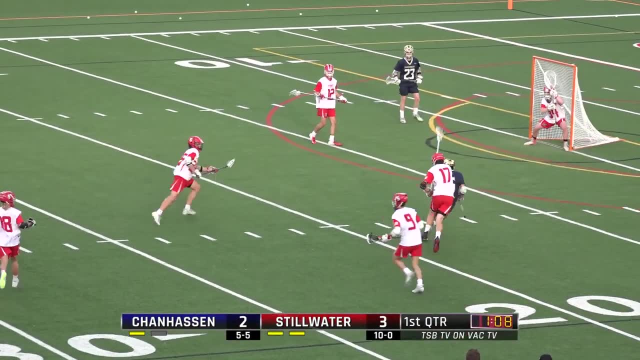 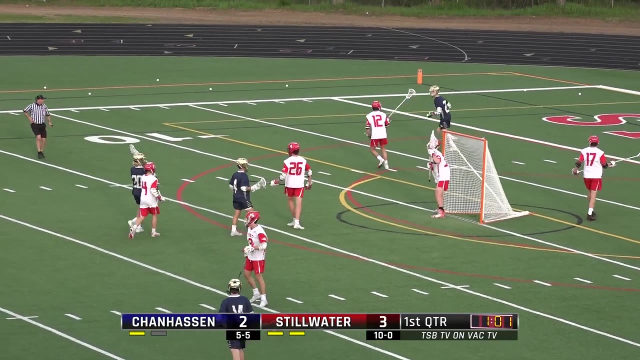 An opportunity for the Storm, but Stillwater putting a lot of pressure. We haven't had any penalties. yet There goes Stillwater playing some pretty physical defense. Hunter Holcomb breaks through Mops not to go for it. He'll back off for a reset. 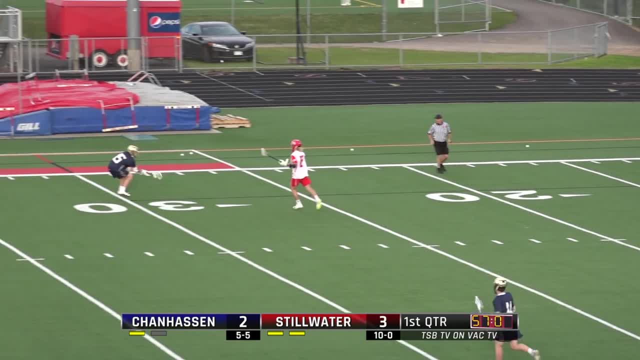 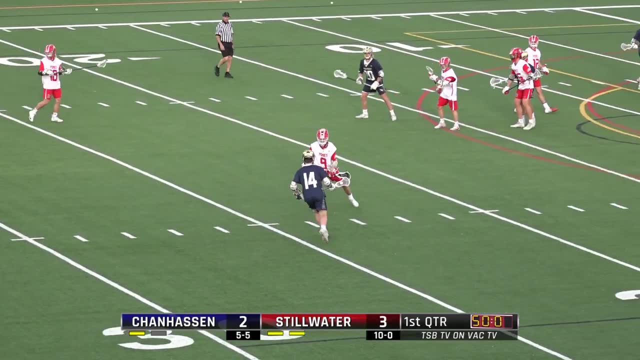 and Chanhassen will run a cycle of their own. with less than a minute to go in the first, I'll tell you this: Jonathan Junker, the head coach for Chanhassen, has got to take some pride in what he's seeing out of the first quarter. 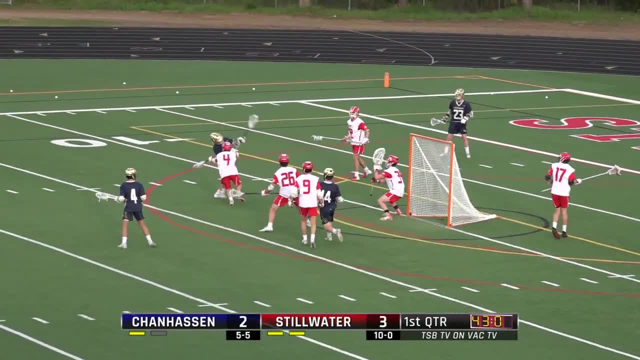 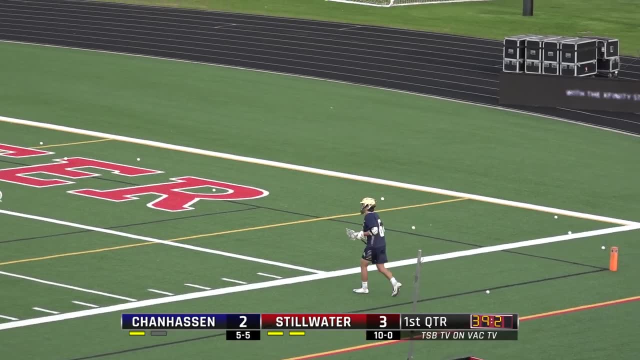 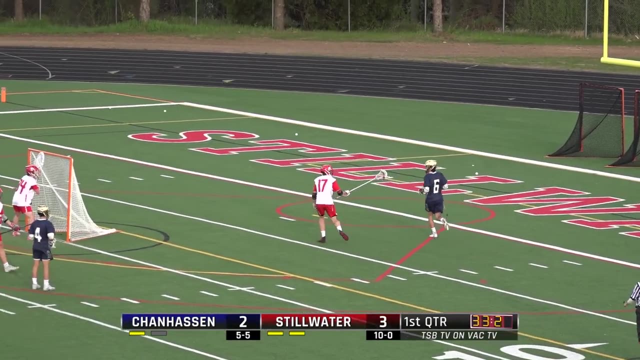 The Storm have not allowed Stillwater to go on that patented big run of theirs and they almost tie it up. Blake Whiteshott goes off the mark. It will stay Chanhassen ball with 39.2 on the clock, Stengel. 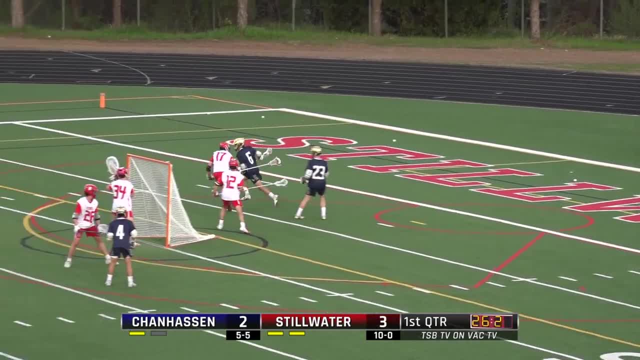 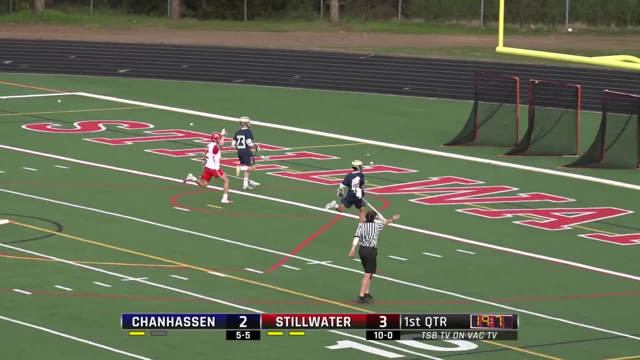 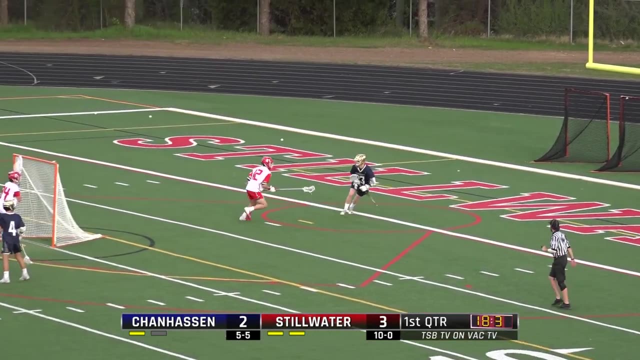 Stengel, Here's Holcomb Runs into a wall, Fires Ahrens, Bats it away with his stick. Wow, a lot of good action inside Chanhassen trying to find that inside seam to get a good shot. but they're really being closely watched and boxed out by the Stillwater defense. 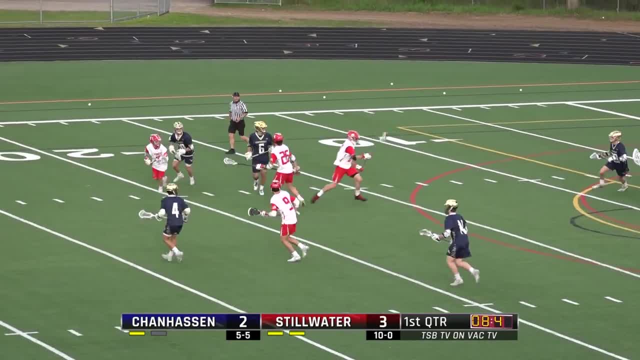 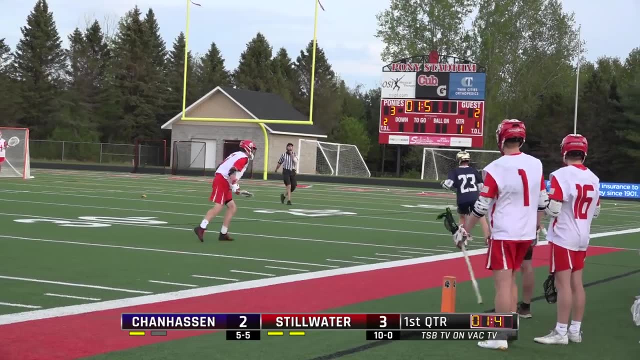 They have 11 seconds And losing his stick is Blake White. so a strong defensive front by the Ponies, A big stand and there's going to be our first penalty of the game. It will go against Chanhassen. There won't be enough time to do anything with 9 tenths on the clock. 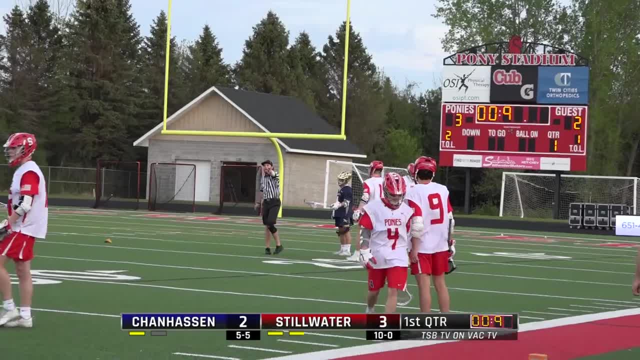 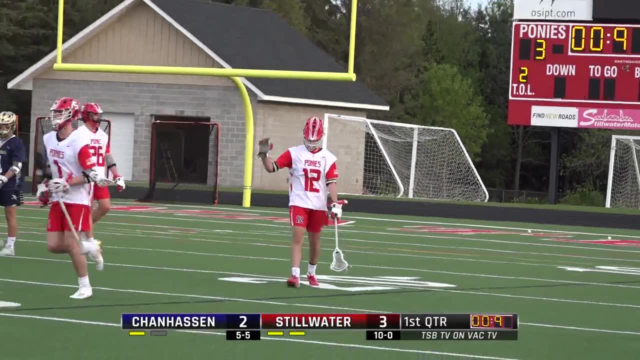 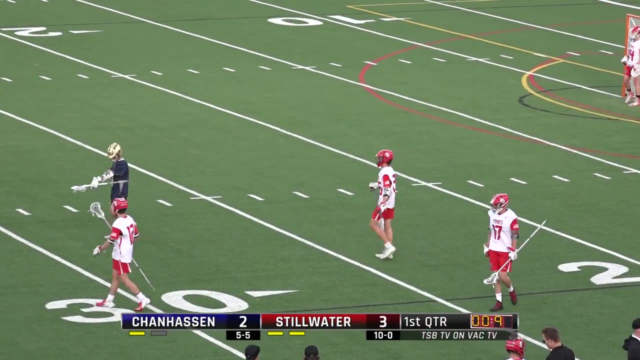 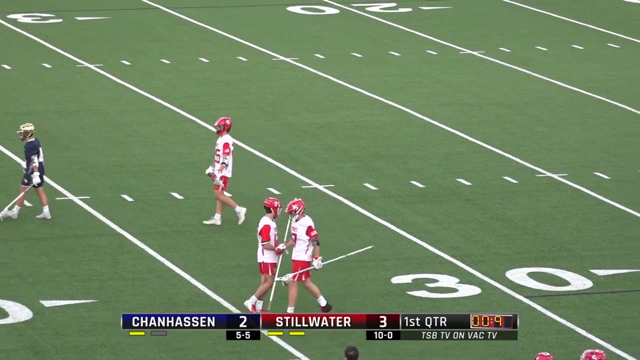 The first quarter will end with Stillwater up 3-2, but the Ponies will start the second quarter with the man advantage, With the penalty going against Cal Davis. Again 9 tenths of a second on the clock, so not enough time to get a shot off here. 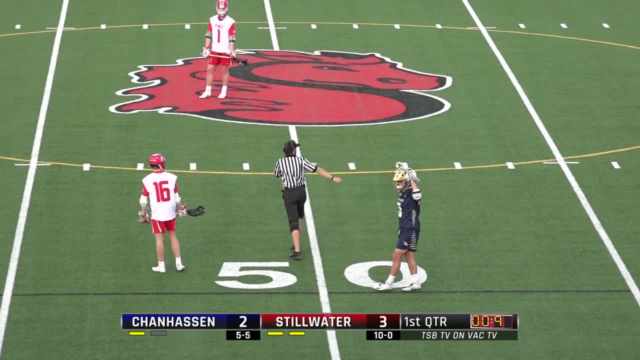 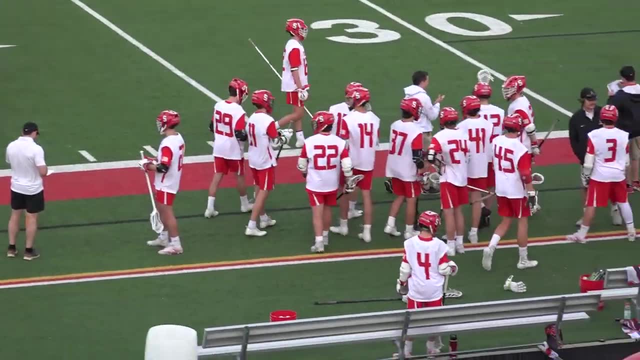 Slashing is the call and a big power play opportunity for the Ponies to start the second quarter. Nice job by the Stillwater to get Cal Davis off the field for a couple minutes. He's one of the top guys for Chanhassen. 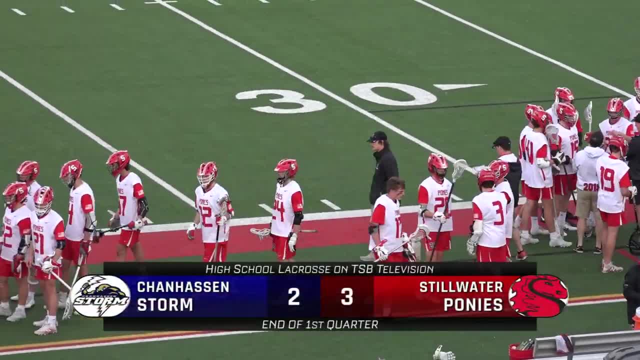 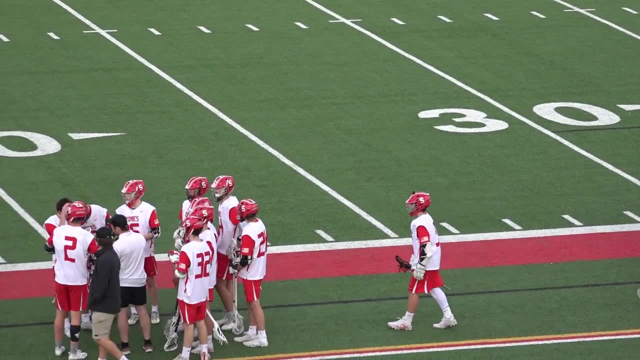 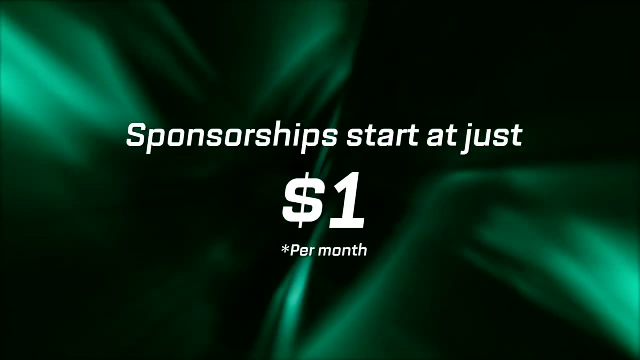 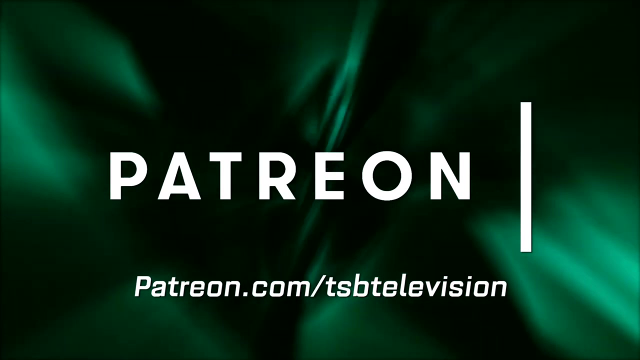 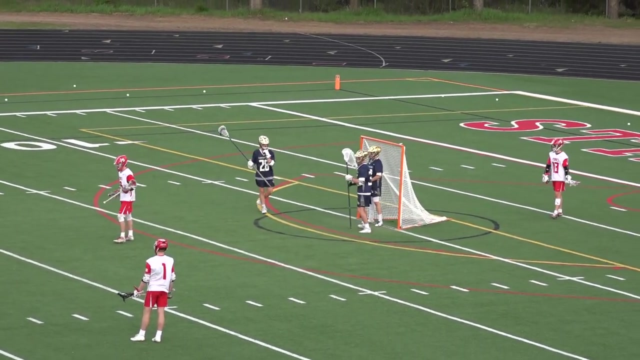 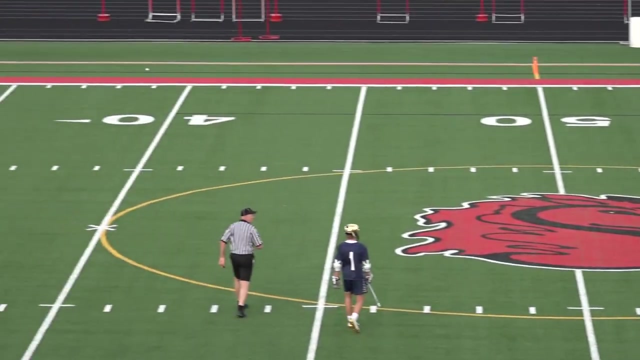 And an impressive job to keep Chanhassen off the board late in that first quarter. We'll take a quick break and bring you quarter number two. You're watching High School Boys Lacrosse- Mike Beaton and Robert Critta with you As the Stillwater Ponies lead the Chanhassen storm 3-2.. 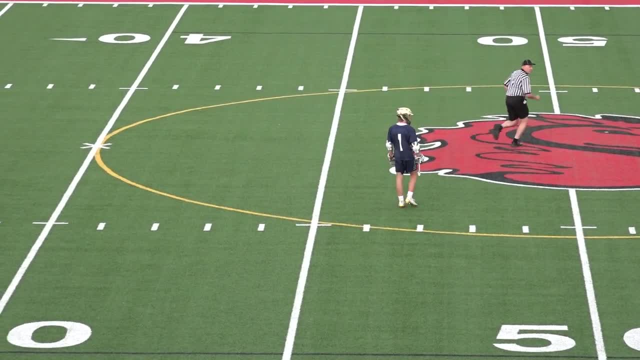 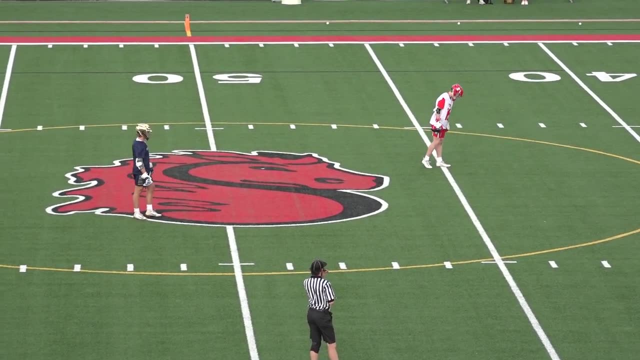 Chanhassen celebrating 10 years of operations as a high school, Taking up shop after Chaska overflowed in their student population and now both schools are 4A Meccas, Maybe not as big as the University of Wysetta. 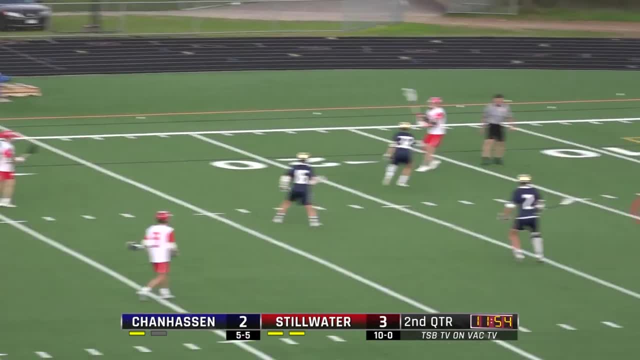 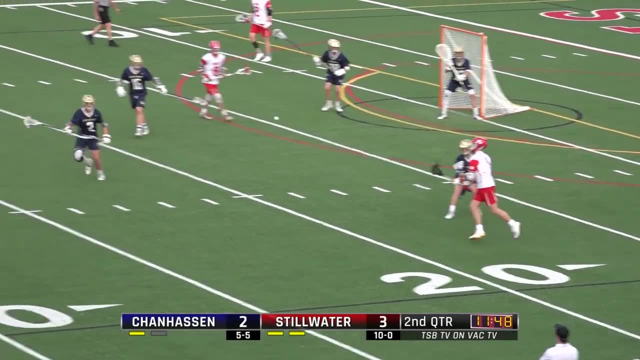 as we like to call it, but Chanhassen, one of those schools trying to develop an identity. They have never made state in lacrosse and they would be an underdog this year. They're in the same section as Minnetonka. 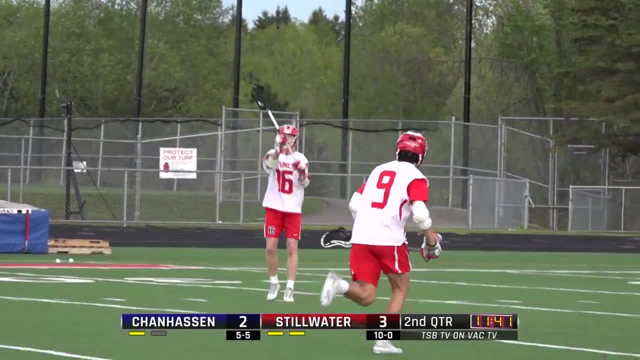 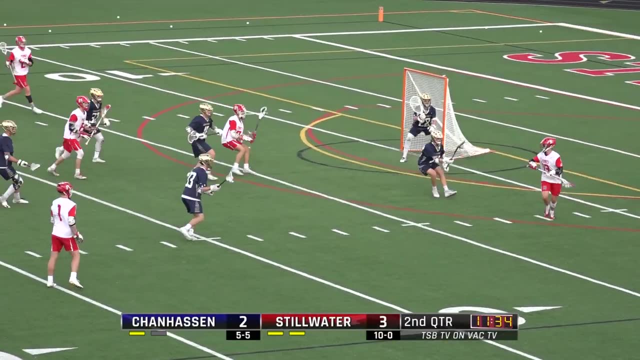 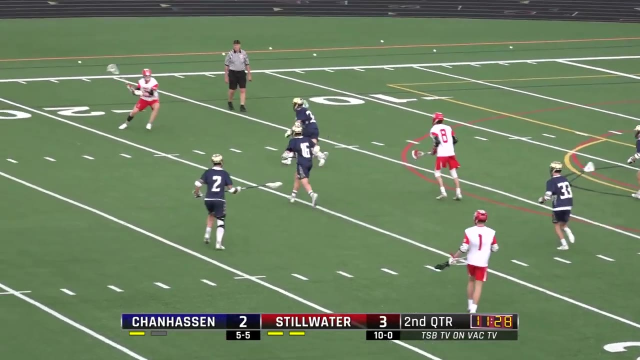 who has been number one most of the season And again, if Stillwater stays undefeated, would probably drop to number two, with Tonka losing to EP Ponies on a one-minute man advantage after a slashing penalty. It was called on Cal Davis. 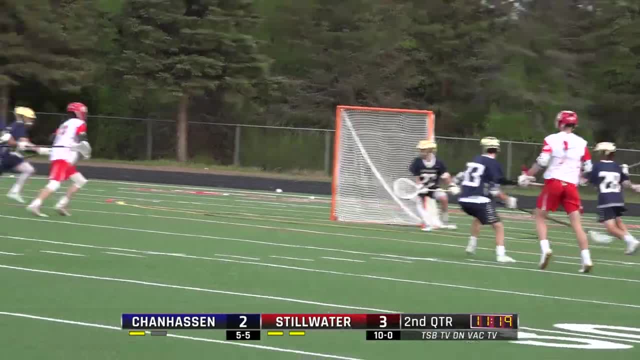 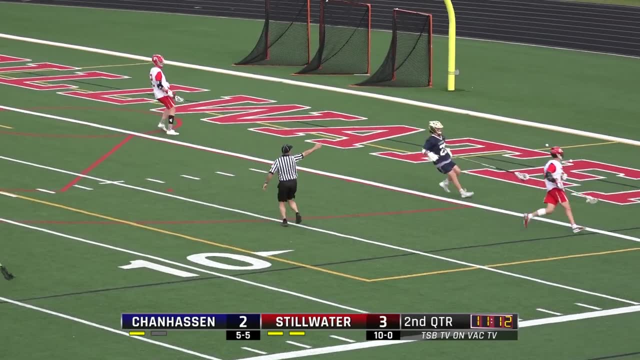 Chanhassen did a good job sealing the Ponies out, except Tyler Thurston had an opening Big save by Rathy Ball's loose. it's picked up by the Ponies. It's a foot race. It's won by the Ponies. 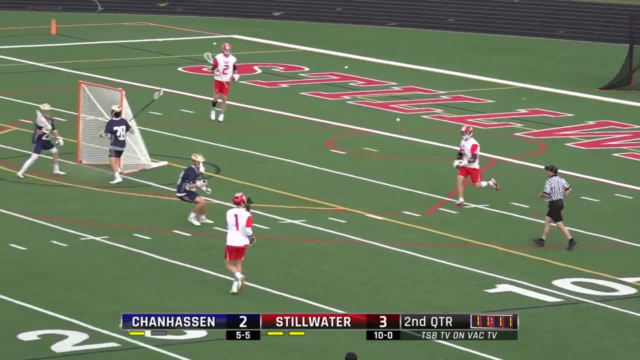 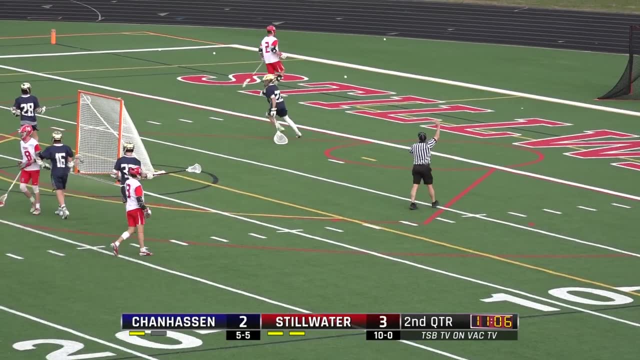 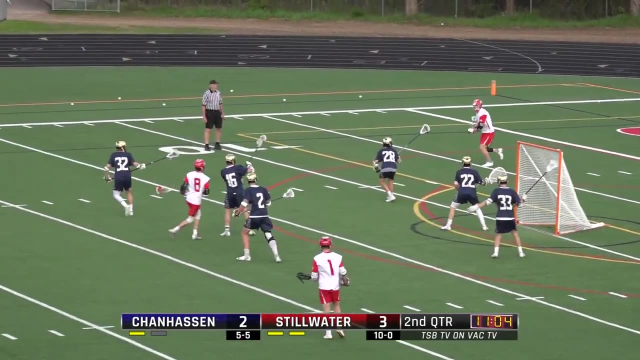 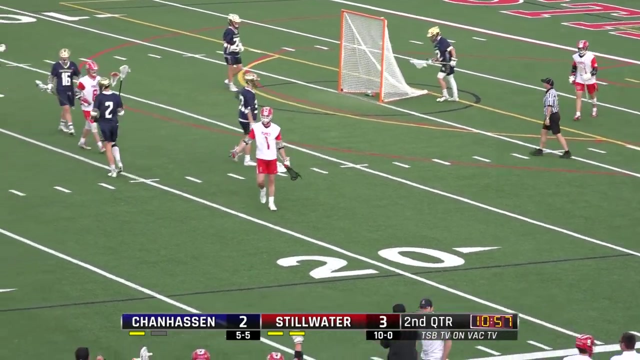 Evanson almost cashed in on the rebound Boy. that was a hard shot by Ty Thurston. Another hard shot by White Stillwater ball Ponies looking to assert their authority here. Thurston this time finds his target. And Thurston, we'll see if he's off to another hat trick. 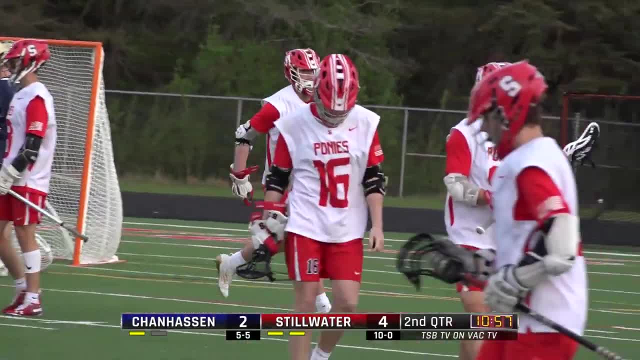 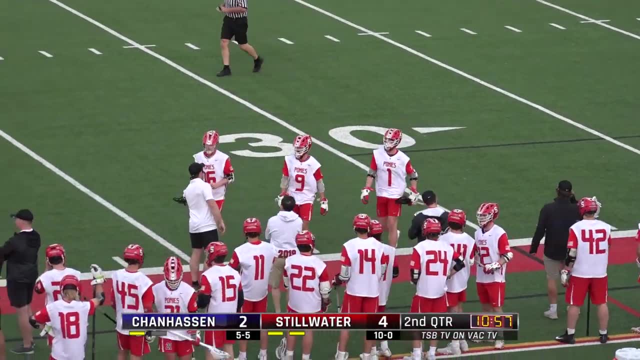 But he does pick up goal number 32 on the season For Stillwater number one, Ty Thurston, who gets hit for number 16.. And Summery gets on the board for the first time. He's on the board for the first time in this game. 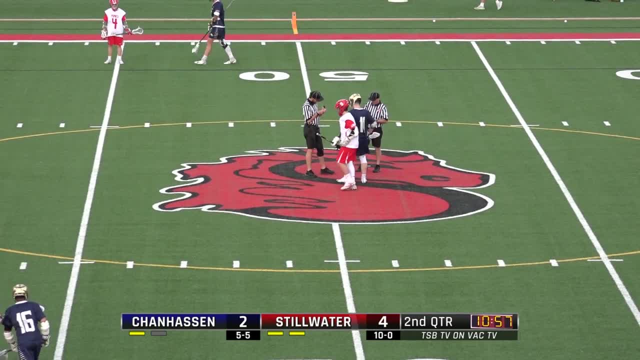 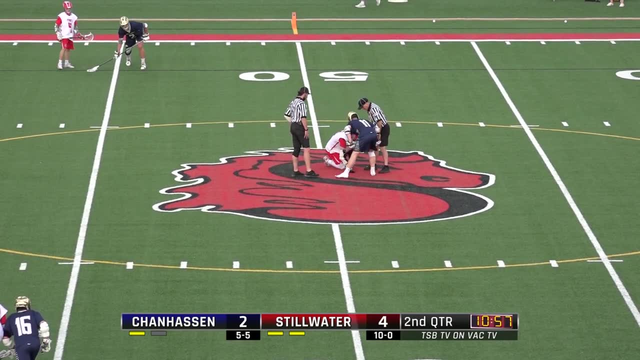 We talked about Evanson and his ball distribution, Nelson Summery. he picked up his 18th assist on the year And Quinton White, picking one up earlier, has 11.. So Evanson may be the point person for facilitating the offense. 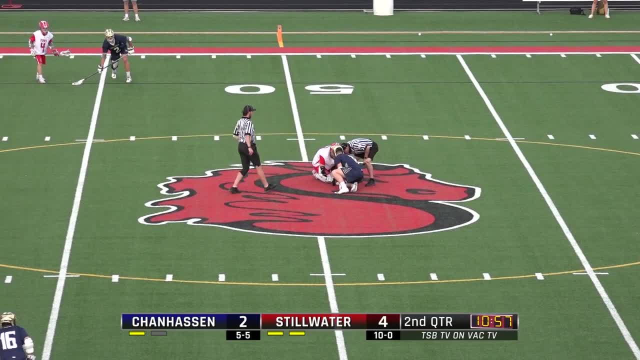 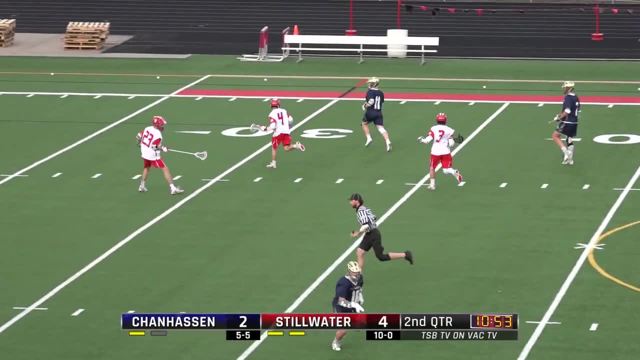 And Ty Thurston may be the lead guy for goals, But any one of those six guys on the offensive side can put up numbers, And we've seen that At even strength. and when they're short-handed- Yeah, short-handed too. 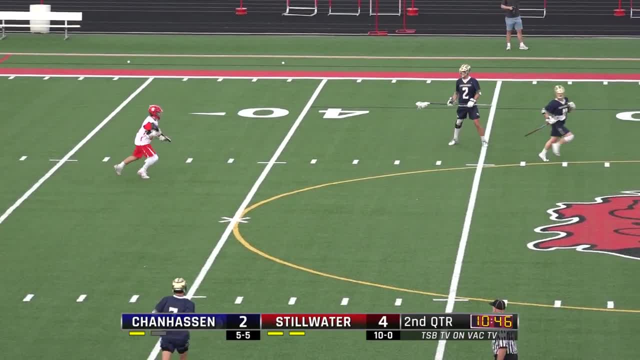 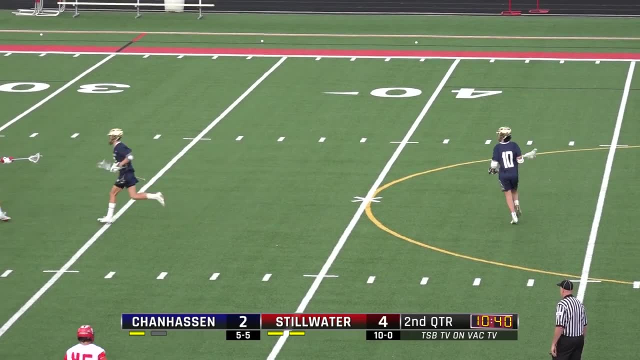 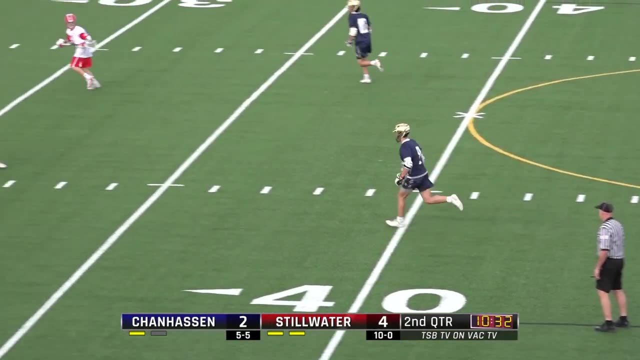 They're especially dangerous. Stillwater has just great chemistry this year. Just the passing is phenomenal. Levinson going to Mercer. Ty Thurston has a college offer in the works. Can't sign the NLI just yet, though, because he's a junior. 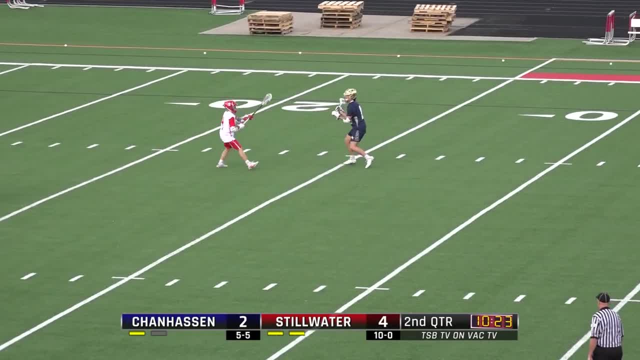 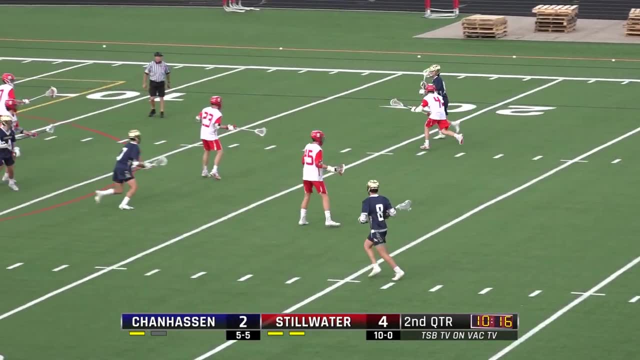 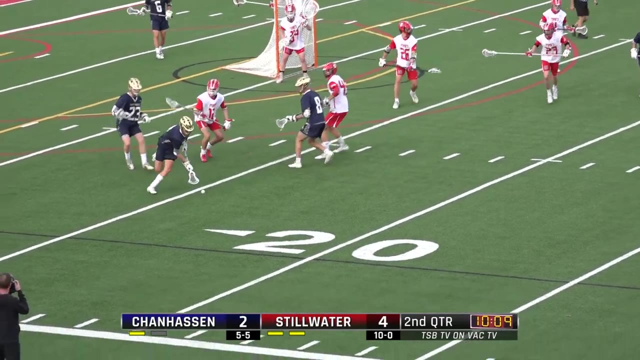 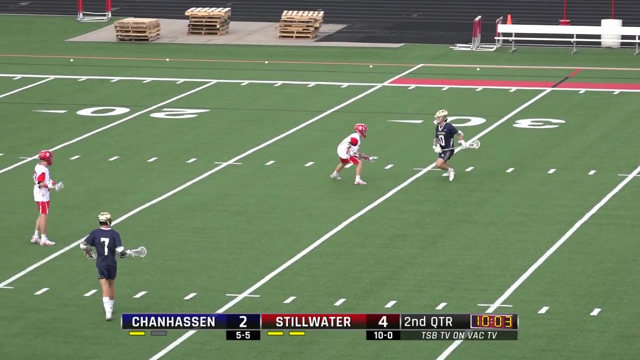 All right. So Chanhassen, once again, Will try to respond. Stillwater has gone up by two goals on a couple of occasions And Chanhassen answered to keep it within one Pass. deflected Loose ball scooped up by Alex Dewey. 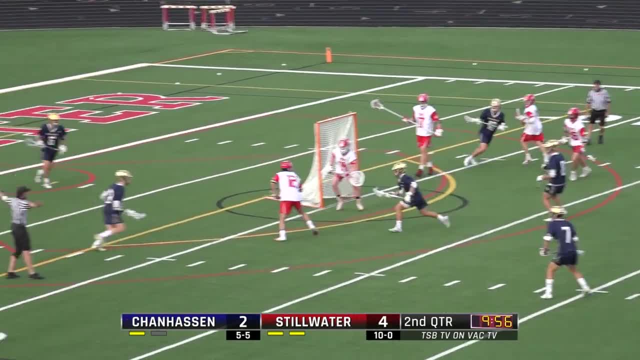 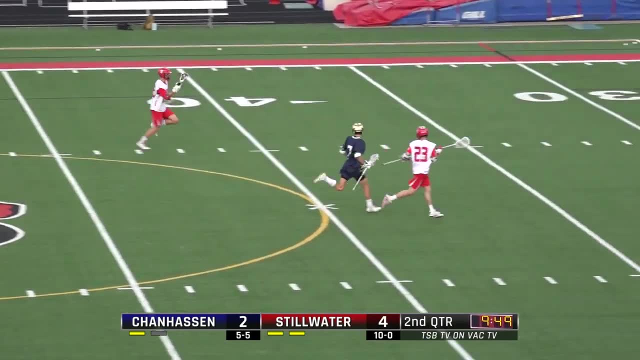 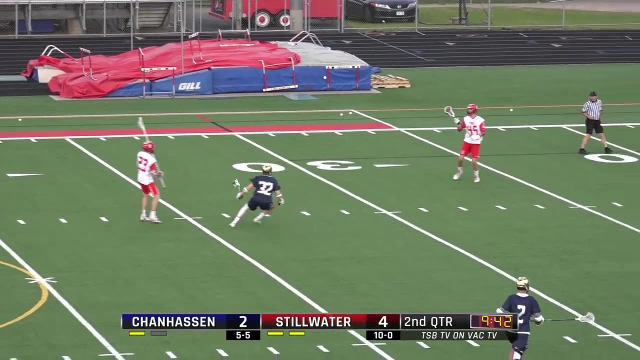 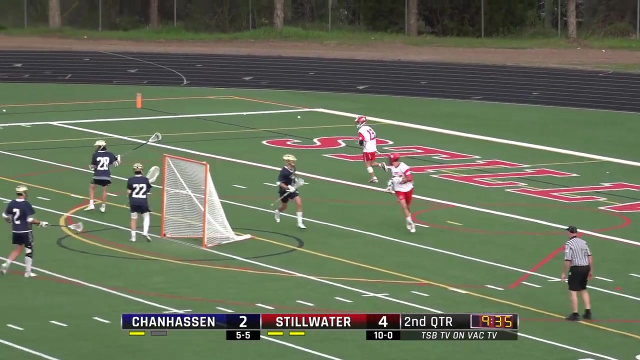 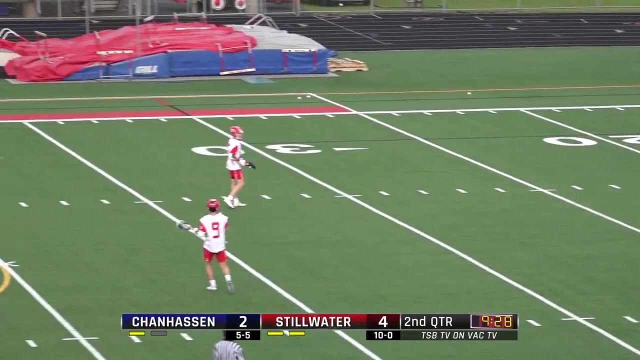 Vincent Manuel Lawrence, with the save, We'll say this: Chanhassen showing a lot of patience in offense here, Not trying to force anything, Stahl looking for Ben Long And the vaunted Pony's offense gets another opportunity to showcase their might. 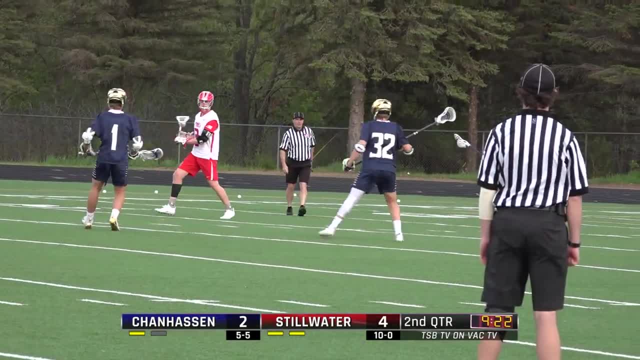 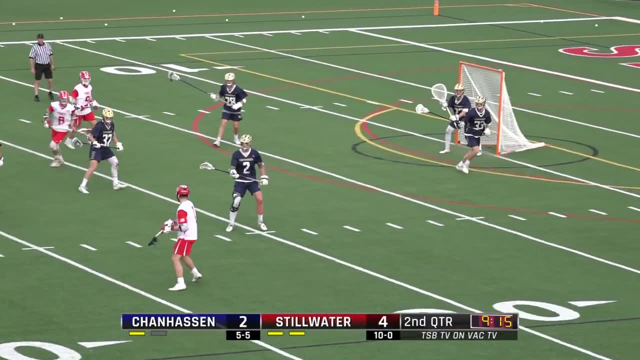 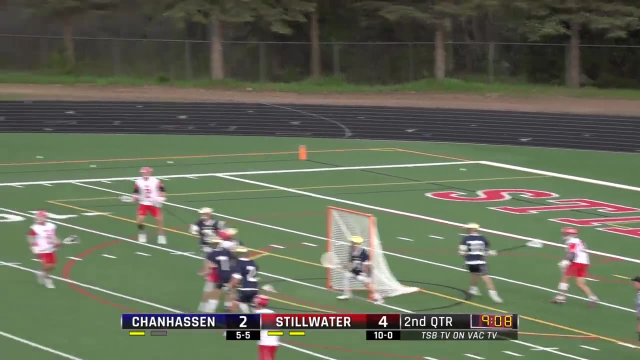 Pony's Stadium Got some cloud cover coming in, but that's okay. Cycle play by the Pony's Evanson with a hesitation move He'll pass back to White The deep pass to Summary. And that was an off-speed shot. 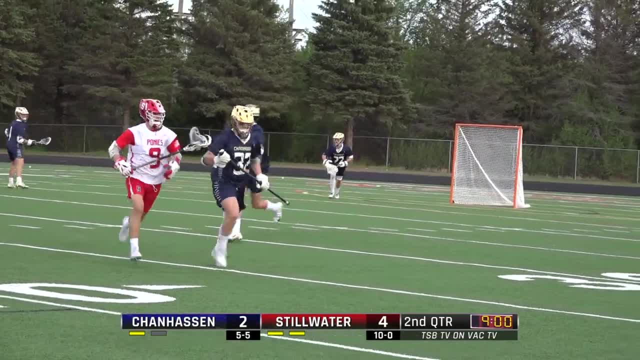 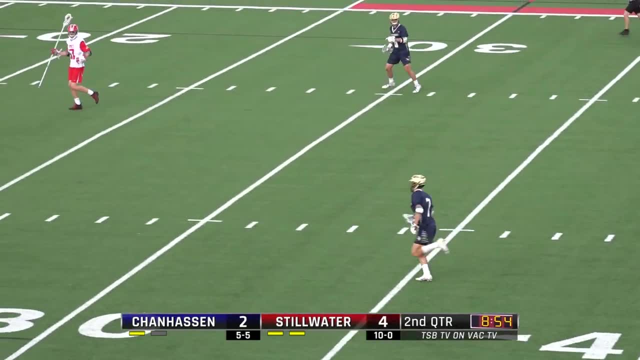 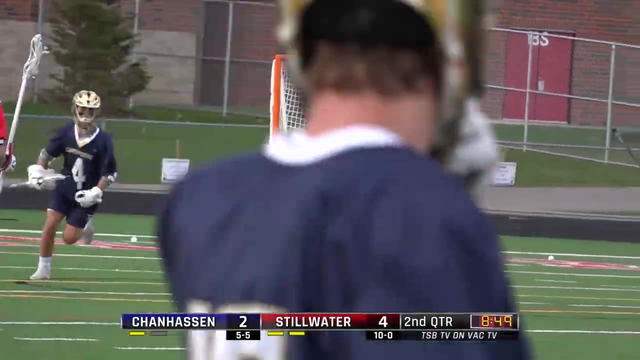 Might have been a pass intended for Berger, but it's picked up by Rathy And the story. Don't have to worry about anything there. Let's see if they can make the most of this. They do. Alex Dewey trots up the field and picks up his second goal of the game. 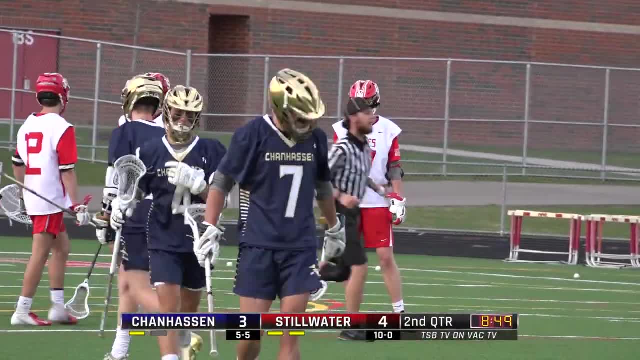 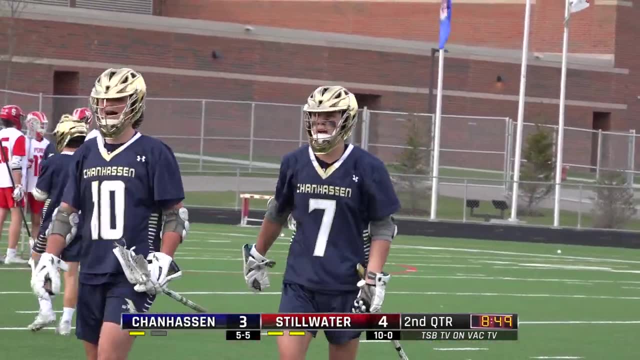 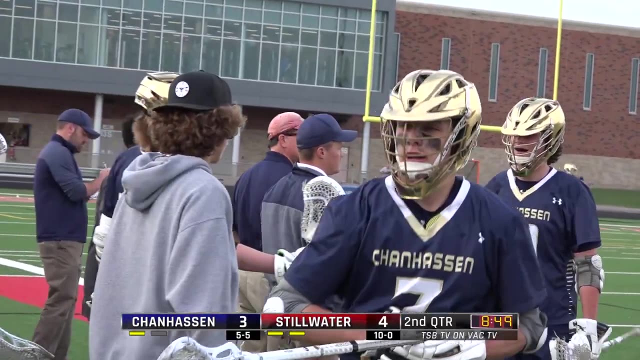 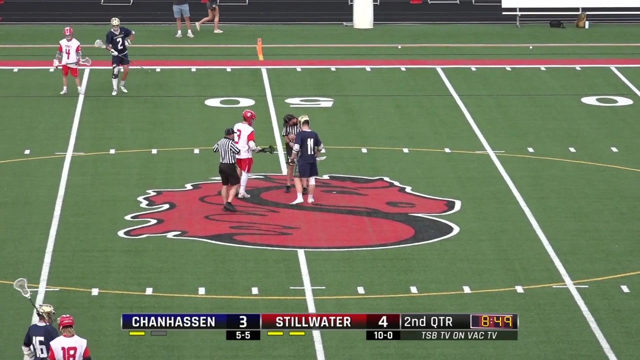 His 12th of the year. Chanhassen has answered: Alternated between teams for a while now And he's got it For a while now. So neither side able to put up a rally. And for Chanhassen that's big because they are hanging with Stillwater here. 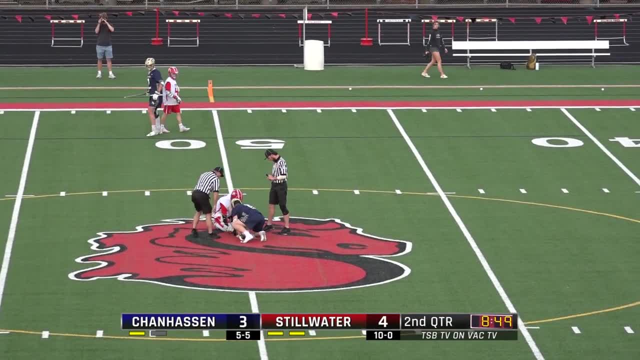 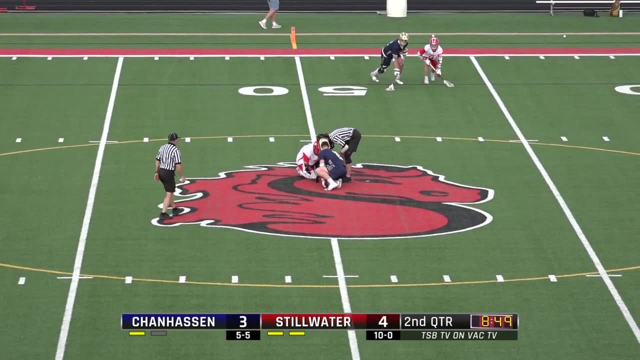 We have not seen this for most of the season, Not since the Matamidai game. No, this game is very close And Chanhassen wants to keep it that way. This game's going to run away. It's going to run away in Stillwater's favor. 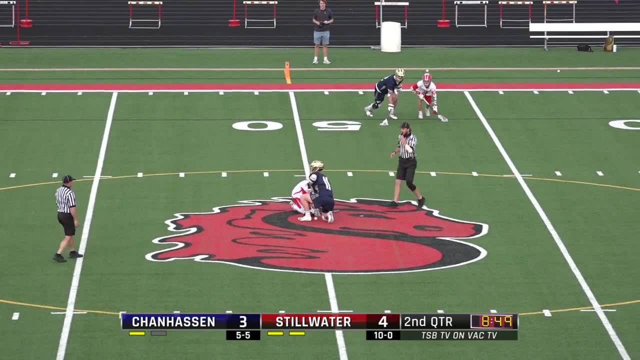 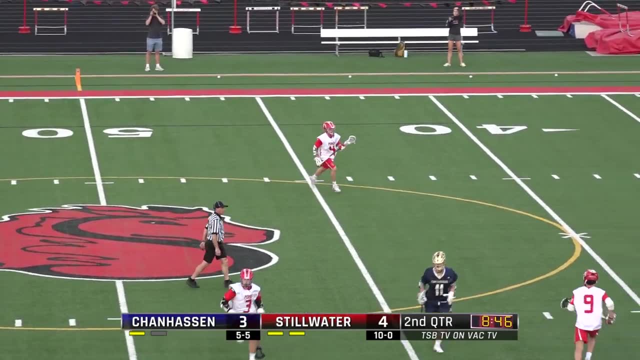 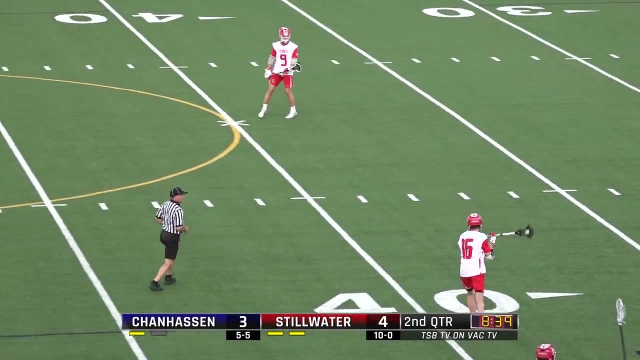 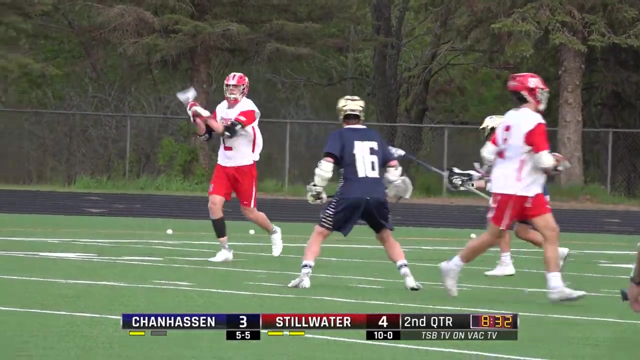 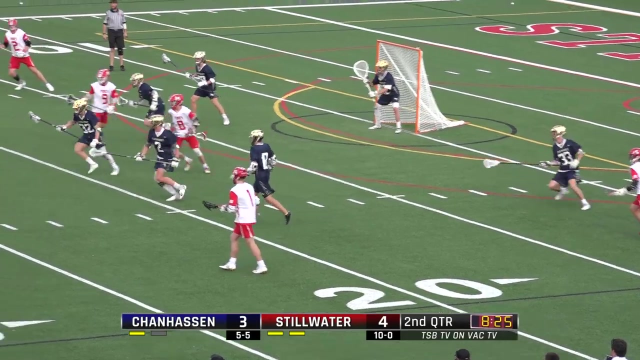 And they do not want that Face-off violation, so it will be Pony's ball. And you don't expect Chanhassen to put up a big rally. as you said. compared to Stillwater, Evanson centering pass, What a beauty. 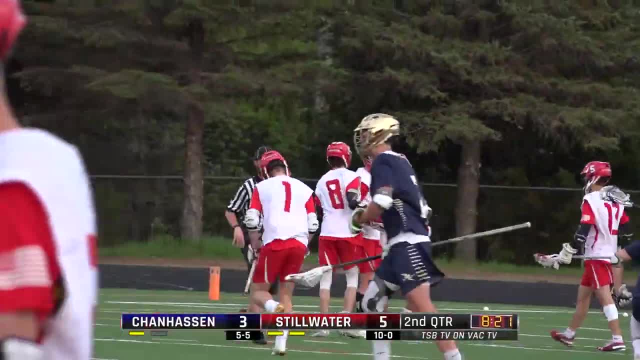 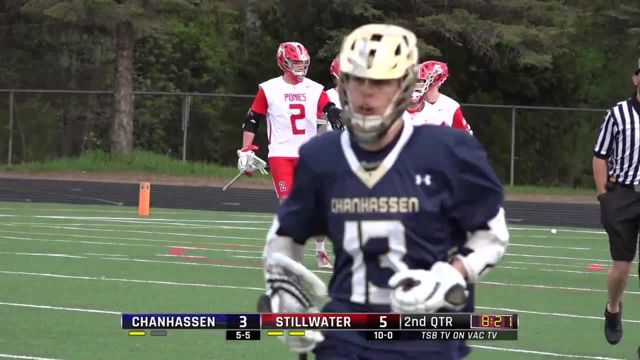 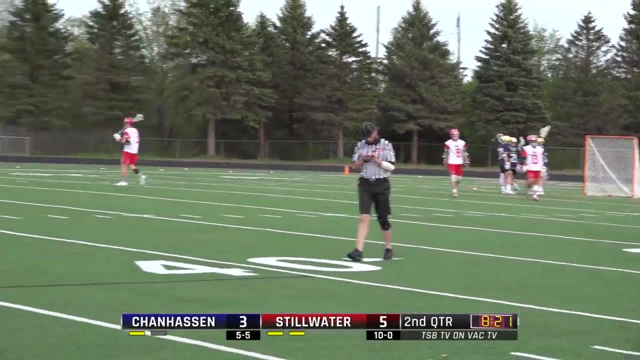 Another assist for Evanson- His third, And Joe Stengel with his second goal of the game. One of those 20 goal scores. It's goal number 24 for Stengel And Evanson. one assist away from 30 on the year. 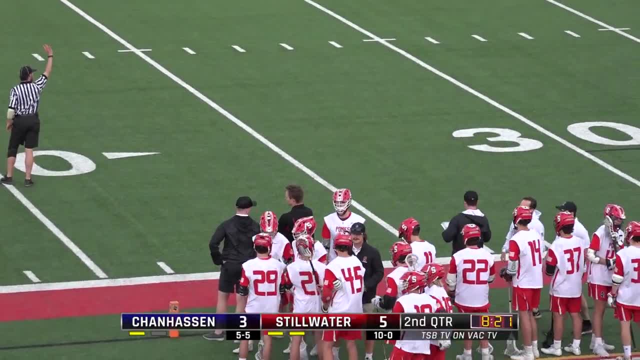 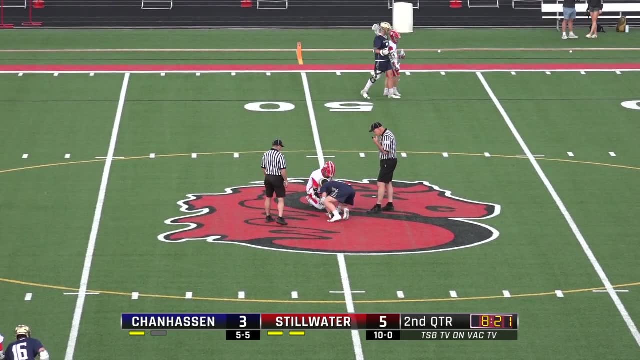 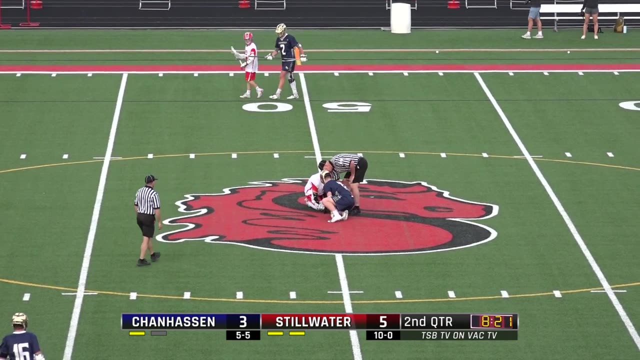 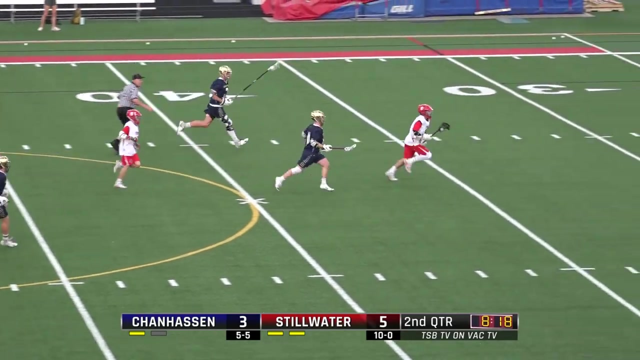 What more can you say? So the Pony's once again go back up by two, But they have yet to get on that big rally And a face-off win for the Pony's. This could be their chance to start this rally. 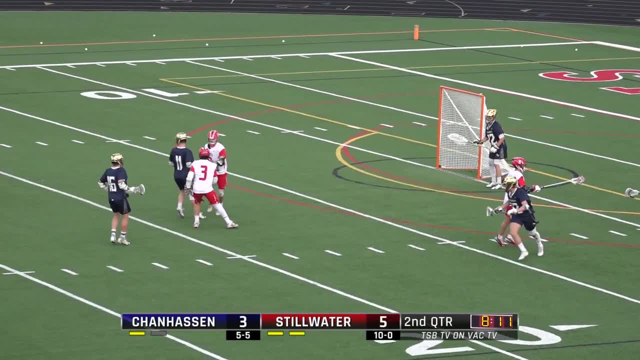 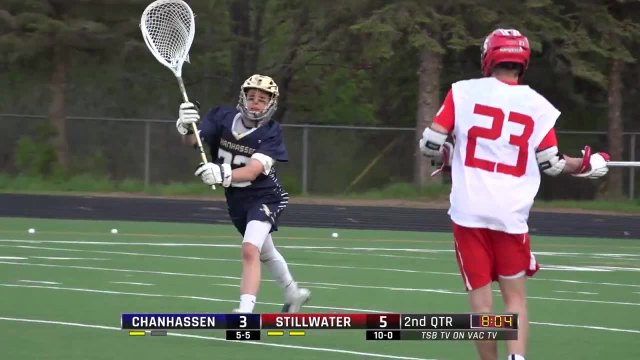 And right away. Corbin Van Dyne took a shot at Rathie And I don't blame him. I imagine the Pony's have to be a little irritated that they can't put Chanhassen away as early as they have against so many other teams. 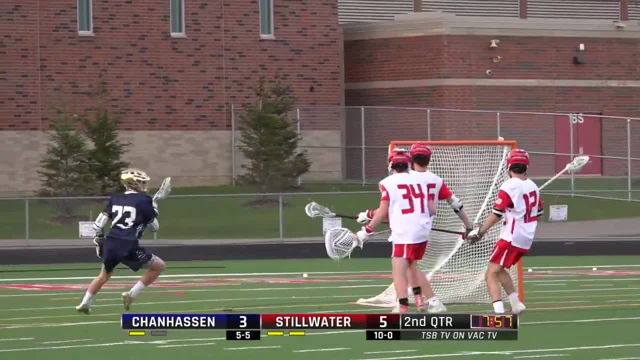 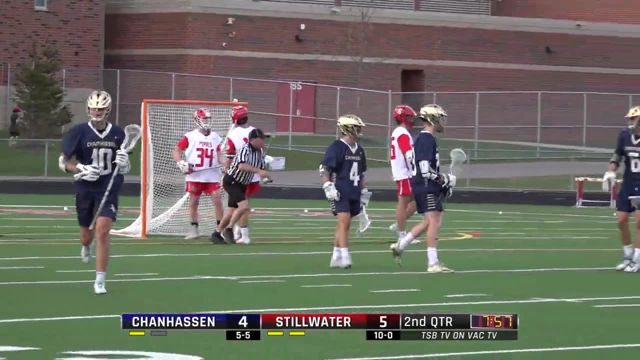 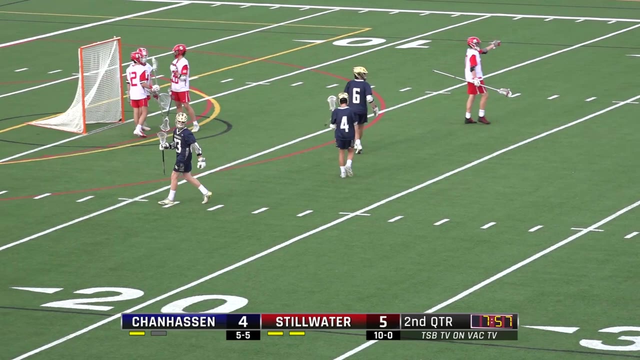 And here come the Storm. Manuel hooks up. Nice move, A picture, a pinpoint pass, A picture, perfect one, and Cal Davis cashes in to catch Davis on the fly. And again, the Ponies denied a chance to build a rally. 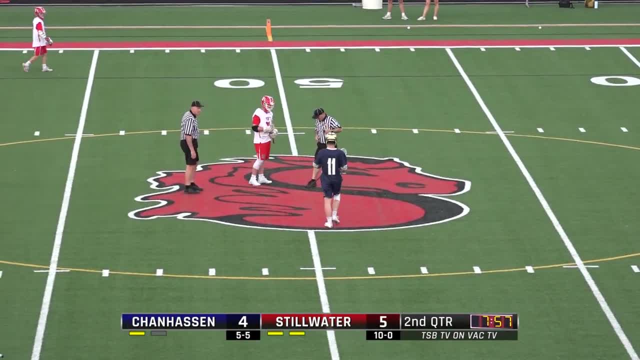 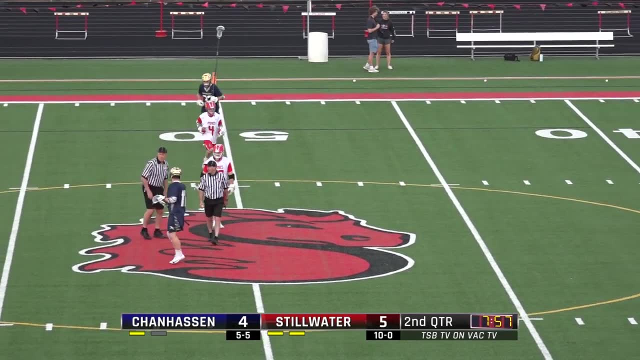 Robert, what do you got to say about Chanhassen's durability? They are not going away. No, no, this has Stillwater not a little bit concerned. They're just gonna tighten up their defense a little bit. They gotta keep Chanhassen outside. 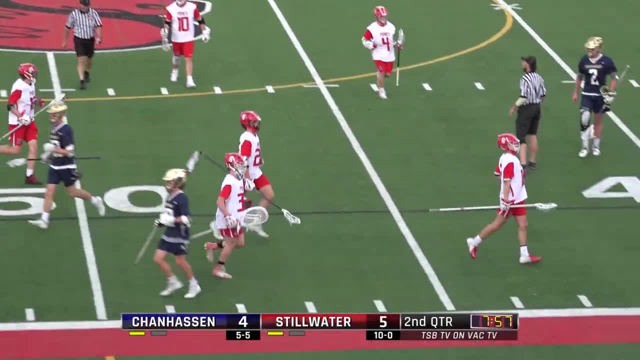 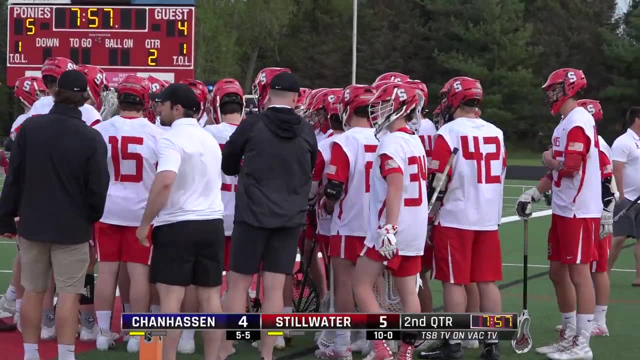 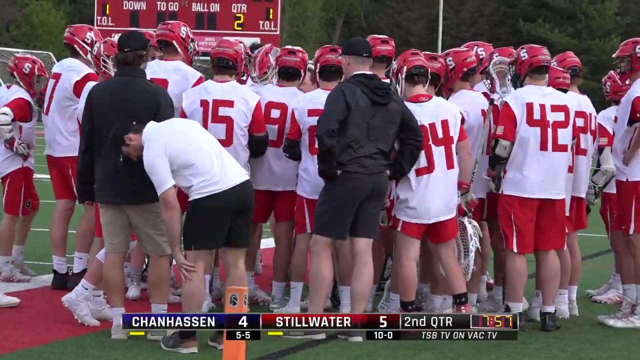 They're letting Chanhassen get into a shooting area. that makes it tough for Gunnar Ehrens to stop those. Well, it's enough for the Ponies to use one of their two timeouts. I can't remember the last time Stillwater called one. 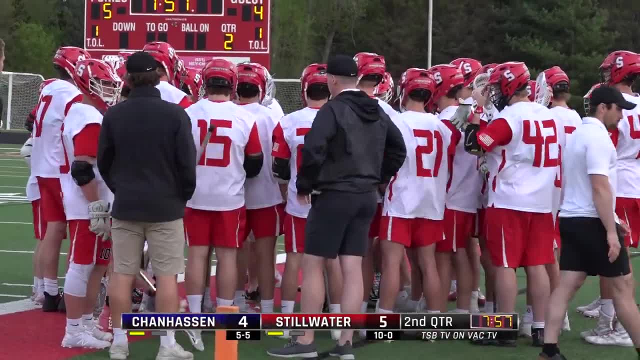 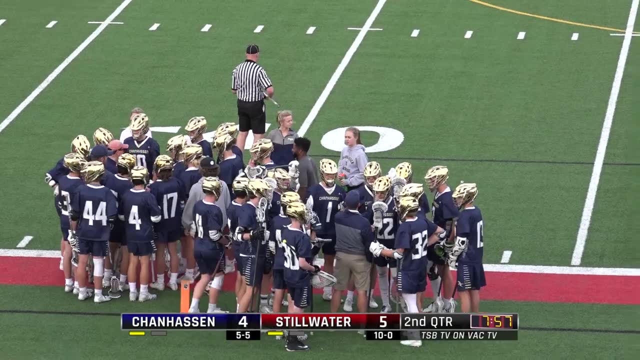 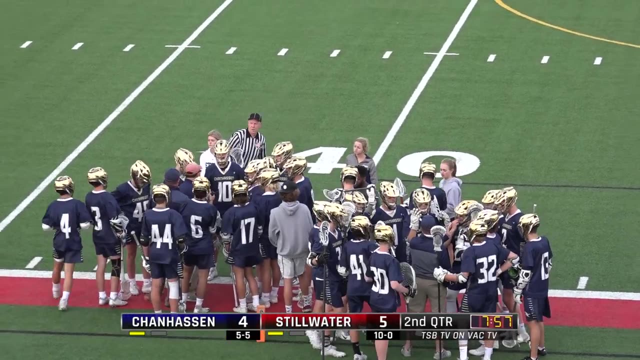 It's been that long. You almost never see them call a timeout, But looking at this game, Chanhassen is averaging 10 goals a game. Stillwater averaging 14 and a half Stillwater, with one of the higher scoring offenses in the state. 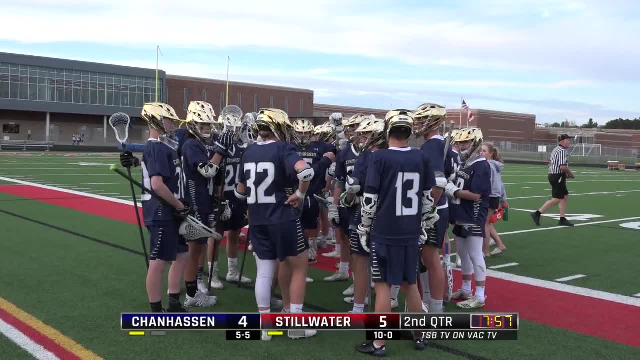 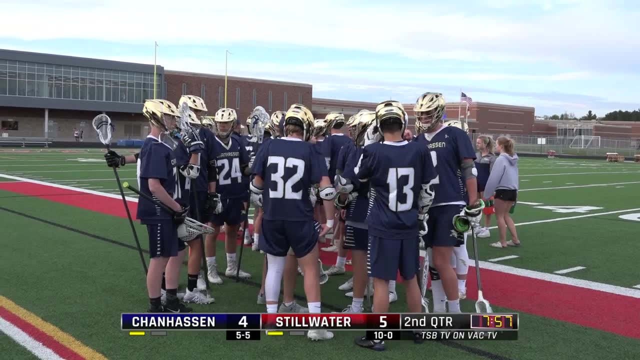 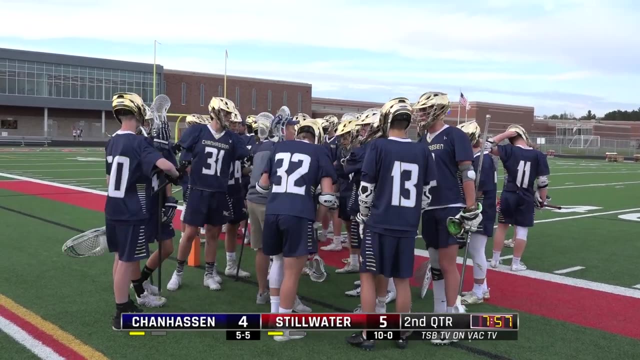 In fact, by my unofficial tally, the Ponies are ranked second, only trailing St Michael Albertville, who has 17.4 game. Stillwater, at 14 and a half, have moved into second place Chanhassen, giving up 7.7 goals a game. 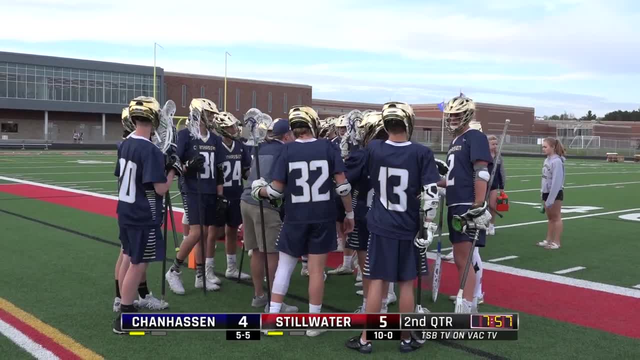 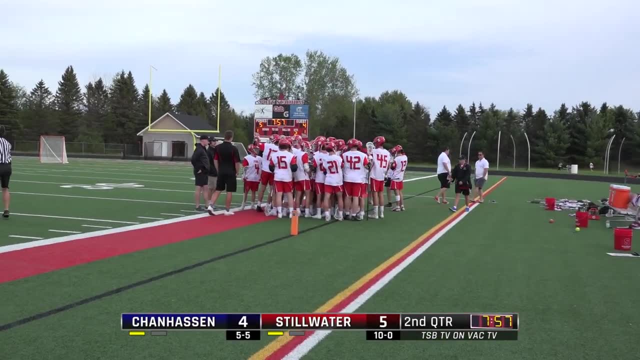 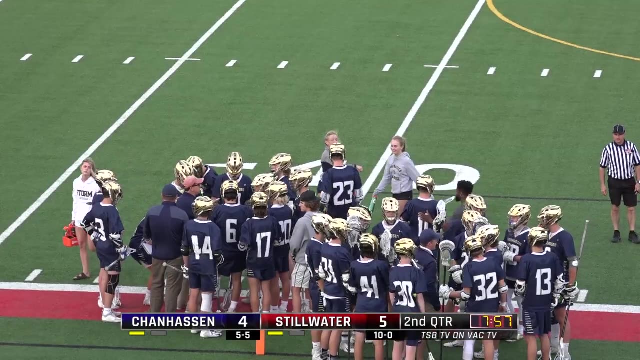 The Ponies giving up 4.7,. so I don't know if Chanhassen found a secret, But here we are And with an illegal stick check for each team by the officials. they're once again huddled together in each prospective group getting instructions. 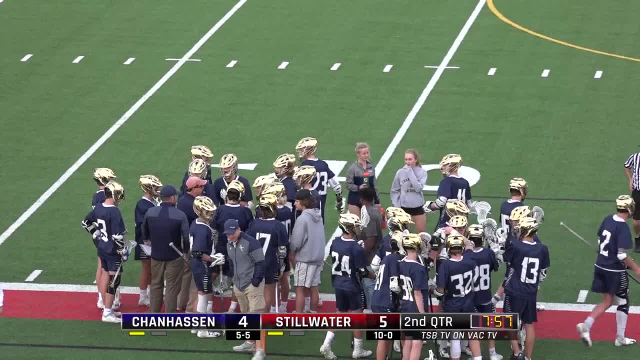 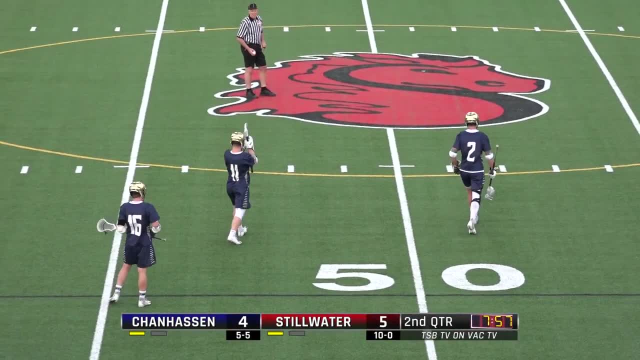 from their coaches. and there's the whistle Stick. checks are important. So you and Alex, one of our camera ops, before the game, you took notice of the helmets. You were enamored by the helmets. I'm not sure for which team. 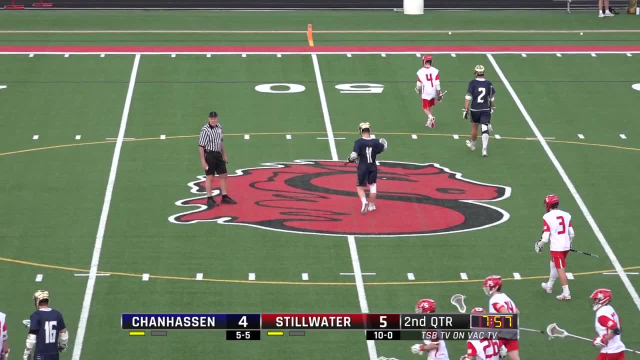 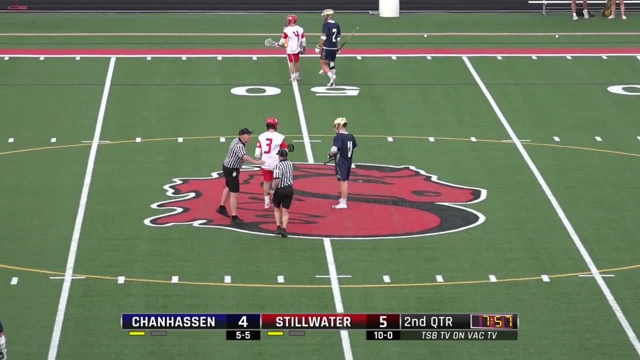 but You seem rather pleased with the design. Oh, I gotta love those gold helmets. They remind me of the new Notre Dame helmets. Notre Dame, yep, And they're very nice, Very, very nice, You're gonna say, Stillwater's, aren't? 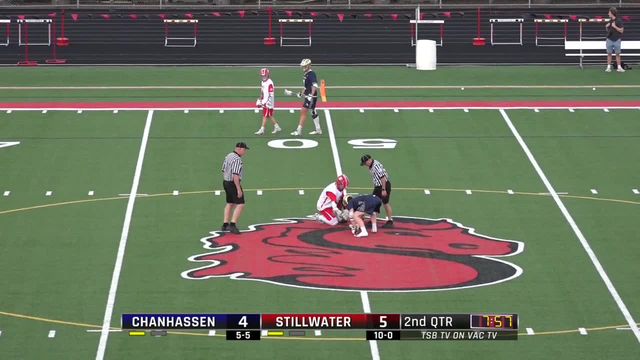 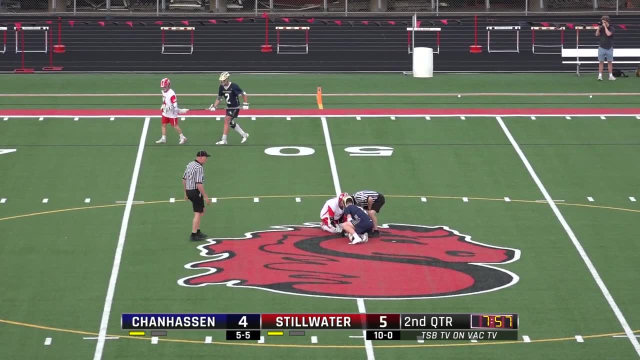 Okay, We'll go with that. So, Chanhassen, you've got some splendid helmets. Stillwater- apparently Robert's not impressed, But Stillwater has impressed us a lot with their play and I think that's a good thing. 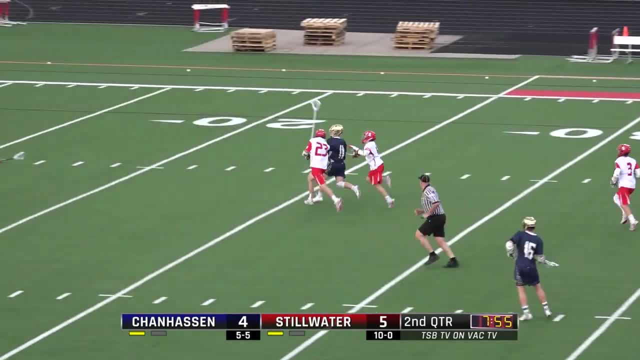 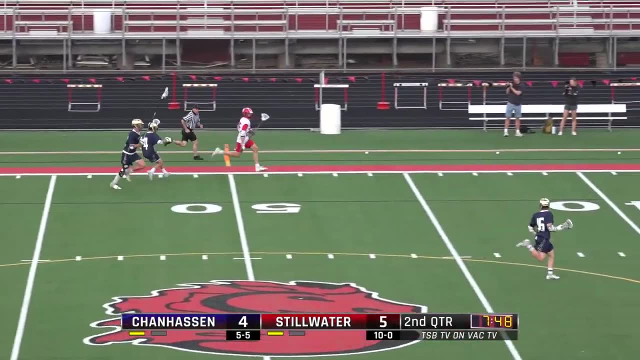 I think that's a good thing. They play on the field and that's what's important. But Chanhassen wins the face-off, They go off to the races and the Ponies all over it. Nate Nicholson won the face-off and the Ponies. 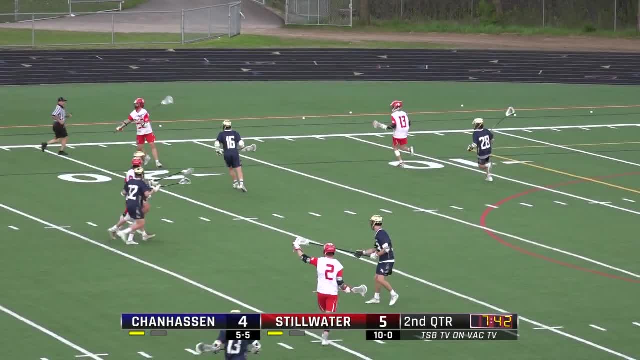 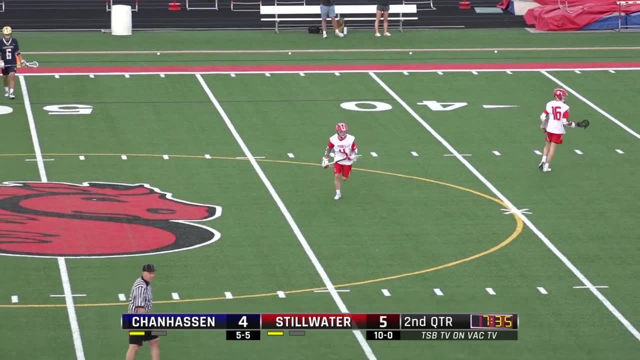 that was a big defensive. stop getting the ball loose on the stick check. The last thing you want is to give up a tying goal. The longer the underdog hangs around, the more confident they're gonna get, and I gotta imagine Chanhassen's. 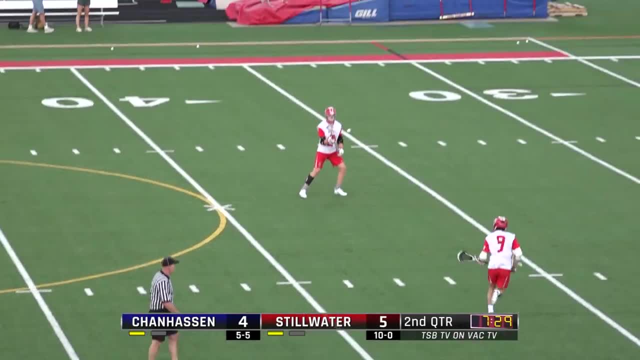 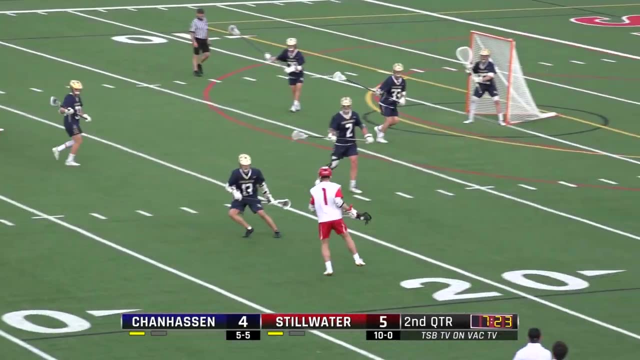 feeling pretty good right now. Yeah, they're feeling real good, Only being down to Stillwater by a goal, where other teams at this point in the game were down by six, seven, eight, nine goals at this point in previous games. 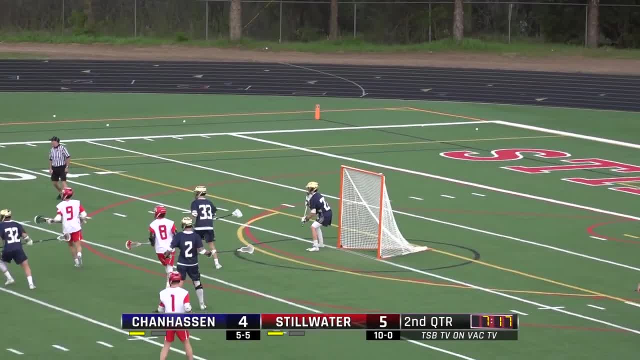 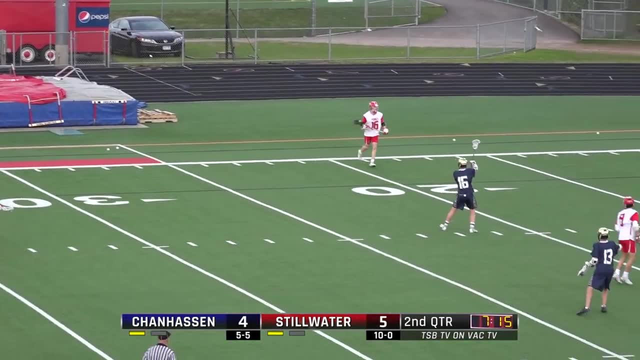 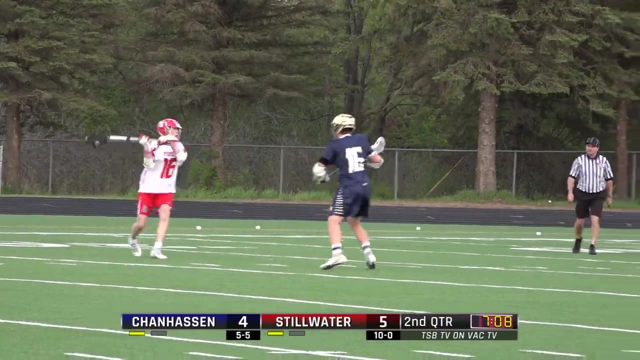 And every time outside of the first goal of the game, Stillwater scored the first two in a row, but after that, second goal by the Ponies, Chanhassen is answered, And so the Ponies unable to develop a rally. We'll see if they'll build one here. 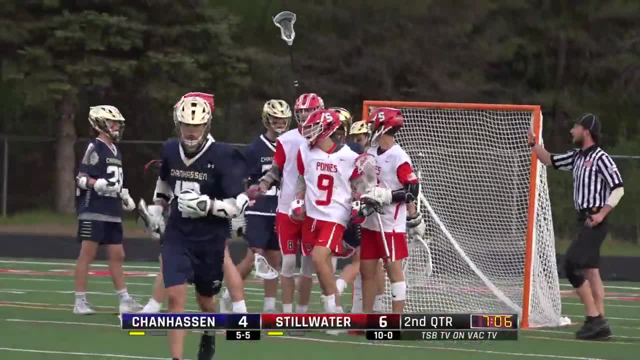 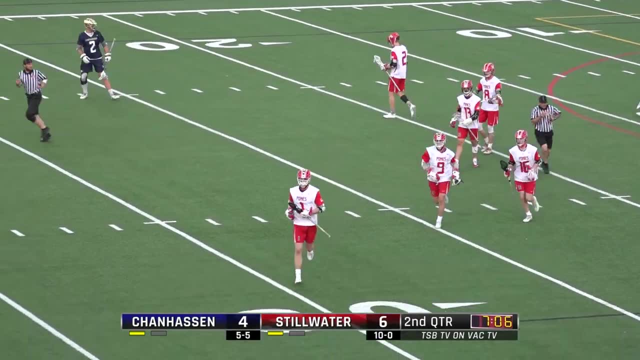 They'll try again. Summary will get the assist as he hooked up with Joe Stengel on the centering pass right at point-blank range And Stengel is our first player tonight to record a hat trick. It comes at the 4.54 mark of the second quarter. 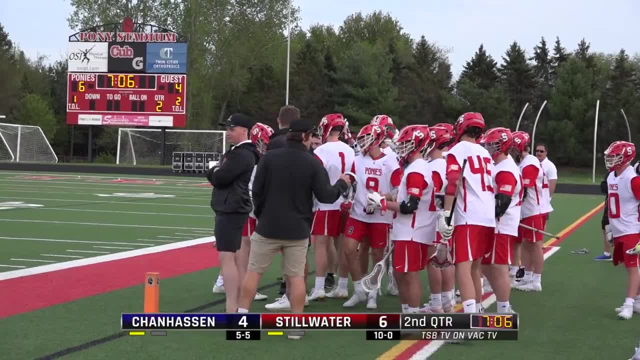 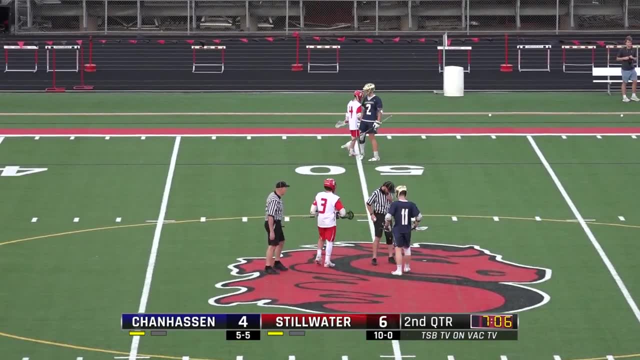 And for Stengel. we were talking a lot about Thurston and Evanson Stengel with his 25th goal of the year, Scoring for Stillwater And for Joe Stengel, The assist number 16, Nelson Stengel. 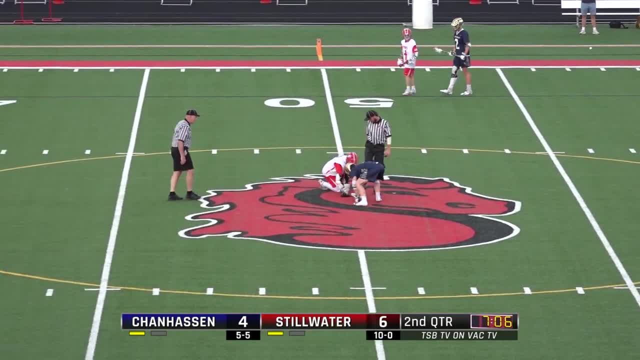 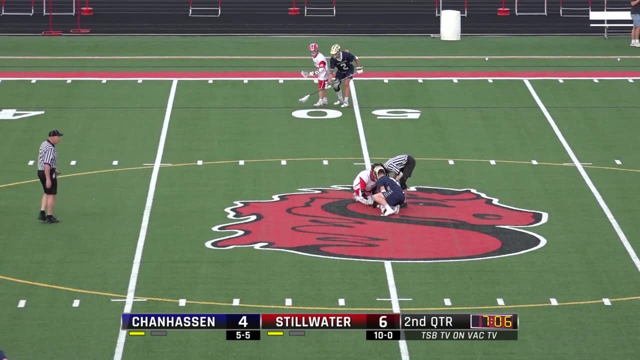 Nelson summary: He picks up his fifth hat trick of the year. Yeah, Stengel's a great shot, a good player And his teammates just love him. And you know in him- Stengel and Nelson's summary on the field- that something's bound to happen. 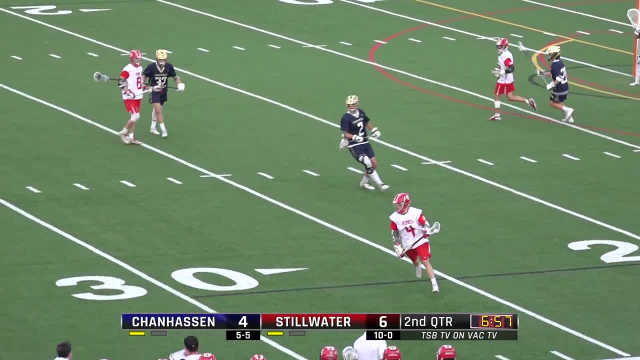 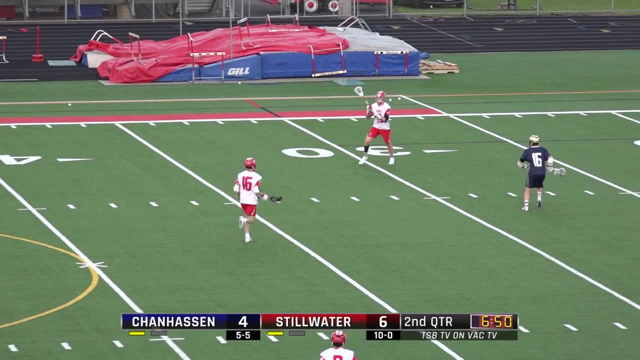 And this is what the Ponies need to get that scoring run A face-off win. There's the speedy Ben Carl. We haven't talked a lot about him so far. Instead, Stillwater will set up for another set. play Berger. 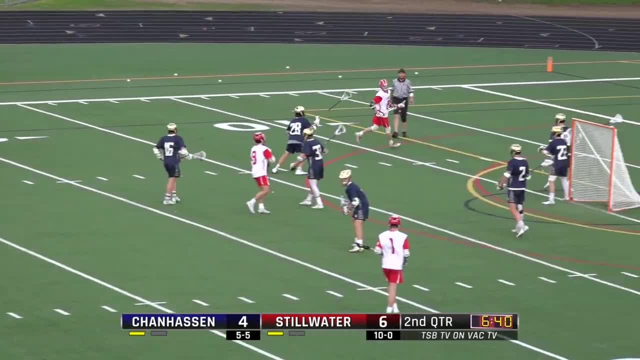 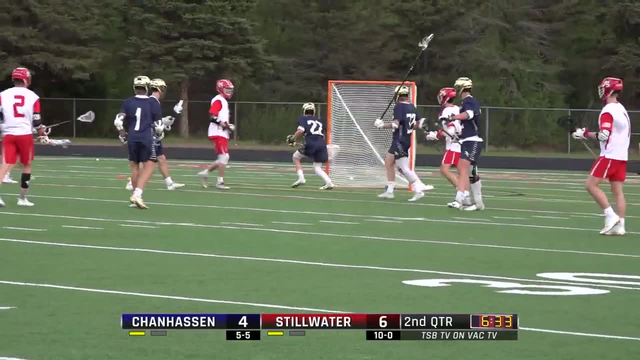 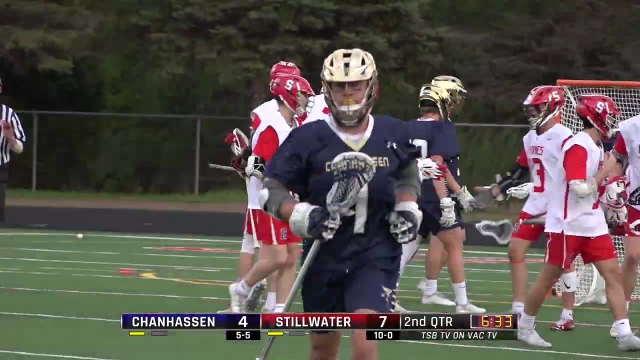 It'll go back to White White deep, to Evanson. He takes the shot from deep- You don't see that often- a shot from the point And Evanson gives the Ponies their largest lead of the game. Could this be the run Stillwater was looking for? 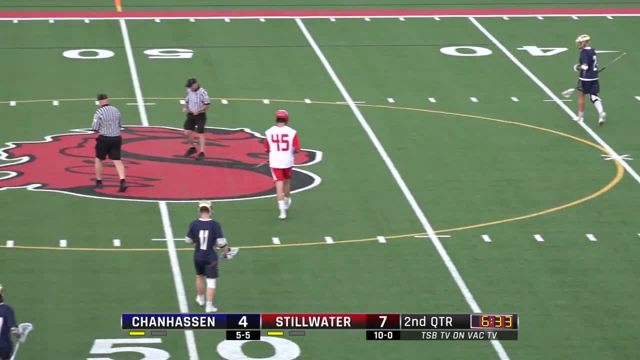 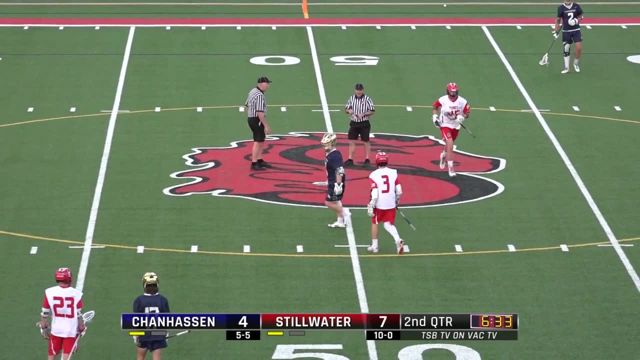 White will pick up the assist. Evanson picks up goal number 26 on the season. So the Ponies finally get back-to-back goals since the first two of the game. Robert, I'll tell you what This could be the run. 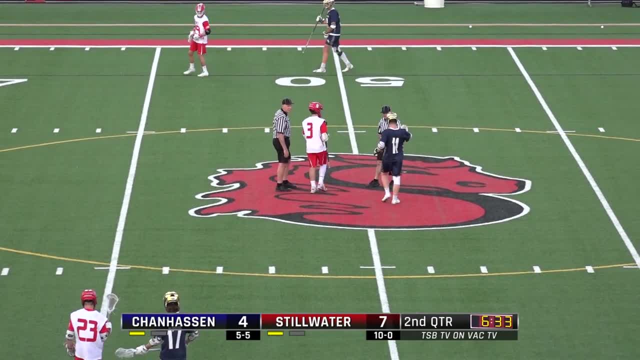 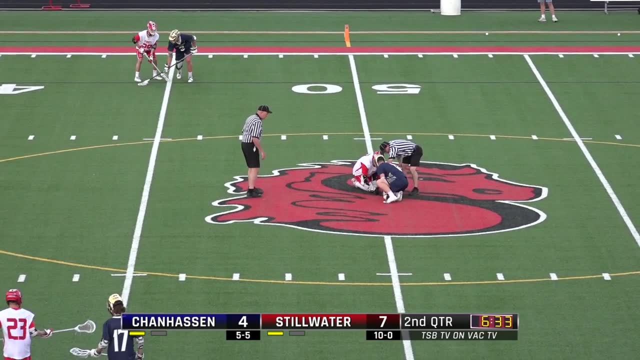 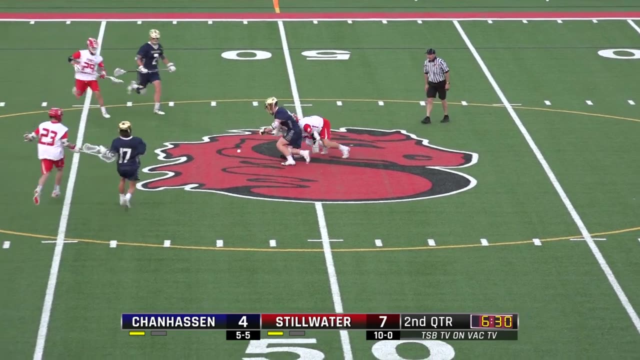 Yeah, this could be it Now. Stillwater's feeling the flow of the game. There's a lot of chemistry in their sticks right now. If they could put up a couple more goals, that might cause Ken Hasson to stumble. Storm, win the face-off. 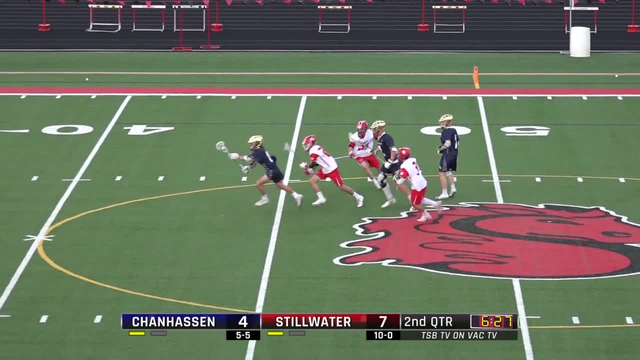 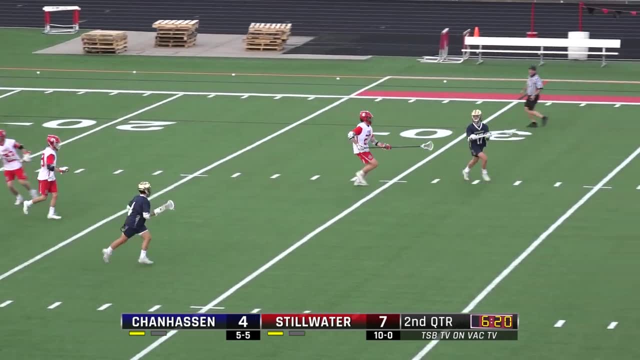 Cade Redding had nowhere to go And we're going to have a Stillwater penalty. It will be there first. So Jen Hasson will get a man advantage here, unless they score. What up, baby? I don't know why I'm hammering. 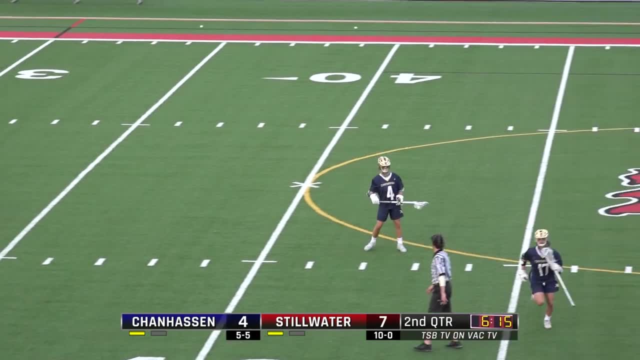 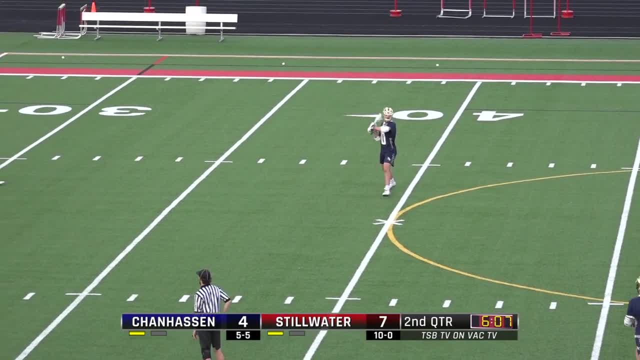 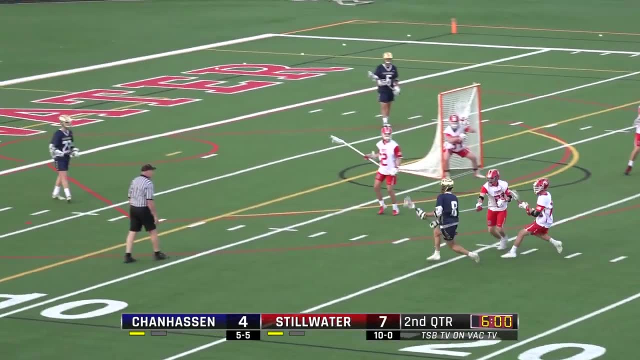 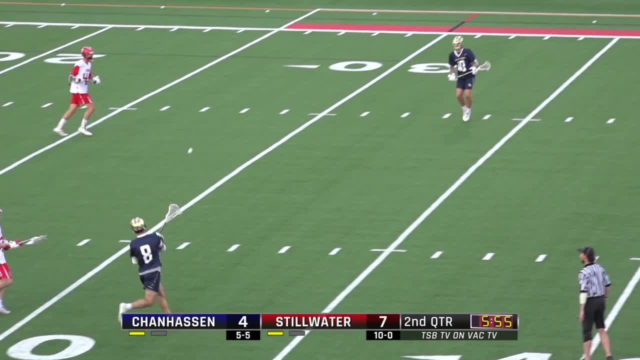 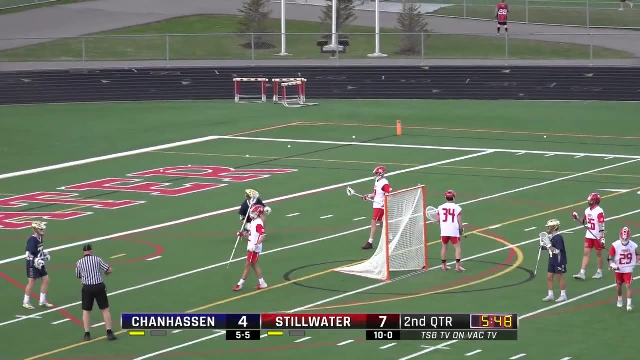 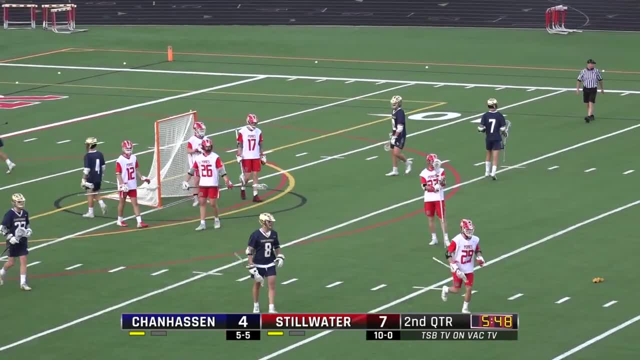 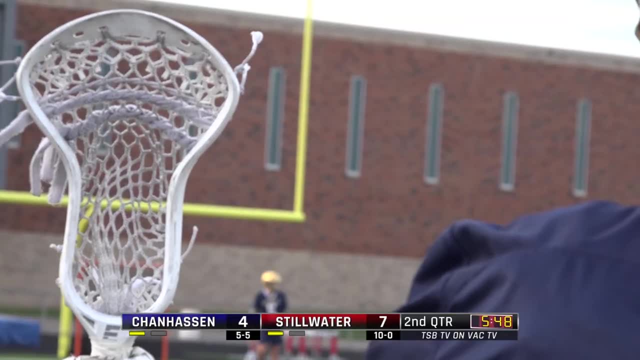 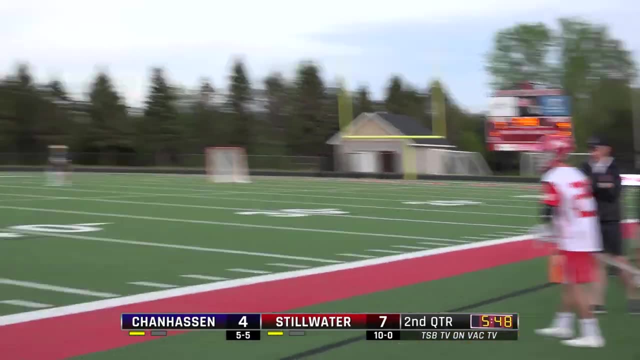 but it will be their ball. It should be One, Two. Jen Hasson turned it over, unless it, We've seen that Chantasson ball. Yeah, that does make sense, And they waste a little time putting the offense. 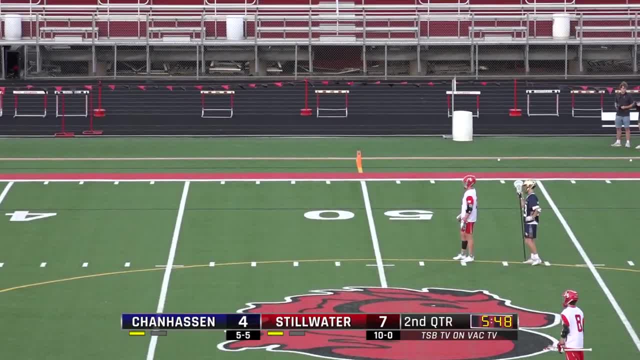 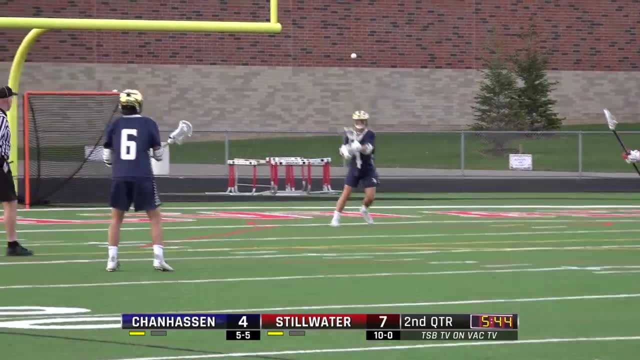 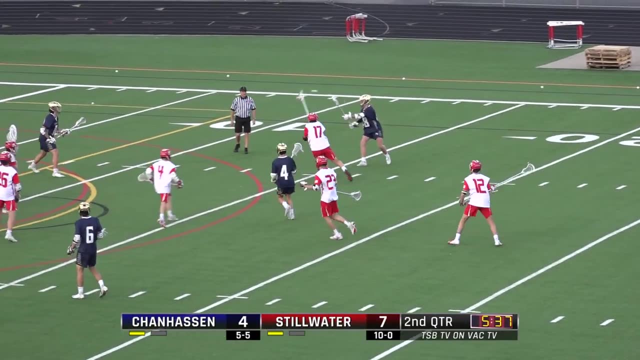 or they try to get the offense going, but officials have not signaled a start play yet. The penalty is on Nick Dario. Nick Dario, one minute for slashing. Slashing is the call. so Chantasson keeps possession, so that misfire does no damage. 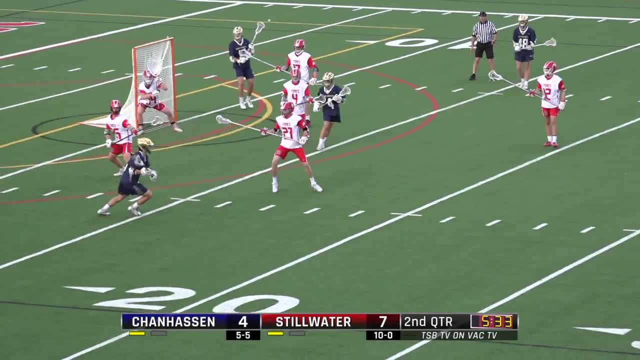 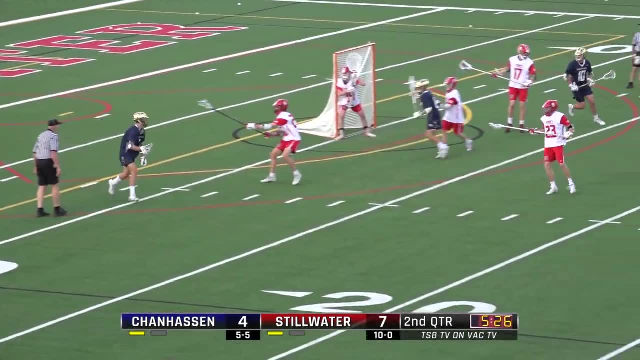 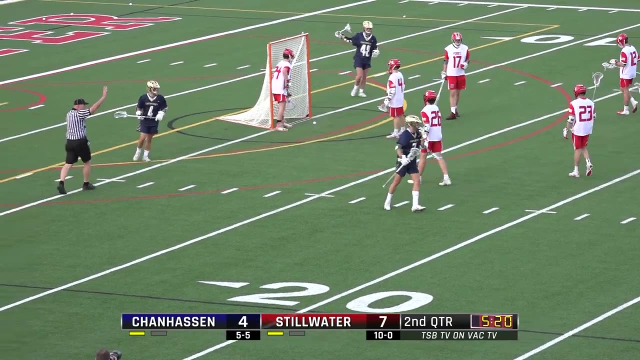 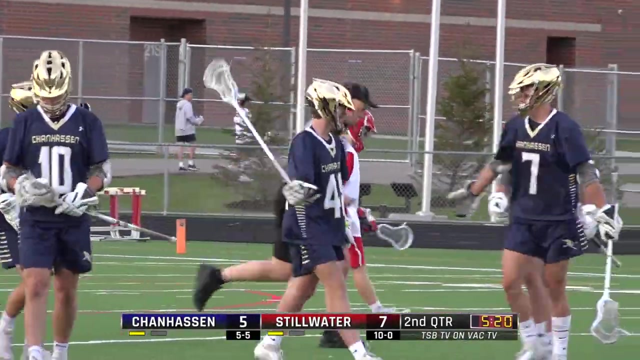 And, as we've seen, the Ponies can be just as lethal shorthanded as they are at even strength. You give them that chance And the Storms score Holcomb. with the assist, Alex Dewey picks up his third goal. 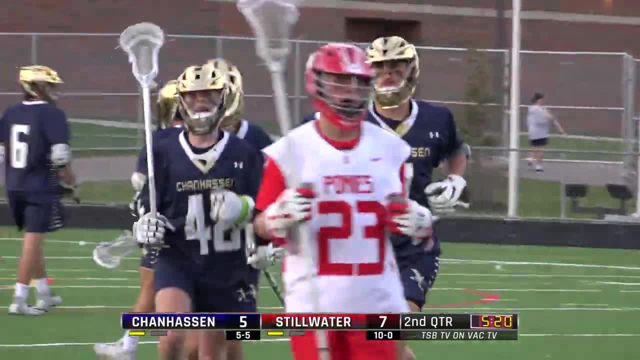 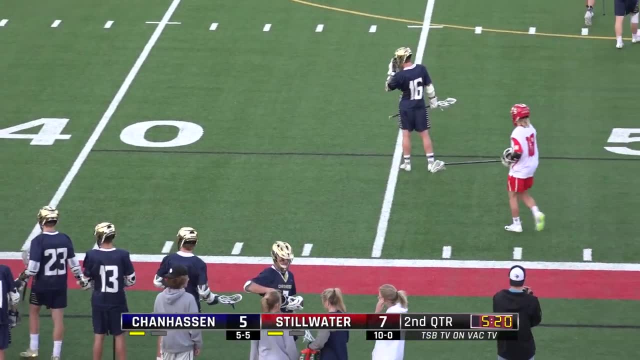 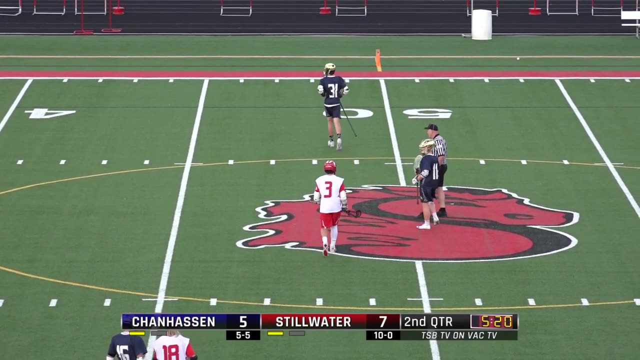 and Dewey with a hat trick for the Storm, And here they are Still hanging With Stillwater. here They make it a two-goal game again. Number seven: Alex Dewey. assists for number six: Hunter Holcomb. Five minutes and 20 seconds left in the second quarter. 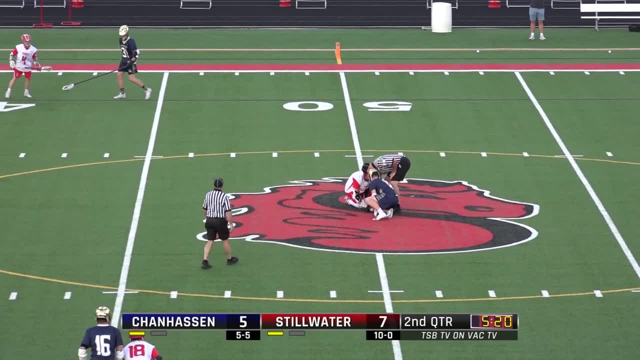 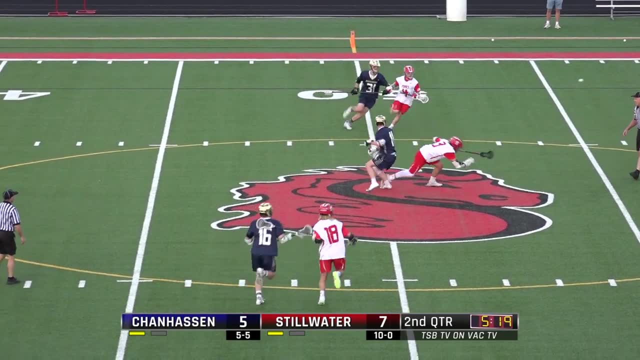 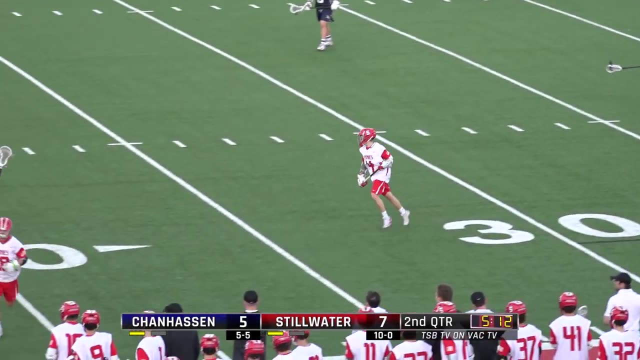 So Dewey has 13 goals in the year And Holcomb leads the team in goals and leads the team in assists. Well, Alex Dewey looking good tonight. His shots are really sharp on target. Another face-off win for the Ponies. 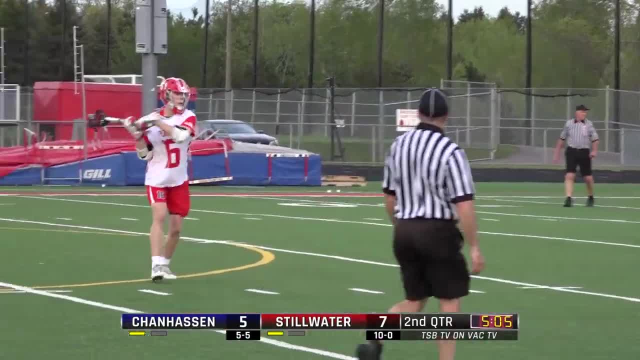 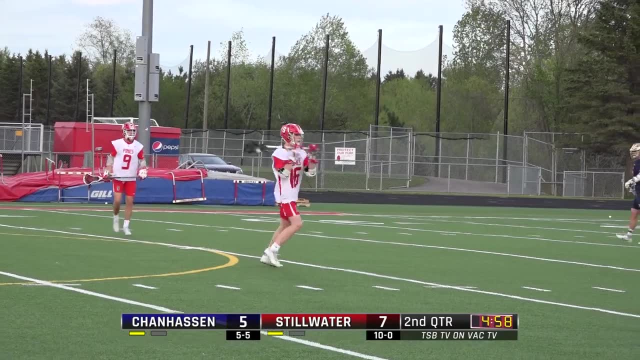 And that's another thing I've noticed in this one. With those runaway wins, Stillwater not only controlled possession, but they won a lot of face-offs. so far, Chantasson has won their share of them And they don't waste a whole lot of time. 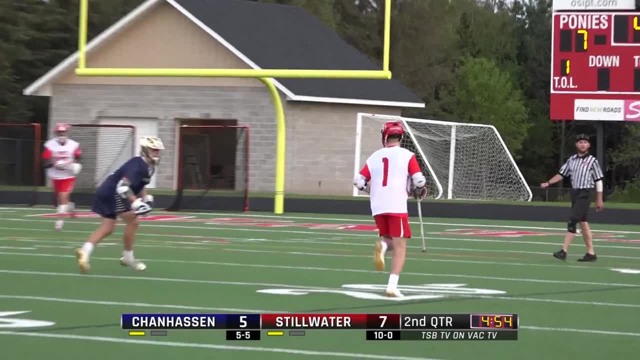 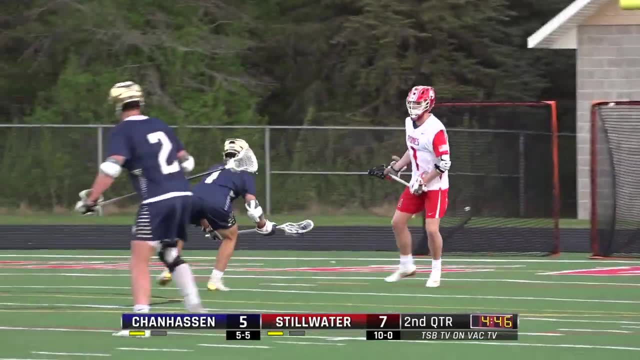 They don't waste a whole lot of time. They don't waste a whole lot of time. They get the ball moving on offense And I wonder if they do that to keep Stillwater from setting up Attack early and try to catch them off guard. 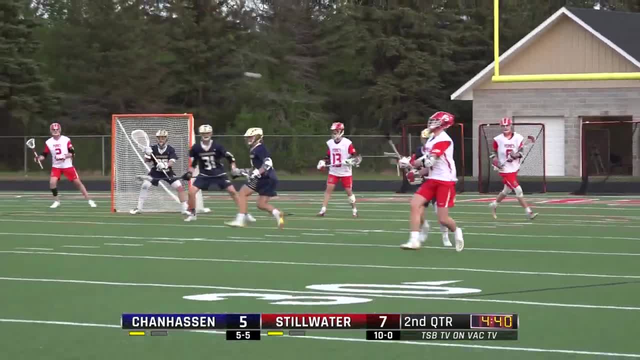 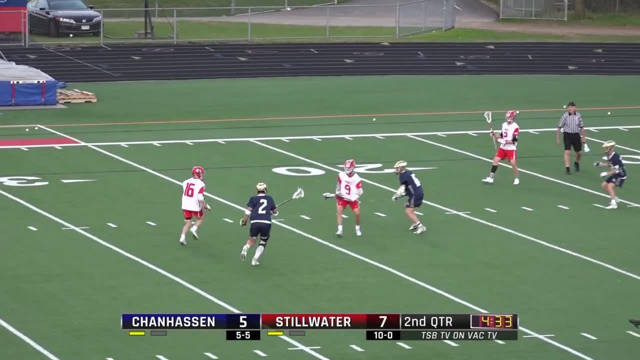 Here's Ty Thurston trying to shake his defender. Jackson Lekoski, Couple of the Stillwater guys, said he wanted to shoot it And it looked that way. But no shot clock here at the high school level, so you can take as much time as you want. 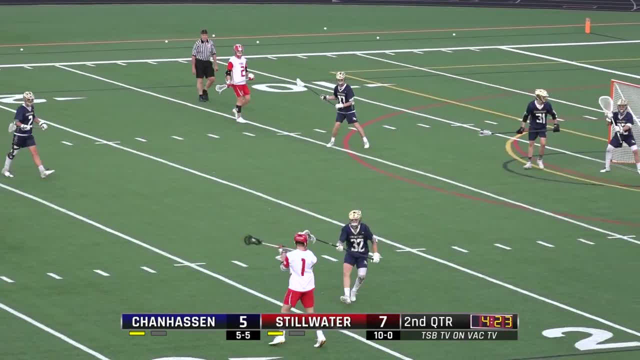 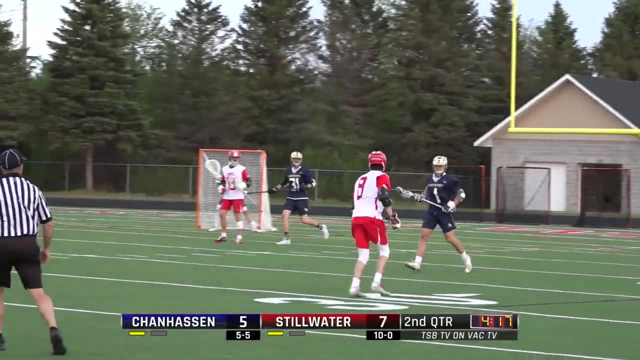 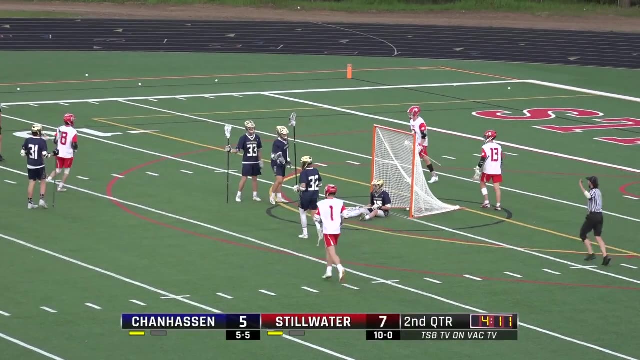 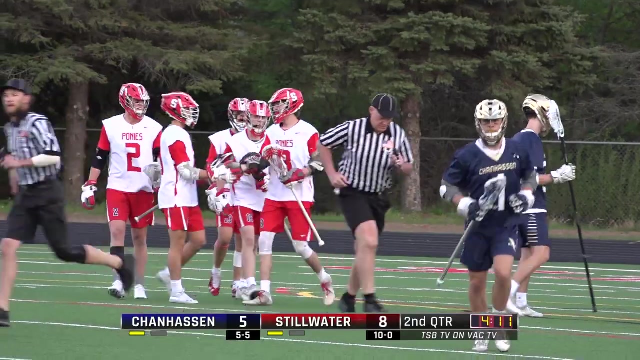 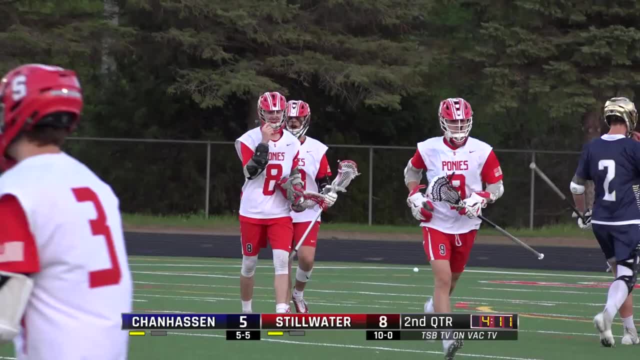 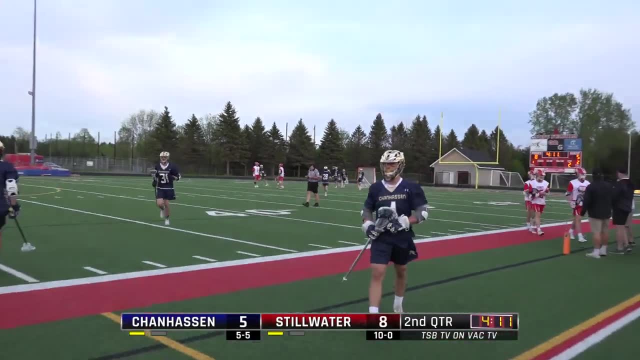 You had a defender on him And didn't bother him one bit. Found just enough of a seam. Found just enough of a seam to get over the shoulder of his defender. Yeah, Chanhassen, needing to respond Again, they're gonna have to respond right away. 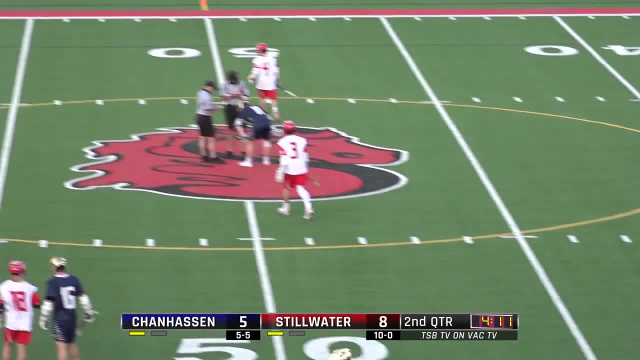 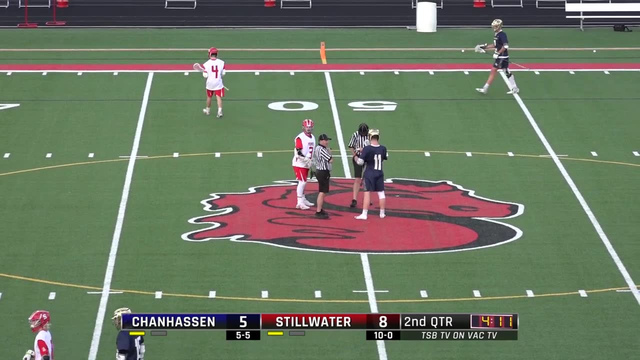 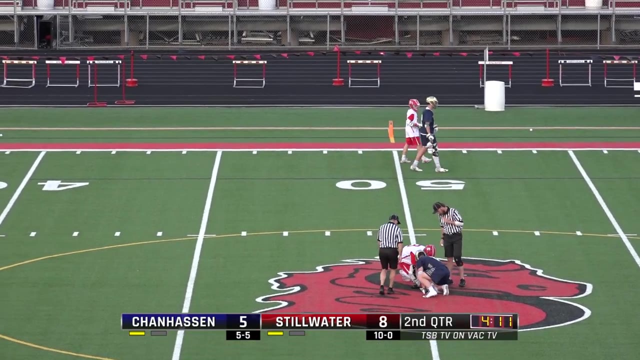 because no response will only distance the score further in Stillwater's favor. They do give the assist to Ty Thurston. So Thurston with one goal and one assist, And the Ponies- for them this is a normal scoring half. They already have eight, but it feels like. 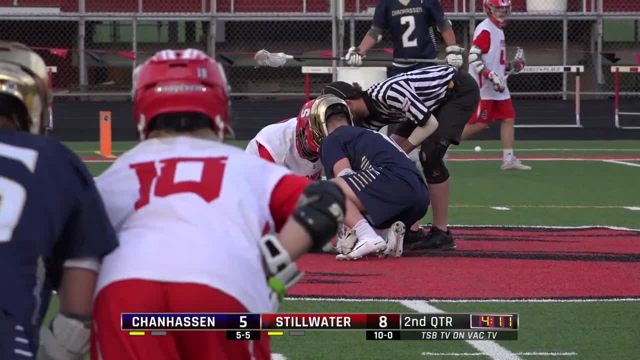 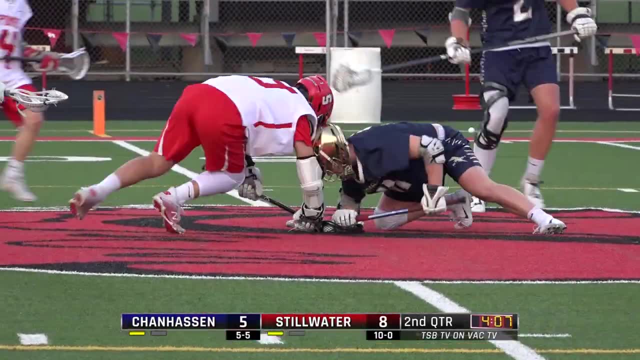 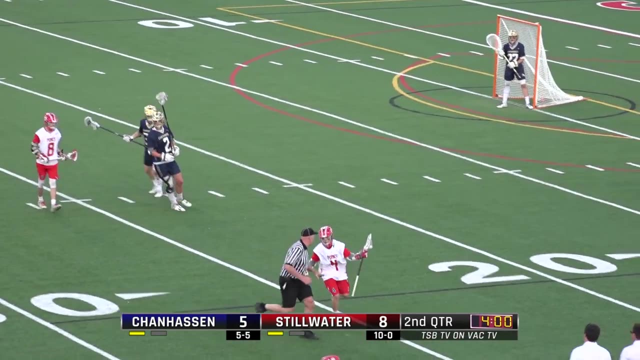 they're gonna need to score a lot to keep Chanhassen away. Usually they score a lot and then just cruise in the second half, but they're having to put up a lot of goals because of Chanhassen's feistiness. Carl wins the scrum on that face-off. 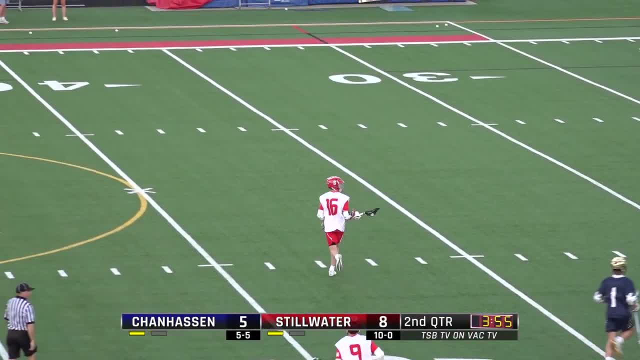 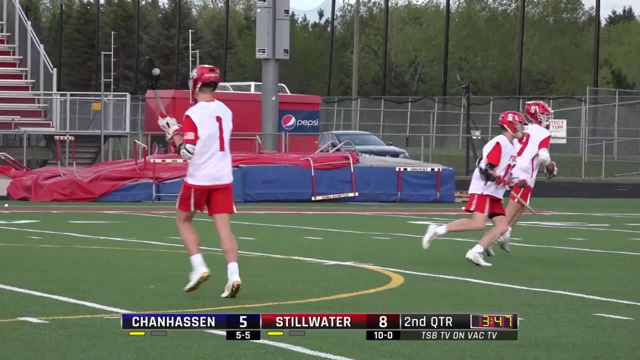 and he'll look for a target to pass to before subbing back out Carl the middie- speedy bingo. They call him the Tasmanian Devil, at least that's what Tom Ho calls him. Here's Thurston launches a sidearm. 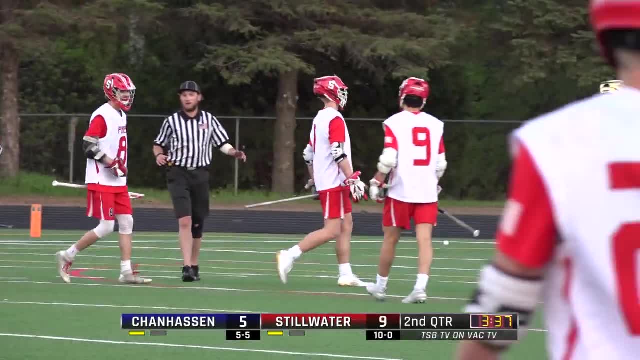 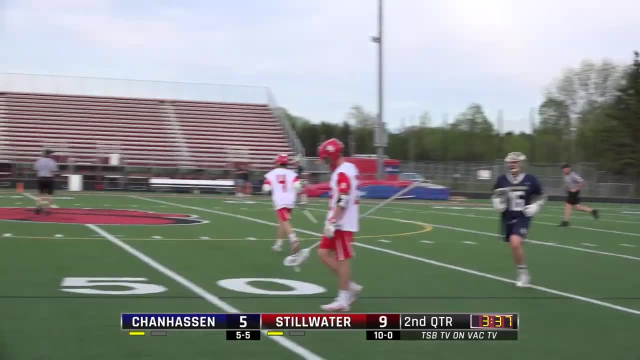 And the Ponies are getting a rally here, not a giant one, but they've built their lead up to four. So a pair of two goal rallies here, and you know baby steps. you don't need that 6-7-0 run. 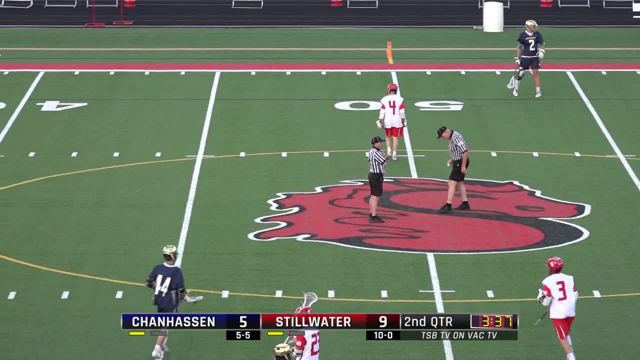 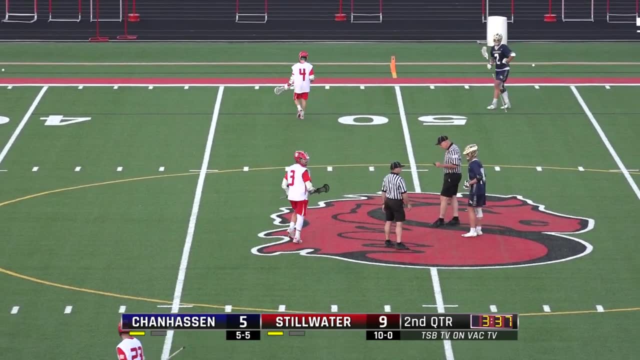 while it's cool to have in the highlights, But Ty Thurston, that was a lot of velocity there wasn't it? It was. it was another strong shot by Ty Thurston, who just has a rocket for a shot- Hard to stop when there's bodies criss-crossing. 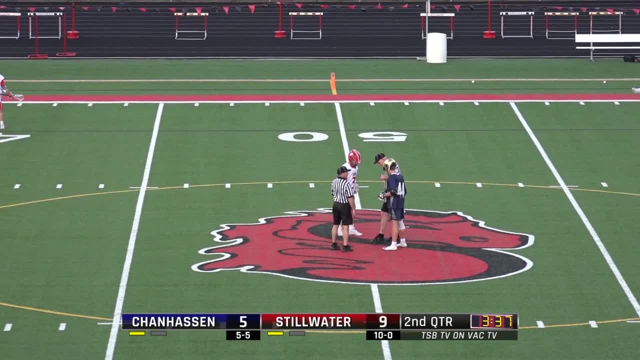 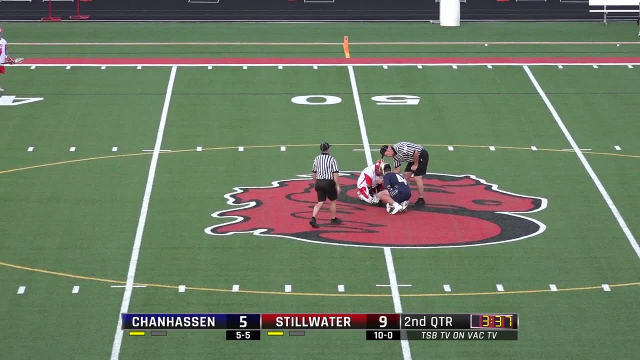 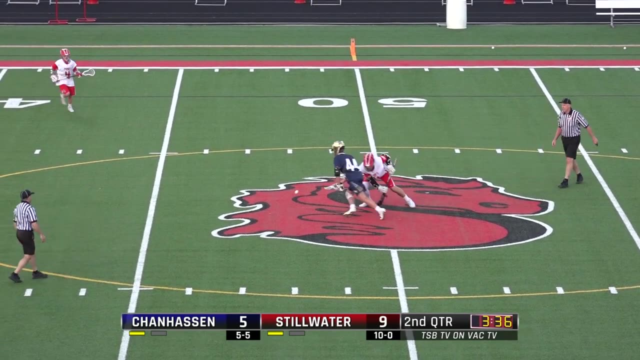 in front of that, goalie Thurston with his second goal of the game: 33 goals this season. He's up to 43 points And the Ponies have scored six goals in the second quarter And that second quarter this season, as we've seen, 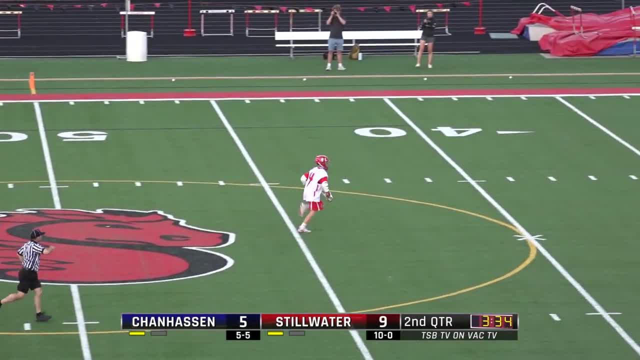 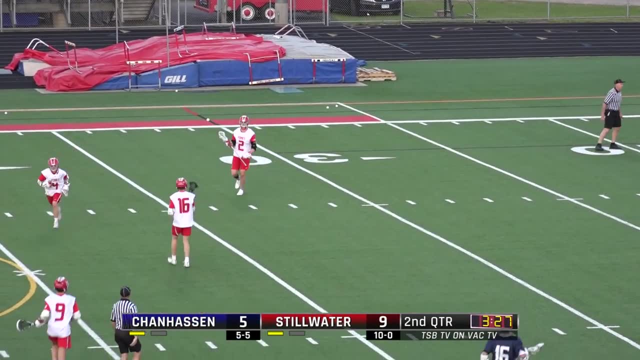 we have a face-off violation on Chanhassen. The second quarter, if Stillwater's in a tight one seems to be where they make their move. That's right, Mike. They'll put some distance between one and the other team if they get that opportunity. 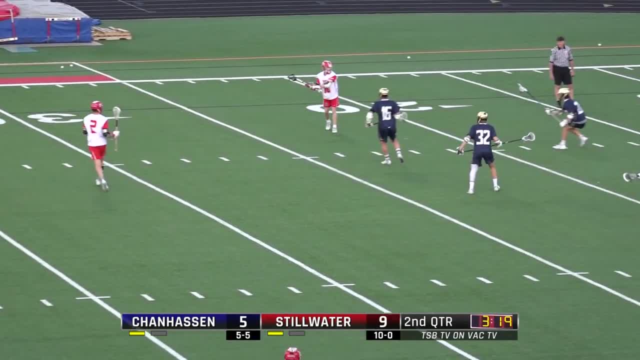 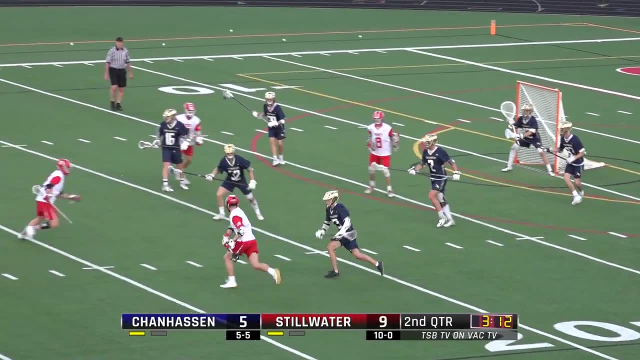 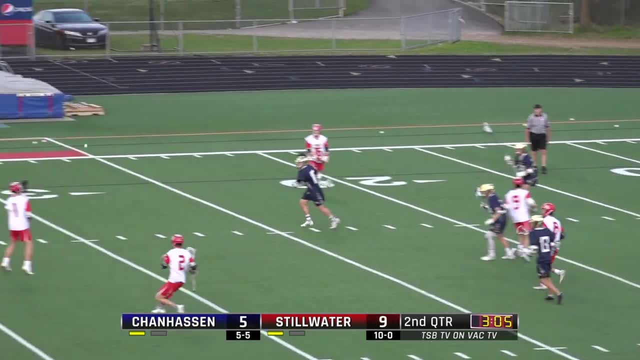 It's a game that's going to be a lot of fun. It's a game that's going to be a lot of fun. This isn't a bad thing for Stillwater either to get some sort of a challenge from Chanhassen. 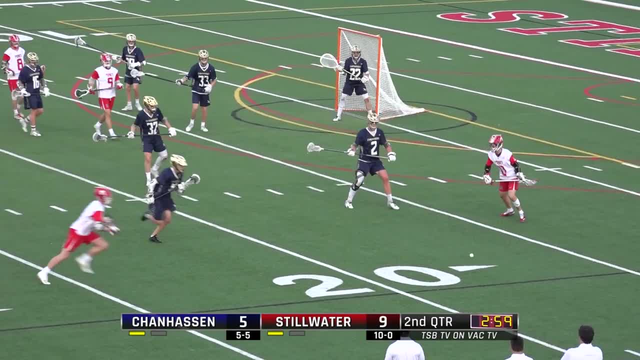 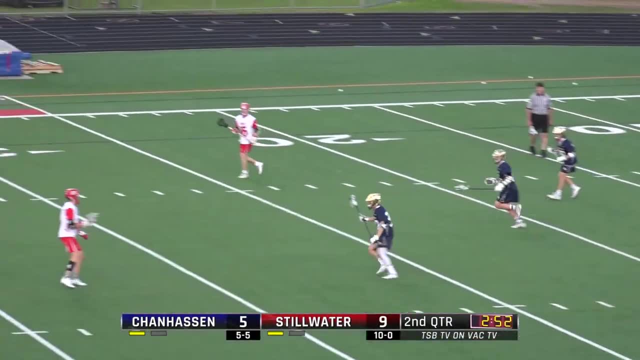 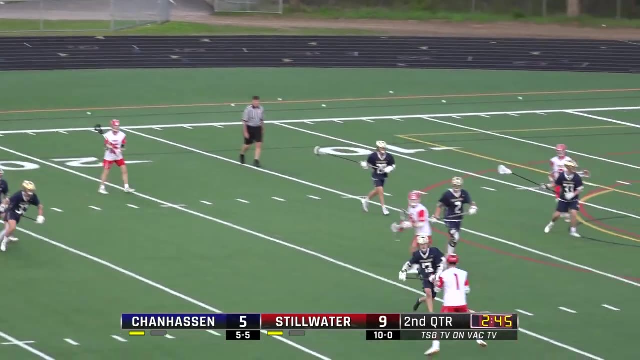 because you don't expect Park to contend And Quinton White lost track of the ball. He couldn't see it. Ty Thurston able to race in there for the save. That's something you don't see often Great team play. One guy can't make it, another guy steps in to do it. 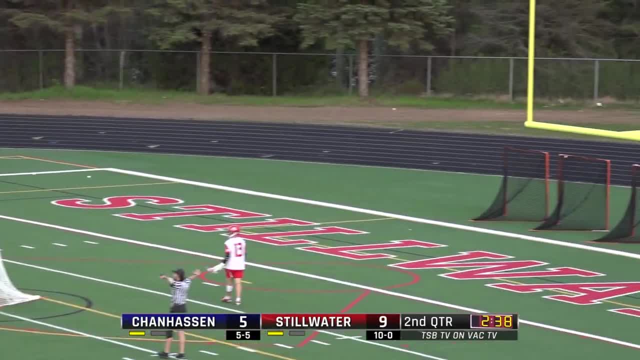 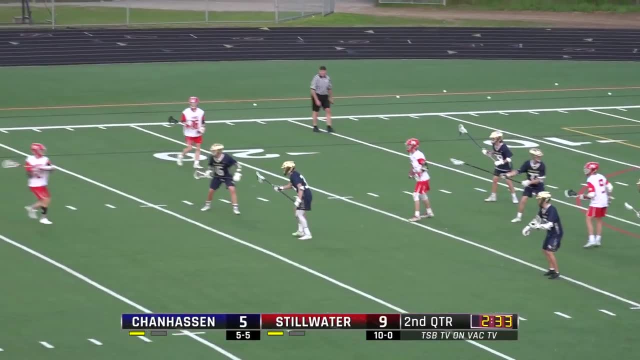 Thurston's shot goes off the crossbar And back out into midfield and Summary will let that bounce away because that was a shot attempt, even though it didn't go behind the net. That time the centering pass for Stengel was off the mark. 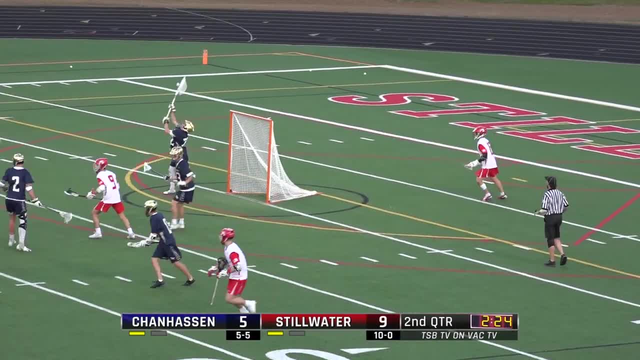 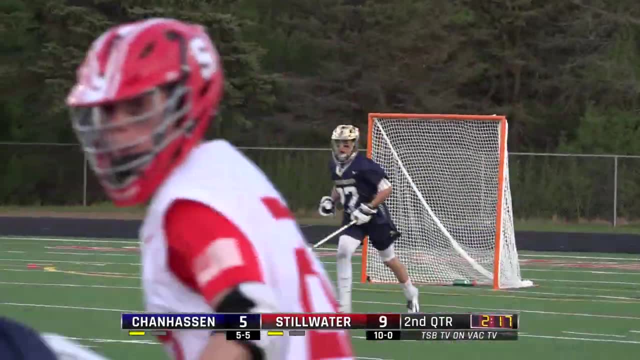 Dorsen, I think he wanted to take another try, Evanson will from the point And Rathie comes up with a save, a much-needed save, for the Storm as they try to fend off that vaunted Stillwater attack. And Rathie's going to take it all the way up. 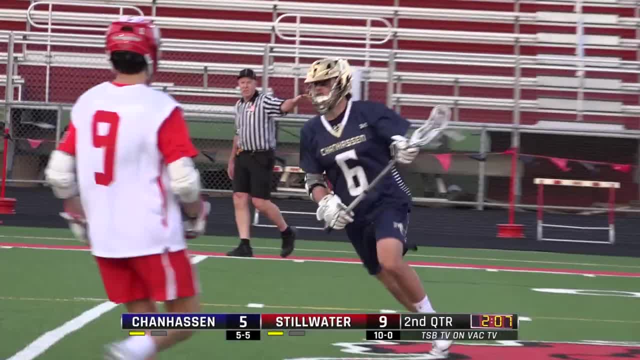 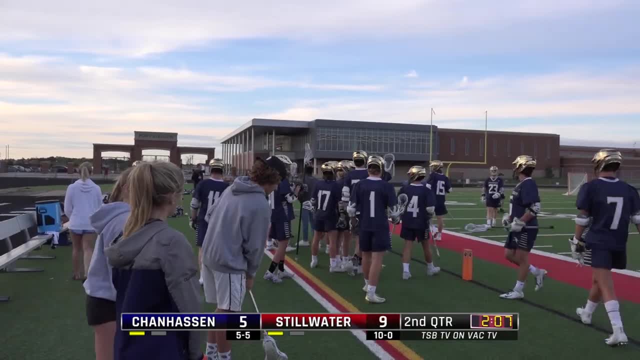 to midfield and he's going to go past midfield. You can do that as a goalie And Chanesson will call a timeout. Maybe that wasn't the design Jonathan Junker was looking for. Well, you don't see goalies cross midfield very often. 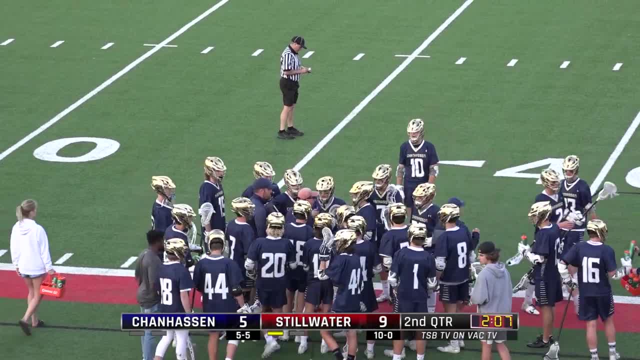 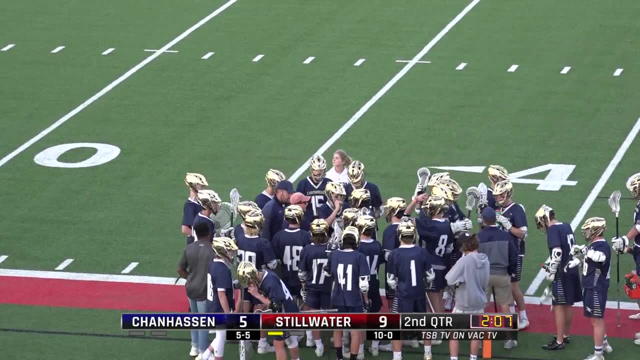 but we did that. Maybe that's what led to the timeout. One remaining for the Storm: 2.07 left in the second quarter. Well, you can really see Stillwater starting to pick up the uh, Pick up the pace. 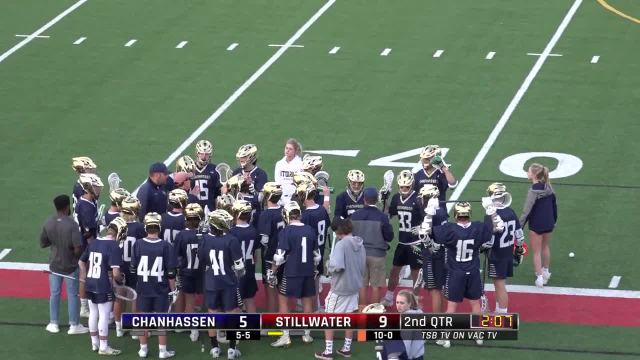 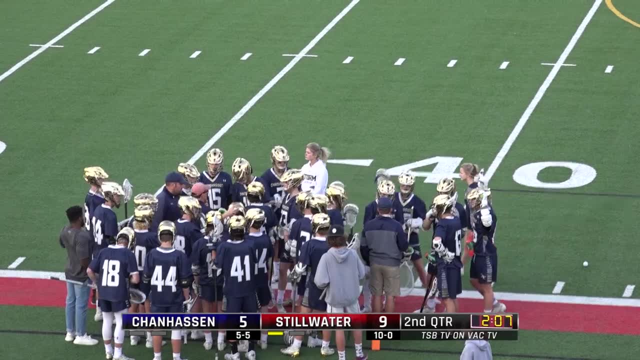 They're just- uh, They're just- reading each other better. They're reading the ball well, They're reading the goalie for Chanesson well And they're getting some nice shots. What I've noticed in this game, compared to the others: 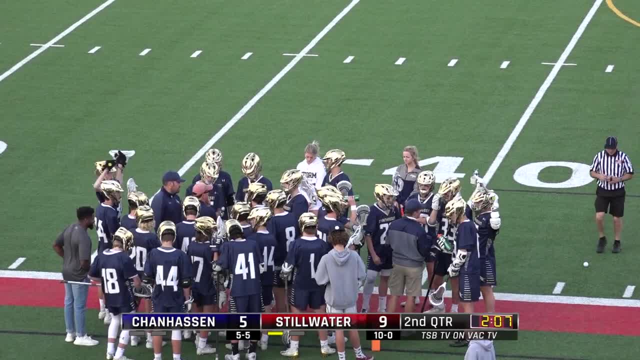 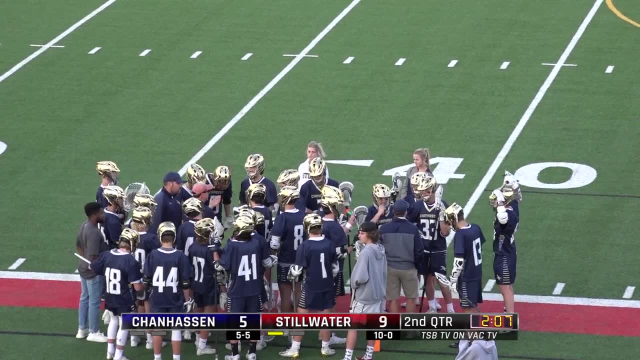 is how quickly and how fluidly Stillwater picks each other up. after a miscue, We saw Cody Berger turn a broken play into a goal back in the first quarter And Quinton White lost track of the ball. Ty Thurston spotted it right away. 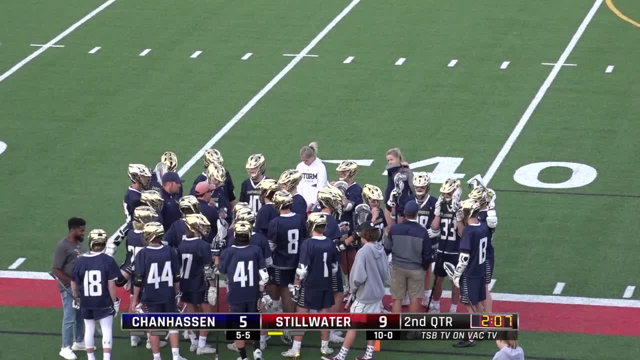 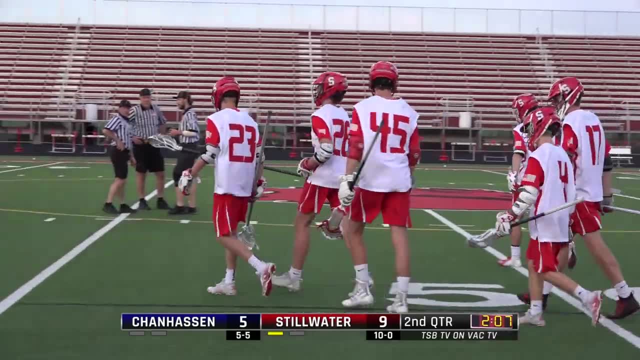 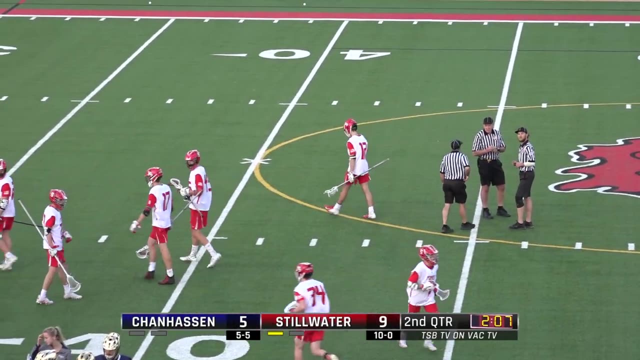 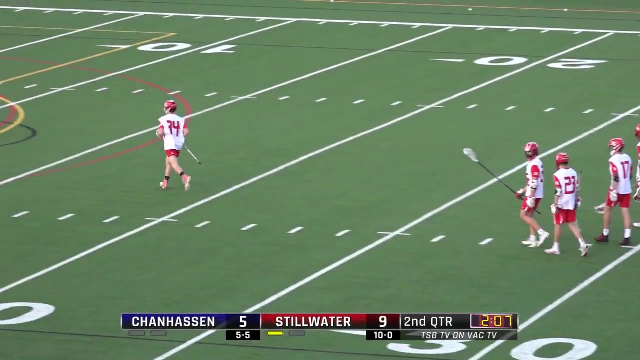 So you have a fallback option in a way, Someone to pick you up. This team is locked in. They're in sync with each other And that is one reason why they have yet to lose. I believe they're undefeated, And if I'm correct here- and I'm almost always right- 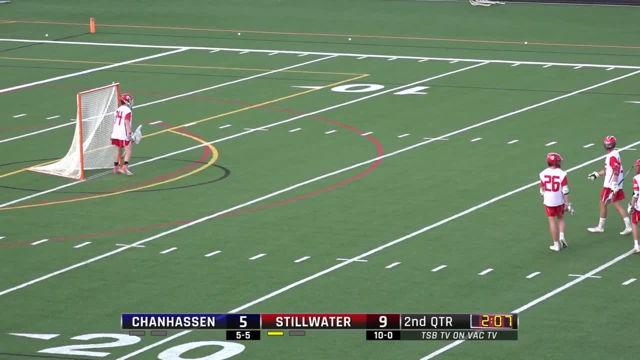 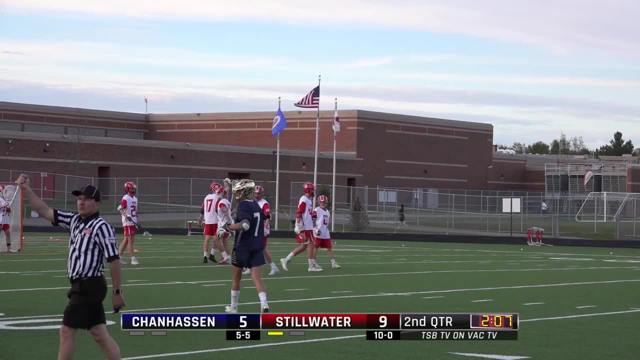 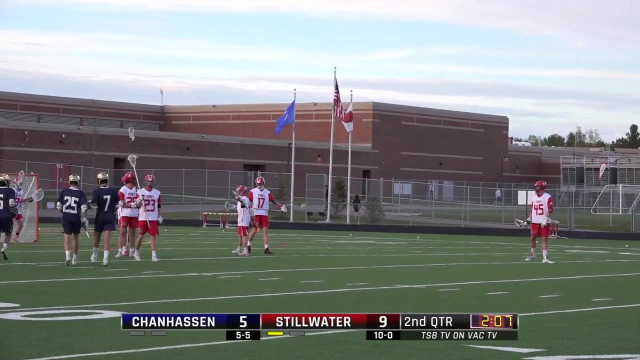 So Stillwater, they are one of two, Two undefeated teams remaining in lacrosse. The other one, the number three team in this state, Benilde, St Margarets. So just two undefeateds left. Only the big boys are left standing in this show. 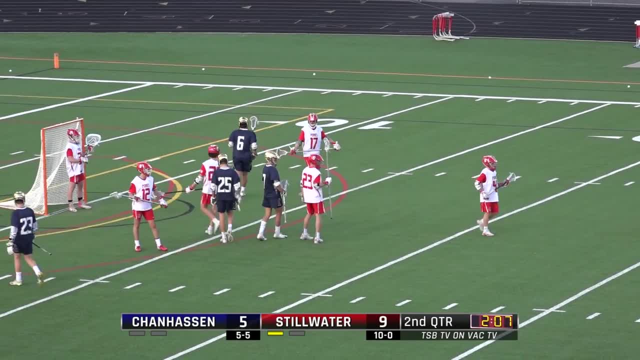 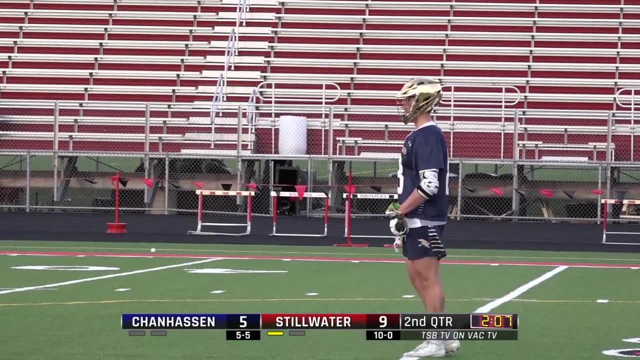 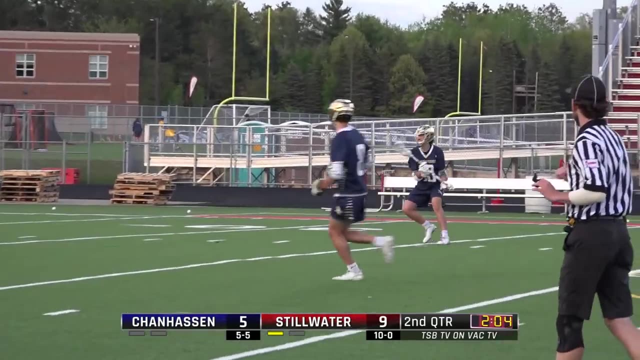 And again, because they're not in the same section. it could stay that way: Benilde, St Margarets in section five, Stillwater in section four. Section three could get interesting. St Thomas Academy Had not lost until facing Stillwater. 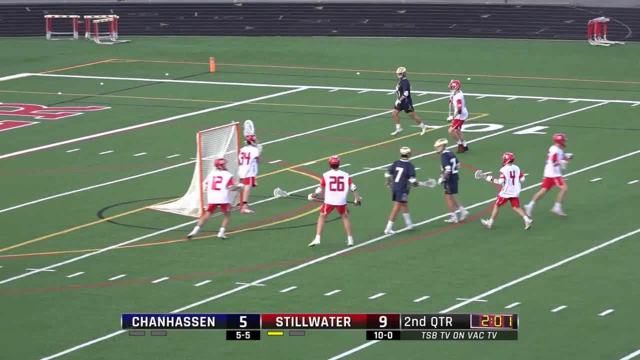 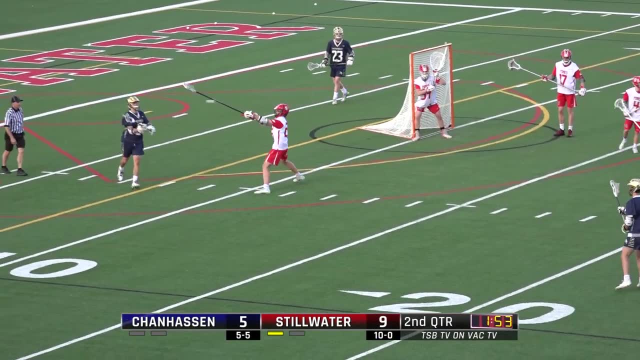 But if you go by, QRF, Eastridge would be the one seed right now And the Raptors a top 10 team. They didn't look like it when they faced Stillwater. Lost that one big, But if you hear the storm, 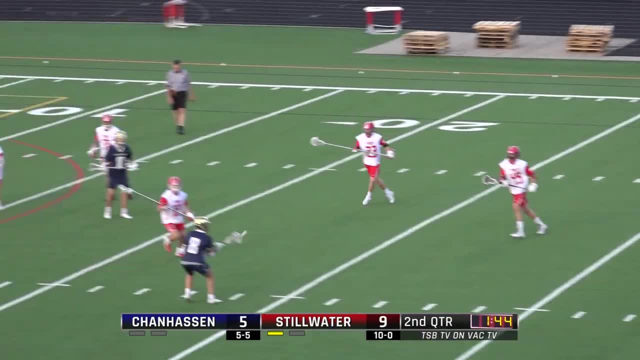 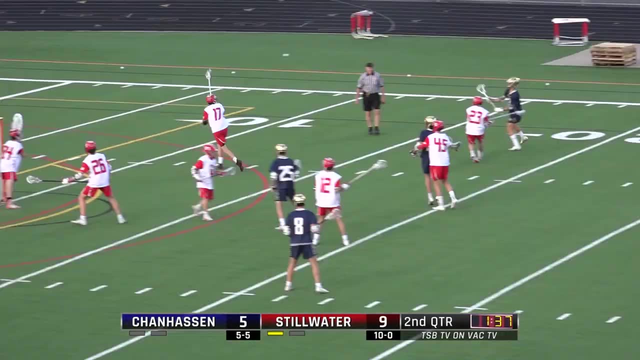 Just got to stay the course. Keep trying to put balls in the net. They were doing a good job of keeping up with Stillwater Almost goal for goal earlier, But Stillwater is slowly outpacing them And I think a big reason for that is Alex Dewey. 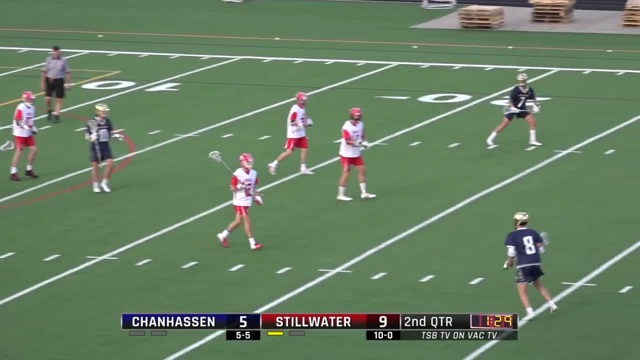 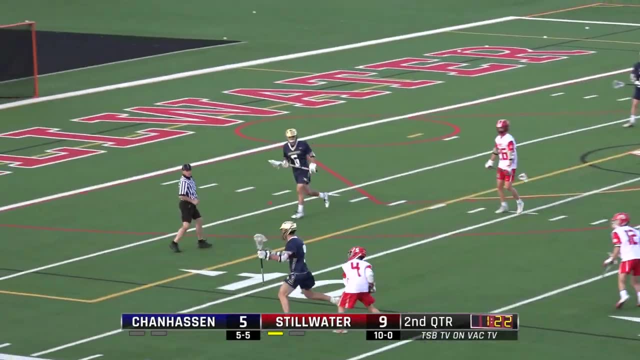 Hunter Holcomb led the team And that's not to say others can't step up. But when you get some other guys it can take some pressure off the big man, Jason Collins, harassed by a couple of Stillwater defenders, He has to go all the way near the sideline. 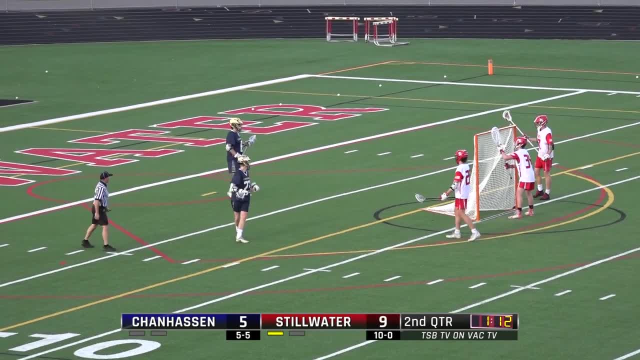 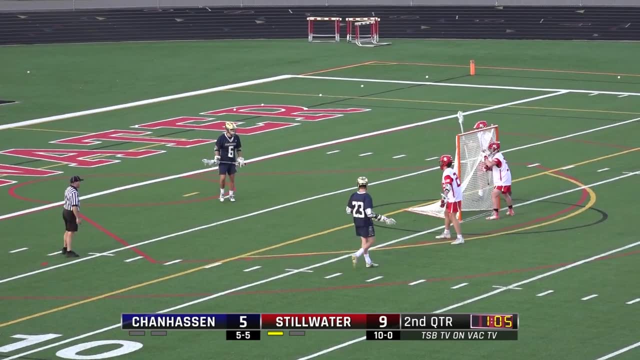 1.15 left. Again, no shot clock, So no sense of urgency yet for the storm. They know they have another 24 minutes after this, But they're going to have to go all the way to the end of the game to build a rally of their own. 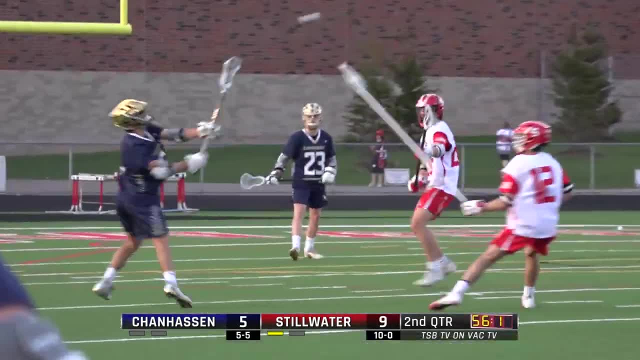 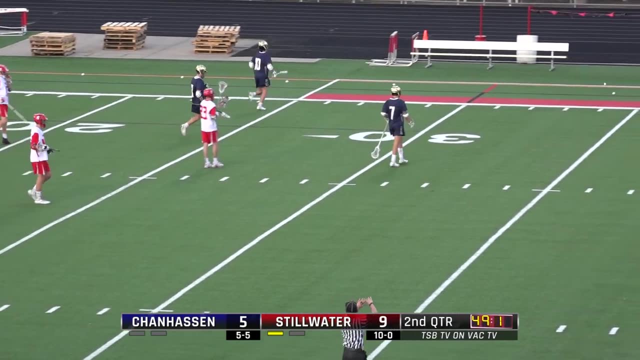 You'd like to have at least one. make it a three-goal game. Dewey, with three of Chanhassen's goals Tried to pass inside Stillwater defense really strong right now. They're not giving Chanhassen anything to look at. 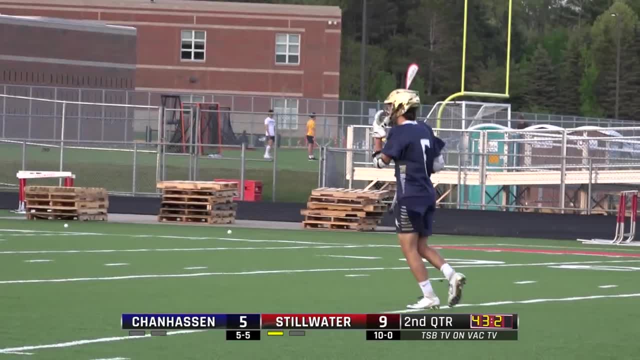 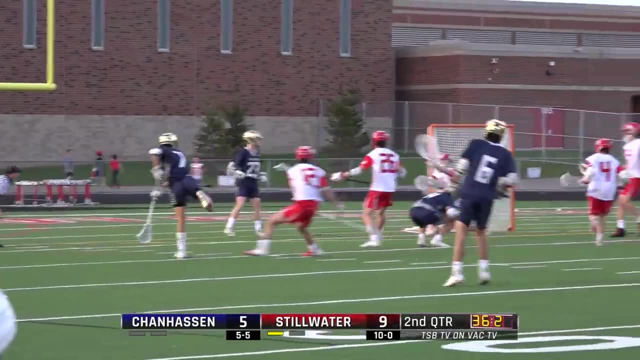 Just forcing him into the outside, Not giving him any inside shots at all. Ben Long, with the deflection It's in Still. Chanhassen Ball with 40 seconds. A tough angle, But Holcomb hooks up with Dewey. 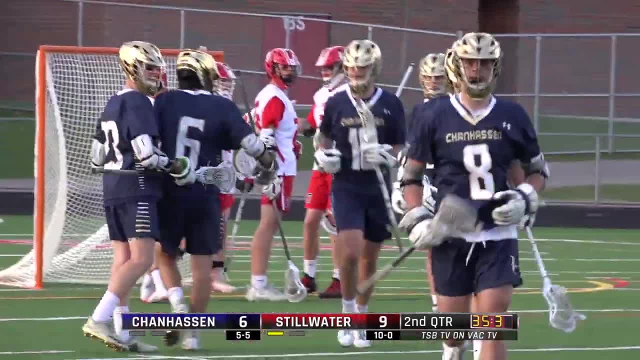 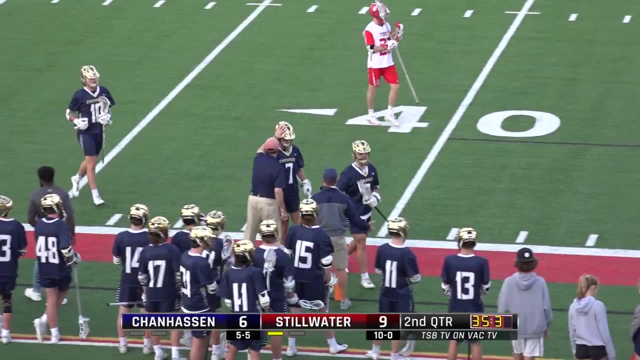 Those two have been the dynamic duo for the storm And they stormed away to a three-goal deficit And as far as momentum is concerned that's a big one for Chanhassen. You know, Stillwater might want to put a little bit tighter coverage on Alex Dewey. 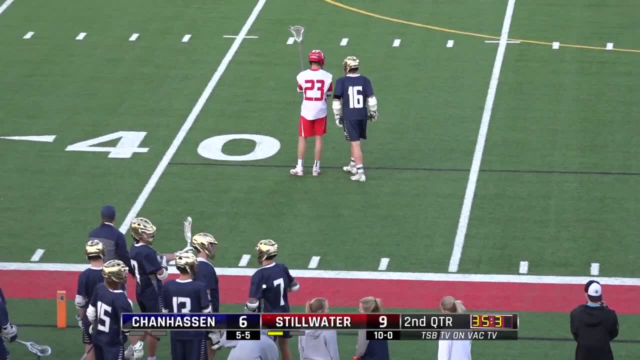 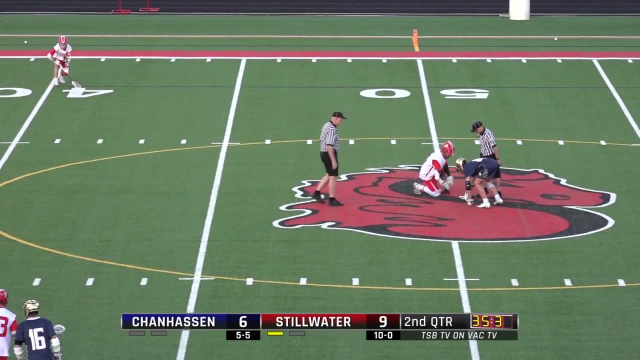 It seems that, since he's doing the bulk of the scoring for Chanhassen, if you turn that spigot off, they could get wet in the score department. I believe that's the first time I've heard anyone use that analogy: Turning off the spigot because it could get wet. 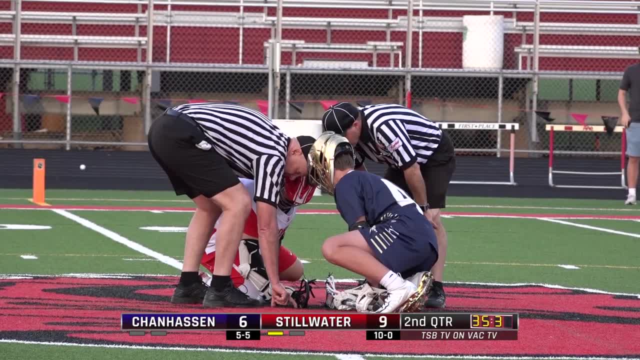 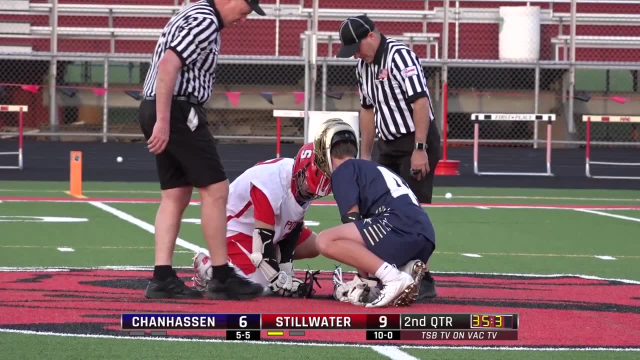 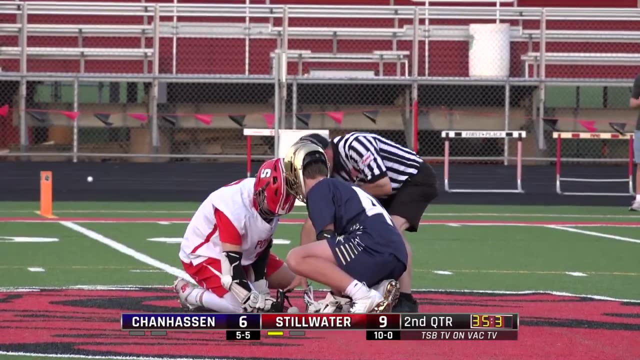 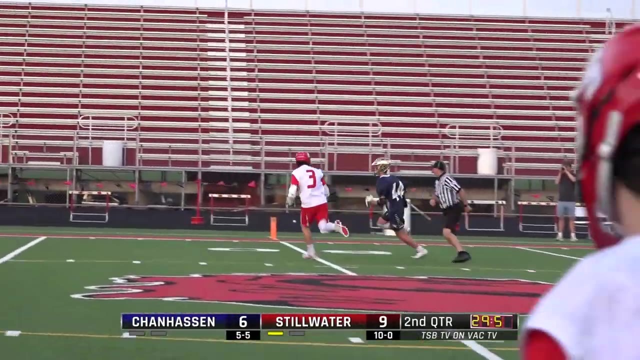 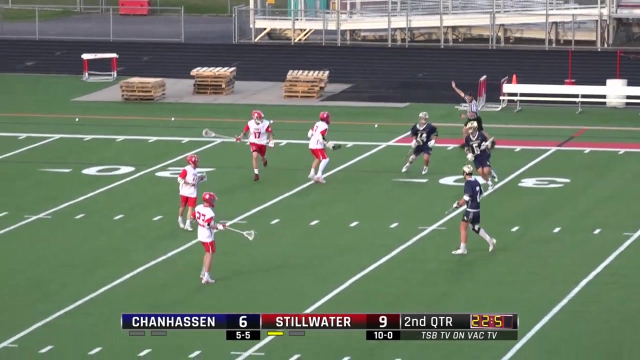 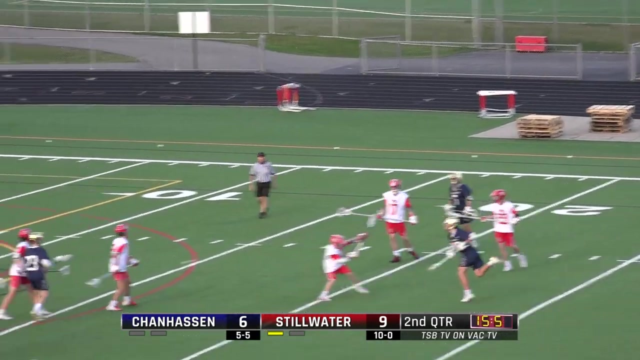 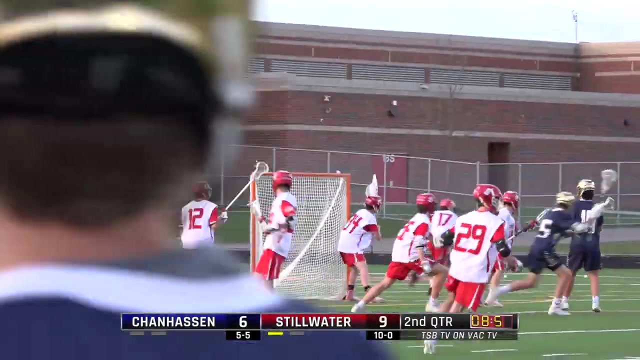 Stillwater, Or I should say Chanhassen, hoping to turn the hose at maximum power. 33 seconds Win for the storm. Critical moment here. Here's Holcomb Finds Manuel And a big save by Ahrens. Manuel was open on the backdoor play. 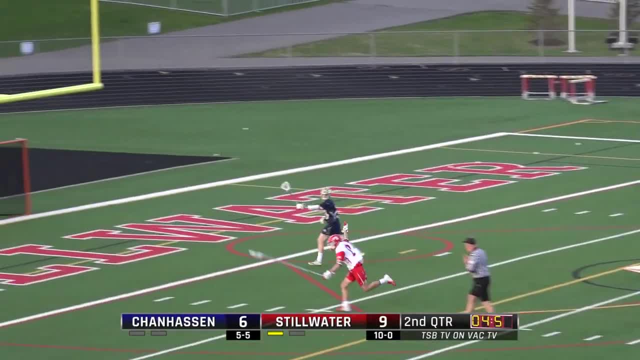 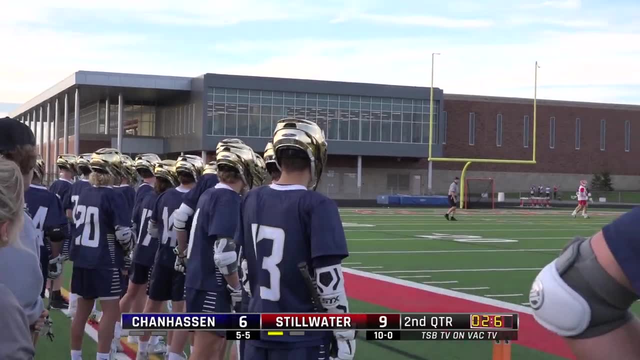 Chanhassen ball. They have six seconds. They still have time And that one was off the mark. I don't know if someone got a stick on Hunter Holcomb. They still have time. They got to get it off And I don't know if they're going to be able to. 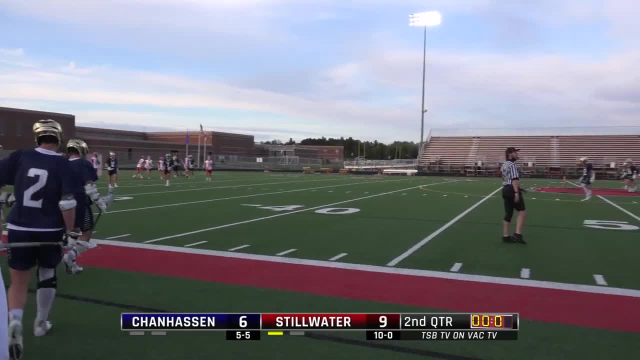 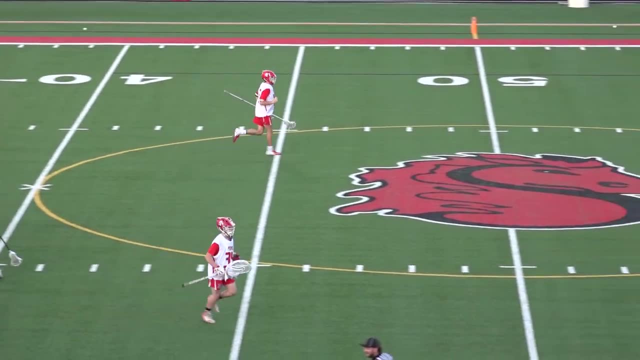 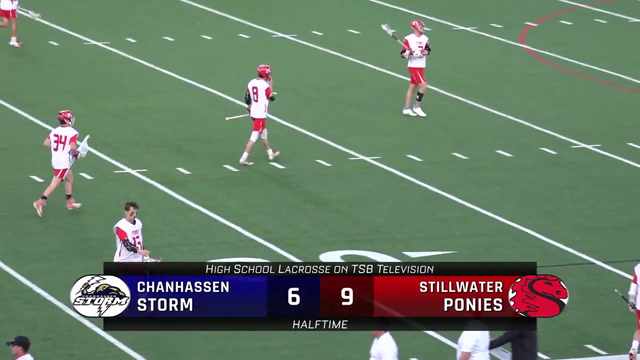 No. So Stillwater with a stingy stand here to end the second quarter, They do outscore the storm six to four, So Stillwater's lead growing ever so incrementally. But they do lead nine to six at halftime. This is about as close as we've seen any team with Stillwater at halftime. 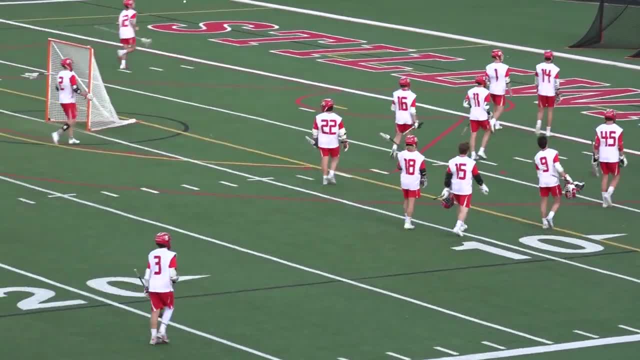 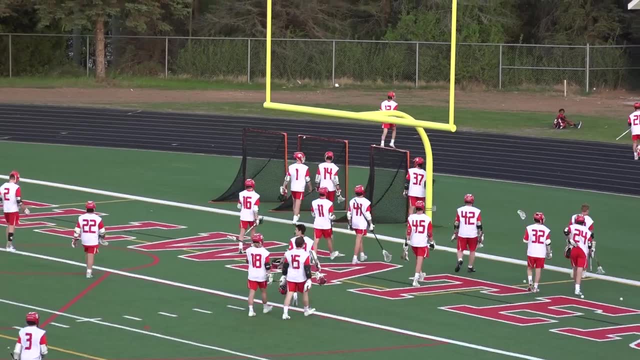 There's, you know, maybe been another closer game, But most of them have not been this close at halftime. They have not. So the ponies have some adversity, Not a ton, But they've got a challenge to work their way through. 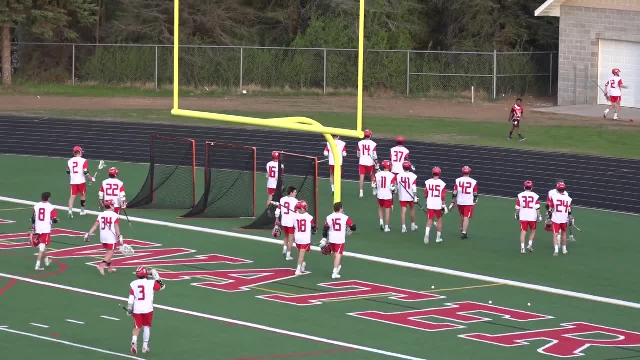 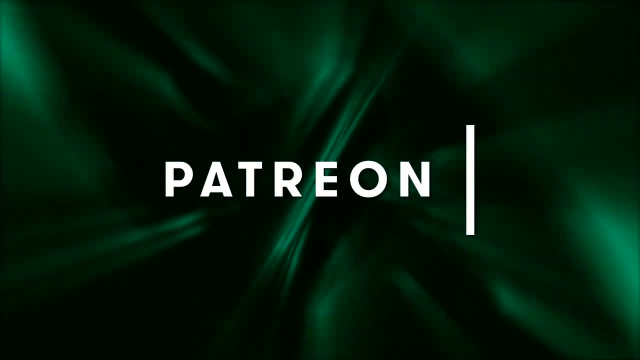 We'll see how they answer it in the second half when we return. You're watching High School Boys Lacrosse. If you'd like to sponsor a TSP television broadcast, Patreon is the place. Sponsorships start at just $1 a month. 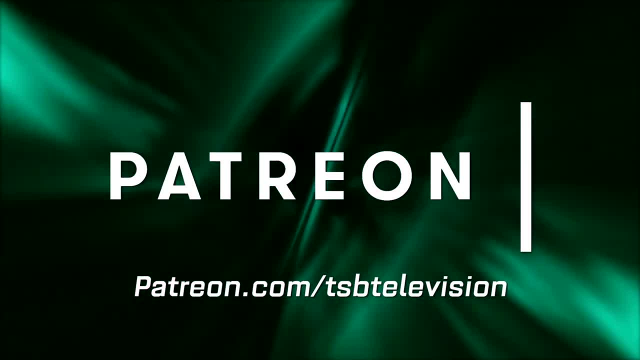 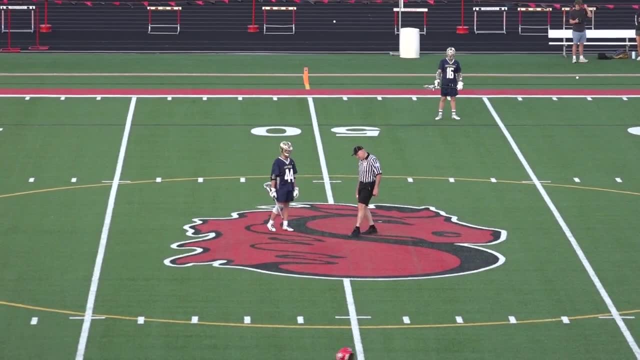 Visit patreoncom, slash TSP television and make a pledge for premier Twin Cities sports coverage. That's probably a reason. All those steps is one reason why I think I've lost about 10 pounds in the past year. Mike, do you have 10 pounds loose? 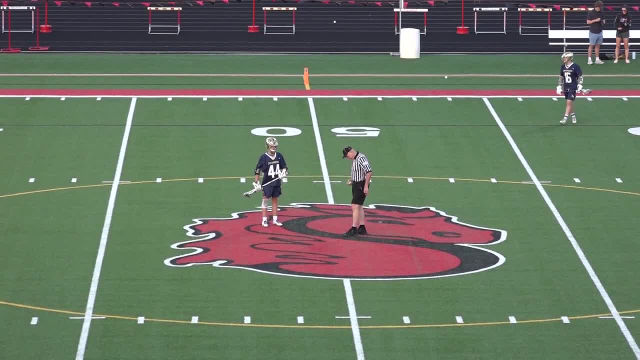 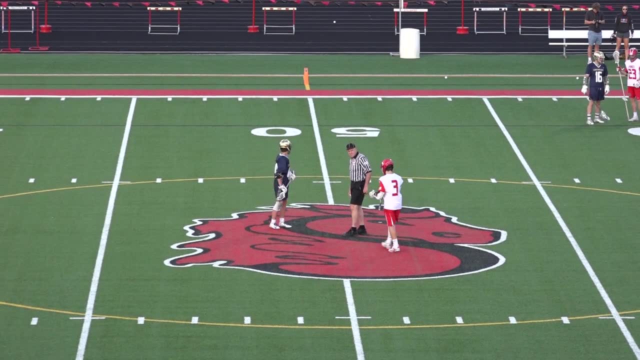 You're already quite in good shape, my man, And on that note, welcome back to High School Boys Lacrosse. Robert, to answer your question, I don't know if I have any more weight to lose, But I'm well under the Mendoza line. 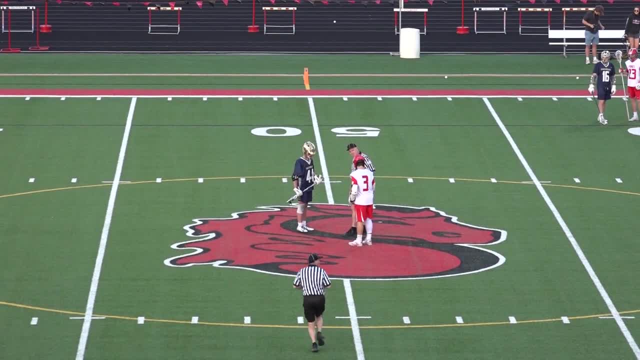 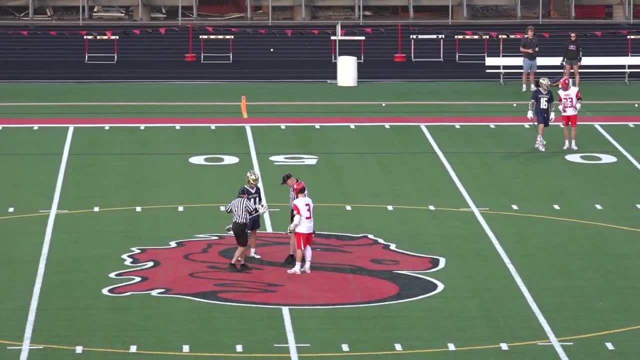 I'll put it that way, But we've got ourselves quite the barn burner here. 9-6 is our score in favor of Stillwater. Joe Stengel, with his fifth hat trick of the year, leads the ponies with three goals. 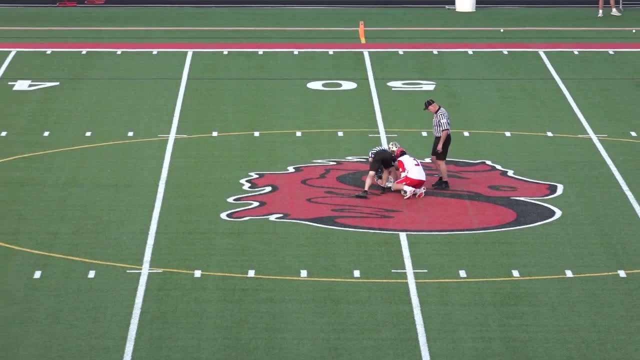 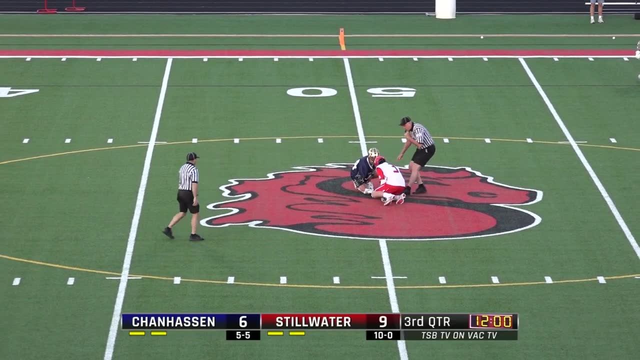 And Alex Dewey for the Storm. a season-high four goals in the first half. Only his second hat trick of the year. Yeah, he's on fire tonight And Chanhassen needs that. They need more of their scorers to come alive here. 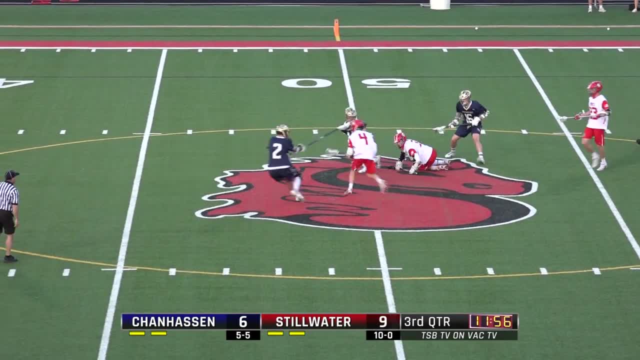 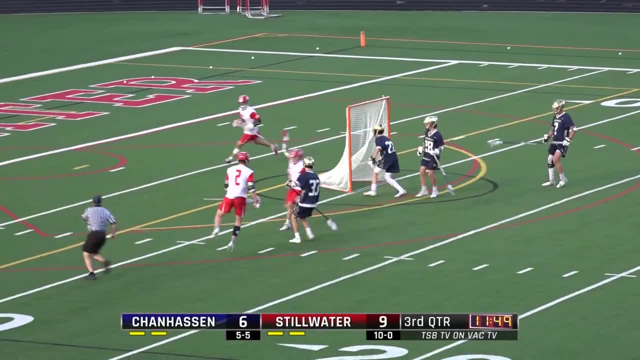 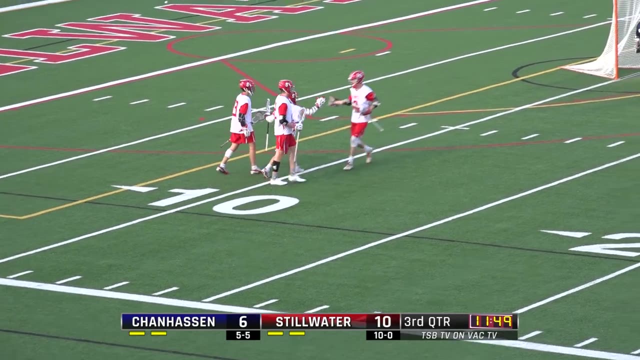 They're putting up a good fight against a hot Stillwater team. Oh, there goes Speedy Ben Carl, And Speedy Ben Carl speeds his way downfield for a score. I was there in the Eastridge game when he took the ball on a short-handed situation. 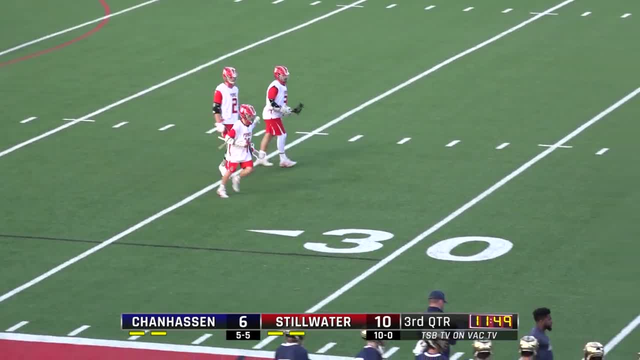 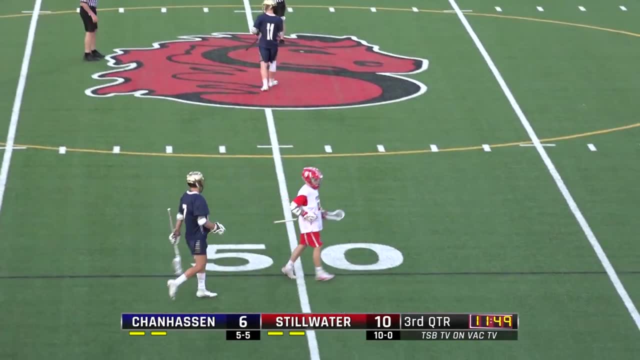 Took it all the way downfield end-to-end for the score. Didn't need to go as far that way. Didn't need to go as far that time, But I can't think of a more electric way to start the second half for Stillwater. 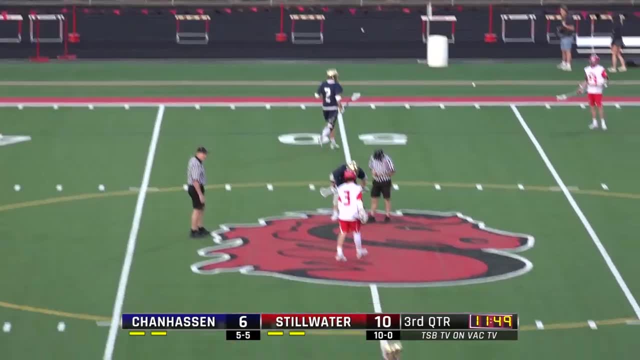 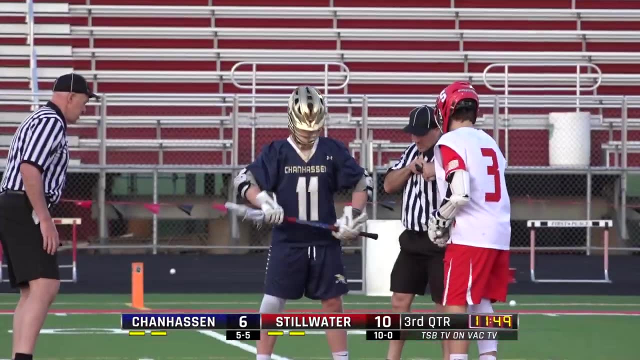 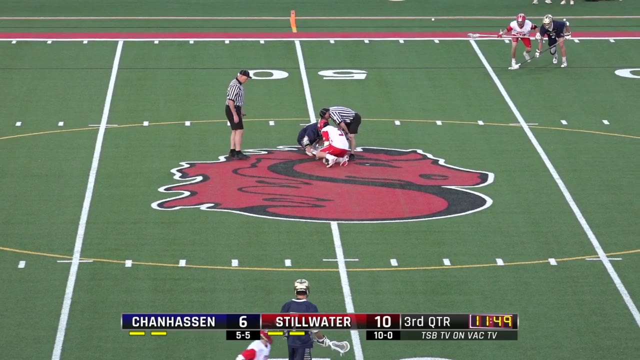 And for the ponies their second quarter is a big one, But it's a good start to the third, as the ponies keep their double-digit streak alive 11 seconds in. So Ben Carl doesn't score a ton. That was just his third goal of the year, because he's usually the guy who brings it up midfield. 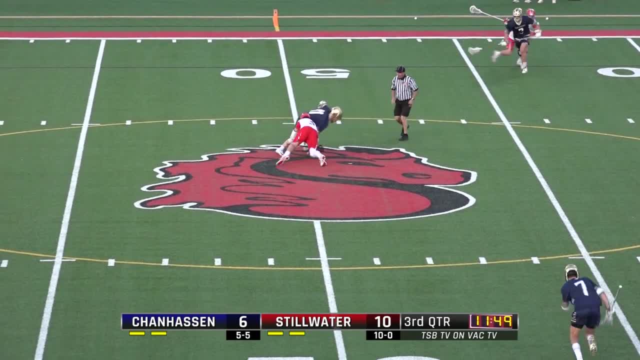 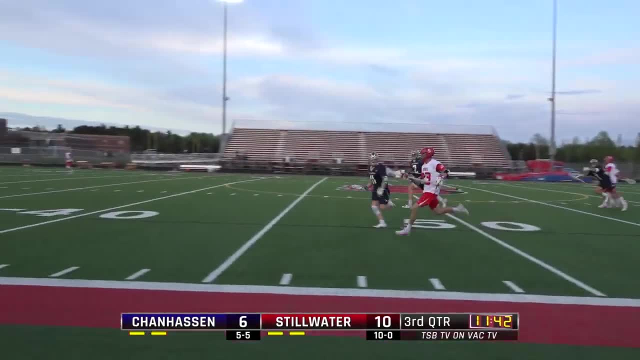 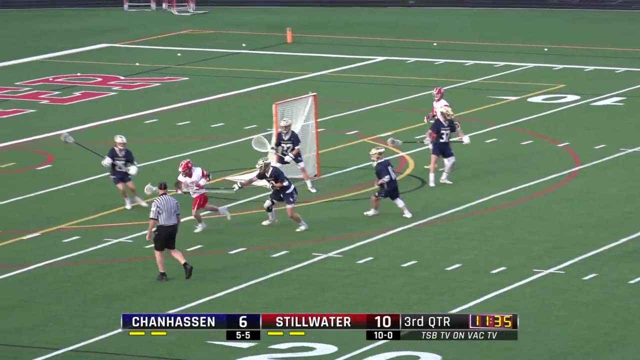 uses his speed to get the ball up and keep possession for the ponies, Ben Carl will graduate. So, Robert, they're going to have to find another source of speed next year, But Tom Ho has done a fantastic job elevating this program. 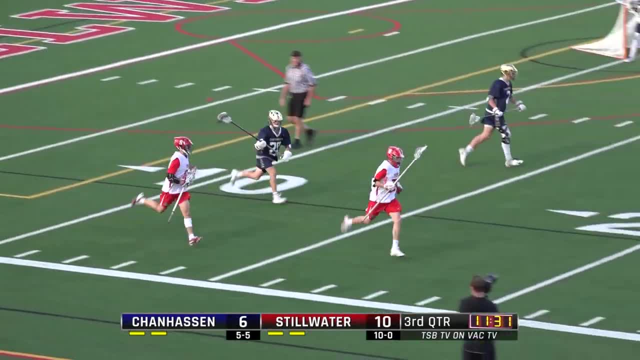 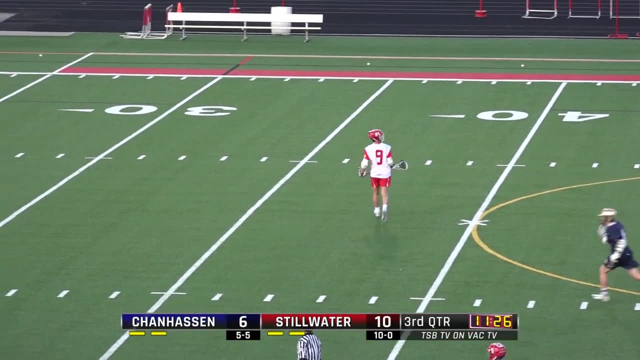 They won another face-off And Ben Long- he was looking to join the party- Couldn't do so. There we go, But that's all right. The ponies have steadily increased their lead. It hasn't been that dominant, runaway fashion that we're used to. 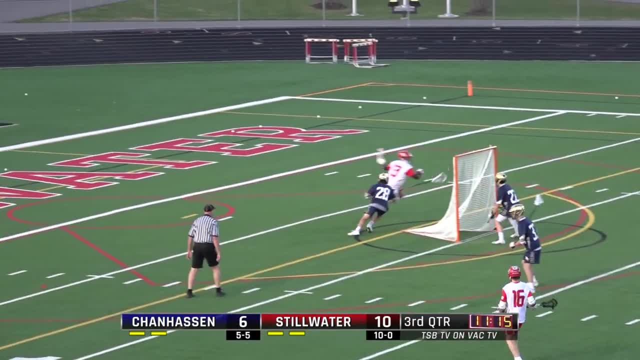 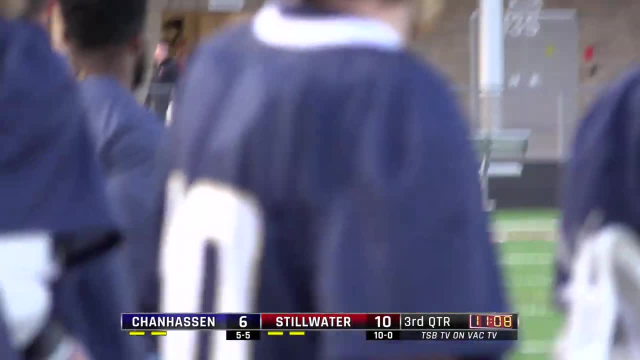 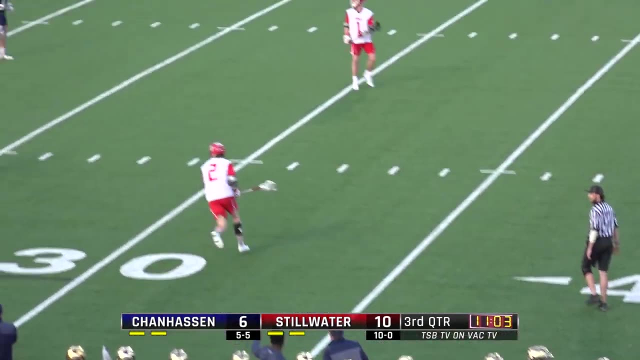 But at the end of the first quarter they led by one. At the end of the second they led by three, And that will be Stillwater ball. Come on, Tony, Come on, Let's get it That one Good. 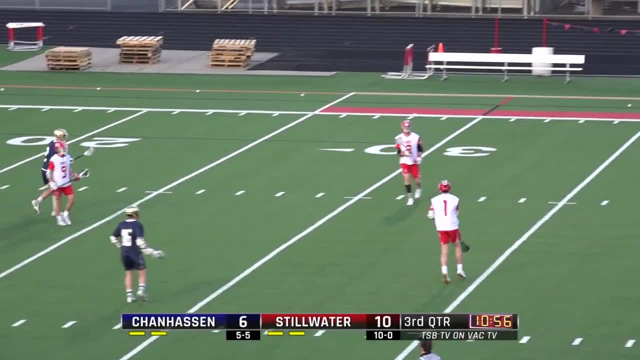 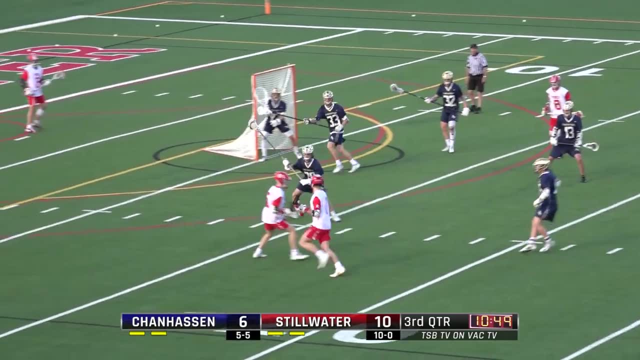 And a score update. You know that game. we won't know the result of it until this one ends, But Edana Minnetonka in a tight one right now. Minnetonka, as we noted, already dropped their first game of the year. 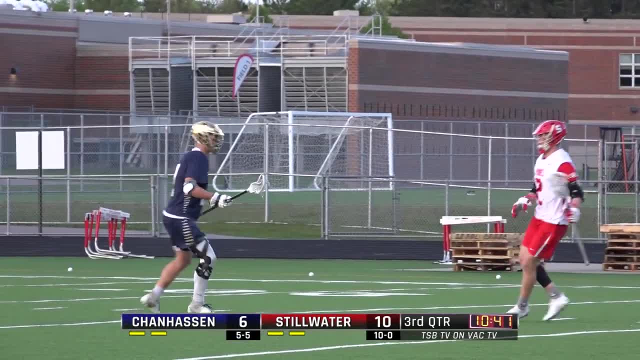 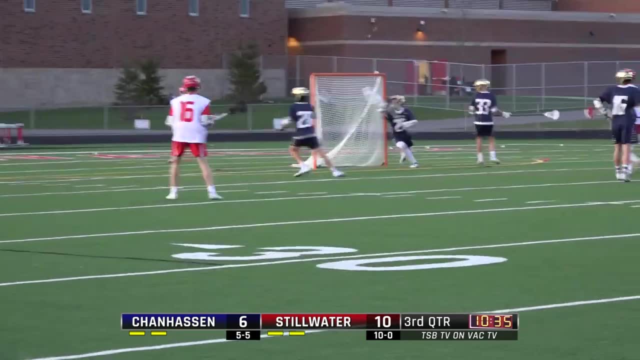 And Stillwater figures to take over the number one spot, should they stay undefeated by the time we get to next week's poll, which could be our last of the season, with next week being the last week of the regular season, Evanson hooking up with Thurston there. 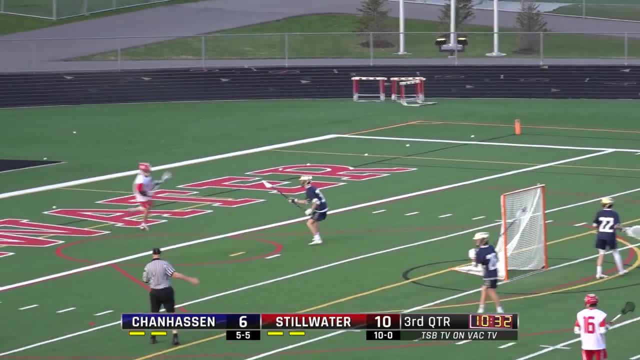 And Thurston with another sidearm shot. Stillwater maintains possession. A great fake by Evanson. I thought for sure he was going to shoot it. It was a nice pass, of course. Evanson's known for that misdirection. This time he tries the centering pass. 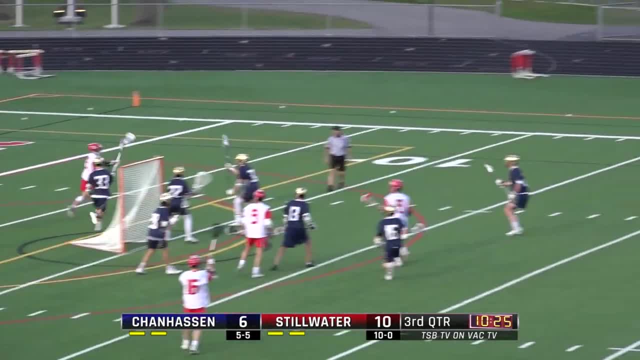 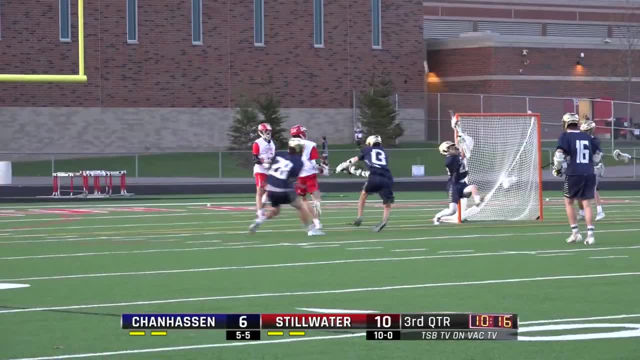 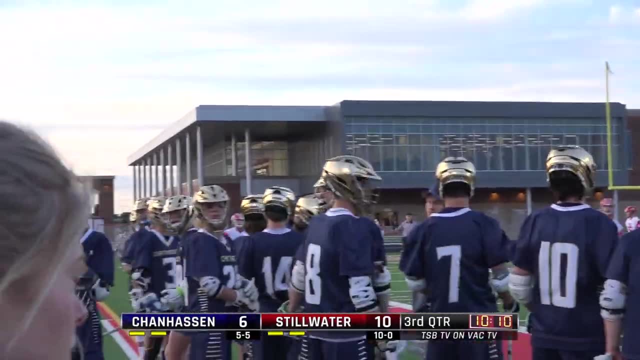 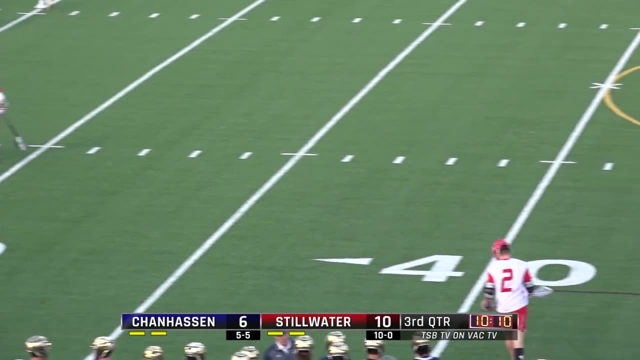 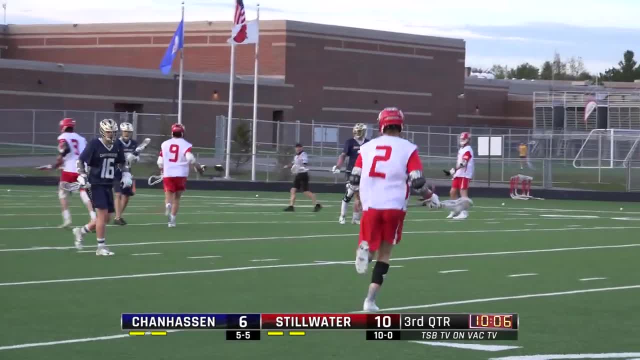 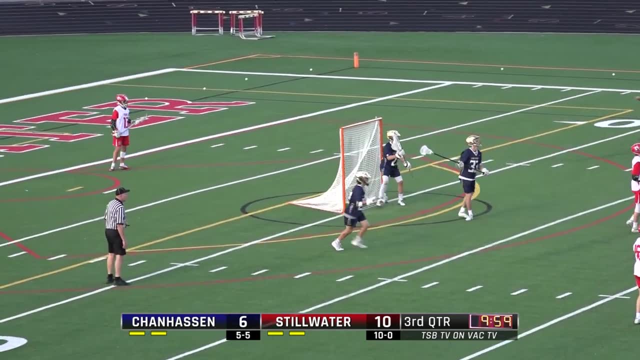 Come down. As we said for the Ponies, not necessarily used to getting a challenge, They have led throughout, so it's not like they've had to play from behind. Whoa Thurston's shot went off the crossbar and right into the stick of Evanson. 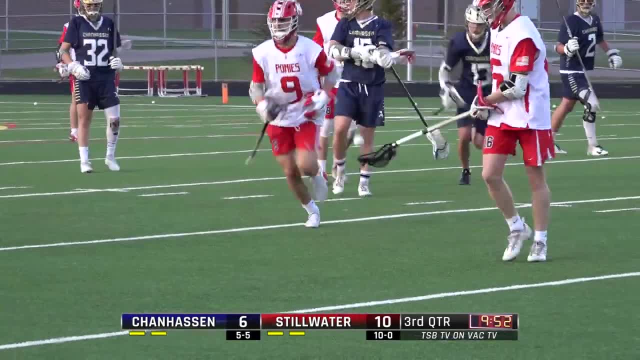 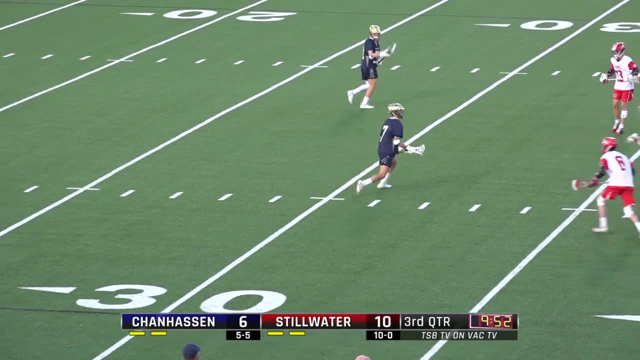 Then he tried the centering pass. That's off the mark Ball's loose And that's going to be a foul on the Ponies. So Chan has some ball Now. Thurston: He has two goals. He could have had four. 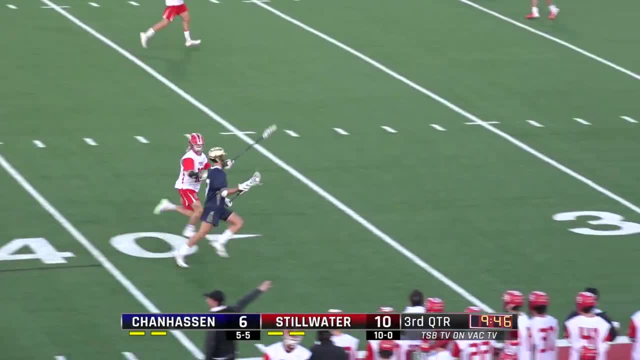 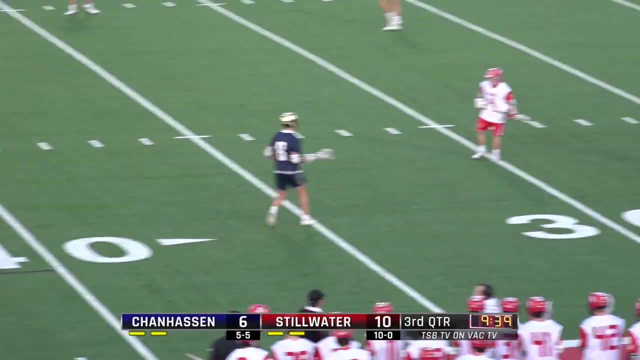 He's had a couple of shots missed by inches. And look who's got the ball. at least for the moment, It's Ben Dewey. We'll hand it off to Jason Collins. Alex Dewey, I should say, not Ben Dewey. 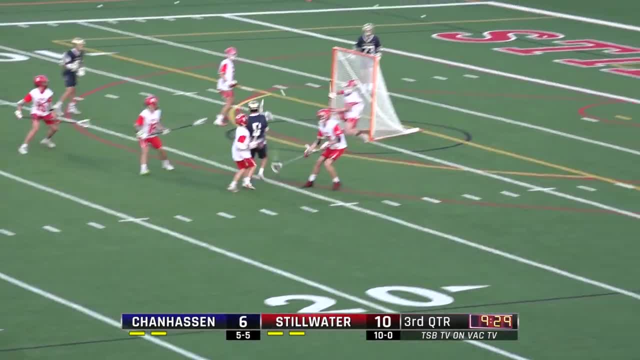 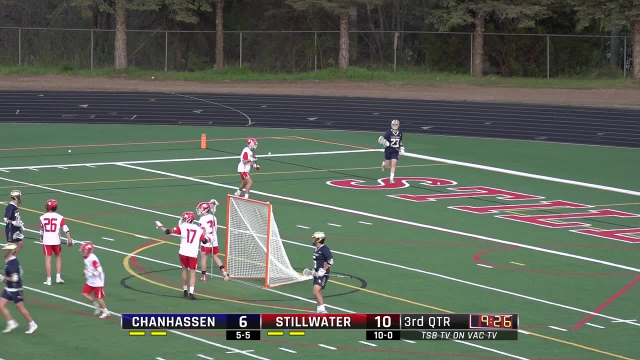 I hope his parents won't hold that against me. Collins was hit from behind, I believe by Karl, And a good stick check by Karl Knocked Collins. off balance It stays Chan-Asson ball, but Collins doesn't get a good shot off. 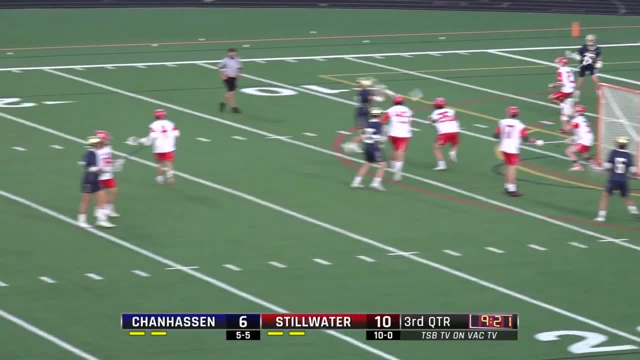 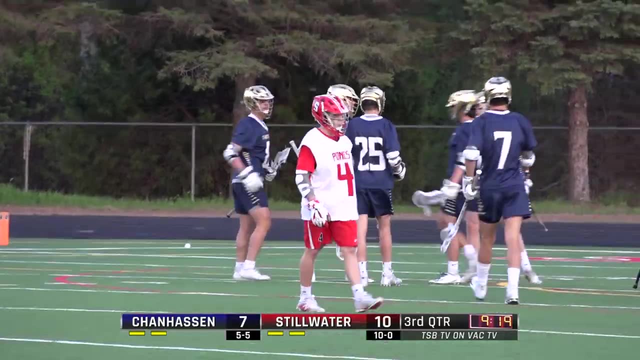 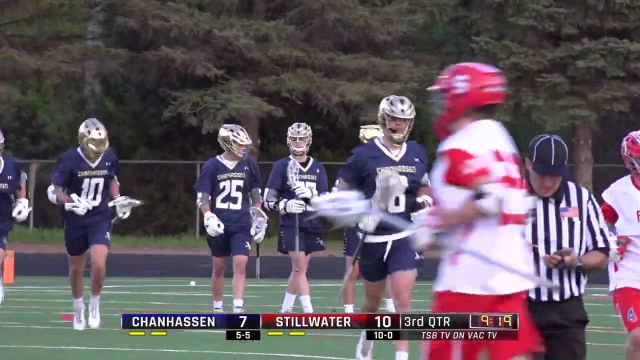 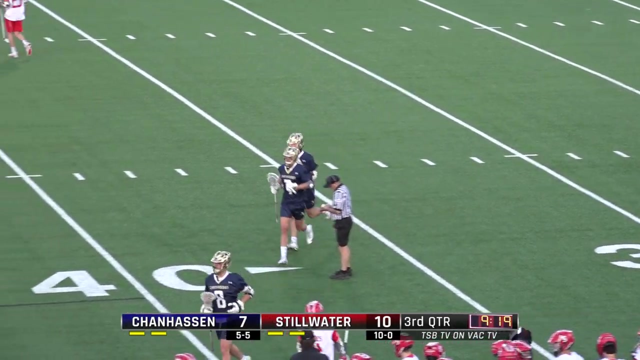 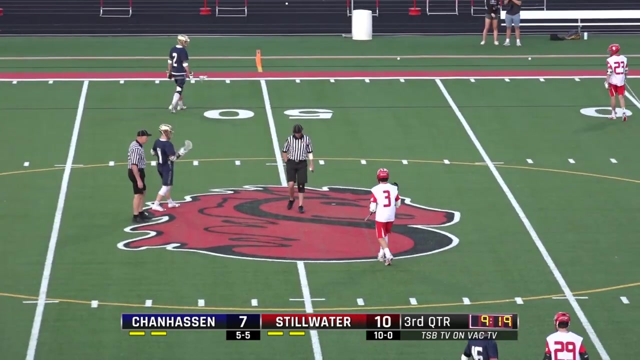 And that's the key Chan-Asson scores. anyway, though, I think Cal Davis got the assist And the goal will go to Tyre Christensen. They're waiting for confirmation. Makes it a three-goal game, though. Okay, it was Hunter Holcomb. 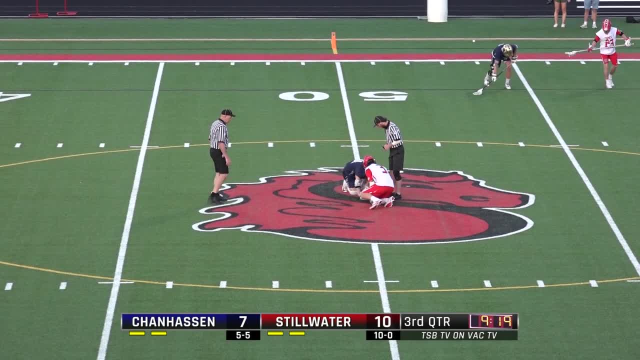 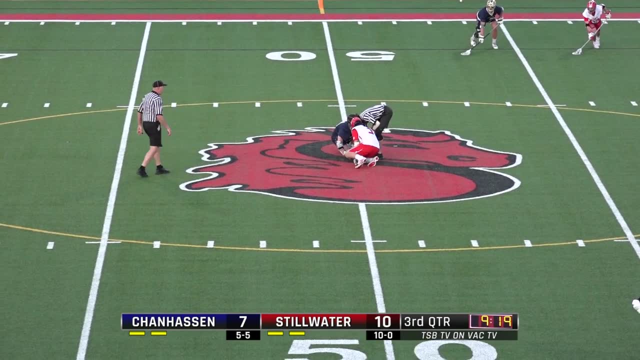 I missed it. initially I knew Cal Davis got it off to somebody. It looked like it was Christensen, based on the celebration, But it is Holcomb. So Cal Davis with one goal and an assist And Holcomb with his second goal of the game. 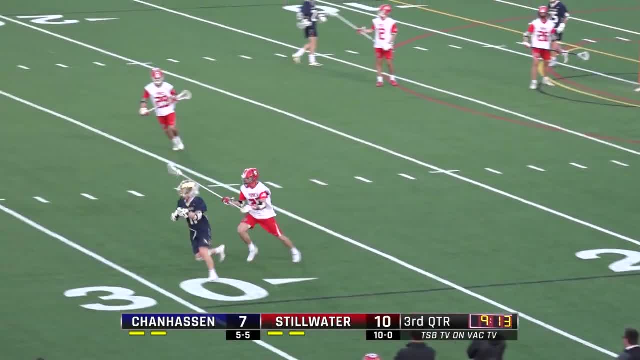 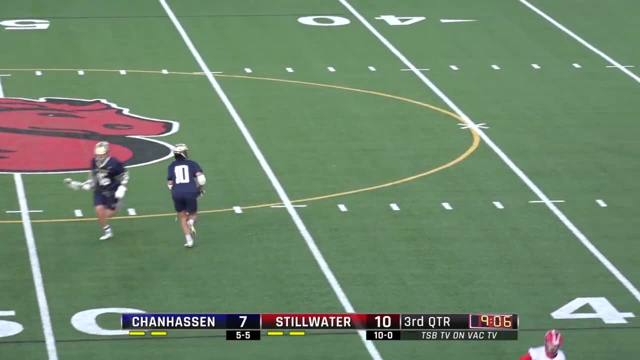 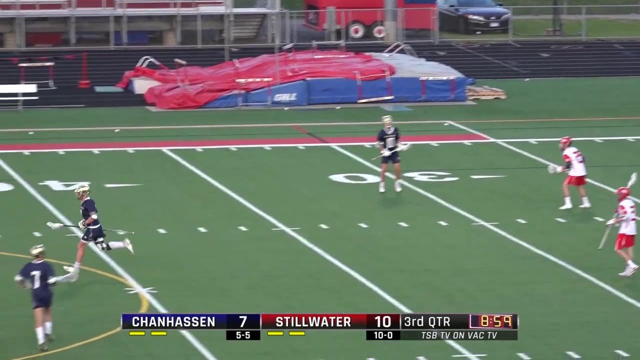 Another face-off win for the Storm. One thing they have not done is go on any kind of rally. They've alternated scores with the Ponies. Okay, Vincent Manuel was the one who scored, So everybody was wrong. Well, you can't be right all of the time. 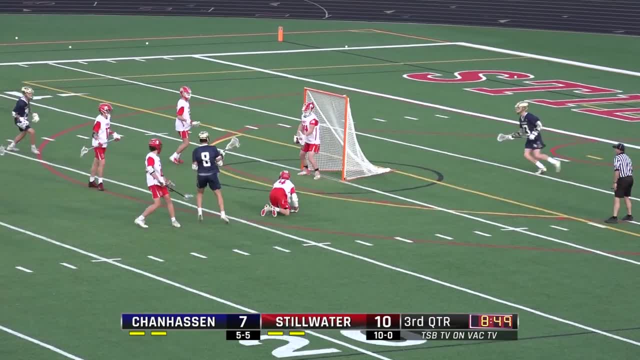 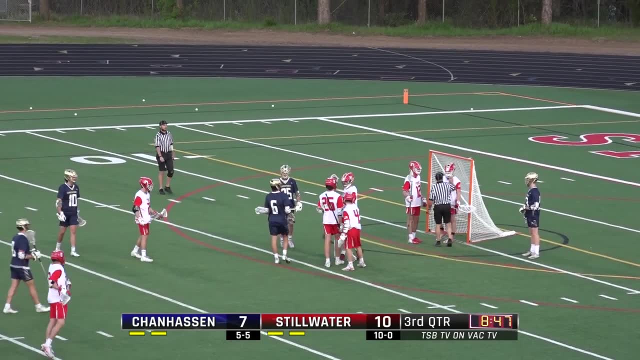 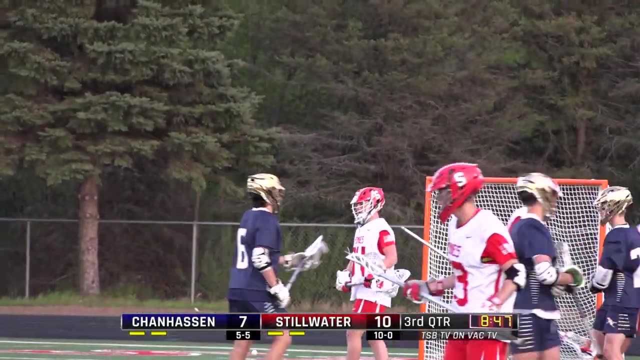 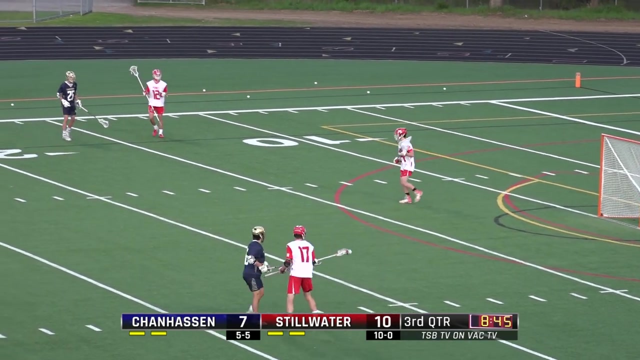 Here's Jason Collins. Looks like it might have hit him under the chin, But he looks okay. Gunner Ahrens goalie for Stillwater Chin save. It is a chin save And the little one Chin save in the literal sense. 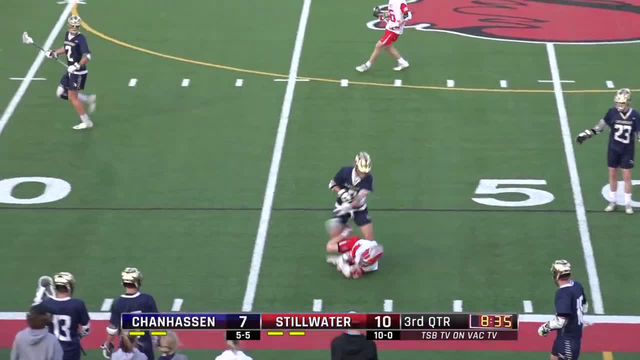 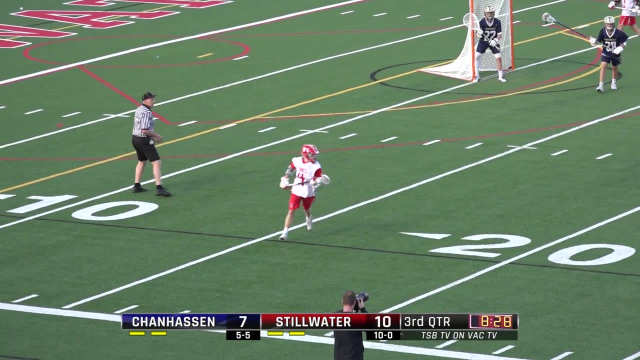 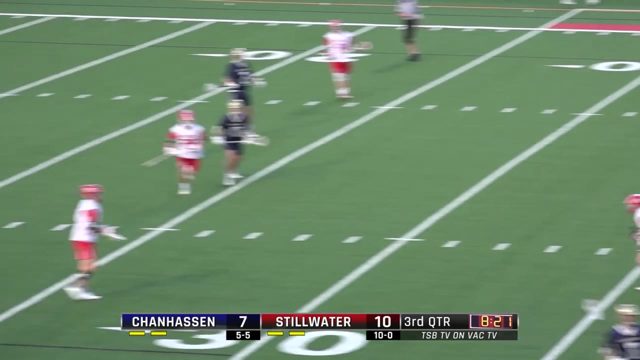 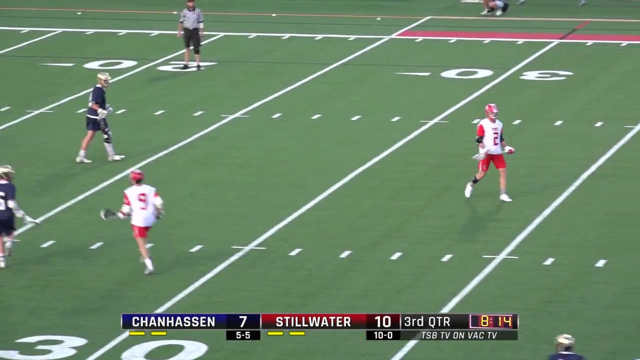 That's going to leave a mark. Carl hit from behind. No flag, But Carl gets back up, Maintains possession. I'm surprised a flag wasn't thrown. It looked harsh enough from up here. But we play on And Carl got back up. 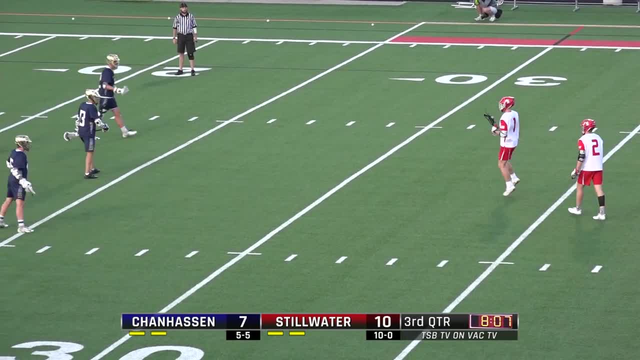 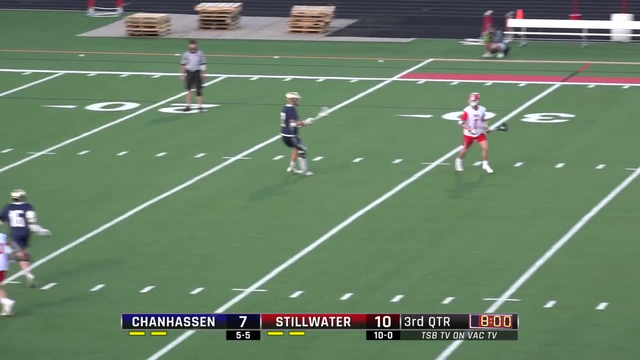 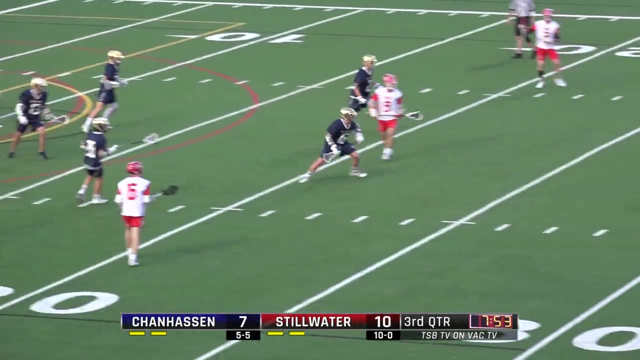 I think he was going to take a look to see if he could channel his anger into a scoring opportunity there. But let's see if his teammates can handle that for him, As they have for her so many times in this 2019 season. 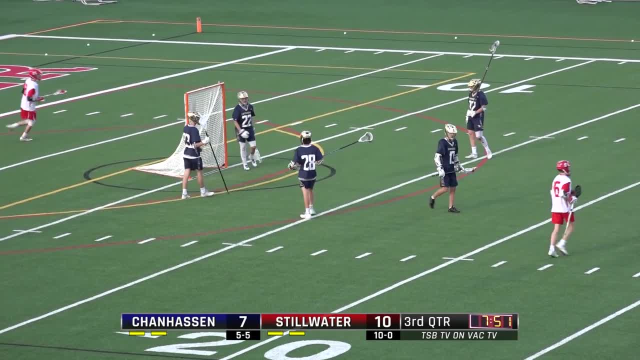 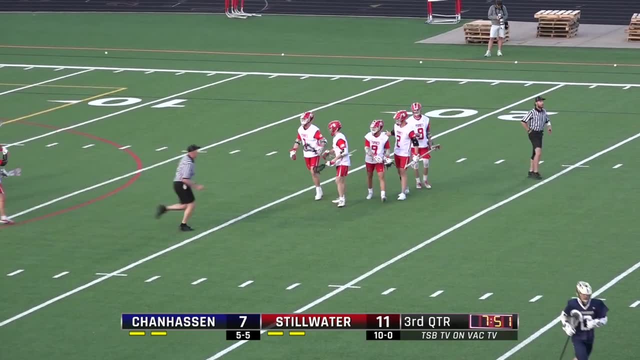 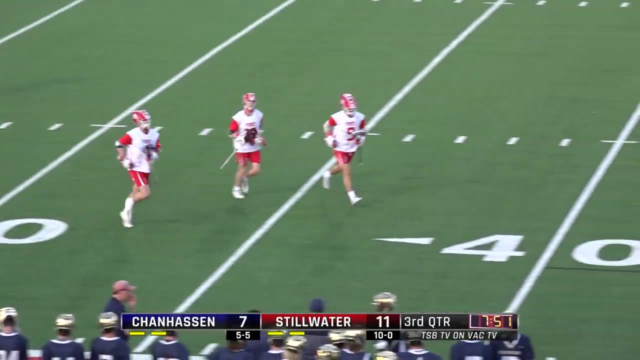 Pass back out. Shot from the point: Ty Thurston, Thurston with a hat trick. Robert, This is another common thread with the Ponies, And they're scoring. It's not one player that gets hat tricks, It's multiple players who pick up hat tricks. 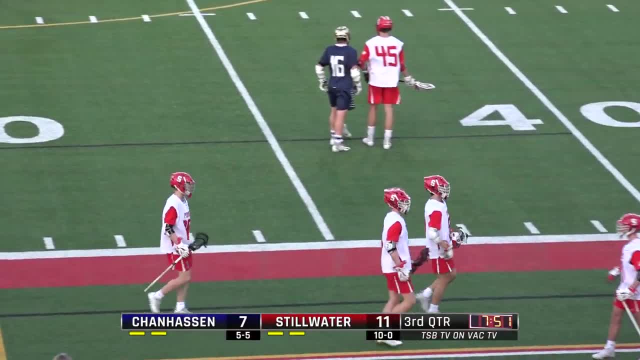 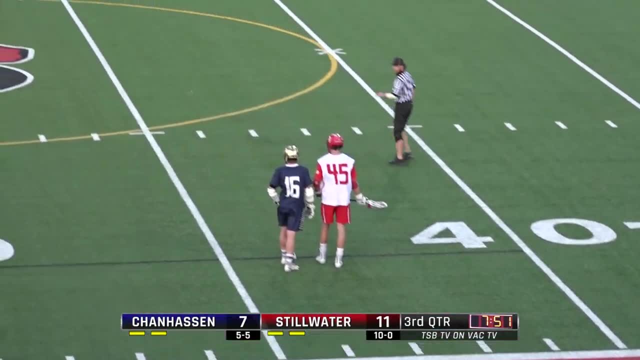 And you know that's a good sign for Stillwater. That means that they're in the game. When they've got multiple people scoring for them, that's really a positive sign going forth in the game. Now they've got to keep this up. 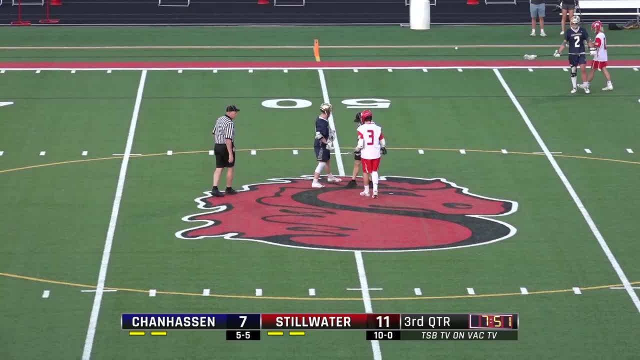 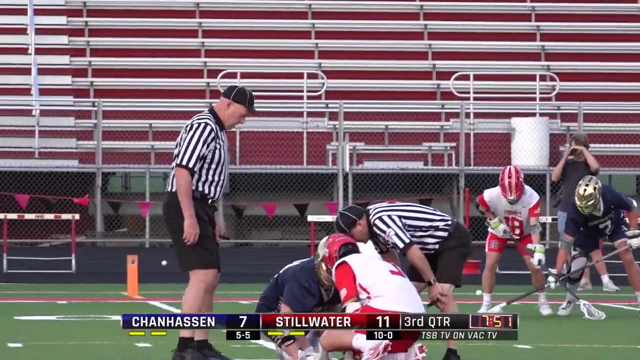 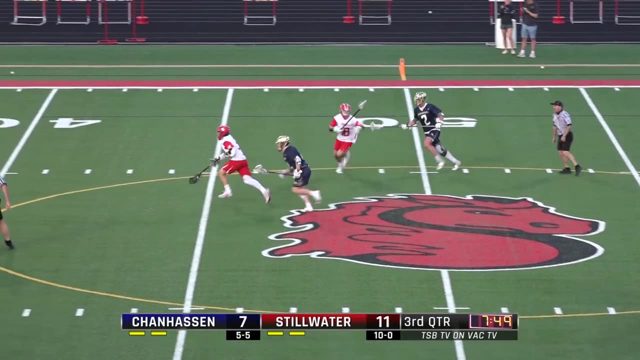 They can't leave. Chain has to keep creeping up on the score. That could be problematic getting toward the end of the game For Stillwater if they let that happen. White got the assist for those keeping track Stillwater: another face off win. 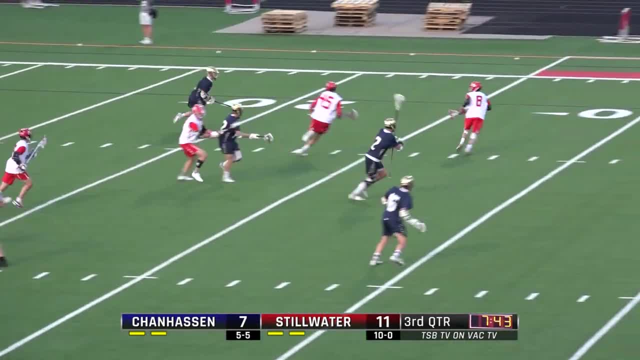 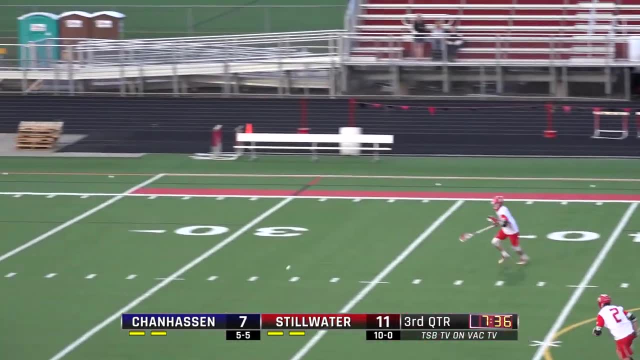 Pushing toward the goal, They lose it in the slot to Chanhassen Stick check from behind. Ty Thurston, by the way, picks up his eighth hat trick of the season And the Ponies answer with a stick check of their own. 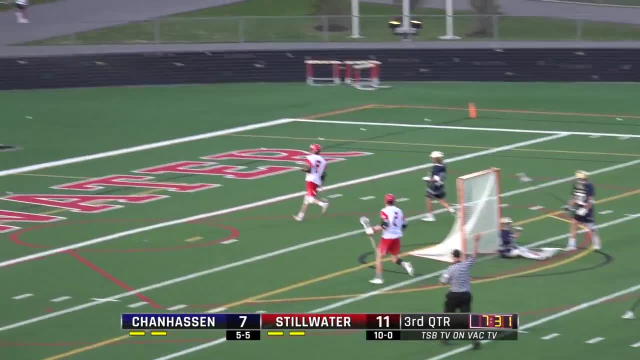 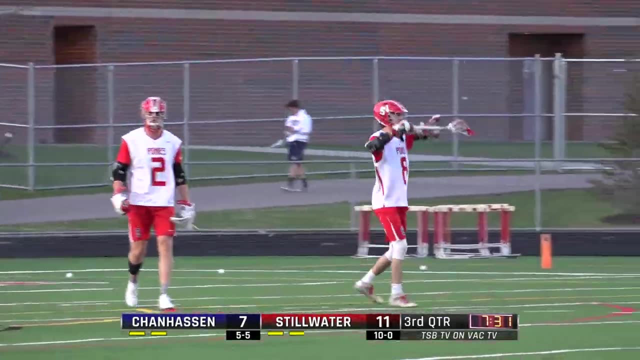 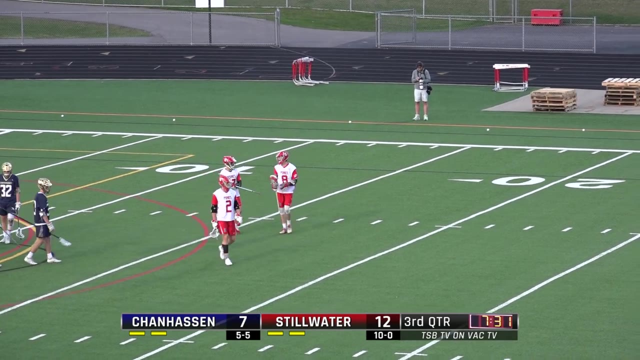 In transition. They've got an opening. They've got a goal. It's Cody Berger making a double order with extra cheese. A hasty misplay by Chanhassen at midfield caused a loose ball that just trickled right down the slot toward their own goalie. 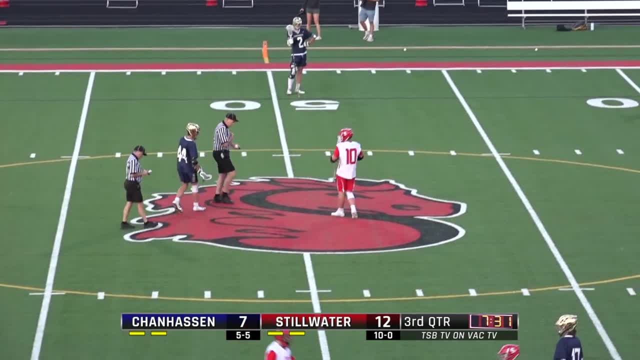 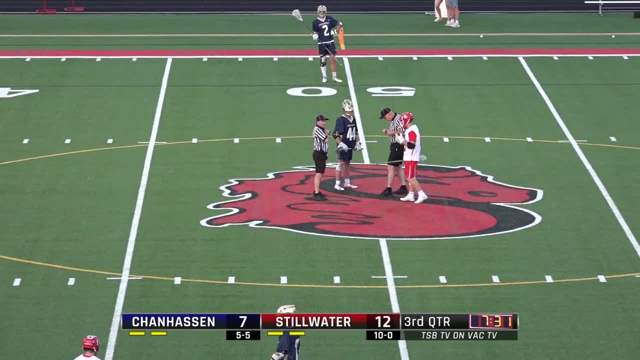 But picked up by Stillwater's Cody Berger for a great up, close bounce, shot off the turf past the goalie, Extra cheese, all the toppings and put some barbecue sauce on it, And Cody Berger- The third Stillwater player in this game- to get a hat trick. 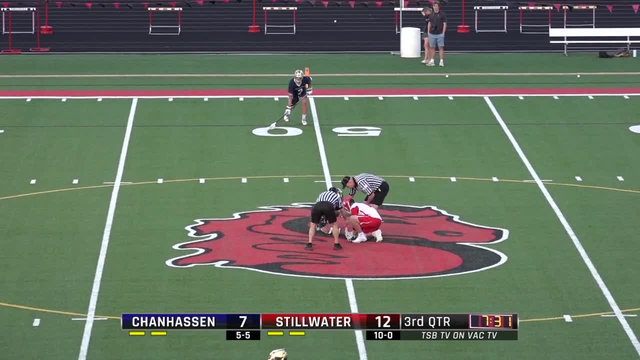 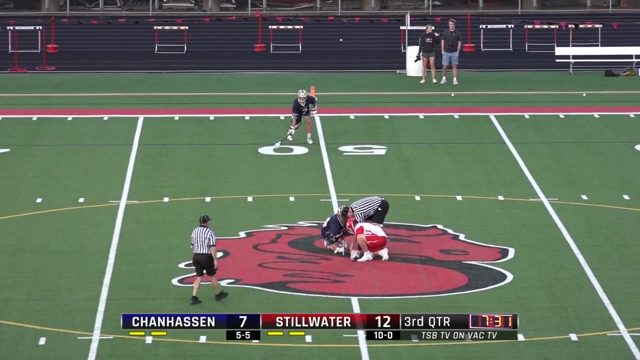 And on the season. I've got the official numbers right here. Berger picks up his second hat trick of the year, So this is looking like another Stillwater win. All the makings of it, All the ingredients, Multiple players with hat tricks. 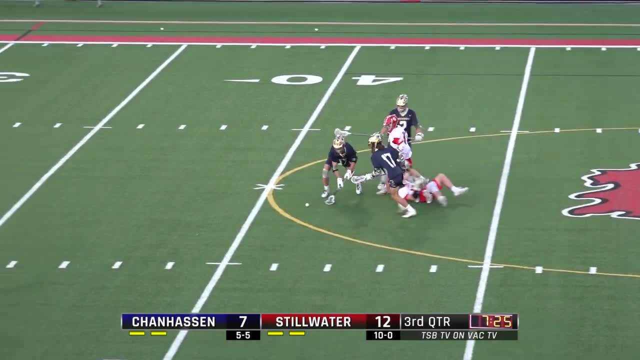 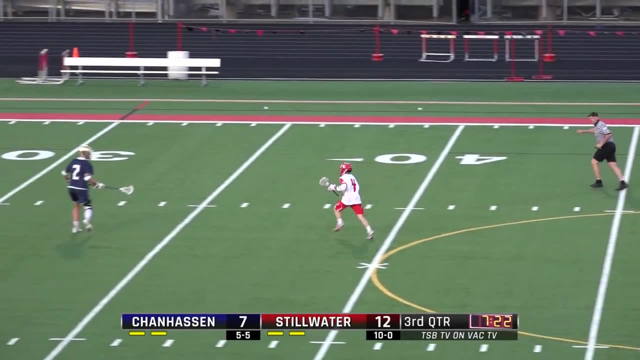 And no giant rally, But they've been increasing that lead And I'll tell you this: I wonder if that no call on Ben Karl Fired up this team. You saw Thurston launch a rocket And then they won the face off. 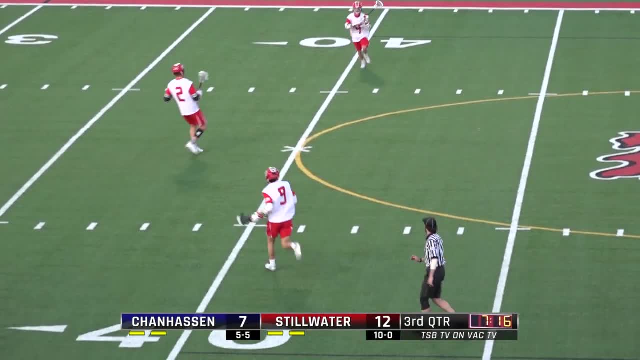 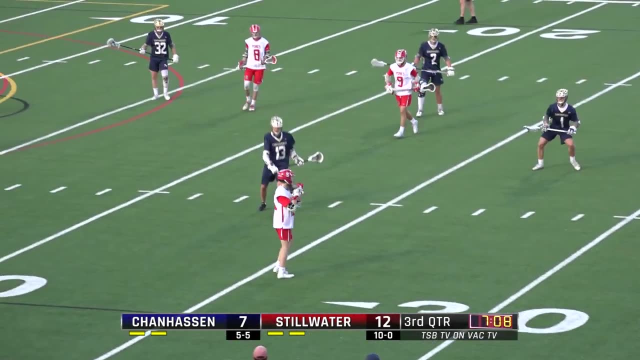 And Cody Berger scoring in transition. Yeah, yeah, That was fantastic. Ben Karl got just mowed, Just mowed into the turf And then comes up with the ball and just starts running again, Just like he never got knocked down. That's Ben Karl for you. 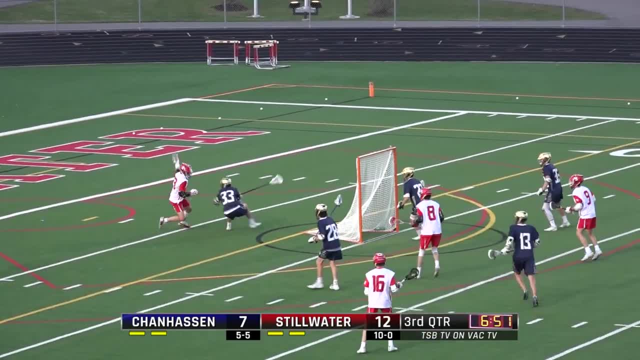 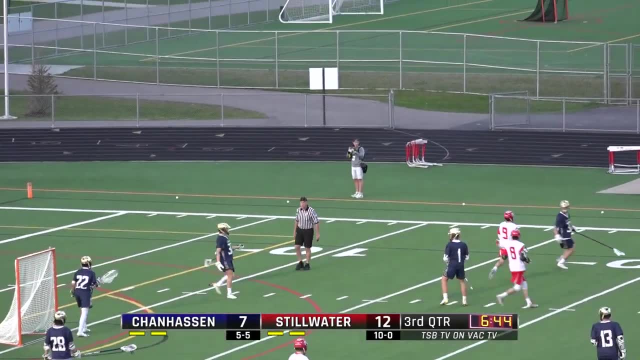 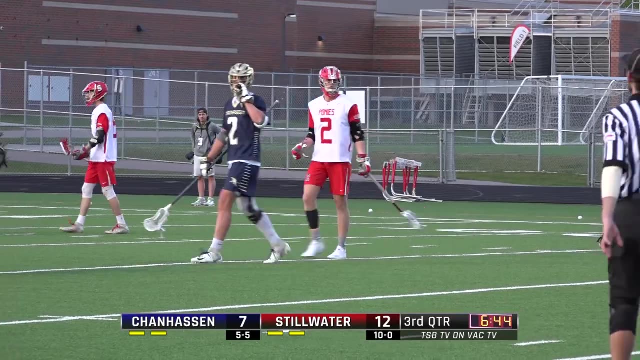 What a pass to. Quintin White: Caught in midair Gets his own rebound. He'll try to pass back out, But there were two Chanasson players there, But the storm might have been a little too physical on White, As they're going to get hit with the penalty. 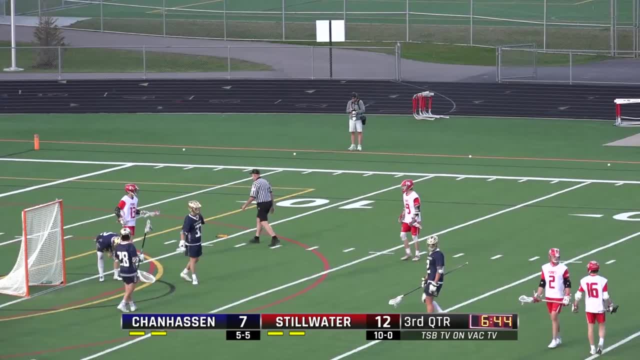 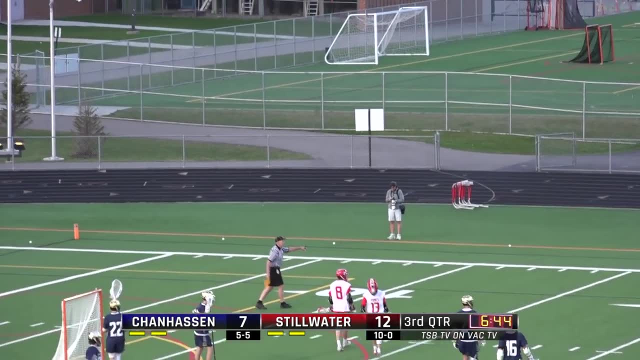 And I believe it will be assessed to Charlie Knauss. Knauss, number 32.. Yeah, a little hasty on Chanasson's part Getting physical there. They had just regained possession of the ball And they were just ready to move it upfield. 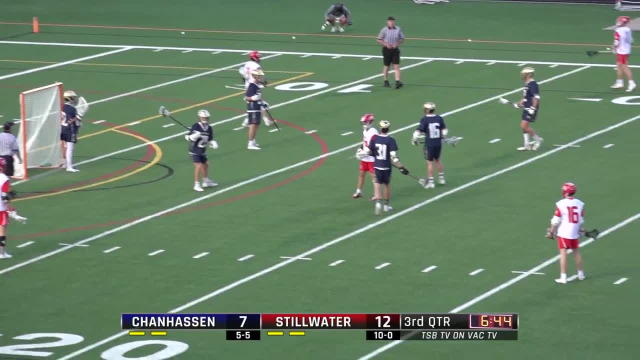 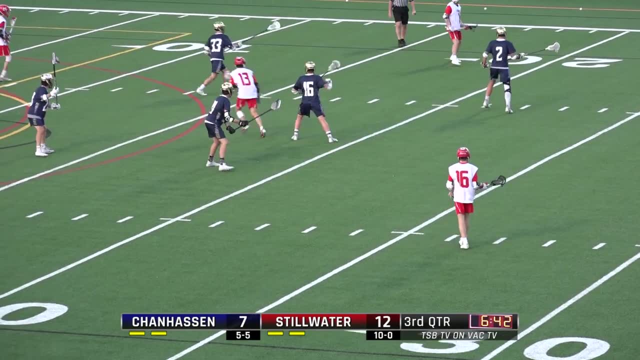 That's unfortunate Because, you're right, White had given the storm a free ball effectively, And instead Stillwater ball. Stillwater ball With the man advantage. We don't call it power play in lacrosse, even though it effectively is. 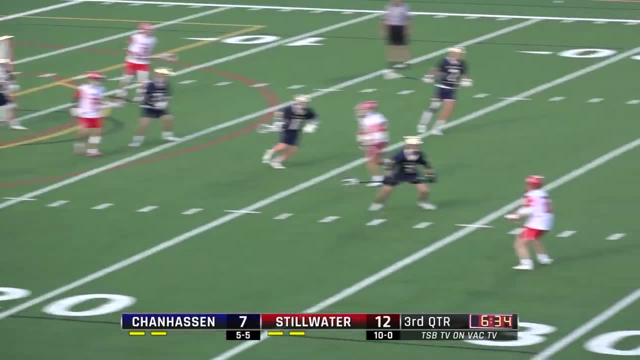 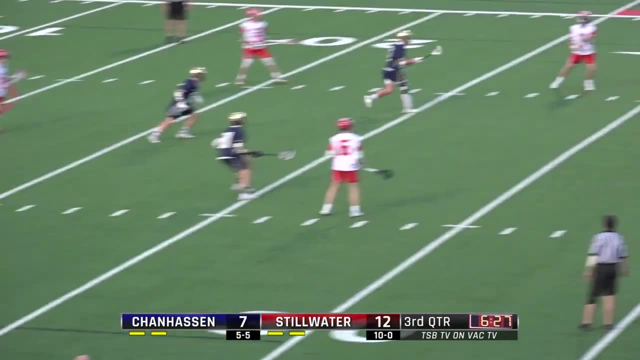 They do in box lacrosse, though Jeff and I could attest to that. We covered the Swarm for three years before moving to Georgia, Or I should say before they moved to Georgia. We're still here. There you go, We're here. 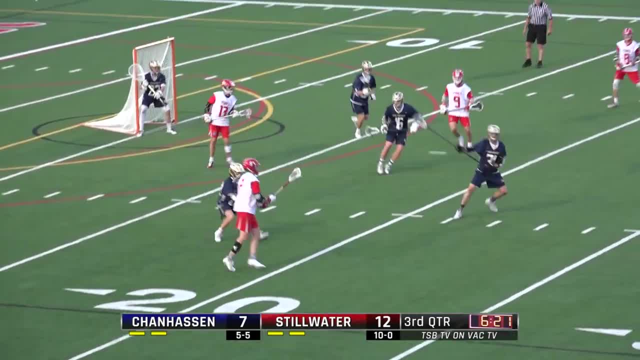 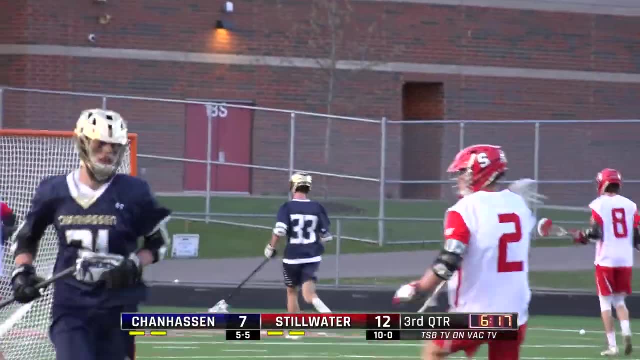 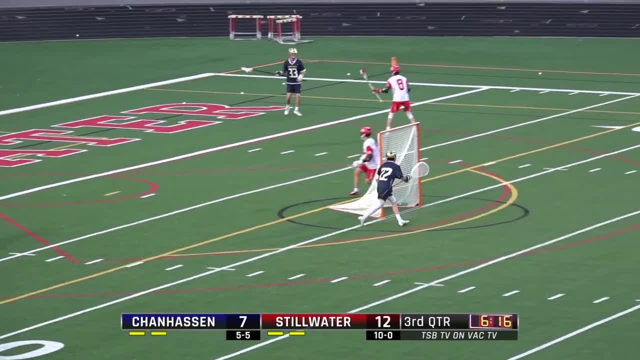 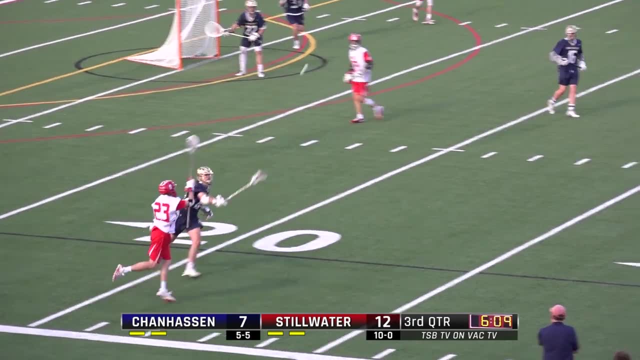 Except when it snows in Georgia, the entire state shuts down. When it snows up here, we can handle it. Business as usual, Unless it's an April blizzard, Pony's forcing the turnover: 24 on the clock. 24 on the clock. 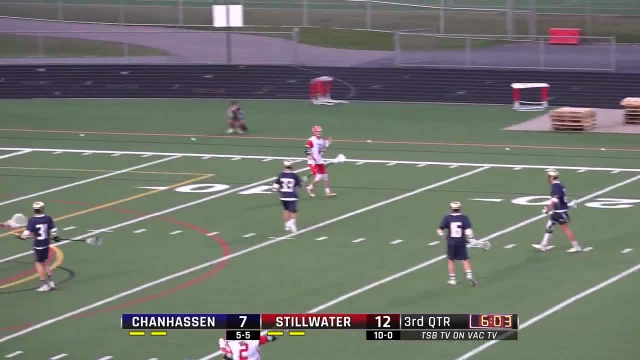 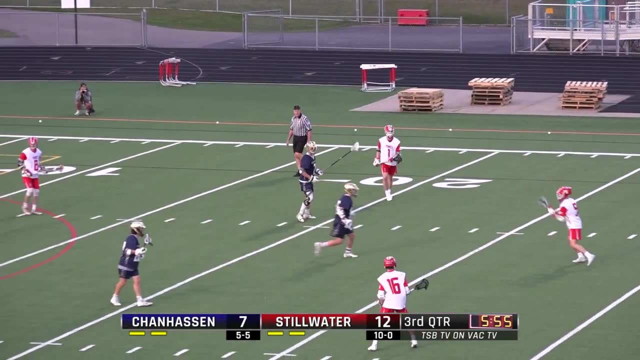 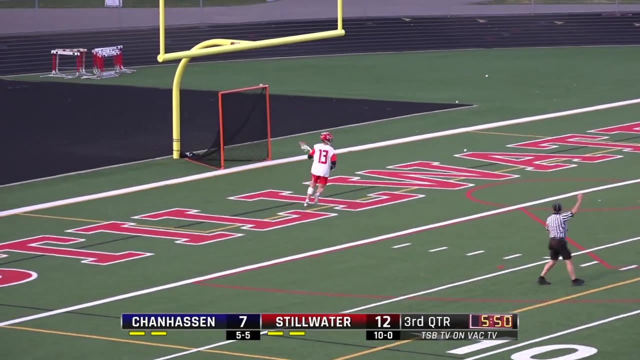 THURSON TO STINGLE OVER TO SUMMERY, A CYCLE PLAY IN PROGRESS OF THE PONIES. AND THAT SHOT- I THINK IT WENT OFF THE CROSS BAR. I HEARD A CLANK. IT WAS A SHOT OFF THE CROSS BAR. 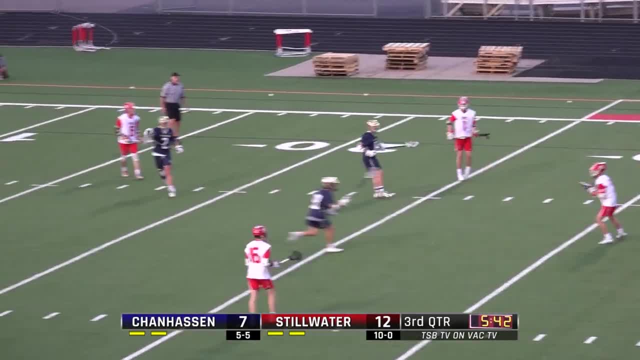 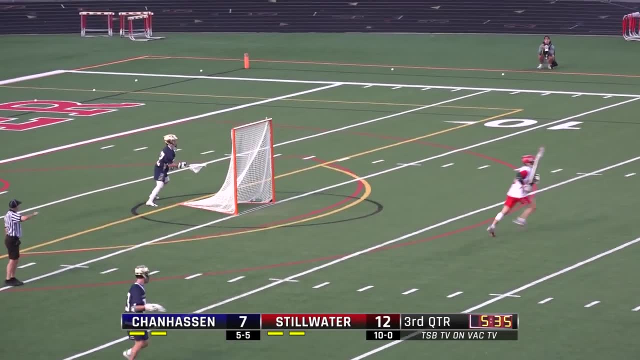 MY EYES DID NOT DECEIVE ME. STILLWATER PLAYERS ARE REALLY CRANKING UP SOME HARD SHOTS TONIGHT, TRYING TO OVERPOWER THE STORM, AND FOR THE MOST PART, THEY HAVE 12-7, IT COULD BE MORE. 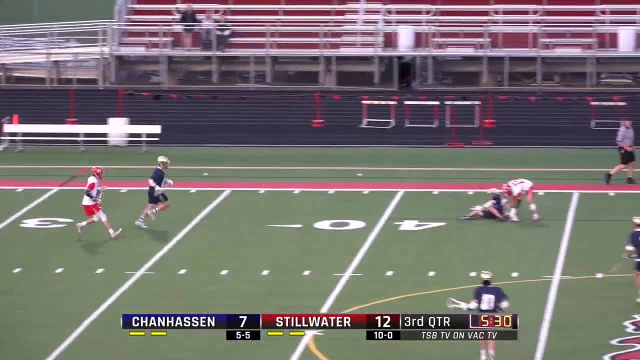 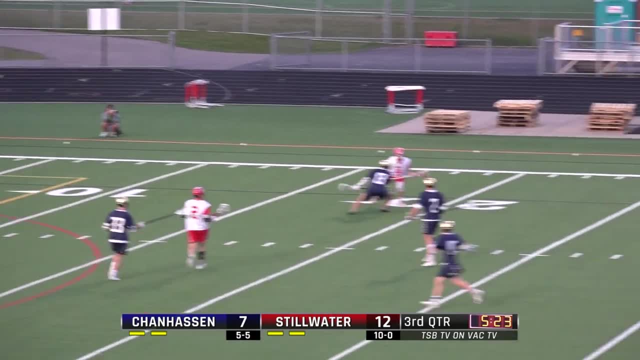 THEY'VE HAD A FEW SHOTS GO OFF THE CROSS BAR BUT, LIKE YOU SAID, TRYING TO USE THEIR STRENGTH TO THEIR ADVANTAGE AND A NICE BODY CHECK ON HIS PART, AND THIS IS THE FIRST TIME IN. 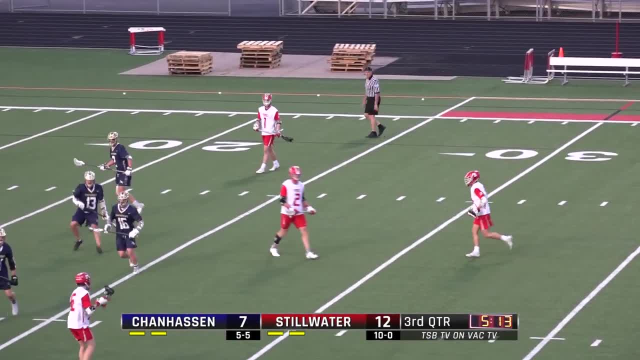 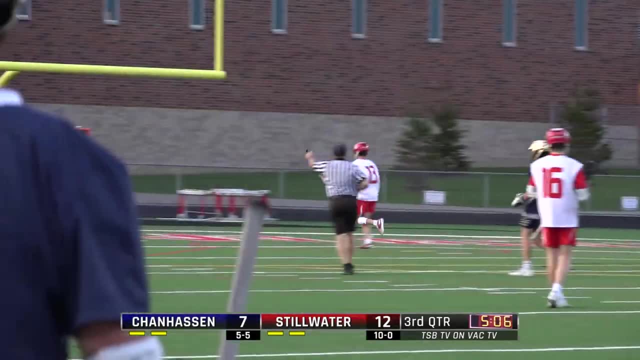 A WHILE WHERE. STILLWATER HAS HAD A SUSTAINED POSSESSION HERE ON OFFENSE THE LINES STILLWATER OUT THERE HAS RIGHT. NOW ARE ALL BIG SCORERS. WELL, WHEN THEY GET IN, THAT SET PLAY. THAT'S WHAT THEY DO. THEY BRING THOSE HEAVY HITTERS. 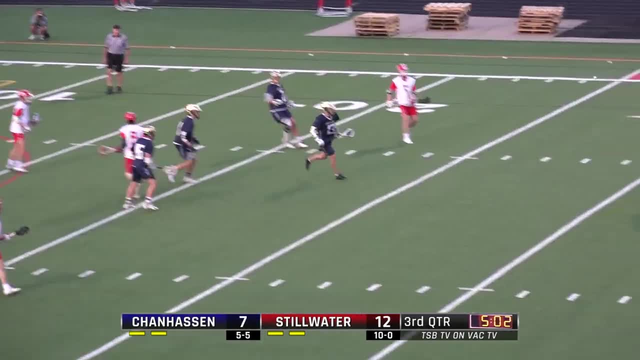 ALL SIX OF THEM CAPABLE. THEY'RE ALL DOUBLE DIGIT SCORES. YOU DON'T GET THAT A LOT ON MOST TEAMS, ESPECIALLY THE ONES. STILLWATER HAS FACED THIS SEASON AND EARLIER IN THE 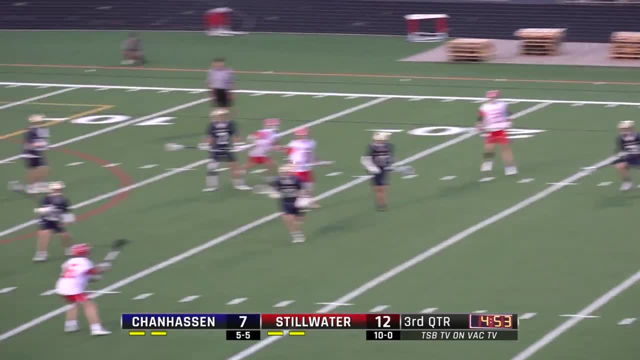 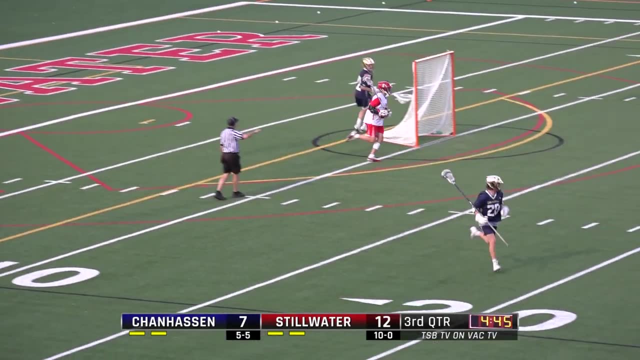 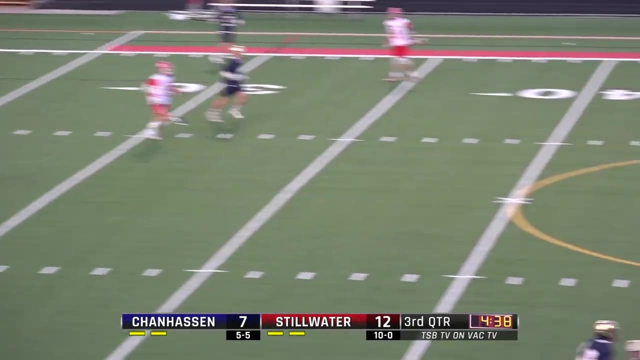 YEAR WHEN THEY HAD THOSE BIG TESTS WITH EAST RIDGE AND LAKEVILLE SOUTH AND ST THOMAS ACADEMY. AS THURSTON LAUNCHES ANOTHER ROCKET, THEY PASSED IN FLYING COLORS. IT'S ONE THING TO BE UNDEFEATED. IT'S ANOTHER TO BE PUTTING UP BIG WINS AGAINST TOP RANKED. 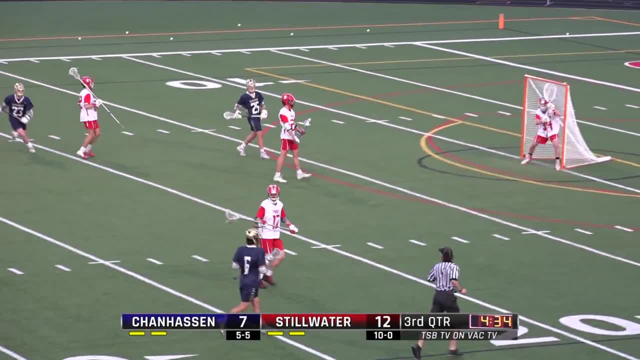 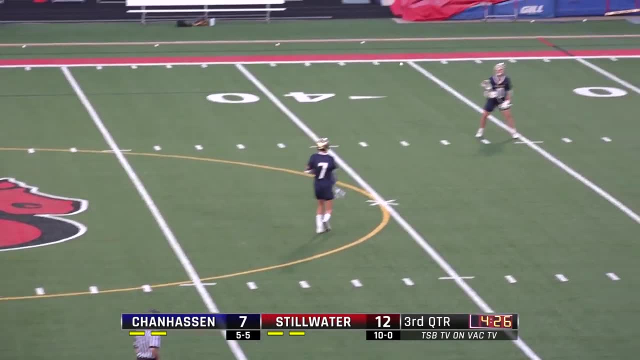 TEAMS AND BECAUSE THERE ARE SO FEW GAMES. YOU KNOW THE PONIES. THEY DON'T GET A CHANCE NECESSARILY. THEY WILL PLAY YZETTA, BUT SOME OF THOSE OTHER LATE CONFERENCE TEAMS- THEY WON'T GET A CHANCE. 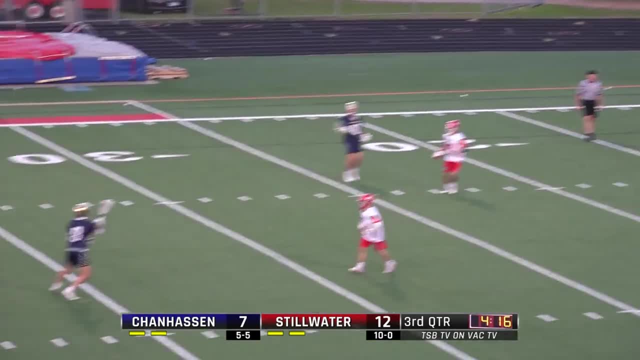 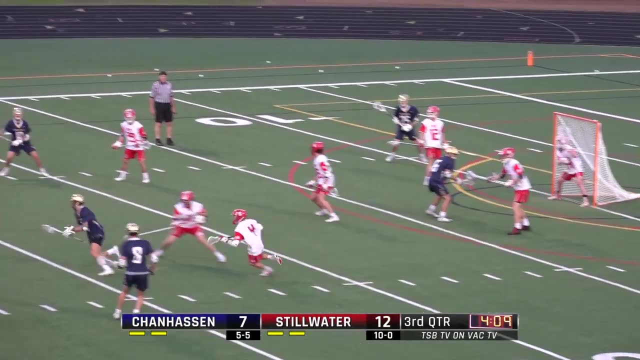 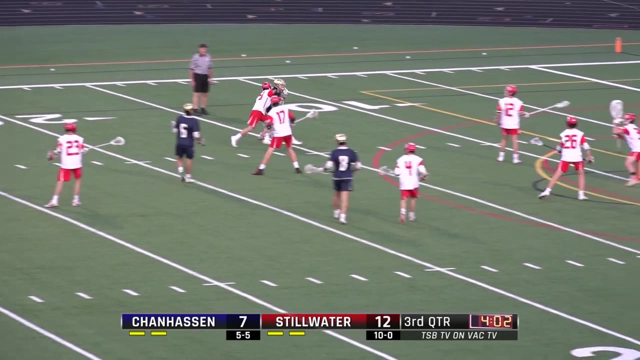 TO SEE IT, UNLESS THEY MAKE THE STATE TOURNAMENT BUT A LOT OF MOMENTUM IT'S GOING TO BE A PENALTY. I BELIEVE ON BEN CARL, WHICH HE MAY NOT LIKE. AS YOU SAY, CARL GOT MOWED TO THE TURF ON A PLAY THAT FELT A LOT MORE PHYSICAL. 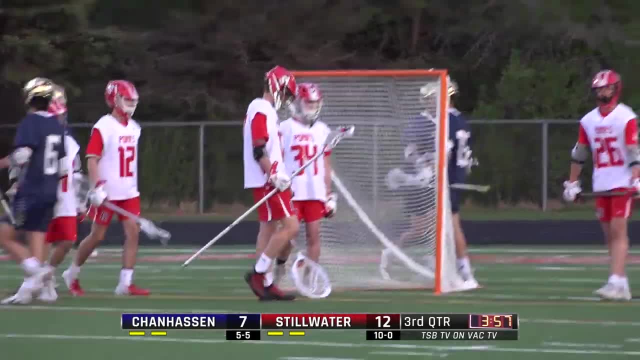 IT WILL WIPE AWAY THE PENALTY. THAT'S GOING TO BE A SCORE FOR JASON COLLINS, OFF THE FEED FROM VINCENT MANUEL MANUEL WITH HIS SECOND ASSIST OF THE GAME, AND THE STORMS STILL HANGING AROUND. 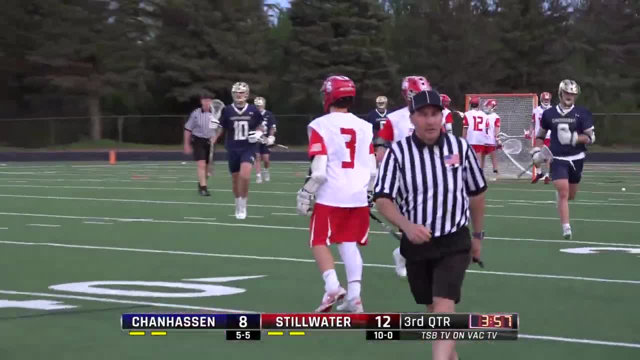 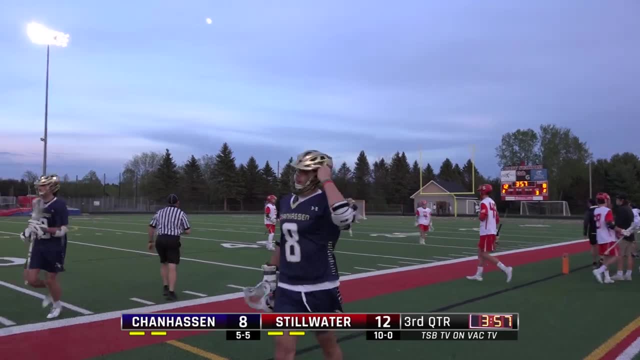 BUT, ROBERT, THEY'RE GOING TO NEED A RALLY OF THEIR OWN IF THEY REALLY WANT TO CHALLENGE THE PONIES RIGHT NOW. IT'S REALLY TOO CLOSE FOR STILLWATER TO GET COMFORTABLE BY ANY SENSE OF THE WORD. 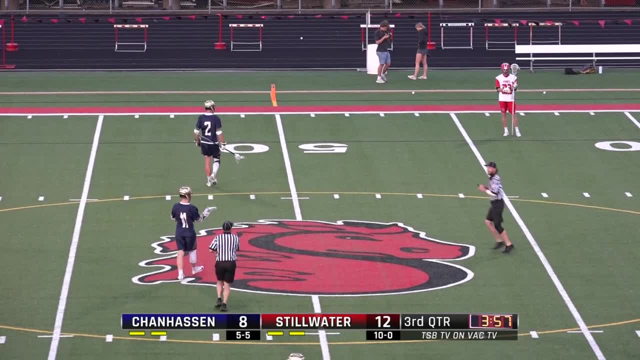 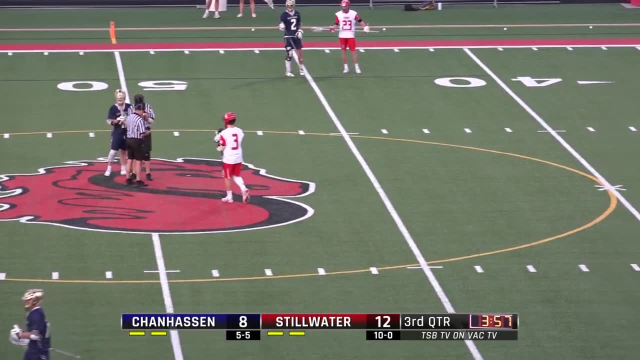 THEY NEED TO KEEP THIS GOAL DIFFERENTIAL RIGHT WHERE IT'S AT. I AGREE WITH YOU: NOT BIG ENOUGH FOR THE PONIES TO GET COMFORTABLE, BUT AT THE SAME TIME, THE STORM HAVE NEVER SCORED. 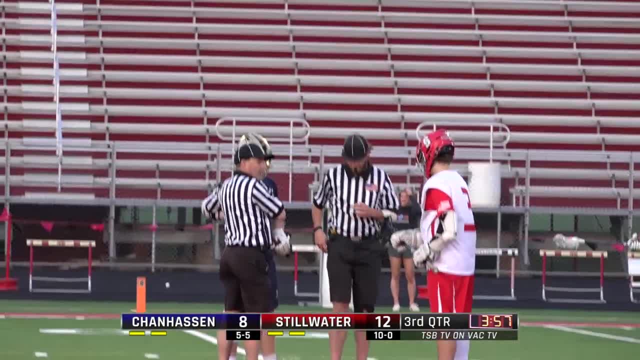 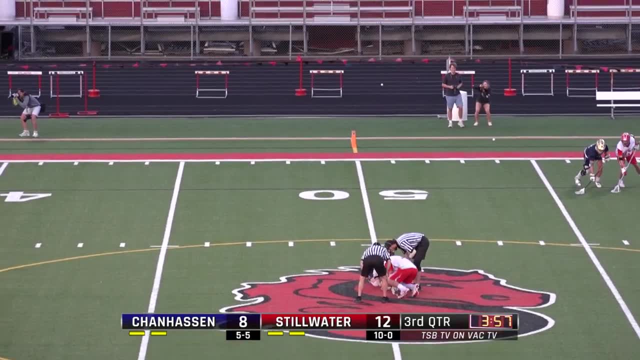 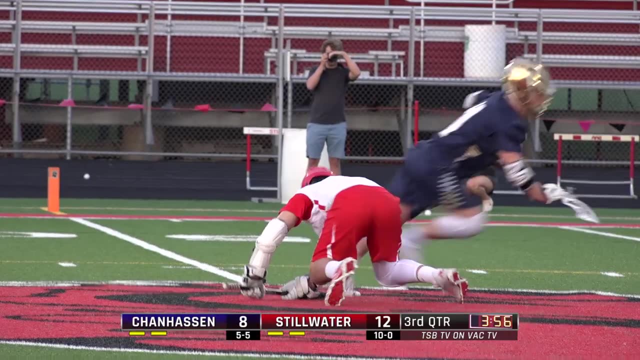 THEY'VE SCORED CONSECUTIVE GOALS AND THE PENALTY WILL STILL BE ASSESSED TO BEN CARL. I'M STILL LEARNING LACROSSE FOLKS. IT'S BEEN A WHILE SO ONE-MINUTE MAN ADVANTAGE FOR THE STORM. 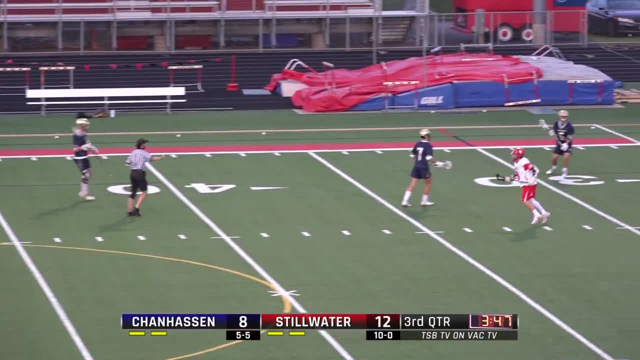 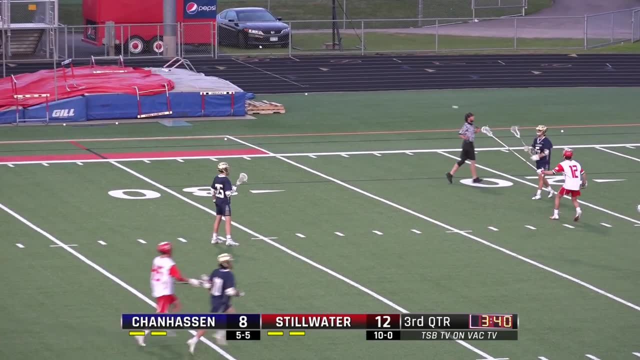 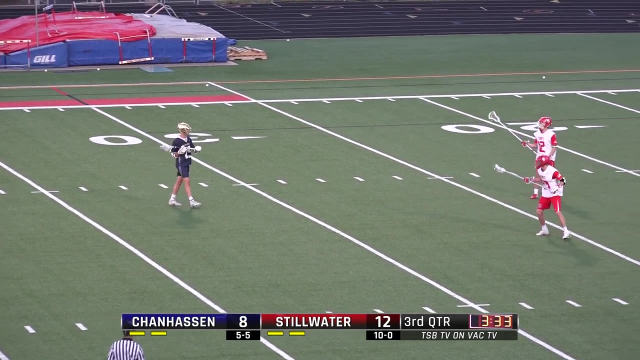 AND THEY DO WIN THE FACE-OFF. A LITTLE SLOPPY OF A WIN, BUT HERE'S THE CHANCE FOR THE STORM. TRYING TO GET THAT RALLY FOR THE FIRST TIME, AND WHAT A PERFORMANCE BY ALEX DEWEY. 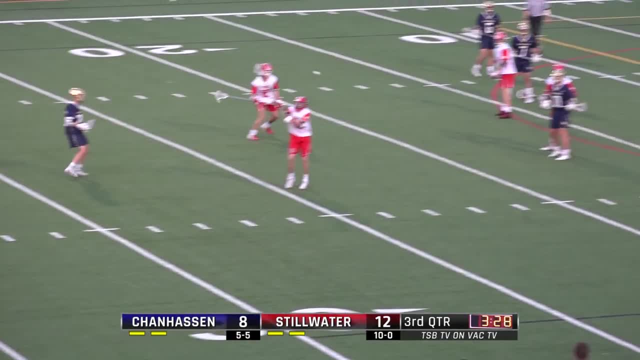 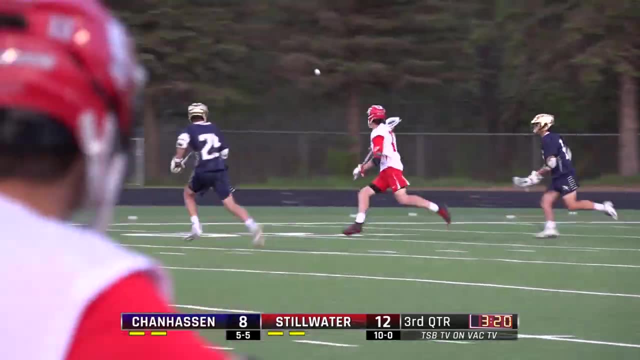 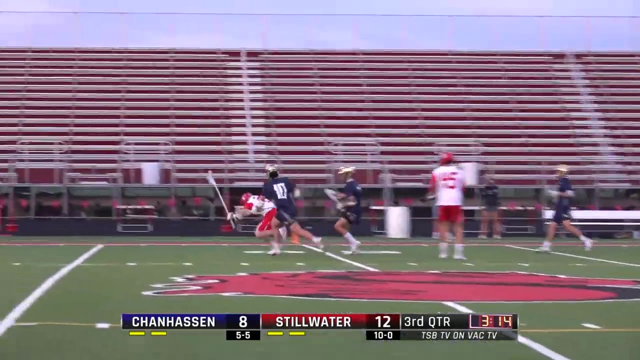 WE HAVEN'T HEARD MUCH FROM HIM. YET NICE PLAY BY NUMBER 17,. JUSTIN SIGFRIED A KEY DEFLECTION. BEN LONG HIT FROM BEHIND AND THAT'S GOING TO BE A FLAG. 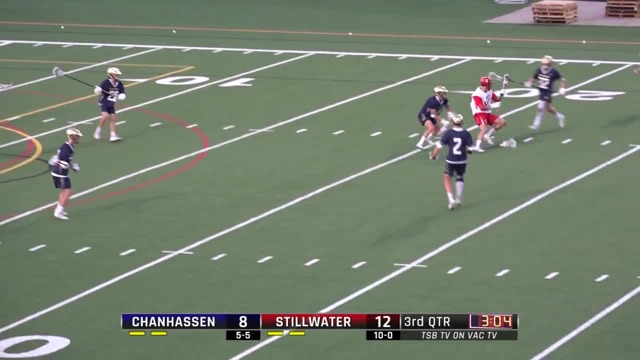 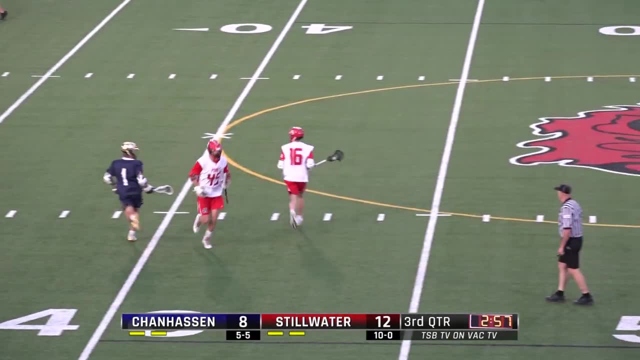 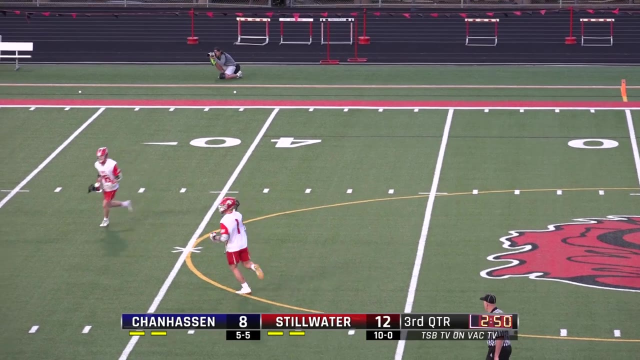 I SEE TWO FLAGS. BOTH OFFICIALS SAW IT, SO THAT'S GOING TO WIPE AWAY THE MAN ADVANTAGE FOR THE STORM, AND THEY DIDN'T DO MUCH WITH IT, BUT GIVE CREDIT TO JUSTIN SIGFRIED MAKING THAT KEY DEFLECTION. 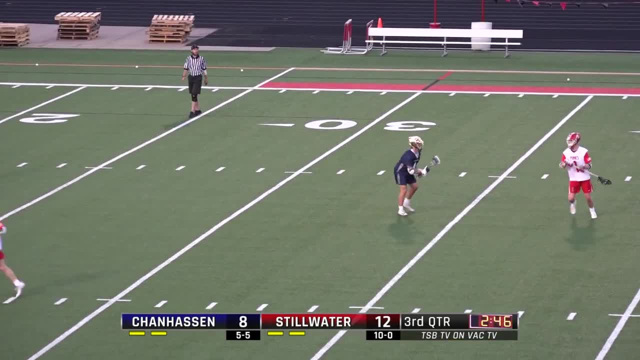 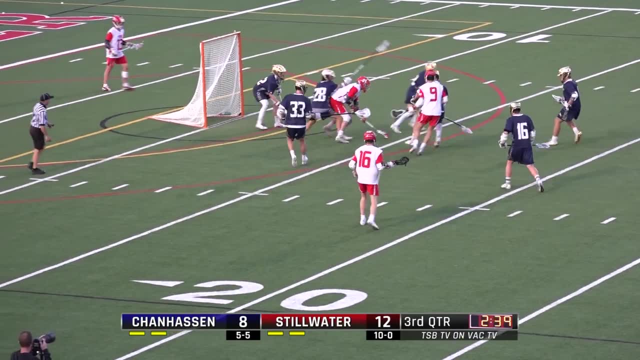 YOU CAN TIME THE PASS LIKE THEY DID CENTERING PASS FROM EVANSEN OVER TO STINGLE IT'S SAVED FIGHT FOR THE REBOUND. WILL GO TO CHAN HASSEN OR NO, IT WON'T. IT'S STILL LOOSE. 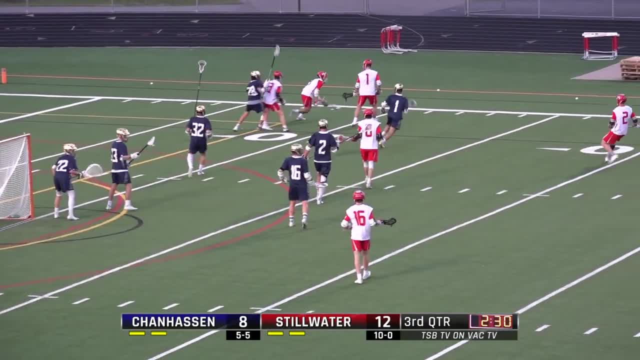 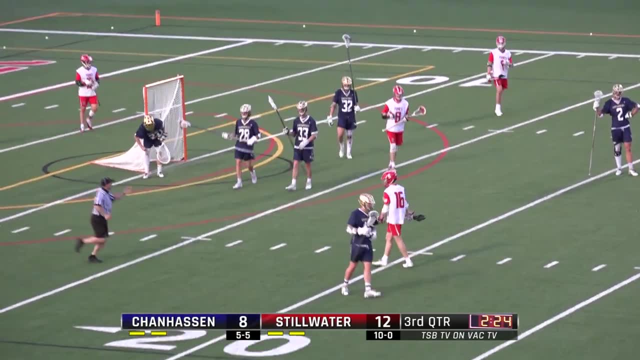 AND I THINK STILLWATER GOT IT. YES, THEY DID. THAT WAS QUINTON WHITE. HE'S TRYING TO GET AWAY FROM TROUBLE AND HE DOES SO NICE HUSTLE BY THE PONIES. WELL, THAT'S UNFORTUNATE. 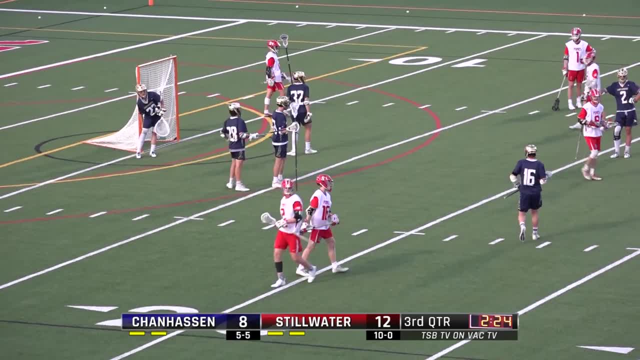 BUT STILLWATER WILL HANG ON TO IT, BECAUSE WE DO HAVE THE PENALTY ON CHAN HASSEN. IF YOU WANT TO HAVE A SLOPPY PASS, LIKE THAT, THAT'S THE TIME TO DO IT. THE TIME TO DO IT. 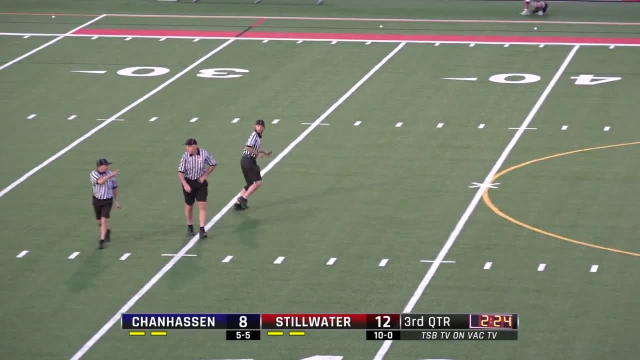 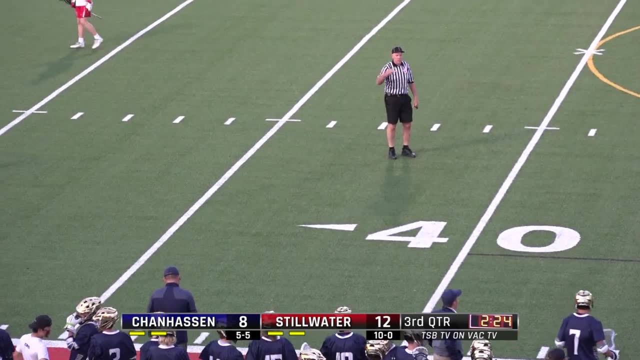 AND A RARE MISS ON A CATCH BY NELSON. SO I THINK HE WAS LOOKING TO WHERE HE WAS GOING TO GO WITH THE BALL NEXT INSTEAD OF FOLLOWING IT INTO HIS STICK. YOU GOT TO HAVE THAT DOUBLE PERCEPTION. 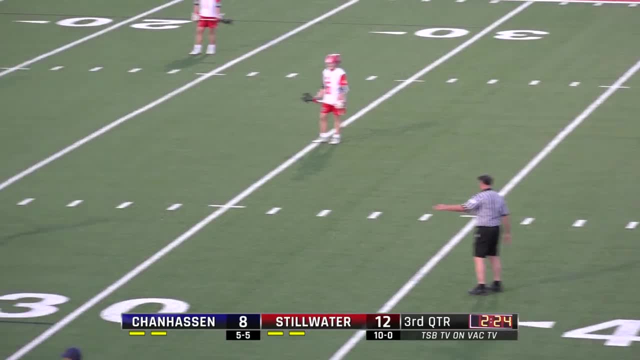 YOU GOT TO BE ABLE TO WATCH THE BALL SO IT MAKES IT IN YOUR STICK, BUT YOU ALSO GOT TO KIND OF KEEP AN EYE ON WHERE YOU'RE GOING TO GO WITH IT TOO, IF YOU'RE GOING TO MAKE A FAST PASS. 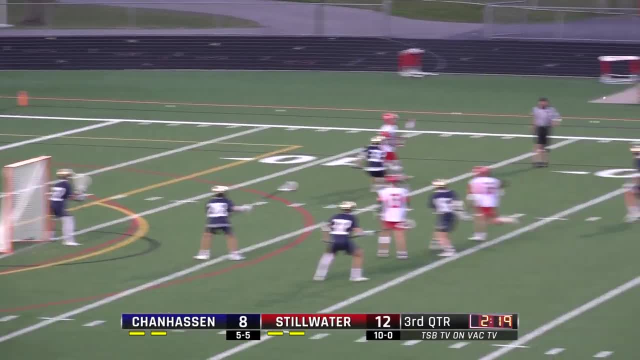 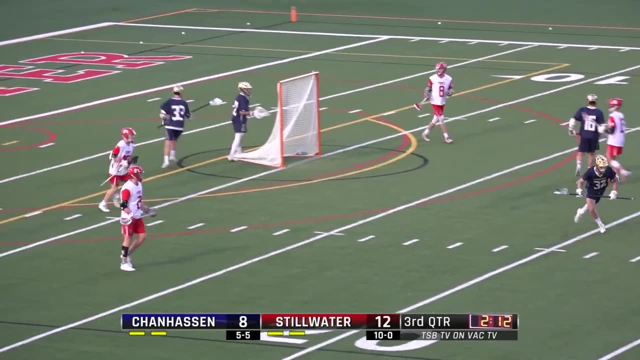 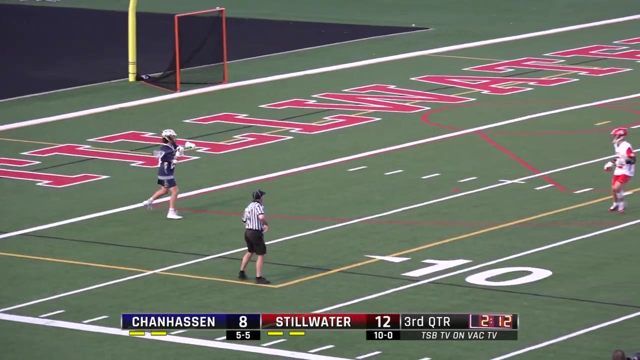 AND THAT'S THE NUMBER SET. ALEX DEWY BELIEVES HE'S GONNA PUSH 30 SEC PUSH PENALTY ON ALEX DEWY AND ANOTHER ERRANT PASS BY THE PONIES. SO NEITHER SIDE ABLE TO CASH IN A WHOLE LOT ON WHAT, EFFECTIVELY, IS A POWER PLAY SITUATION. 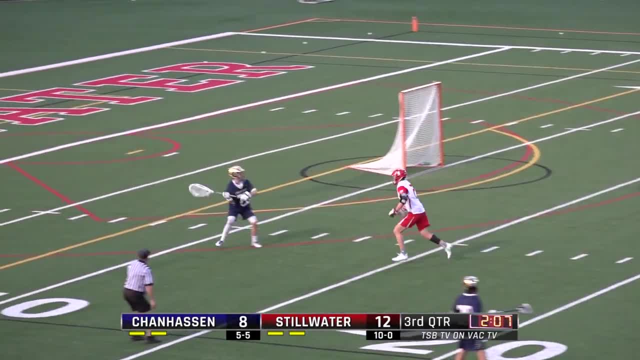 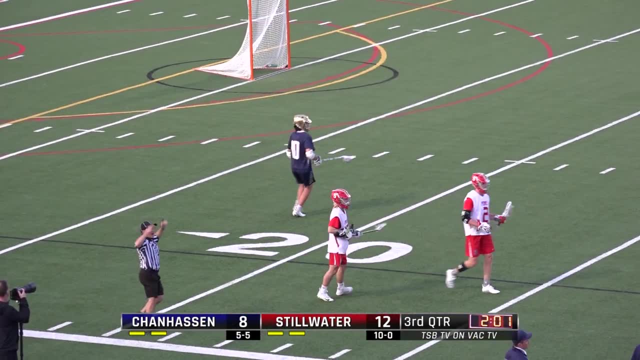 WE'RE JUST HOPING THAT THESE SLOPPY TURNOVERS BY STILLWATER OF RECENT HERE DON'T COME BACK TO BIKE HIM. THEY STILL LEAD BY FOUR. BUT THAT'S NOT WHAT YOU WANT if you want to preserve your chance at a win. 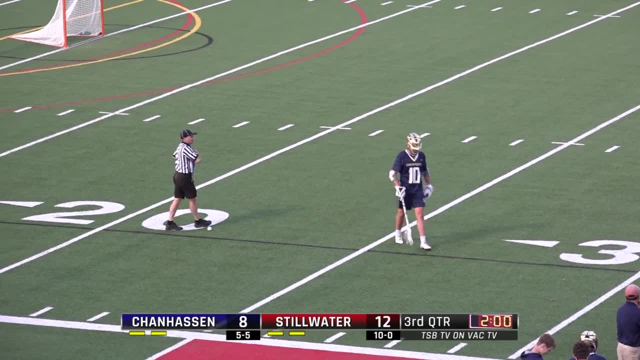 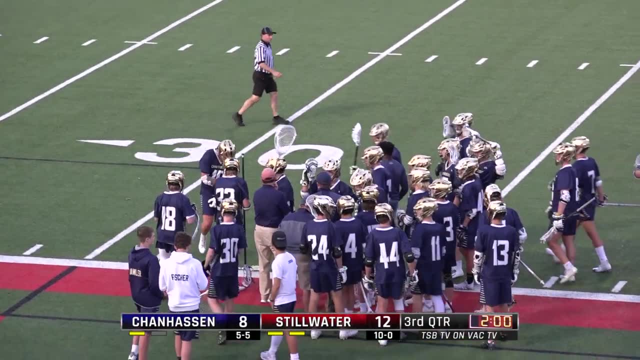 or keep Chanhassen from rallying. We have a timeout called by the Ponies. No, Chanhassen, I should say With two minutes left in the third quarter: 12-8,. this has been the closest game that Stillwater has had in a long time. 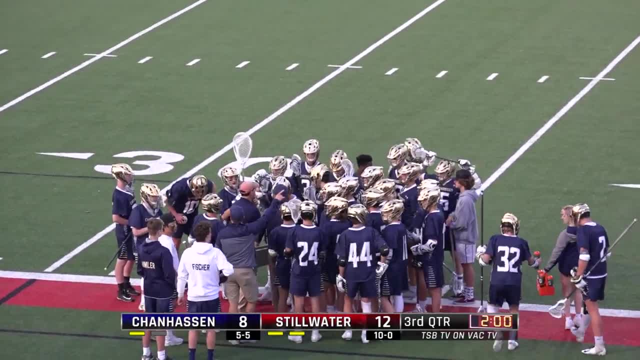 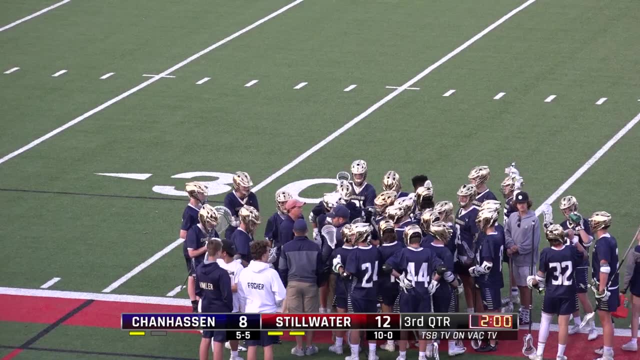 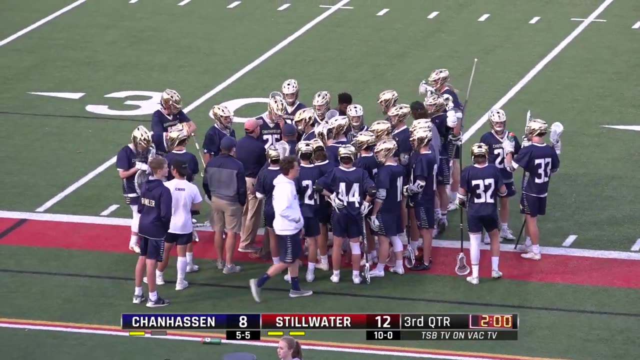 Looking at their recent performances, as Robert is rocking along to some John Mellencamp- Well, he does that Stillwater. they've had a bevy of ten goal performances and Robert's still rocking along here. I wish we had a camera on him. 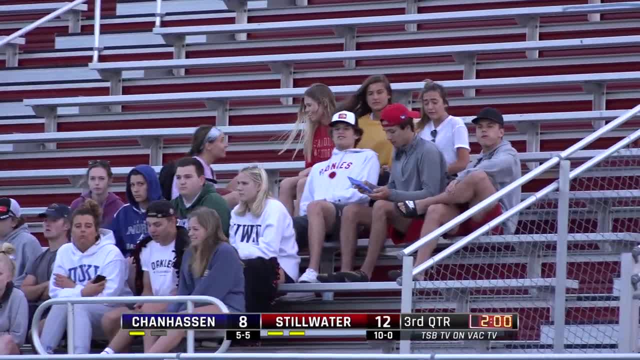 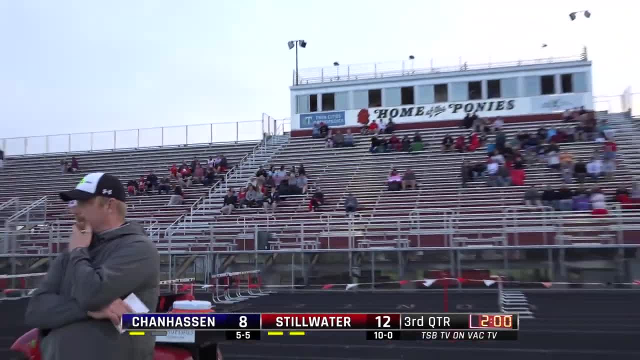 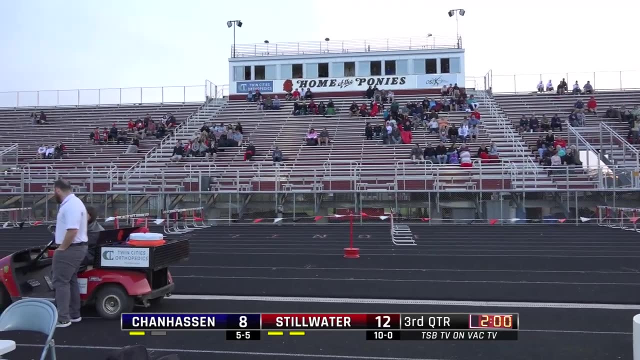 Somebody make him a viral sensation. Okay, where am I? Stillwater? Yes, so for the Ponies, as we said, a lot of big wins. They came off a huge one against Roseville, 17-3.. And they've had a lot of big wins, a bunch by ten or more. 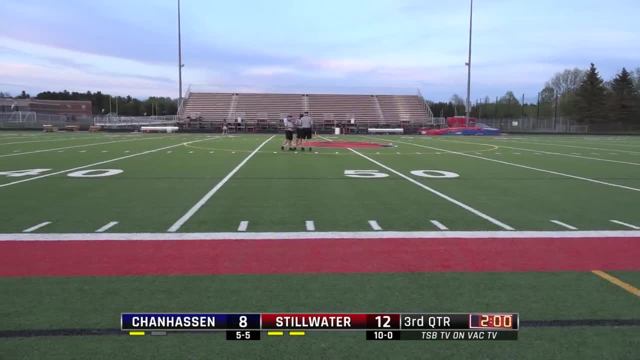 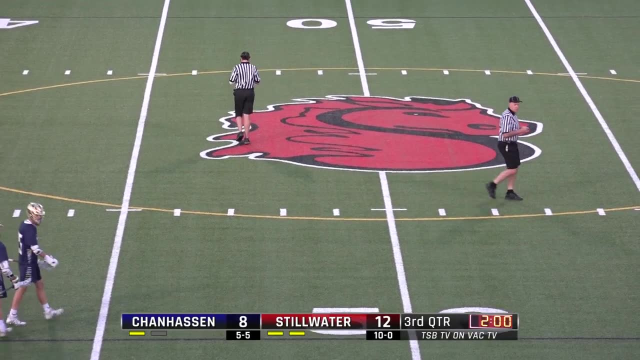 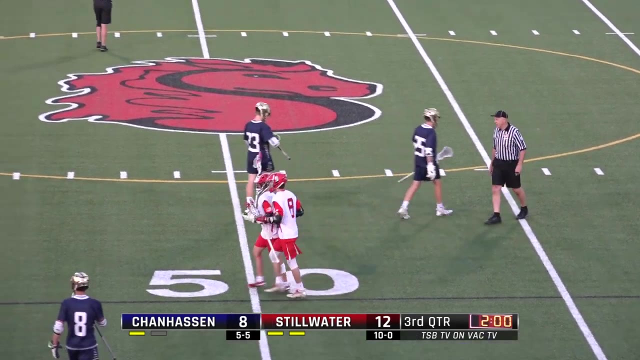 If you look at their season 14-3, I should say against Roseville And one, two, three, four, five wins this season by ten or more. Five by ten or more, their closest margin of victory all season, Robert, seven goals. 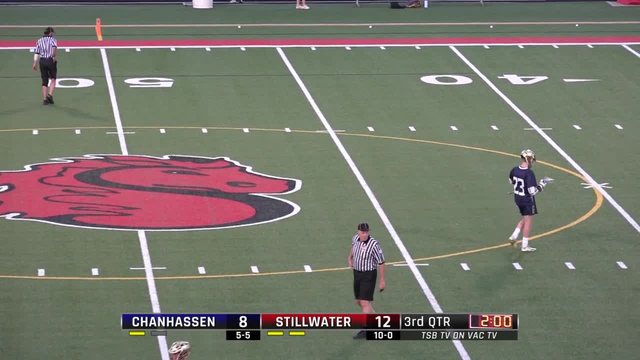 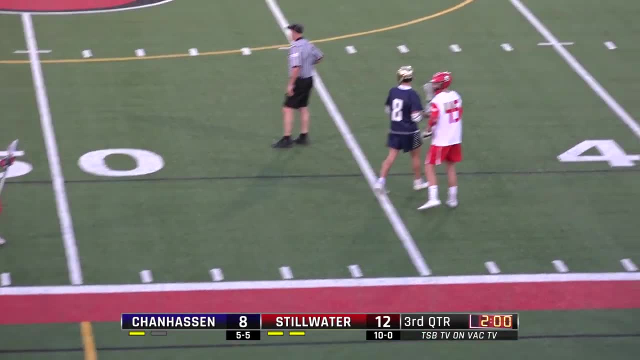 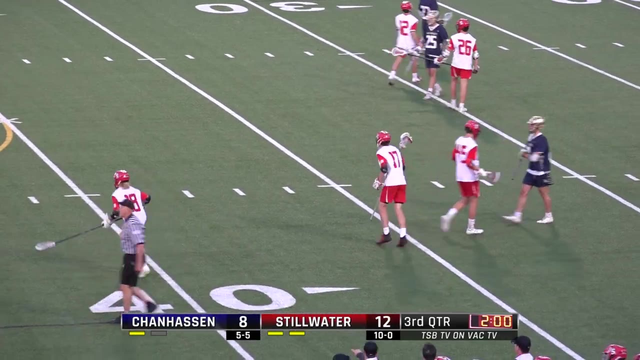 I know we're talking about a first world problem here, But every game you win by seven or more. that is insane. Yeah, that's a good margin. We are not there yet. The Ponies have had a hard time getting there. 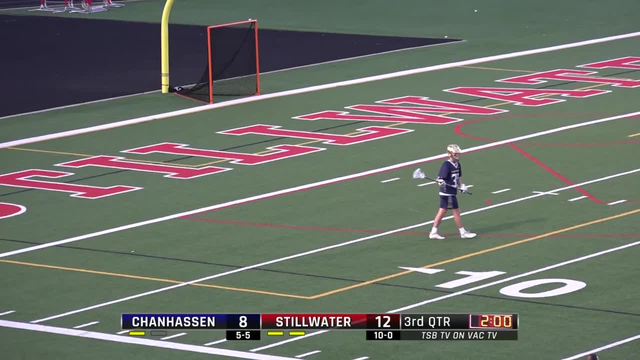 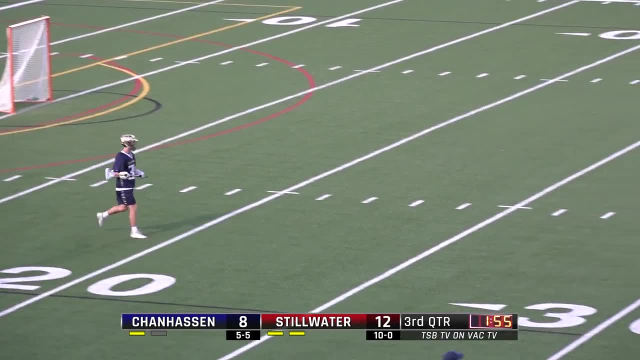 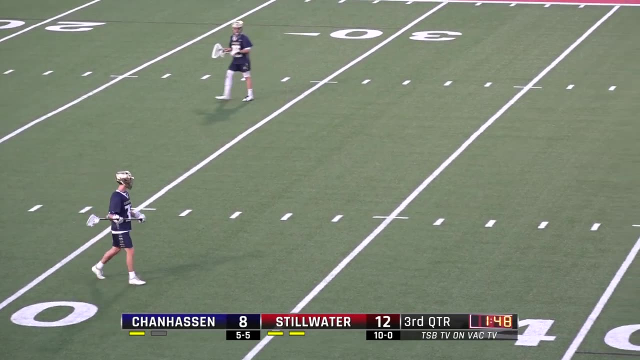 Shane Nasson. just not Stillwater's solving now, but not completely. Like I said, right now we're talking about a first world problem here. It was like Those Lynx dynasty years, especially in 2015,, 16,, 17,, oh, 13, too, where they would win. 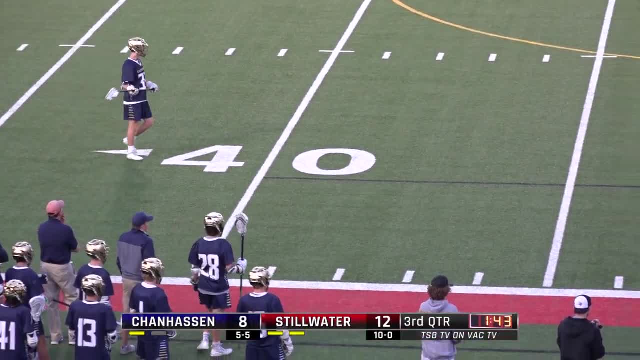 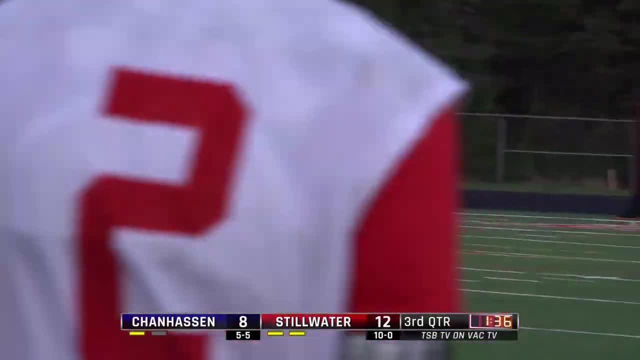 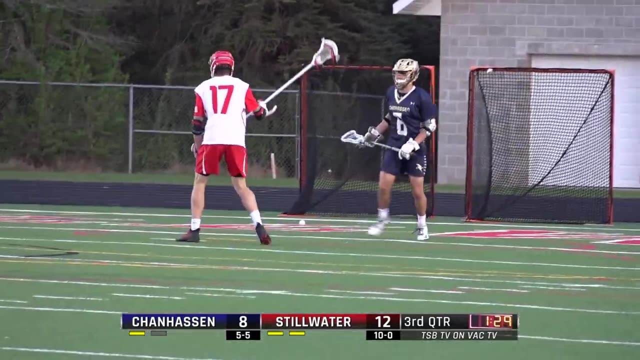 If they didn't win by 20 or more, everyone was wondering what's going on with them. It's an embarrassment of riches. But as the saying goes, a win is a win is a win. So if the Ponies, if they win by five or four, that won't bother them a bit. 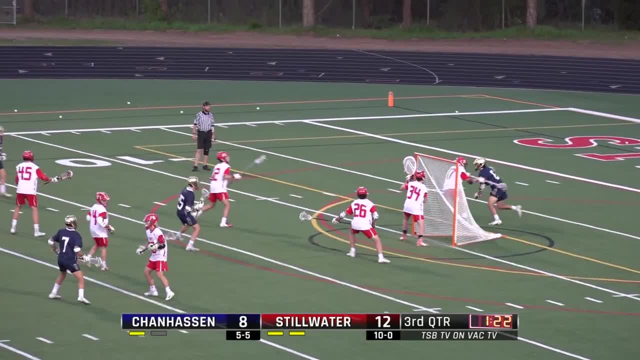 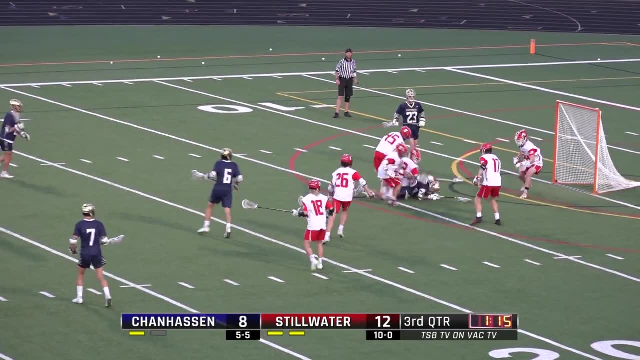 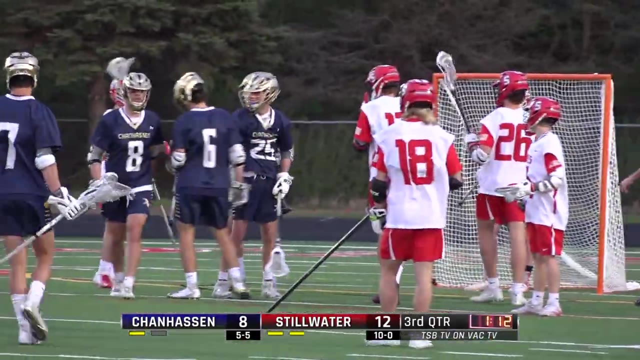 Got a stick, A stick shooting lesson from Neil Dottaridge of the swarm when they were here. Holcomb double team And that's going to be a penalty. Stillwater pushing Tyre Christensen from behind And it looks like it's going to be the 30-second variety. 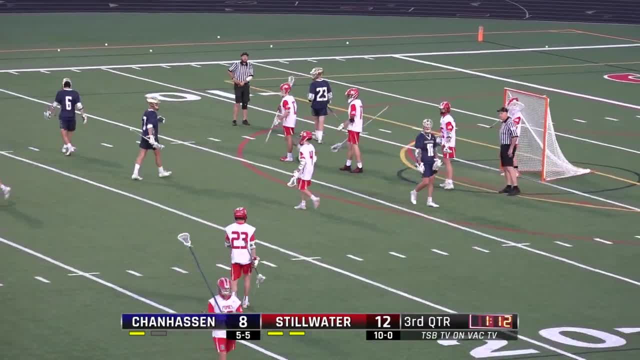 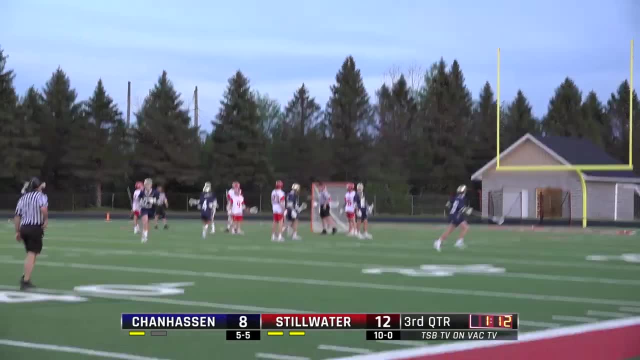 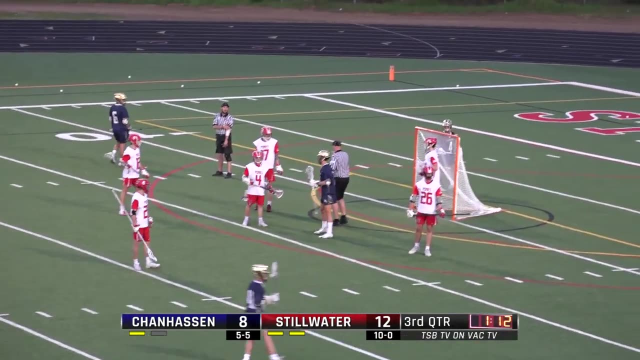 Three, four, five, four, three, two, one, Two, three, two, one Harder. Make sure you tell them, Hunter, There's Splitter, Splitter, Splitter. Big opportunity here for the storm. 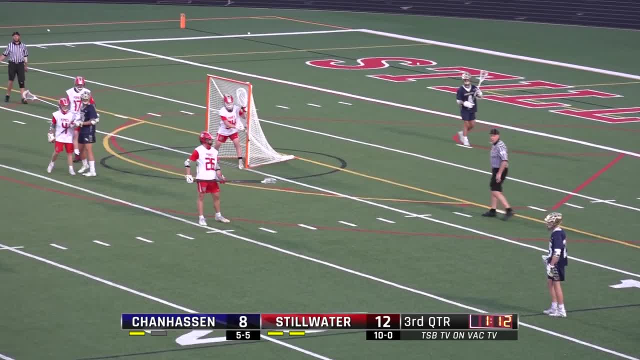 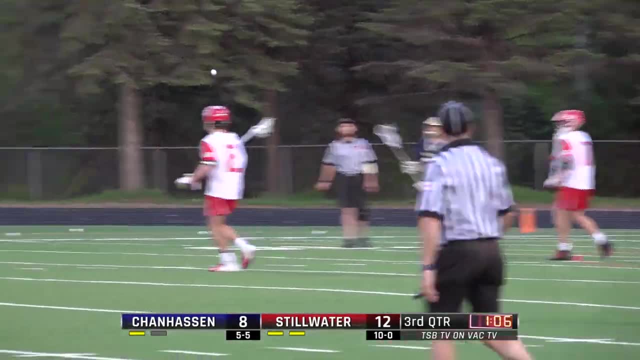 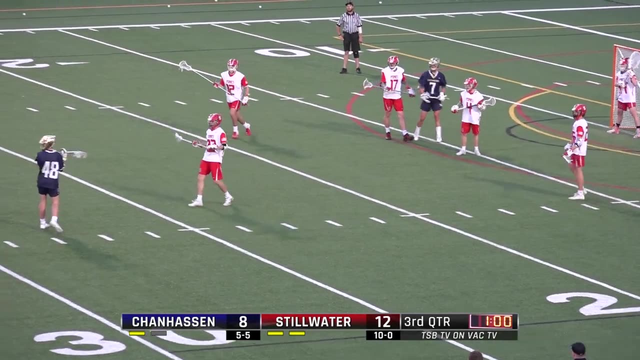 Penalty goes against Jamison Stahl. They'll have the man advantage for 30 seconds And even though they're down by four, so it's not like they can tie it up. this is big. You get a goal here And once again they've had two man advantage situations in this quarter. 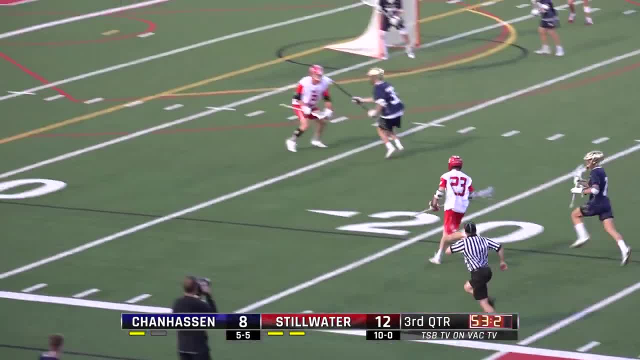 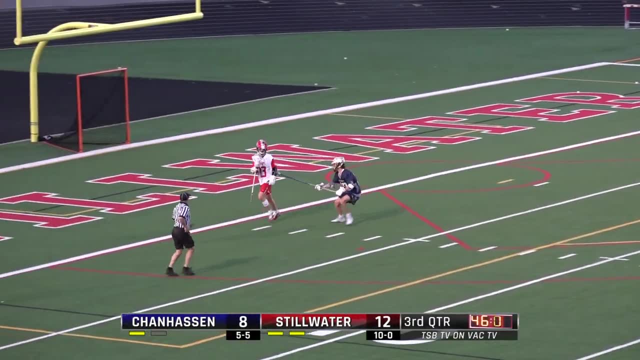 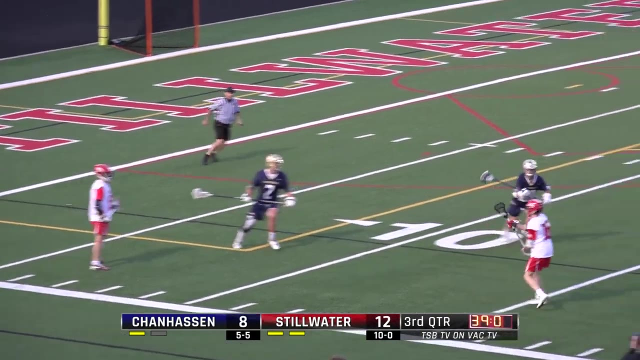 And a couple of poorly executed possessions to show for it. Conversely, if you're the Ponies, can you get a shorthanded goal or even just get one more to throw down. the dagger Release Saw some quick movement by Benjamin Long, the long stick midfielder. 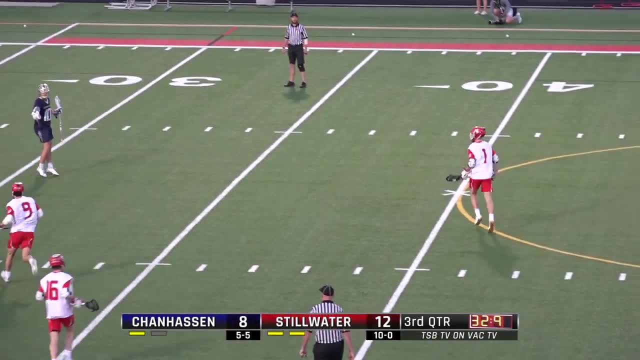 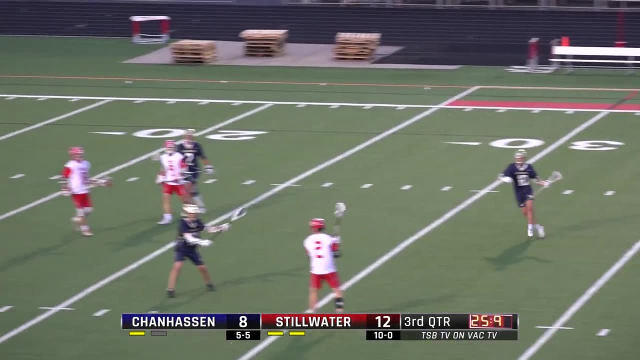 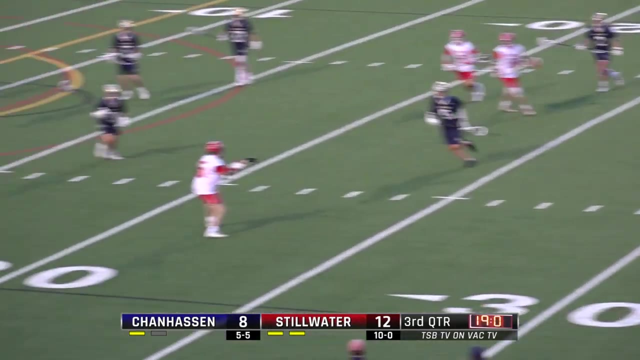 Stillwater just moving fast And the Ponies look content to run out the clock. They can't see it on this end, But they have 22 seconds and counting. We haven't reached the era yet of dual-sided scoreboards in high school sports. 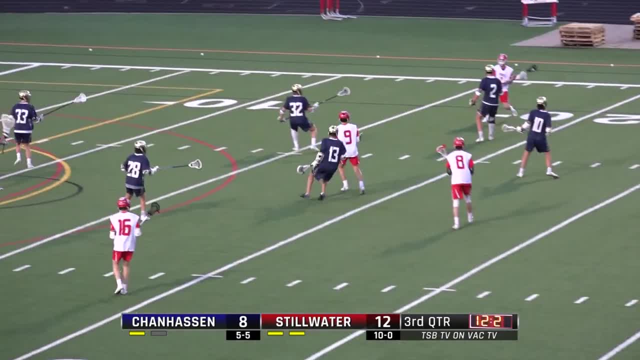 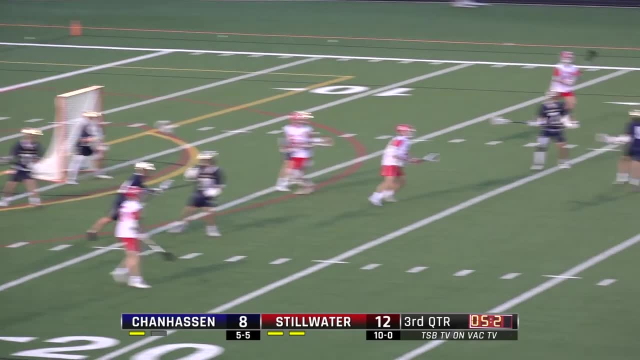 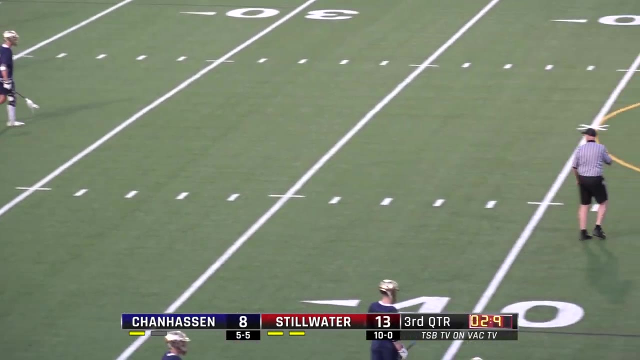 at least on the outdoor facilities. Deep pass to Summary: Seven seconds. They run the clock down as far as they can. Now they've got a launch and Evanson does just that, Blake Evanson, with his second goal of the game. 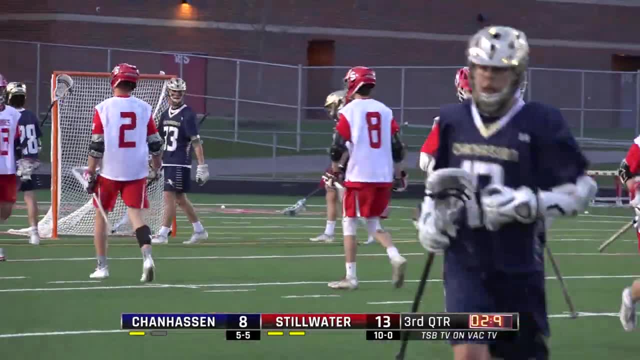 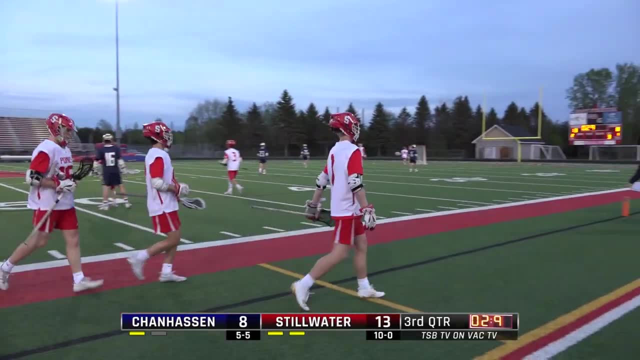 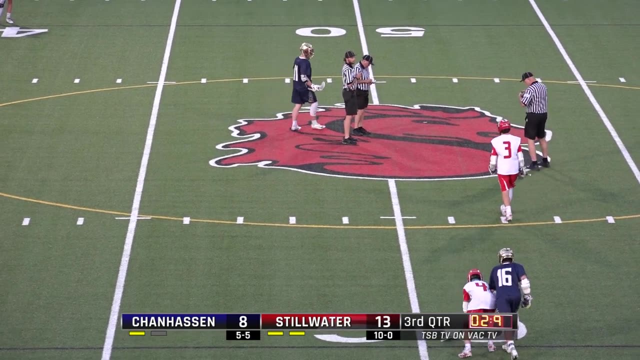 27th on the year and that could be the dagger play by the Ponies as they go back up by five. Blake Evanson, the Mercer recruits. A five-goal deficit is sizable at this point in the game And Nelson Summary. 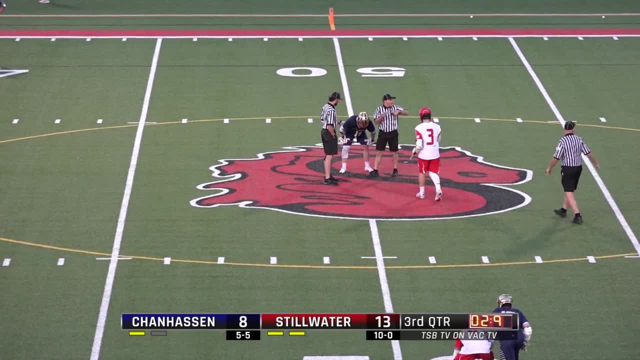 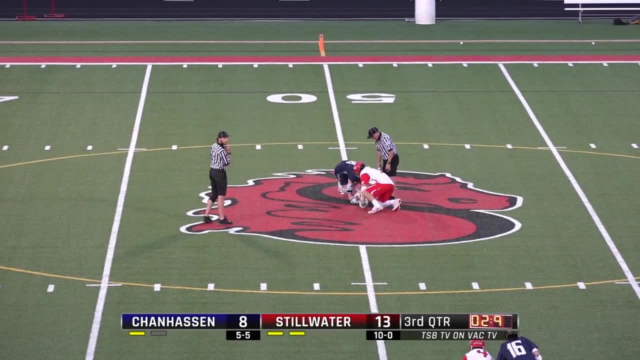 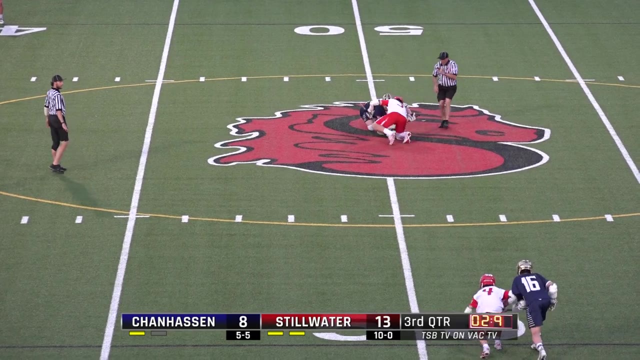 With his third assist And on the season, that puts him at 20.. So Evanson and Summary: Evanson may get the numbers- He leads the team in points, But Summary not that far behind him. Both are just as proficient scoring the ball and setting someone else up for a scoring play. 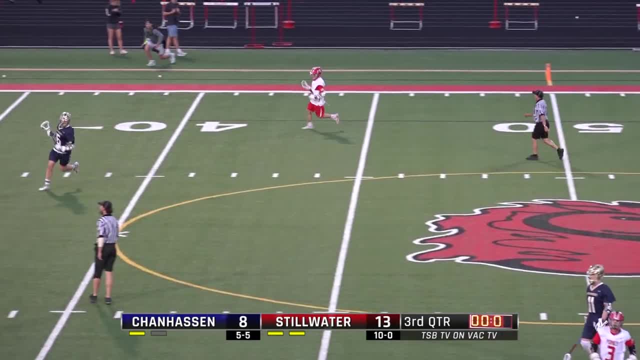 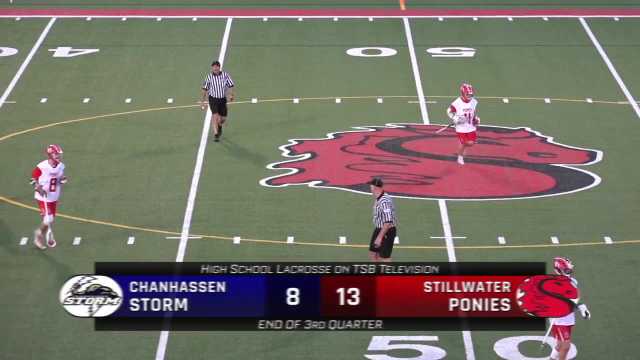 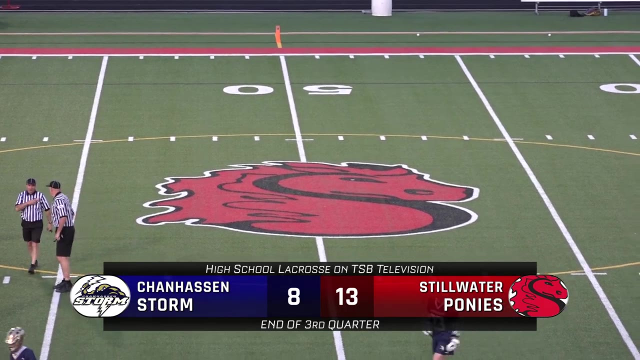 So the Ponies with four goals in the third, Chanhassen with two And again another steady, The Ponies lead the Storm 13-8 with 12 minutes to play. So we'll see if the Ponies can continue this unbelievable run. 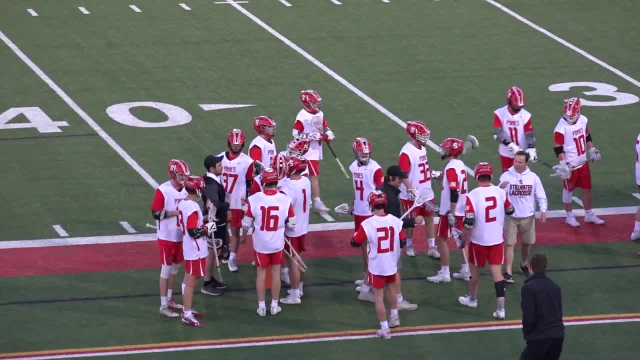 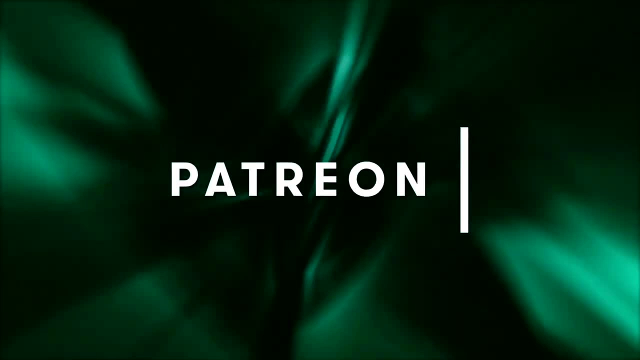 They have already met their mark of 13,, which they have done every game this season. Join us for the fourth quarter in a moment. If you'd like to sponsor a TSP Television broadcast, Patreon is the place. Sponsorships start at just $1 a month. 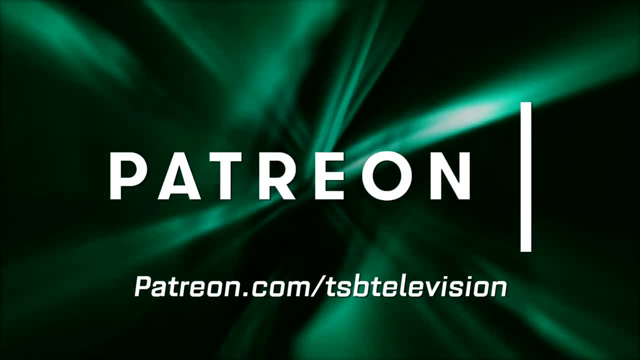 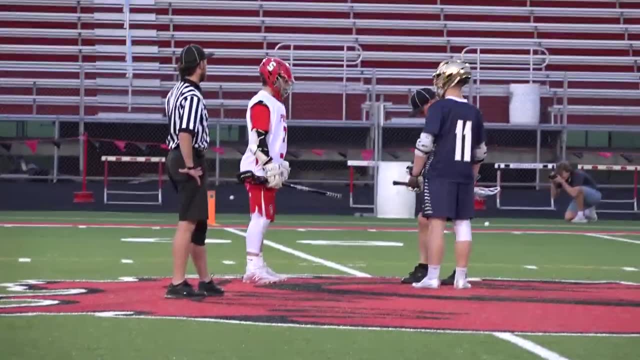 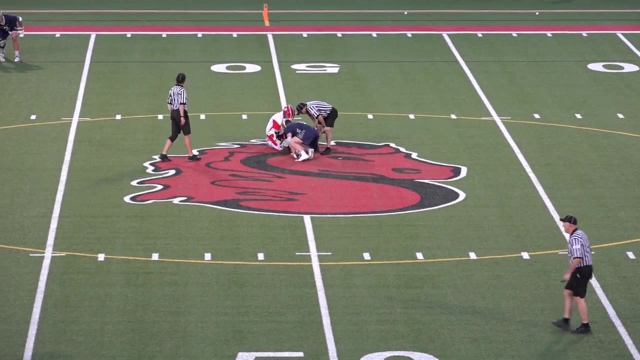 Visit patreoncom, slash TSB Television And make a pledge for premier Twin Cities sports coverage. Fourth quarter about to start. Mike Beaton and Robert Critta, I'll say this: The Ponies PA guys, they know what tunes to play. 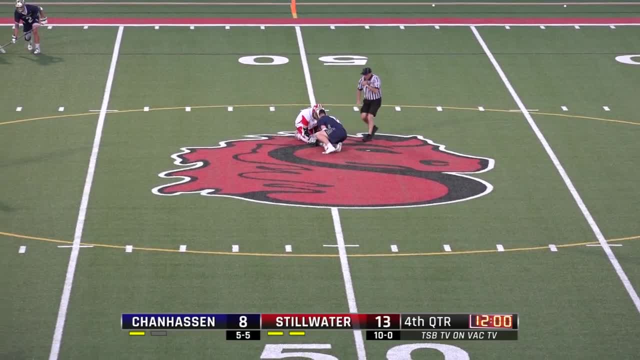 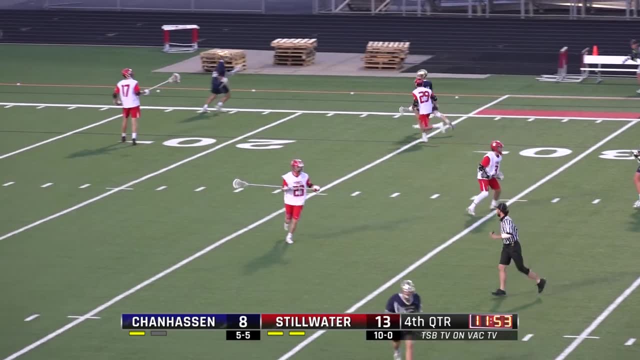 They've come up with a lot of fitting choices, Unbelievable being one of them, And if there's one word you could use to describe Stillwater's season, unbelievable would probably be it. You know, But I find it totally believable. 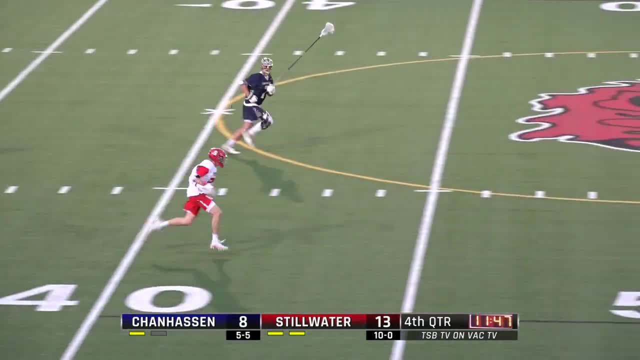 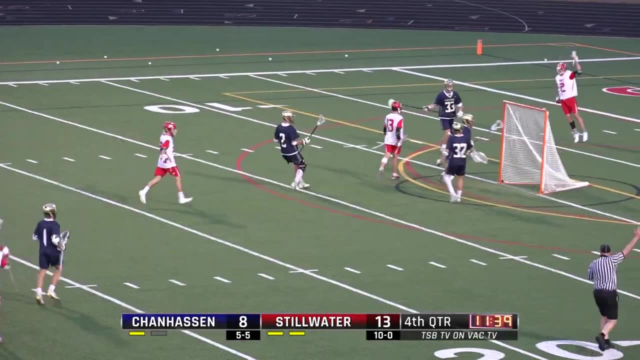 Well, we're seeing it with our own eyes. So I guess seeing is believing, Believing is seeing. Unless your eyes deceive you, Well my eyes don't Berger. no Rebound Score: Quinton White. Quinton White indeed. 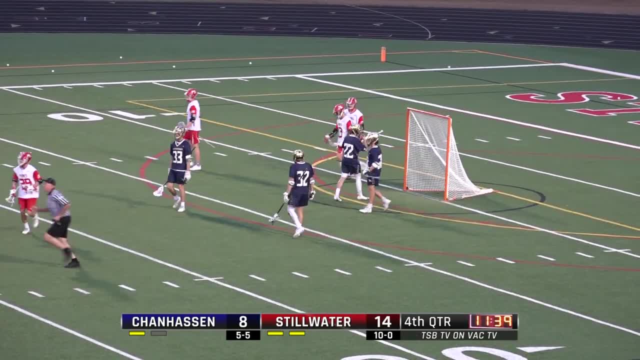 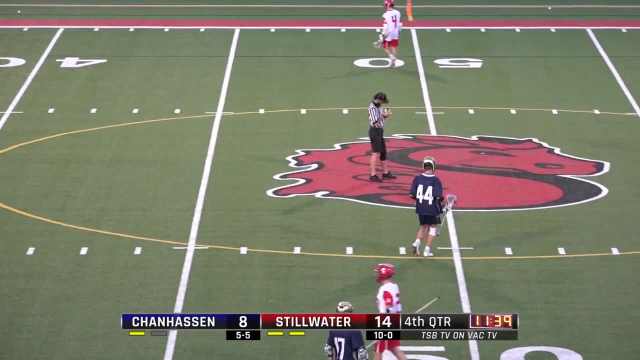 And it doesn't happen often. You see it in hockey, though sometimes You see it in this sport. If the first shot doesn't work, I think that rebound is often your best scoring opportunity, And Quinton White picks up his second goal of the game. 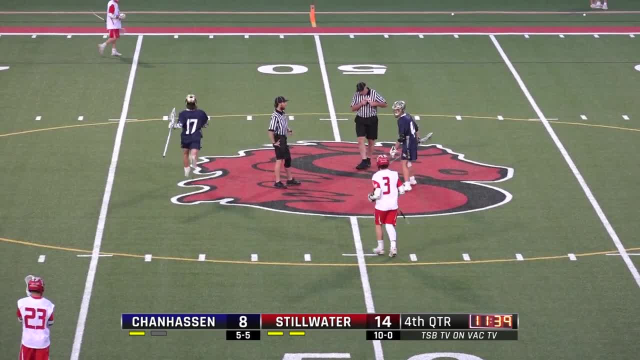 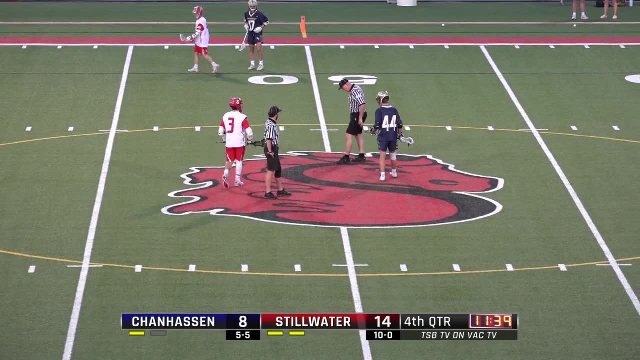 Will they give the assist to Berger? Okay, they don't. I was wondering about that. I don't know how they count assists in this sport, At least at 100% yet. But another quick score to start a period. We saw Ben Carl do that to start the third after he won the faceoff. 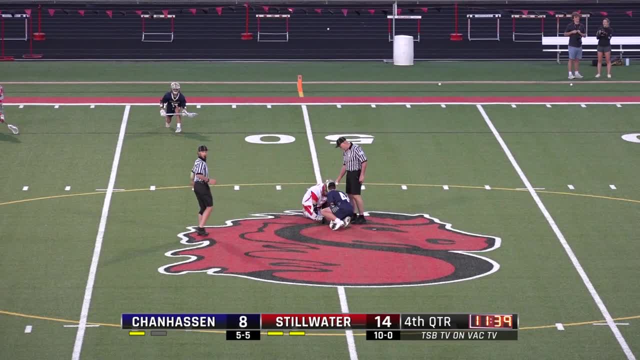 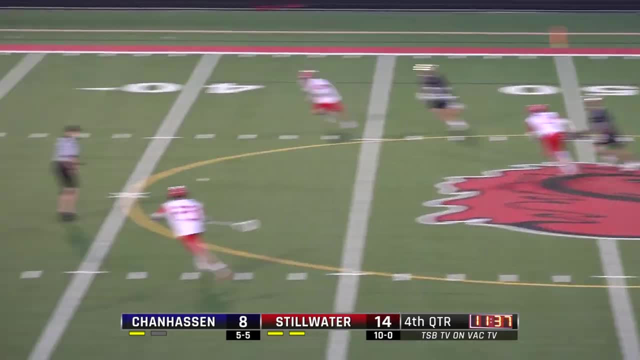 And we see that here, And I think Stillwater. it may not be a 10-goal win, But I think they've got it. They've done enough here to hang on for a win. It would take an awful lot for this Chen-Asson team to make their way back. 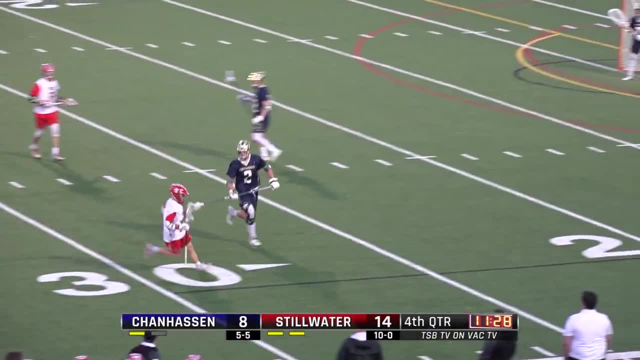 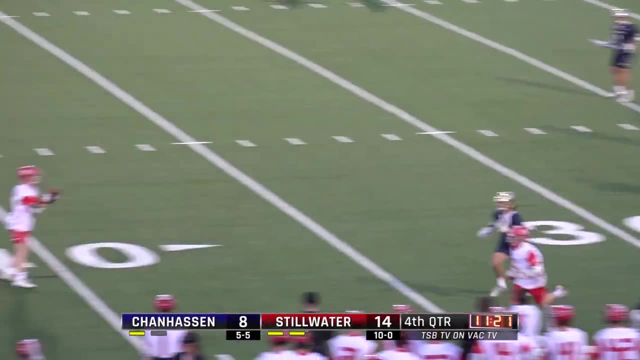 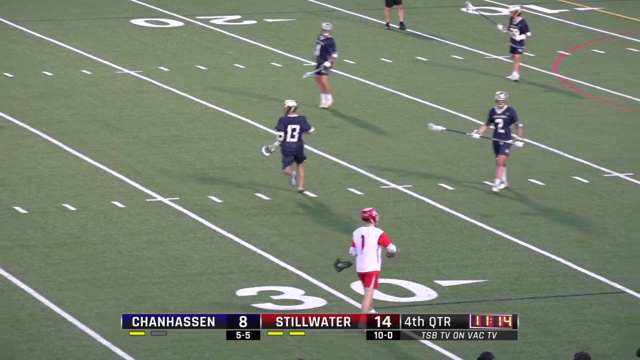 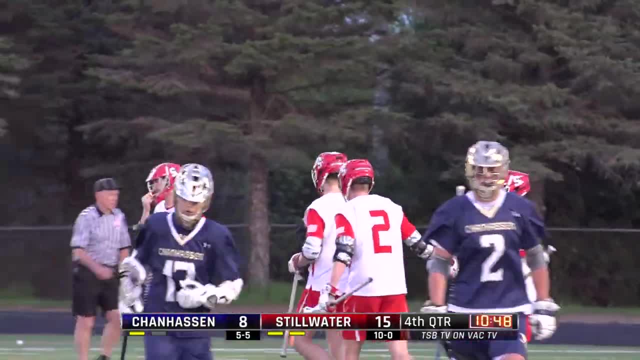 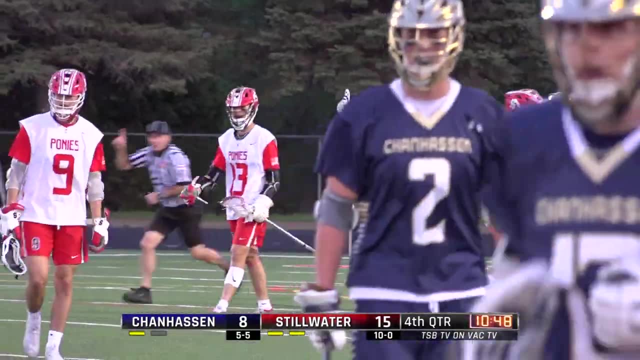 And Thorson makes it four goals with another dose of velocity from the points. Now, if pára´s h aguado a posarão- Oh, you were talking about that runaway ability, Mike, earlier- that Stillwater has, and right now they're doing just that. 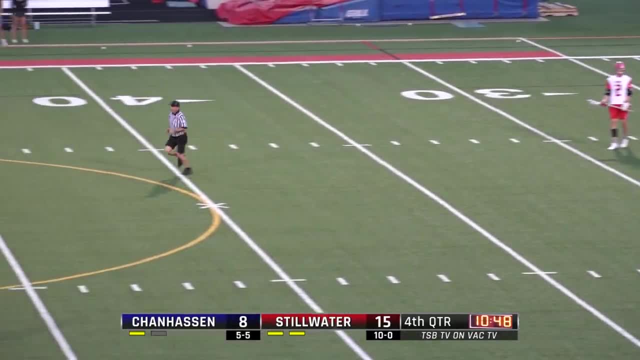 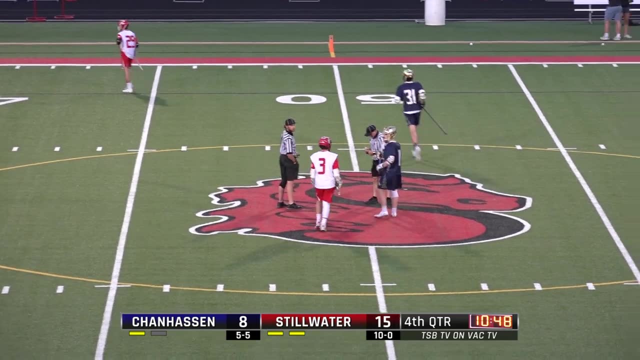 It took a little longer than we thought, but here we are, The Ponies building the lead up to seven. This was a gradual runaway. It was, you know, one goal lead at the end of the first three goal lead at halftime. 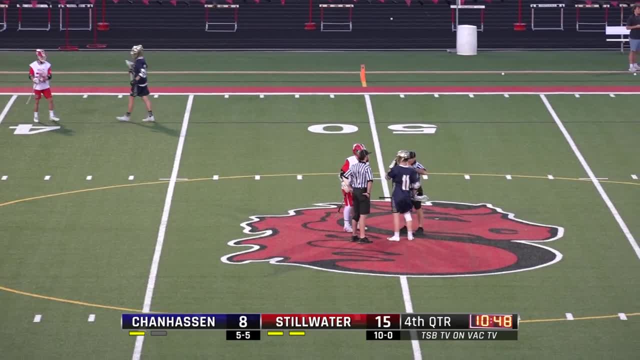 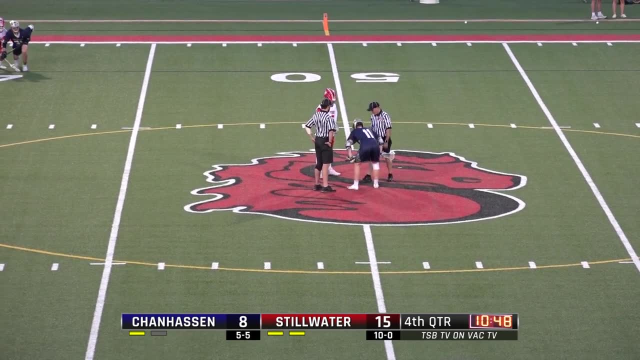 and so we're all waiting. when's that big run going to come? As Summery picks up the assist- his fourth, Okay, Robert. I guess Stillwater can do it gradually too. It doesn't seem like a big win, but here we are. 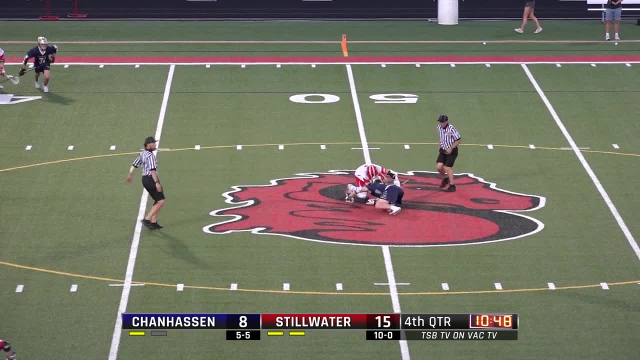 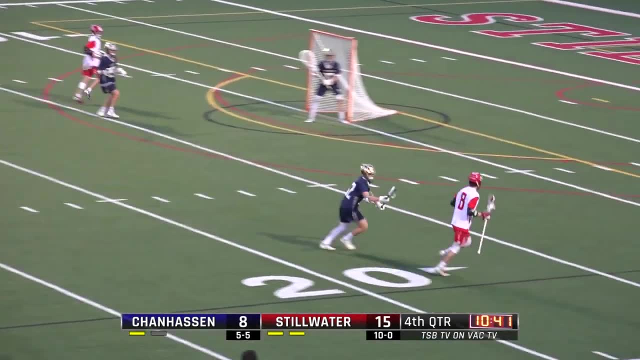 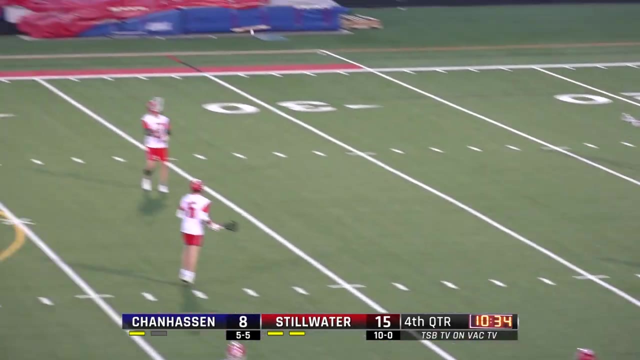 They're at that magic number. every game they've won by seven or more. Jeff was asking us at the quarter break: could Stillwater exceed their season high? They have not scored more than 17.. They haven't needed to. Lots of time left here, Mike. 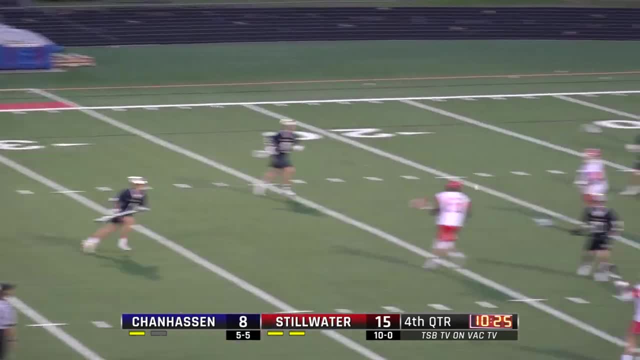 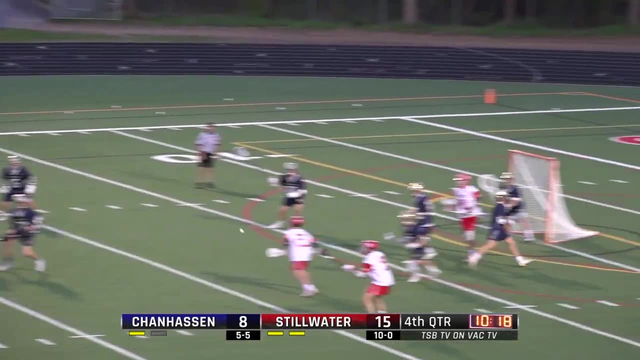 That's completely plausible in this game, Right, They haven't needed to score more than 17,. but it's just a crazy stat to think about And they're second in the state. But when you score anywhere from 13 to 17,, I mean you've got consistency on your side. 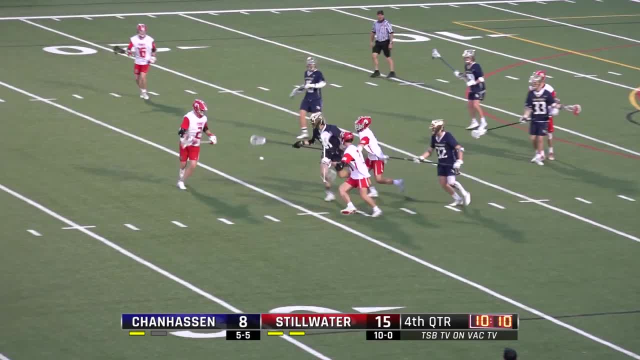 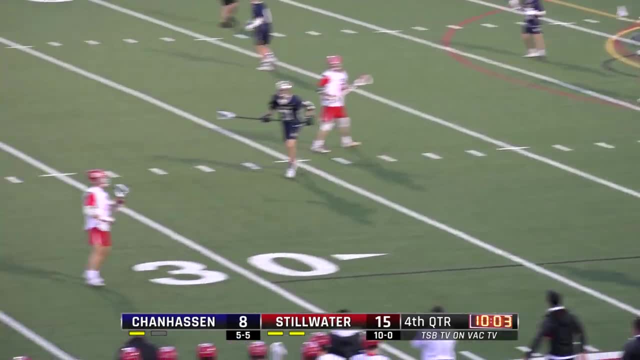 Some fancy passing on the part of the Ponies. maybe a little too fancy, but Okay, we still have a loose ball and it will be scooped up by number 21,, Alex Corbett, And it looks like we might see some of Stillwater's backups slowly get some time here. 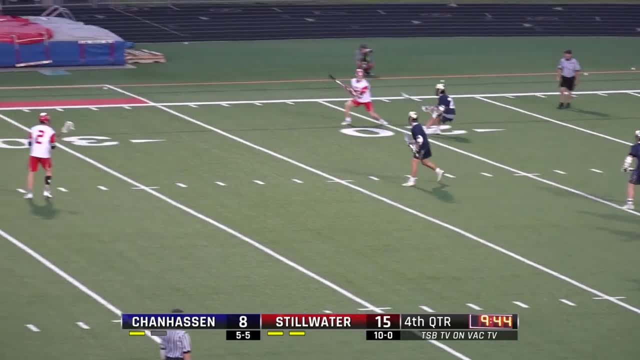 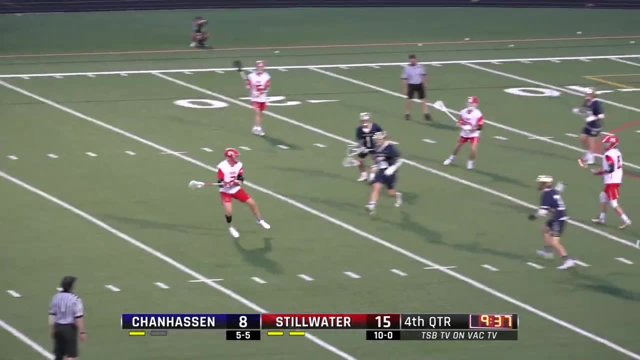 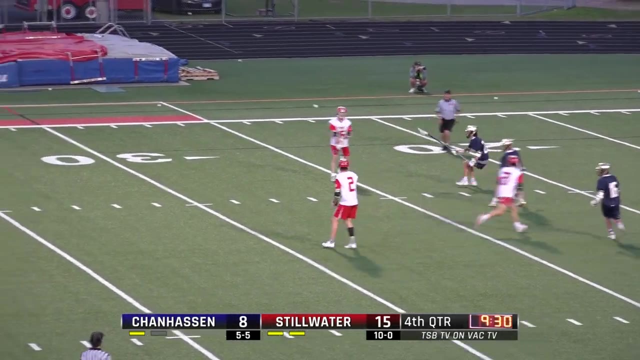 Robert, I'm going to borrow a line from Warren Zevin to describe the Stillwater team and how we should honor them. enjoy every sandwich. Oh gosh, I thought you were going to go with lawyers, guns and money. No, my knowledge is not that deep. 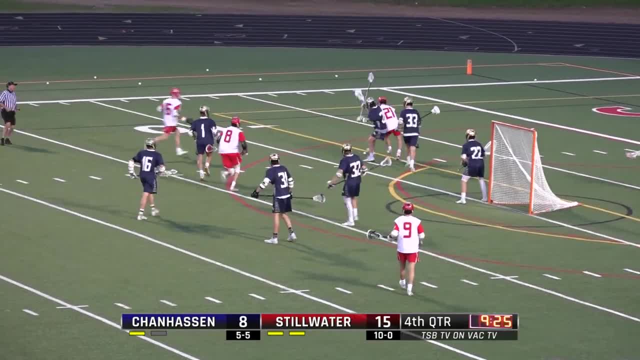 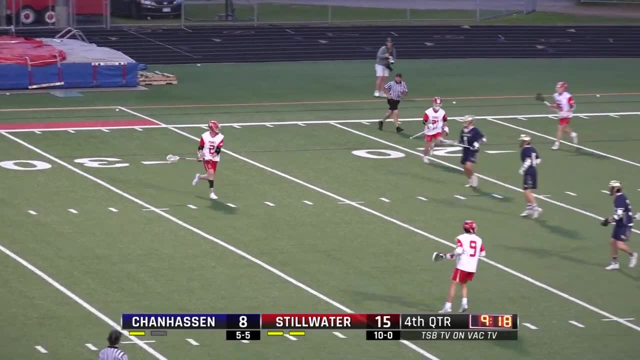 Warriors, guns and money. well, they've been cashing in a lot this season, haven't they? 14-and-a-half goals a game, second in the state in scoring and will likely take over the number one spot in the rankings. 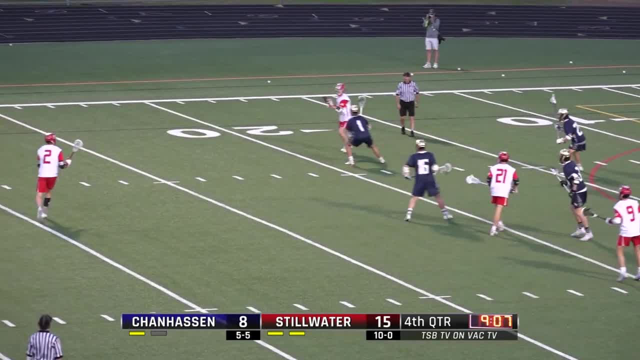 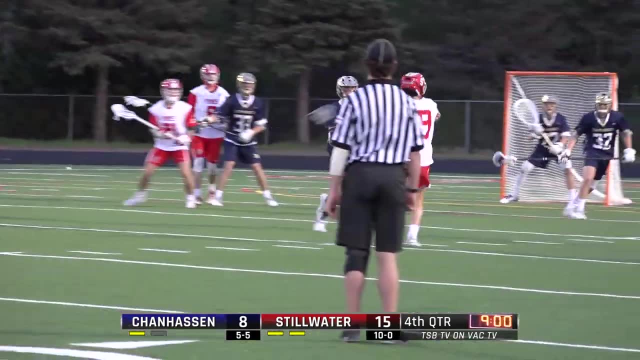 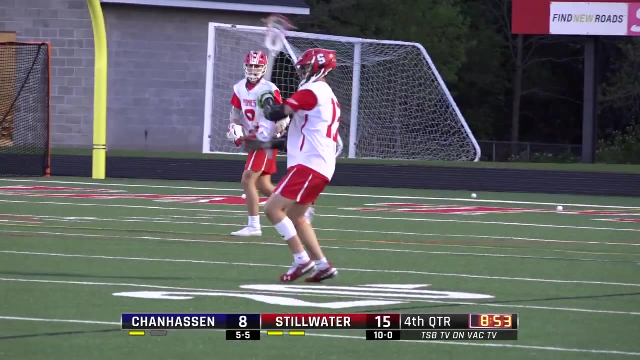 Heading into the final week of the regular season, I wonder how fast they're shooting. He's rolling the headless Thompson gunner. I've got no response to that. Your knowledge of classic rock all of that probably runs a lot deeper than mine. 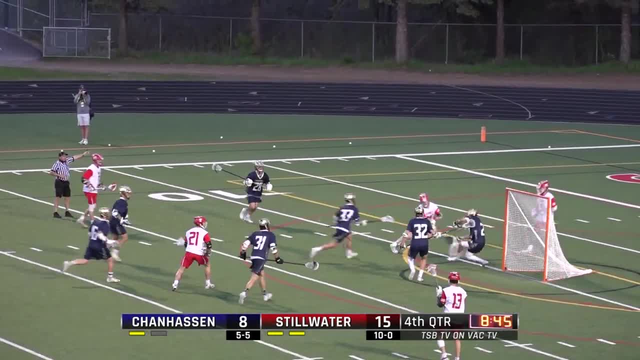 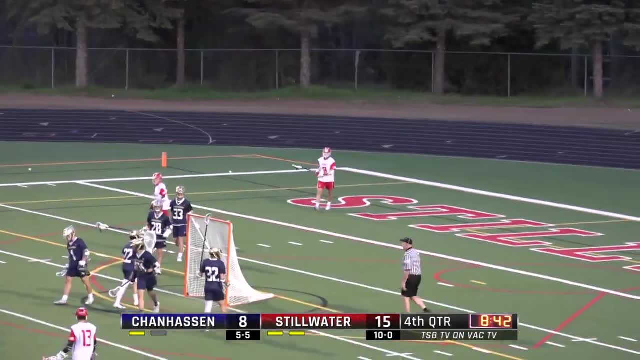 Off-balance. Corbett couldn't get a shot off Summery. where did he come from, Boy? that was a messy play in the slot there, Mike, And it's still a Stillwater ball and another one of those sustained hits. 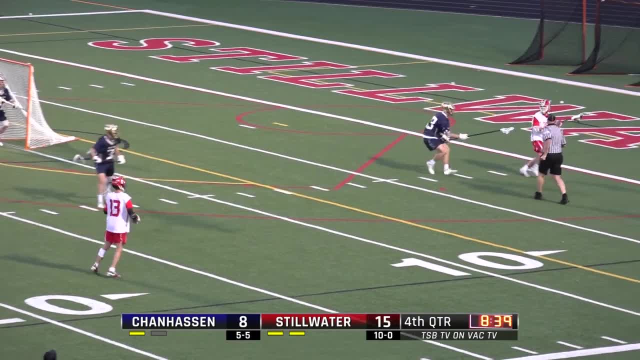 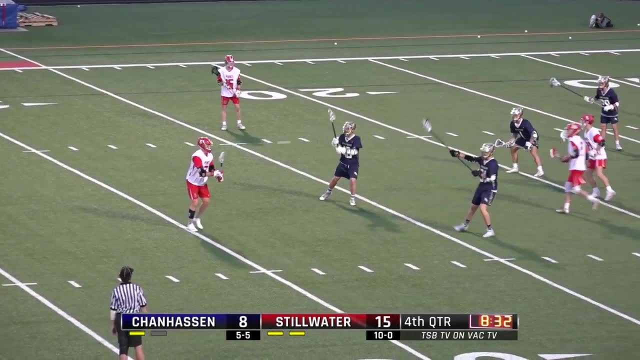 He's got a lot of possession. Well, Chanasson gave them a charge in the first half. This was not an easy win for the Ponies, even though they've built up their lead to normal levels, But what they're doing is completely abnormal. 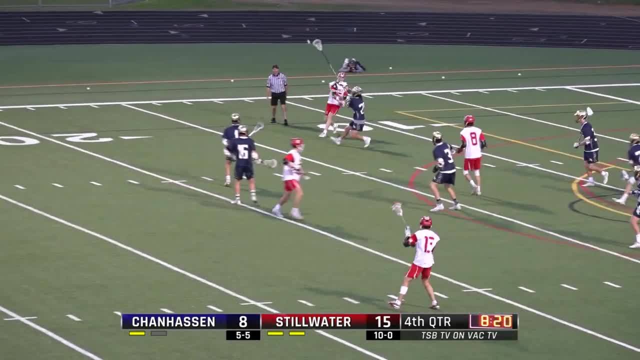 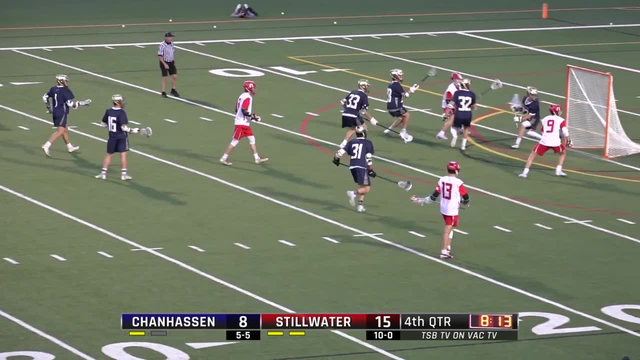 You do wonder, if this comes up in section or state, what would happen if the Ponies run into some trouble or if they have to play from behind, how they'd respond to it. But they haven't had to think about that situation. 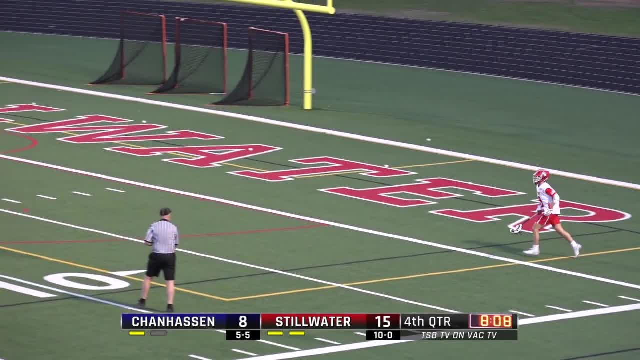 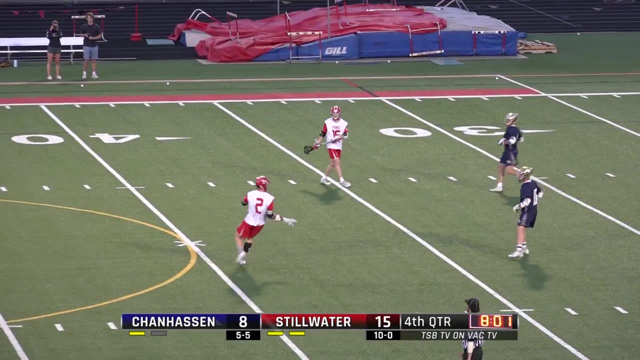 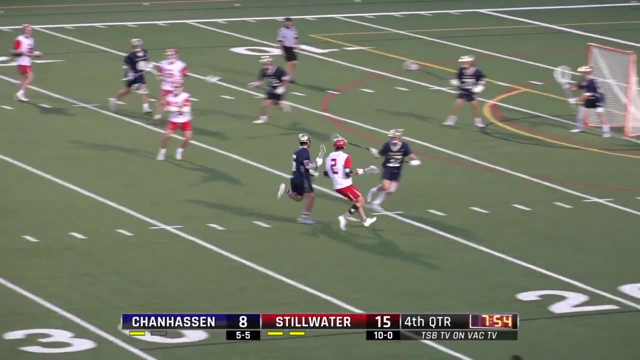 I mentioned this when I shot highlights of the Woodbury game. Going up against a Stillwater team is like going up against James Holzhauer, the Jeopardy champion who demoralizes his opponents. Ken Jennings could take him. Well, Ken, he's not so sure about that. 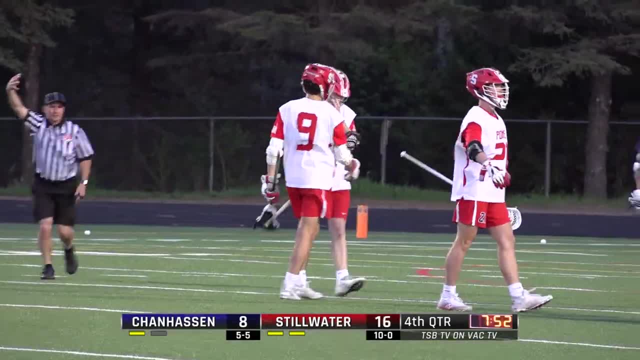 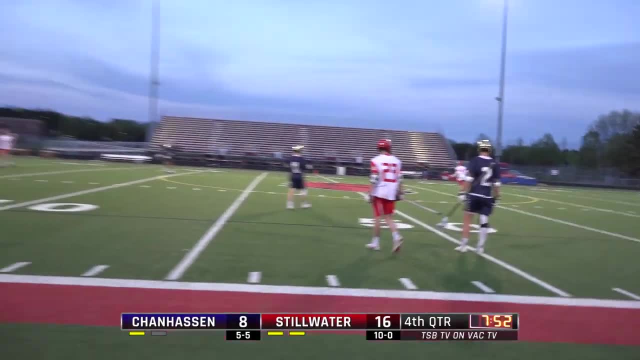 We've got another score for the Ponies. Here's Evanston with another assist And Joe Stingle With his fourth goal of the year. Robert, who would you take? Ken Jennings, James Holzhauer? Well, Brad Rutter. he has yet to lose to Jennings. 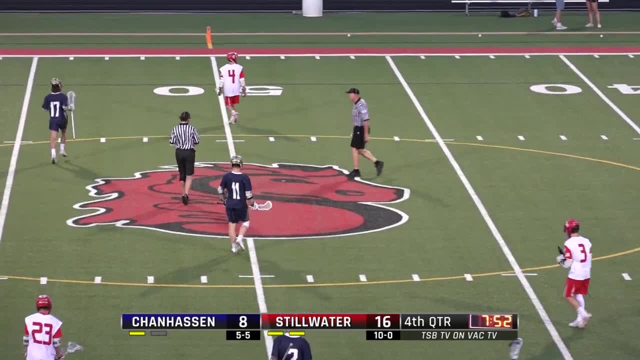 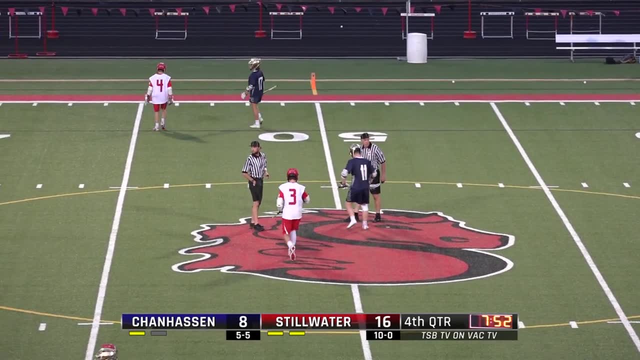 Neither of those. I'll take Joe Stingle for nine, please. You'll take Joe Stingle for nine. Well, you'll find a couple of daily doubles with Joe Stingle tonight, With four goals in this game and on the season. 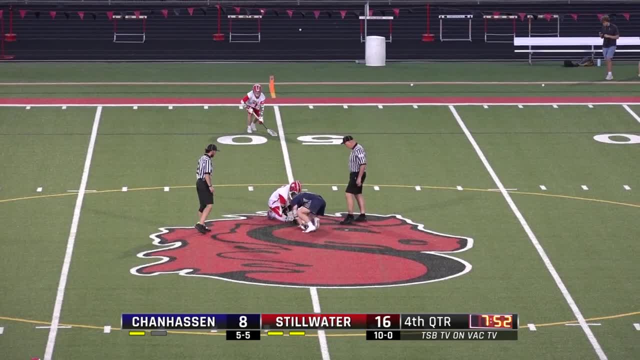 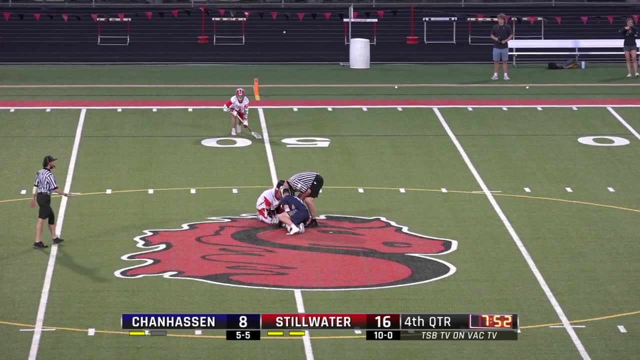 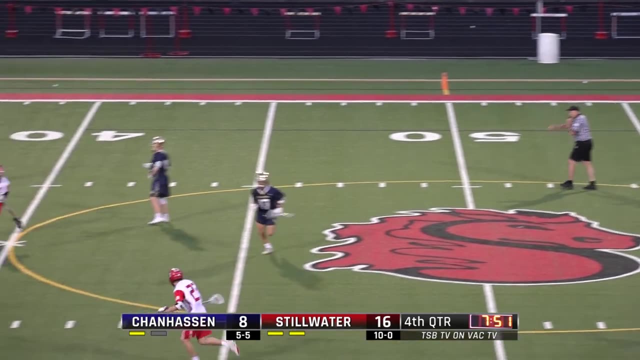 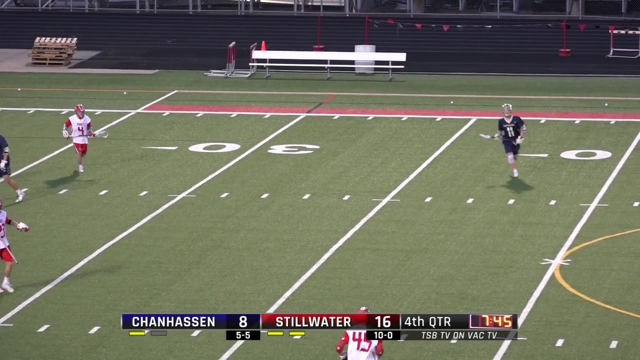 Joe Stingle with 26.. So He is. He's close to Blake Evanston for second in the team race And Thurston we'll see where he matches up with 35 goals on the air. Come on, Nate. Well, and I mentioned James Holzhauer because the way Ken Jennings played. 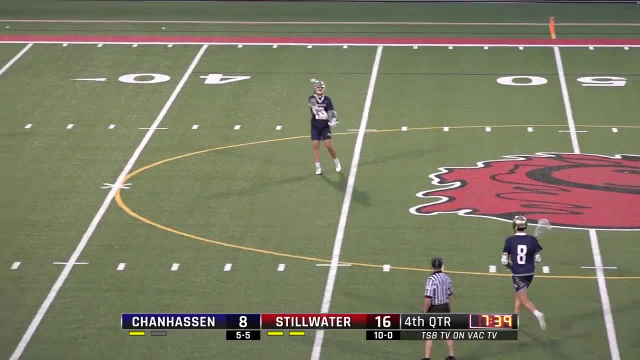 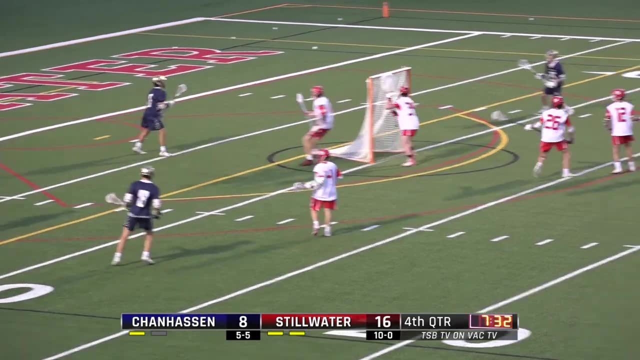 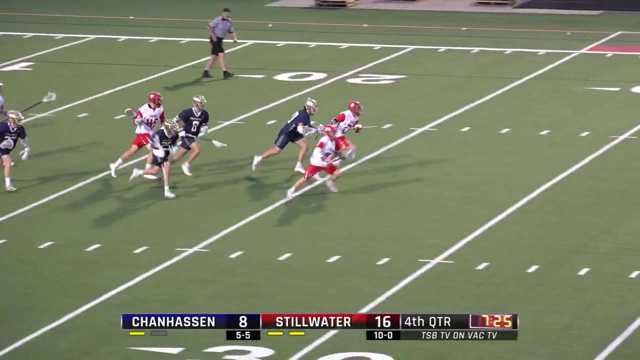 he was a Well. I followed his run immensely back in the day when he won. He won 74 games in a row. but James is doing it with a dose of analytics on his side, And so by the time you get to final jeopardy, he's built up these big leads, big wagers. 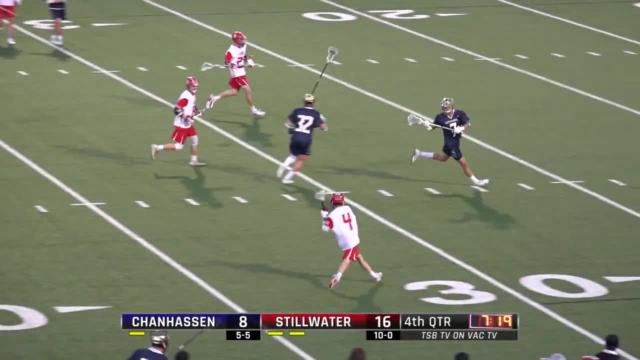 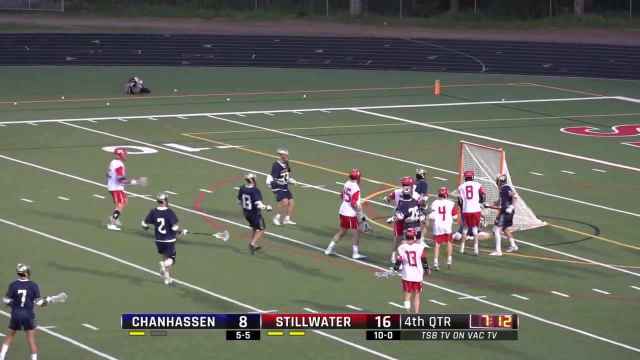 And Stillwater. it took a little longer, but they build up these insurmountable leads and they just take the life out of you. And oh, that shot just hit the top of the crossbar And Stillwater scores anyway. Cody Berger cleans up the mess on the ground. 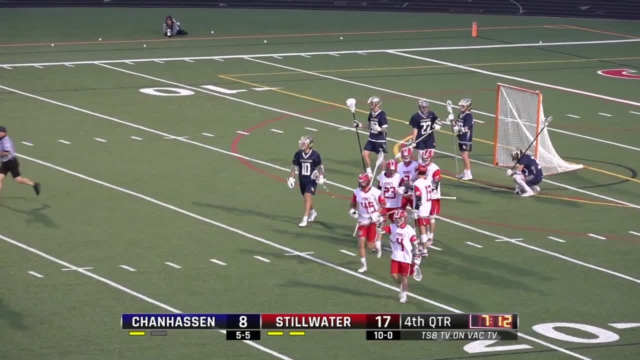 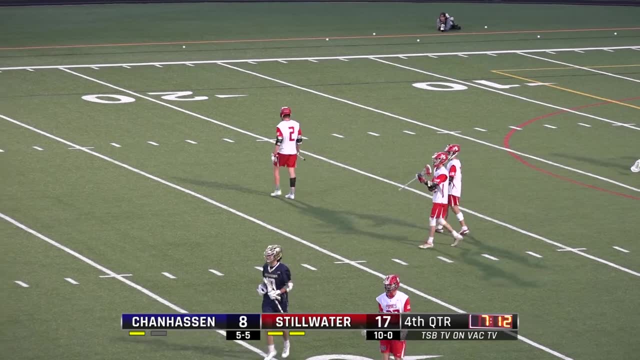 People are trying to scoop up a loose ball right in front of the goalie, but Cody Berger ends up picking it up, Scooping it right into the net. Cody Berger's one angry whopper, isn't he? And I'll show myself out. 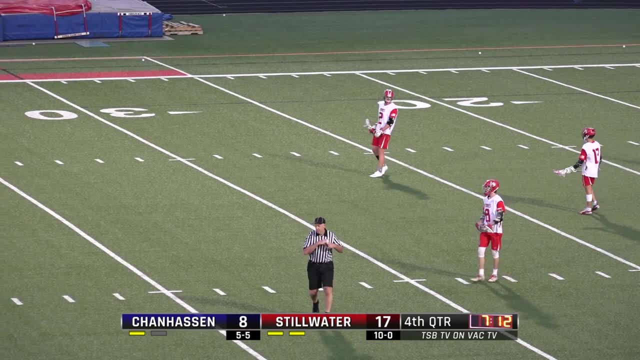 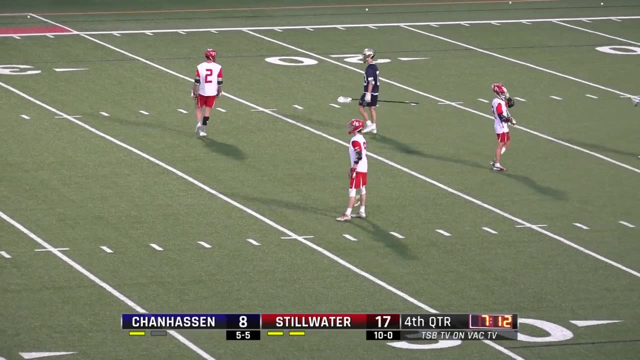 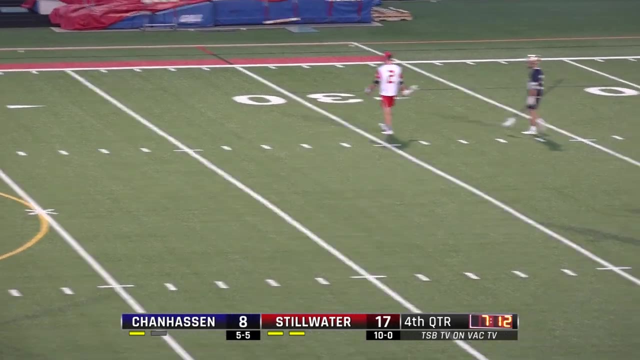 All right. Stillwater has matched their season high. Cody Berger scored, but Ben Long was inches away. It hit the crossbar. Ben Long could have added his name to that list, but the Ponies: another big win. I don't know if I'd say whopper Mike. 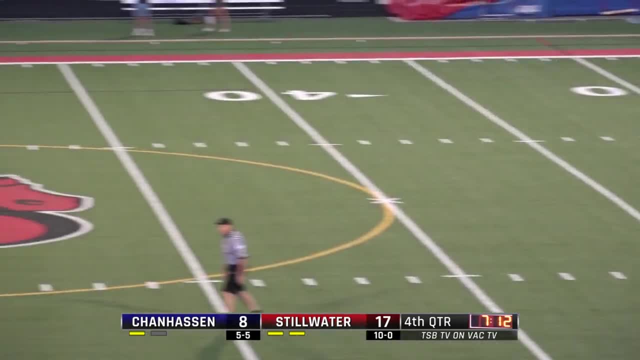 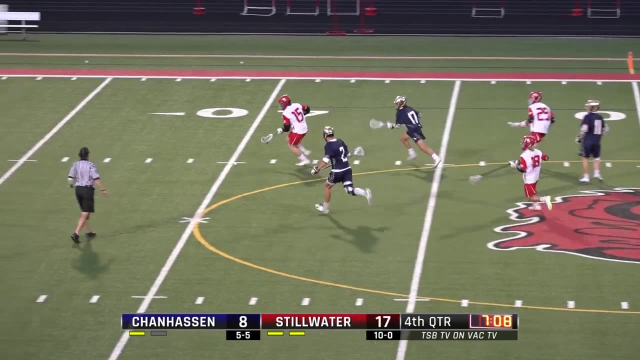 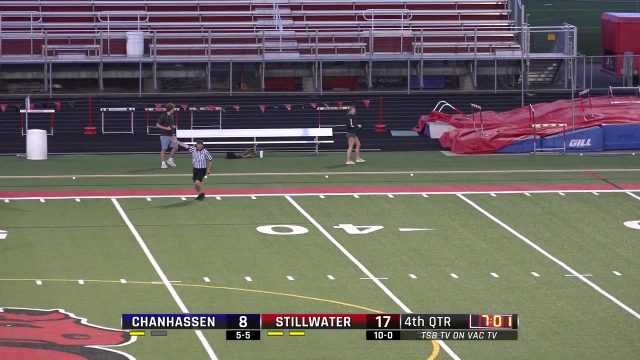 but last week I had the finest venison burger that I've ever had. Compliments of Cody's dad. I have not been invited to a cookout yet by the Ponies, but it's been nice to get to know all these folks. 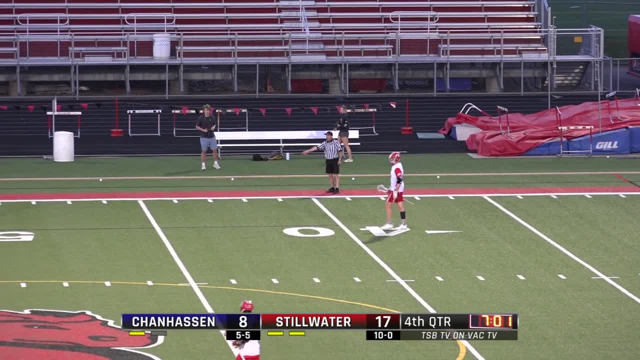 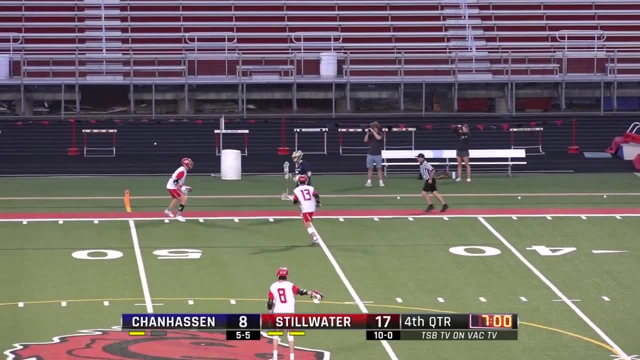 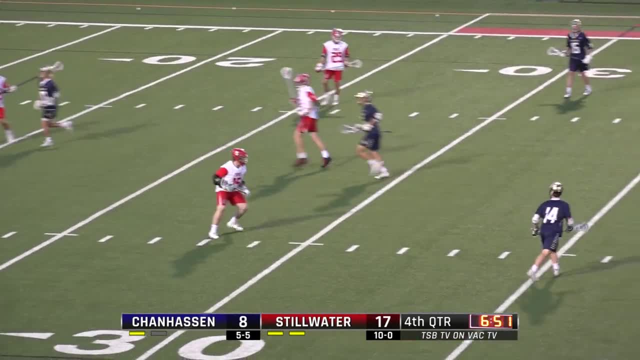 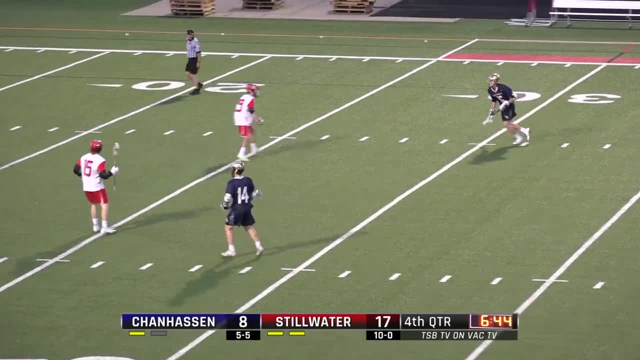 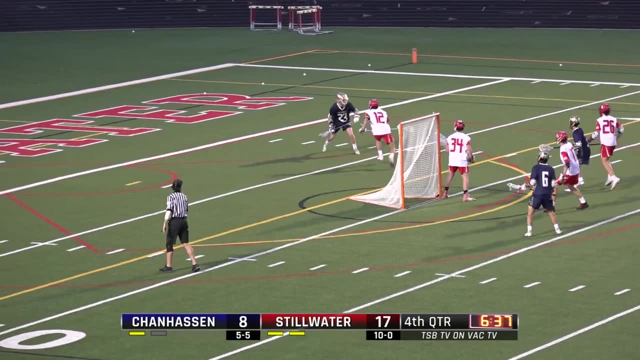 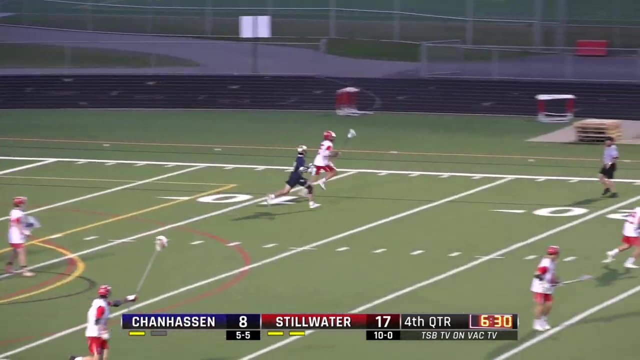 Well, it doesn't matter. They're going to go to 11-0, and they're very likely going to be the number one team in the state in the final poll of the season. I've not been invited to a cookout, Robert, so I can't take your word on the burgers. 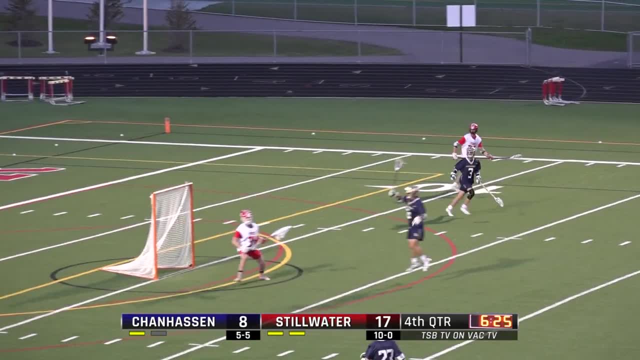 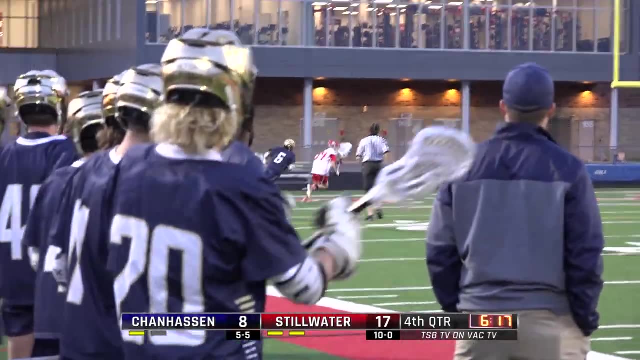 but the girls' basketball team did invite me to their banquet so I got a ticket taste of Grand Pizza. I think it's Grand. yeah, the Grand Pizza Ballroom downtown Stillwater, Ahrens under duress, dumps it. 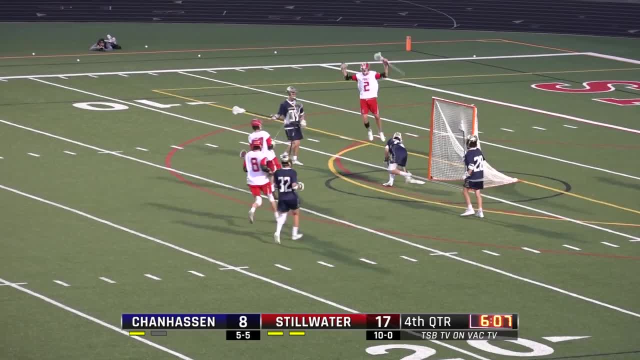 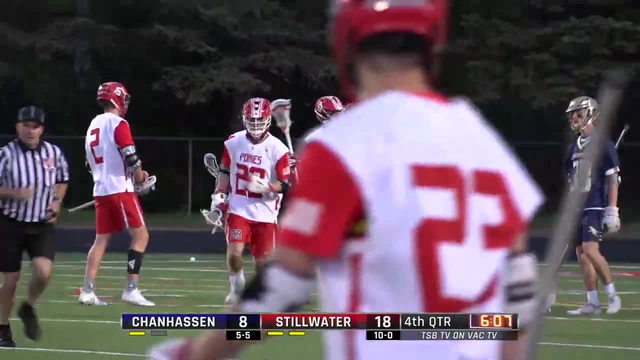 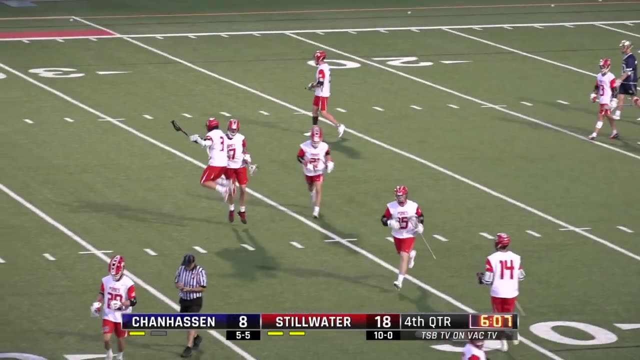 That was a touchdown pass, Aaron Rodgers-like and Justin Siegfried with the score. That was like an Aaron Rodgers Hail Mary, where you pass it all the way from midfield and you find your receiver downfield for the score. Does Ahrens? will he get the assist for that? 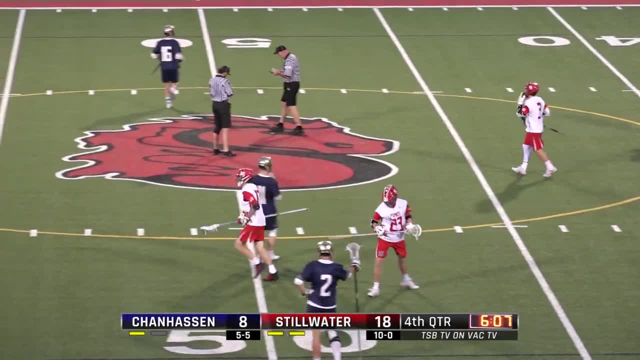 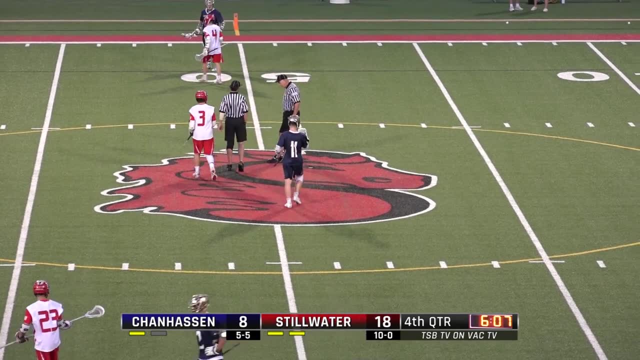 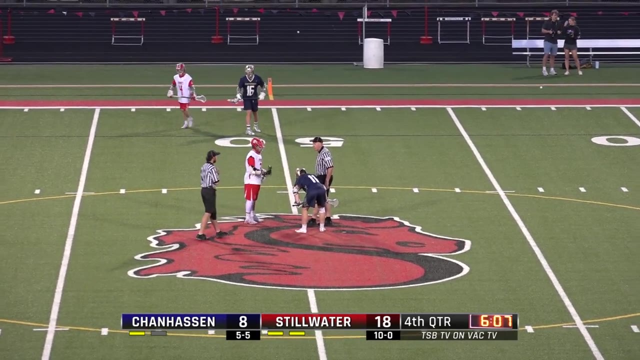 That's what I want to know. Yeah, he will. Let's find out He should. Yes, he will. Gunnar Ahrens with an assist, And that's great for Gunnar: he gets an assist. and it's great for Siegfried because, as a defenseman, 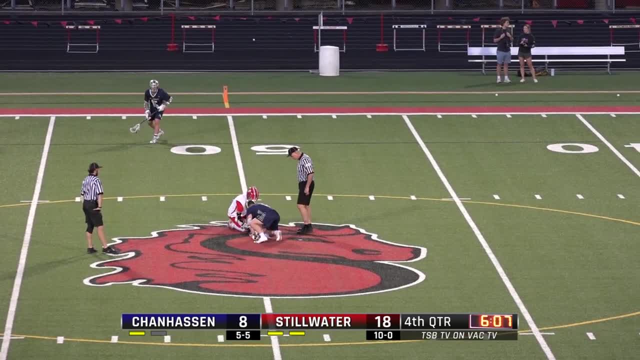 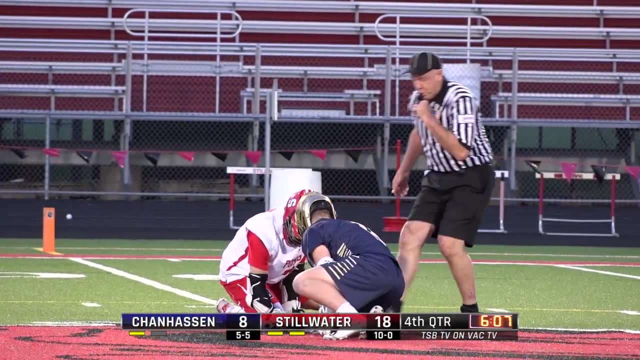 you don't really get. you don't usually get a lot of good looks at the net and he got a great look and he made it pay. In fact, Justin Siegfried- his first goal of the season And it's the one that broke the ceiling. 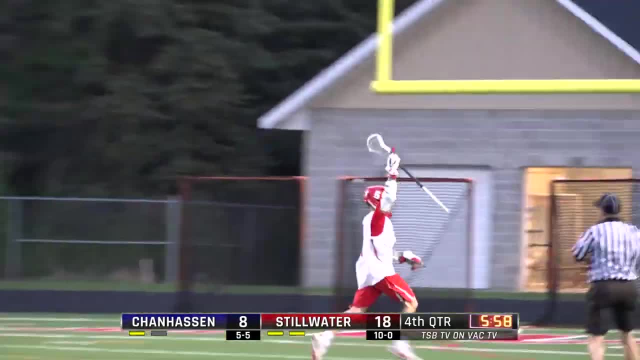 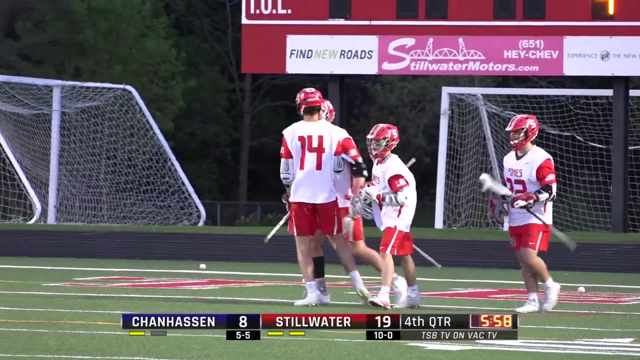 and Gunnar Ahrens. that's his first assist of the year And Stillwater wants more. They'll get more. Ben Karl with a face-off win, his second goal of the game. I'm going to say that's a season high for him. 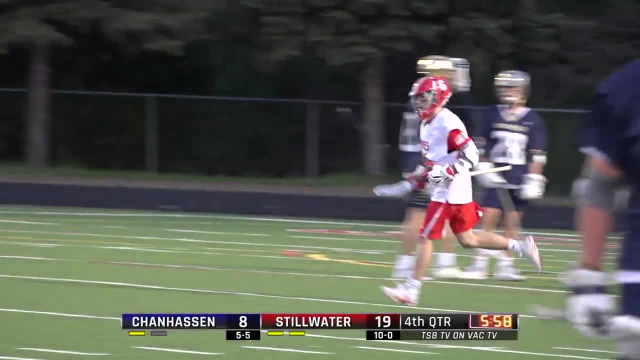 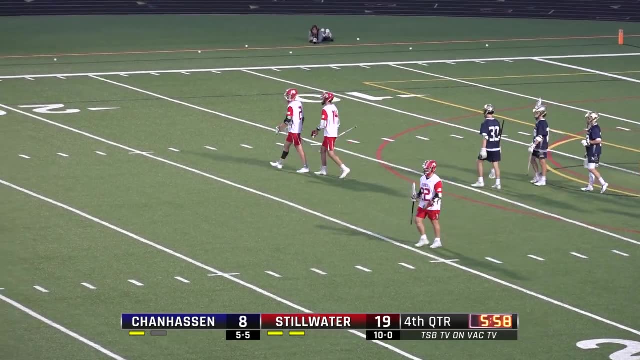 I'll confirm it. That has to be because, yes, he's only scored one goal on two occasions. The Pulitzer Prize. The Ponies are piling on, They've broken through the ceiling and they want to go straight to the stratosphere. 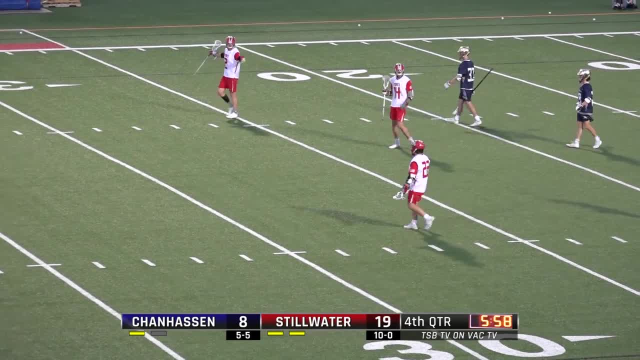 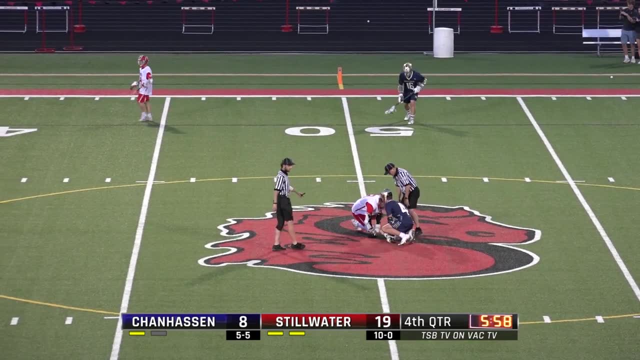 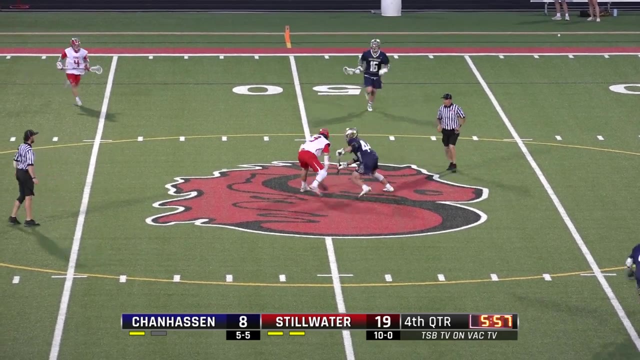 The speedy Ben Karl, showing what speed is Indeed. All right, Can they get 20?? They have not scored 20 at all this season. Can they get that mark? What is the mercy rule, by the way? What's that threshold? 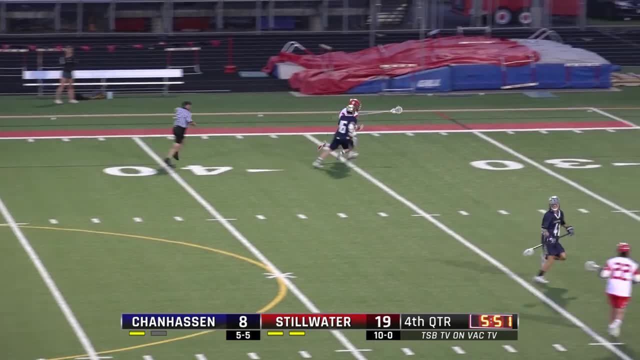 One one. Do they have one in lacrosse? 50 goals, 50. If it's 50, we've got a long way to go. Robert, I don't think we're going to get 50 by the time this one's over. 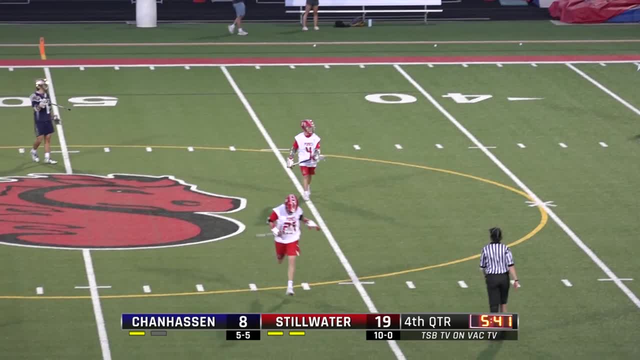 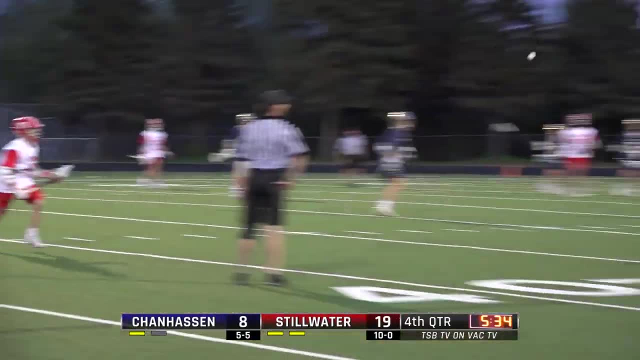 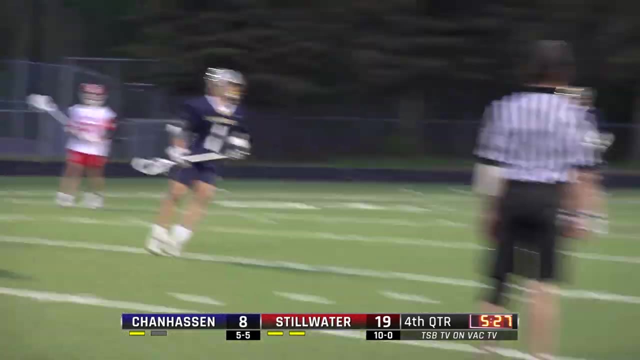 This is where you can tell the Ponies are having fun, Ahrens, with that Hail Mary, that deep pass downfield to Siegfried. Like I said, that's something Aaron Rodgers would love, The master of the Hail Mary. 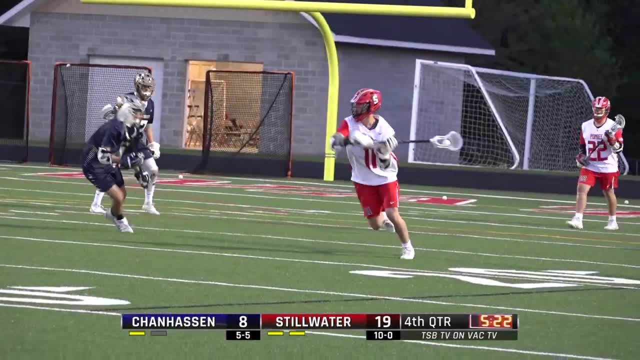 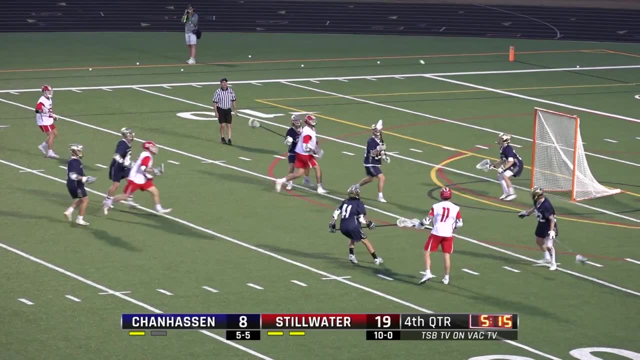 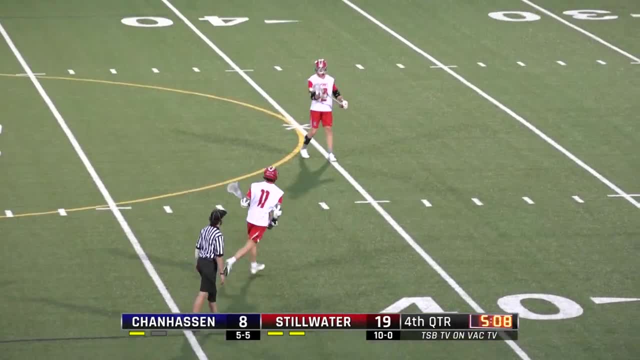 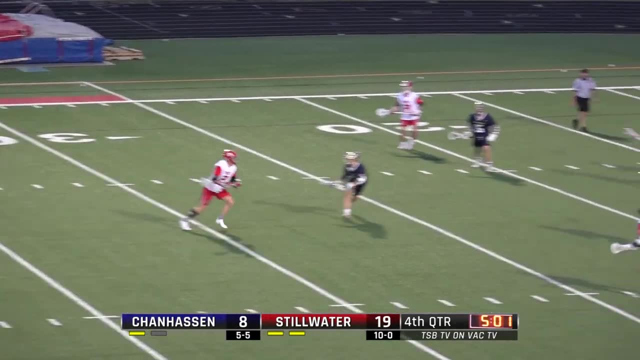 You get an assist. I'm sure it's not his first one this season. It was his first Gunnar's first assist. He had not had an assist all season. Well, he's been plenty due then. Well, he's had plenty of saves. 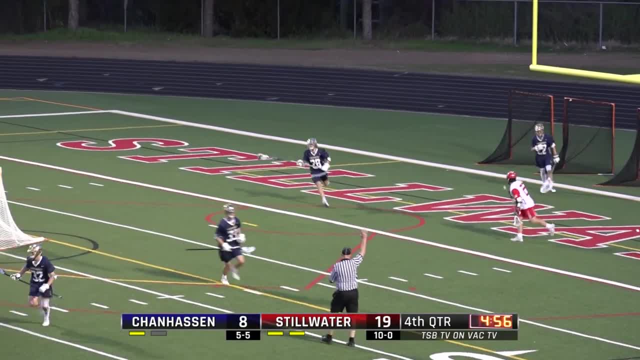 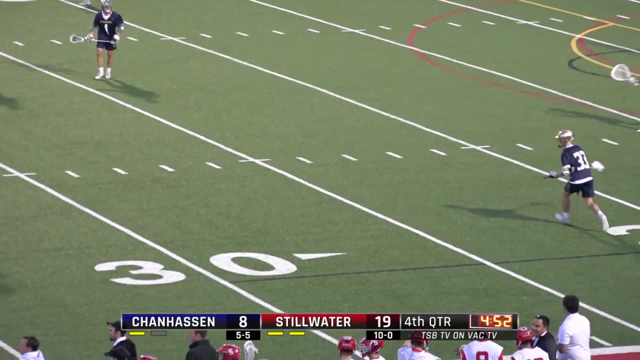 I guess the last thing he would need is a goal, right? Uh, It could happen. The way this game is going, Stillwater with five fourth quarter goals. I'm sure Stillwater has some trick plays in its Playboard. 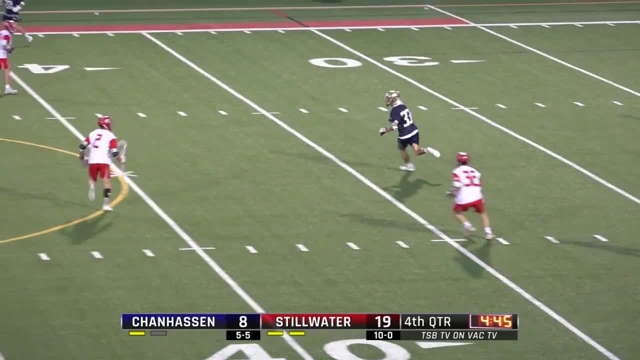 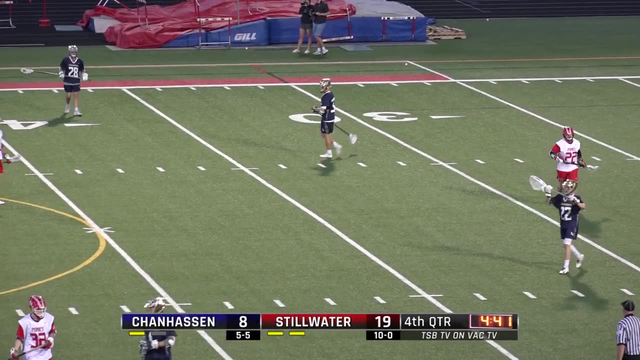 And it's crazy to think we were talking about how close a game this was and when's that Stillwater rally going to come. Well, it came here. Yeah, up to the first half it was pretty close. After the second half it's been all Stillwater. 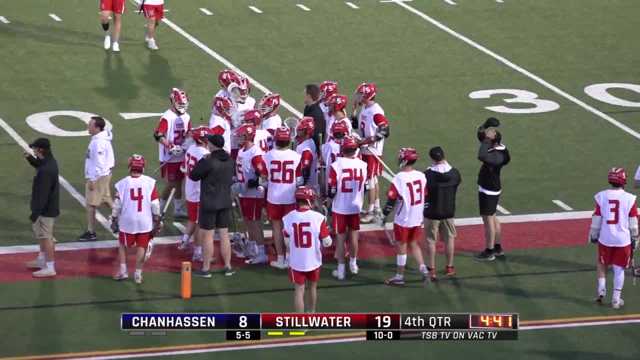 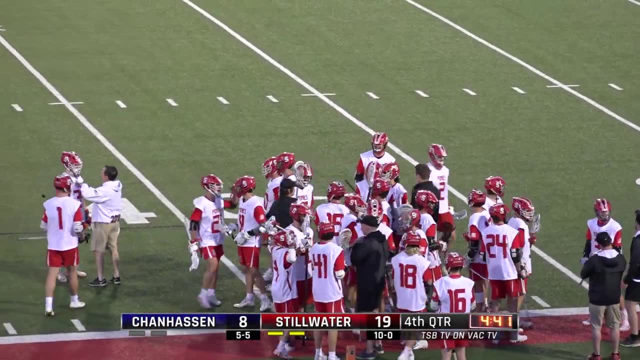 Well, and sometimes it doesn't matter when you get that first half well, sometimes it doesn't matter when you get that big run. sometimes it comes early, other times you gotta weather that storm. no pun intended, i'm sure chan has only heard that 50 times. 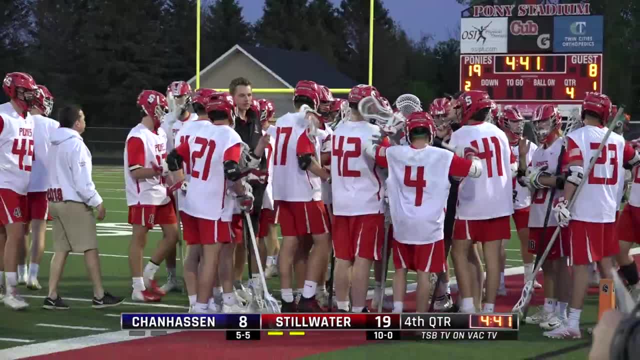 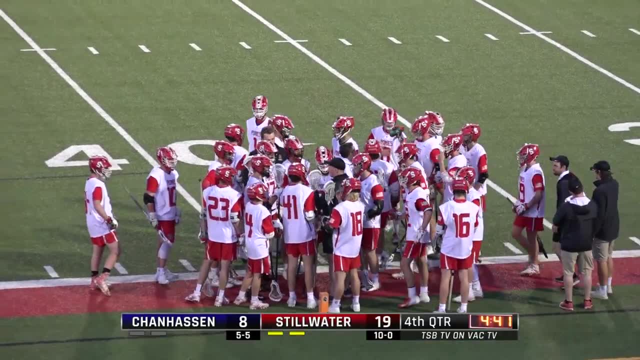 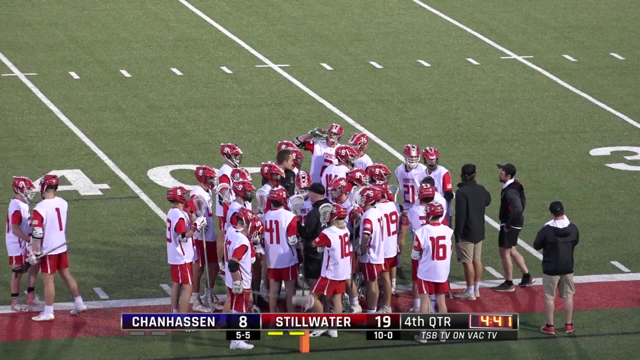 yeah, i, i know no storm, no storm is going to affect stillwater tonight. nope, not with that stable offensive there's that gallops to giant margins. so i think chan hasn't got the time out there. robert, this will be the last regular season game we cover on the boys side and we expect them to do big things in the playoffs. 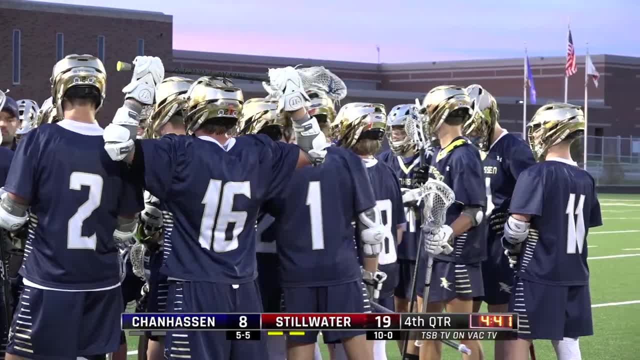 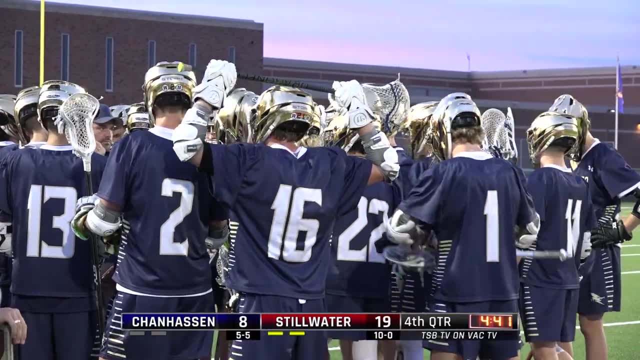 yeah, maybe the turnovers. you know they still have that on a couple occasions once, or you know, here and there, but i think that's the only thing you really got to clean up. if you're the ponies, at least going into section play. oh, they're looking really good and this is this you know. 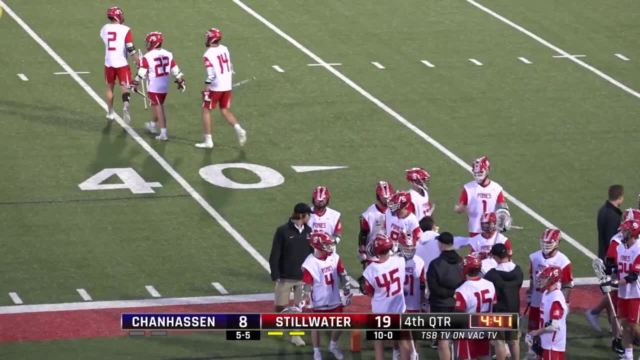 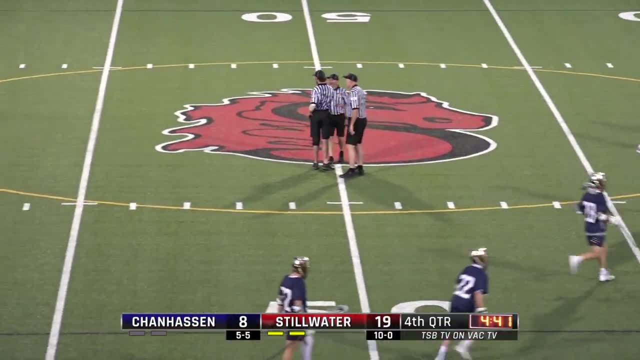 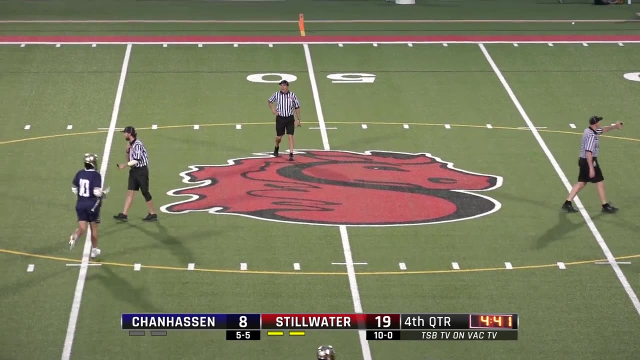 this is their year. you know, minnetonka, eden prairie, some of the perennials prior lake may have something to say about that, but we won't know until we get to the state tournament round. you know, the ponies one and done right the ponies, the host park of cottage grove next week, that. 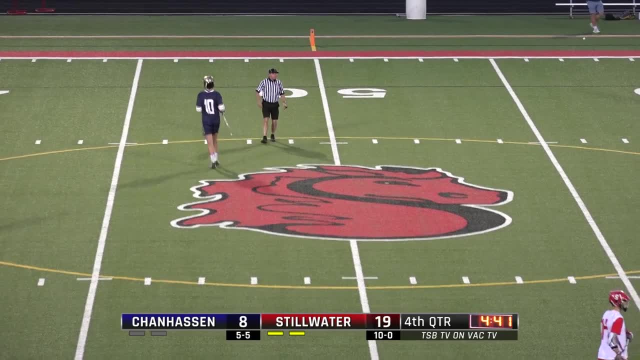 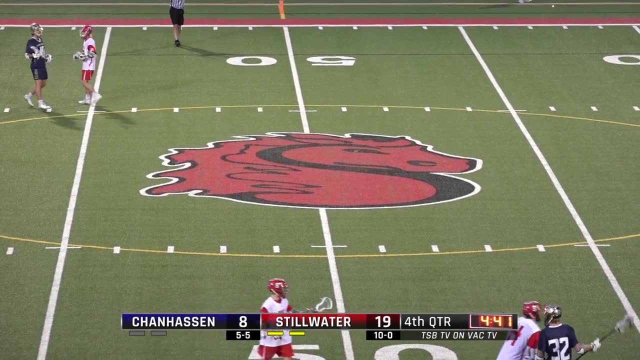 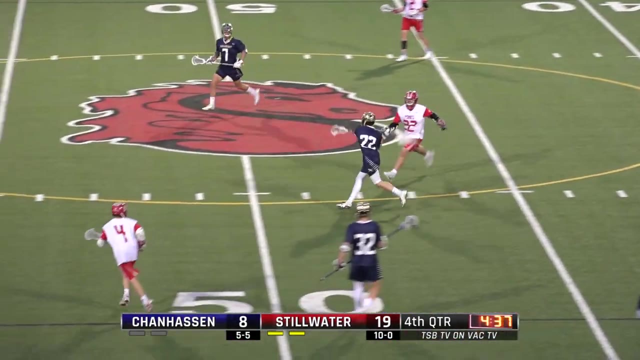 should be a winnable game. wyzetta, not one of the lake conference powers, even though ted and i joke about the lake conference and how much they win stuff. yeah, it's like: hey, stillwater, they're the pride of the east mexico. There are a lot of teams from Stillwater that make it to state, as we have seen. Soccer, volleyball, basketball: lacrosse has a good chance of sending both teams to state. Baseball: softball: won state last year. gymnastics: The ponies won five state tournament titles last year, 15 section titles. Ted and I have put in a lot of hours. 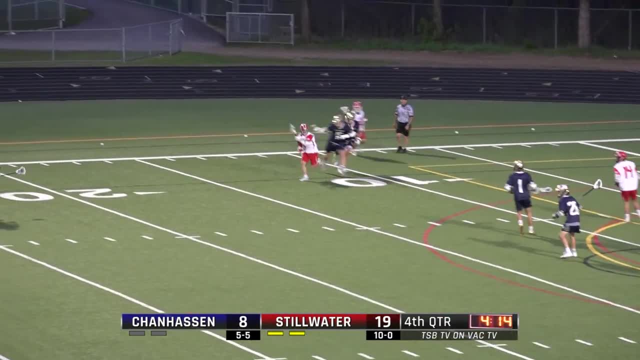 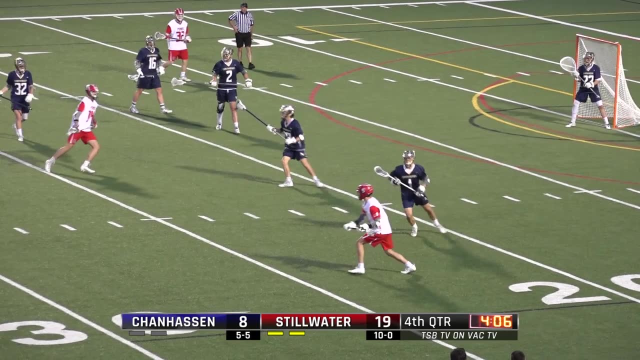 It's not like covering the Detroit Lions, where you know you'll go home, most likely at the end of the season. Let's see. And they get 20.. Will they push for 20?? That's the other thing. Lots of time on the clock. 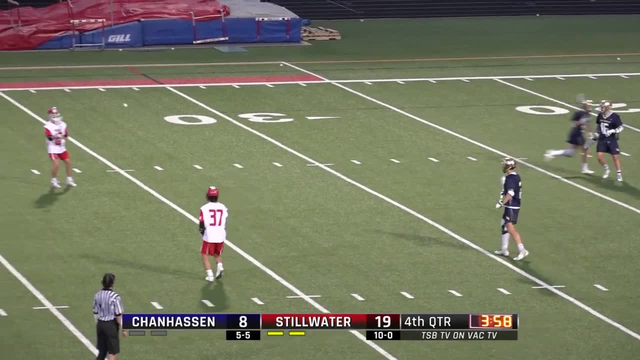 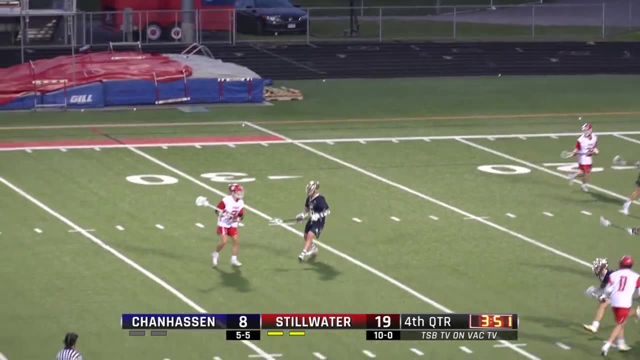 I guess it all depends on if they want to run out the clock or if they want to get that 20th goal, And it's going to come from the backups, as the starters have been pulled out And it makes sense at this point. 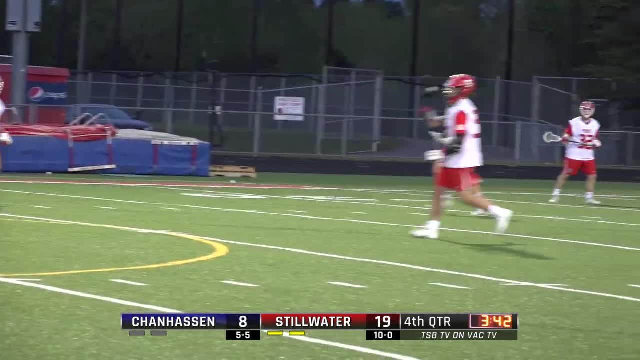 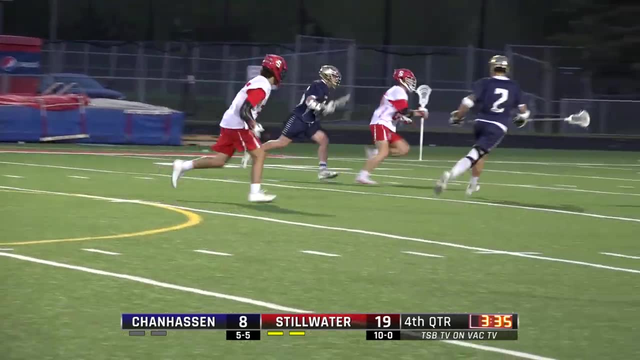 They've done more than enough. So you see Logan Bees and Carter Bees, One, two, three, One, two, three, One, two, three, Number 21,. Alex Corbett's going to get some time. Clay Batterton, number 14.. 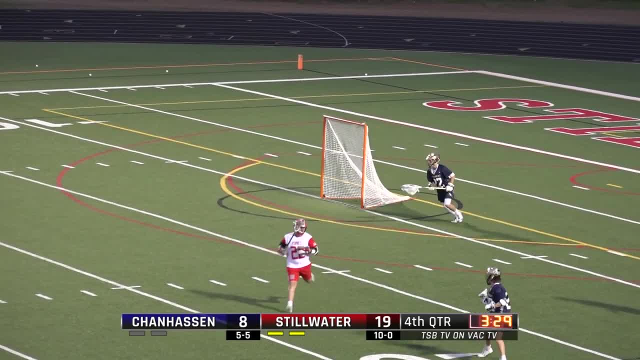 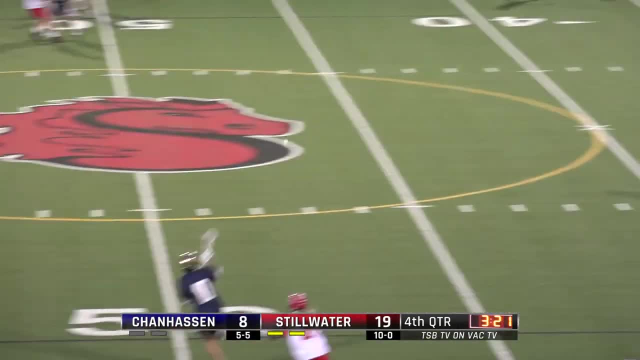 There's Corbett with a shot, Some other guys on offense who will get some playing time here: Theo Robinson and Sheedon Von Buren, number 32.. Hope I got that name right. And we've been praising the offense for Stillwater so much. we should not ignore what they did to them. 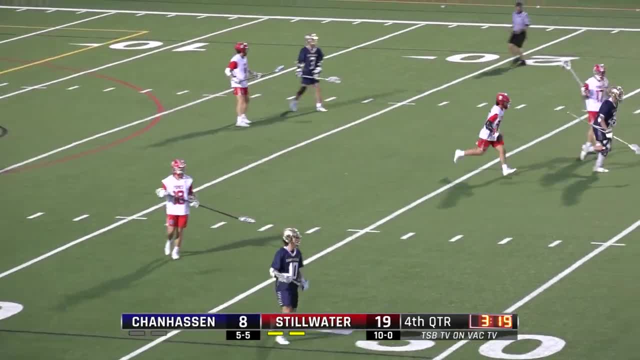 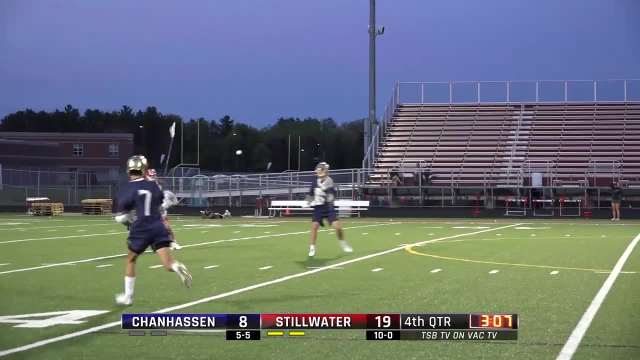 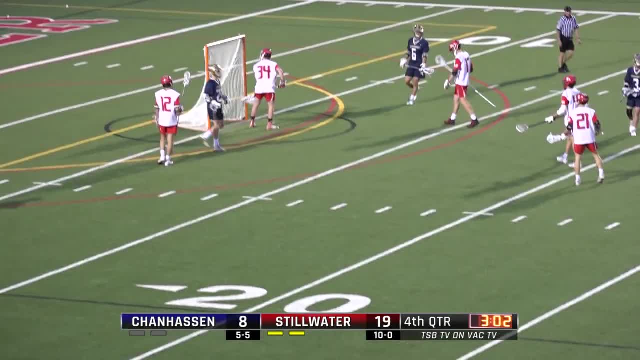 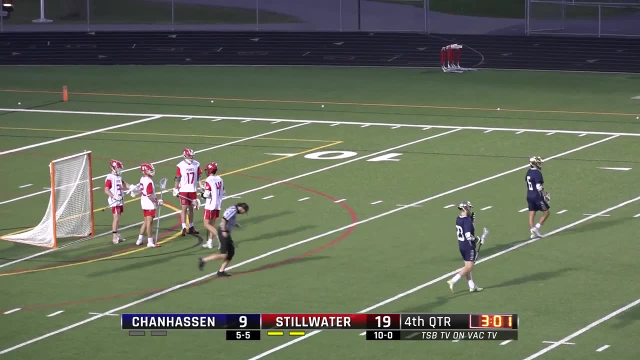 And we've been praising the offense for Stillwater so much, we should not ignore what they did to them second half. until there he had four goals. make it five. it's gonna be a season high for him, Alex Dewey, the MIDI, getting five goals. he only had two hat. 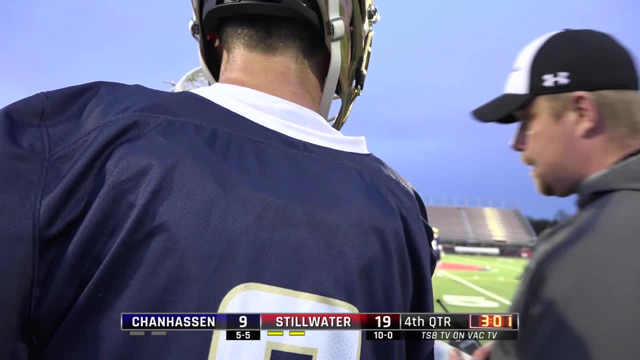 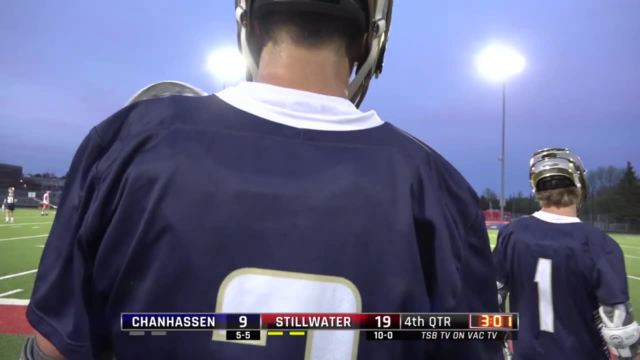 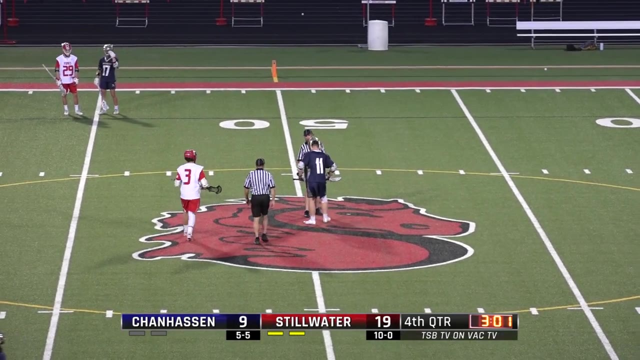 tricks or one hat trick entering this game. that's another one here. but up until that point, Robert Stillwater did a great job neutralizing him. in the second half he was the big reason. Chanhassen hung around, absolutely, absolutely and and when one player is shouldering most of the scoring load and you can shut. 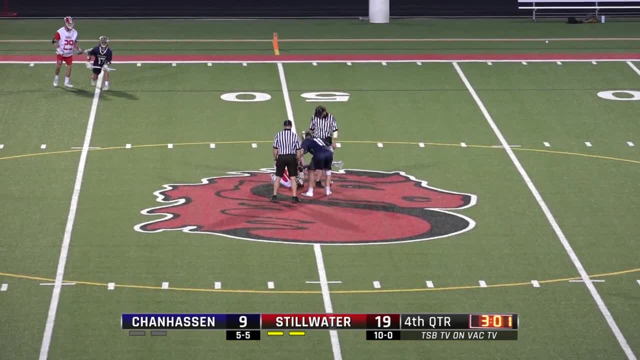 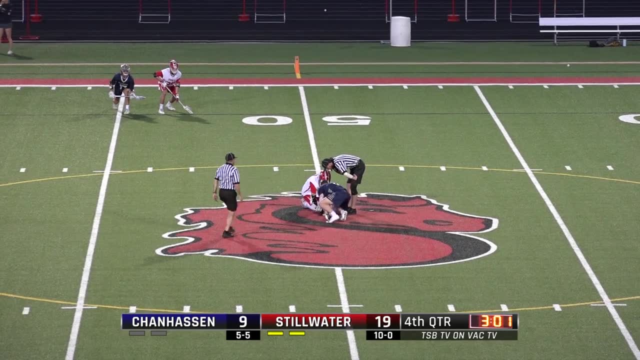 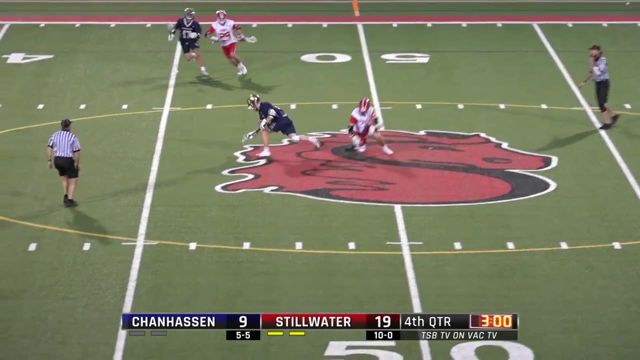 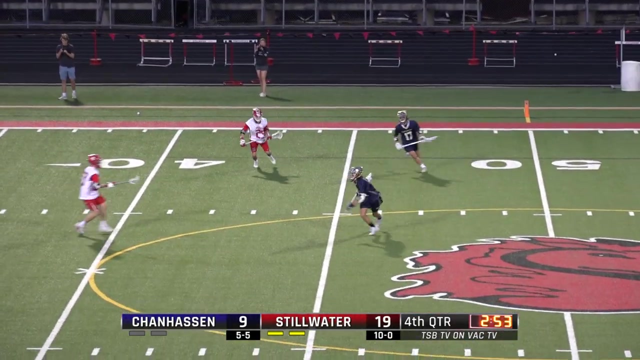 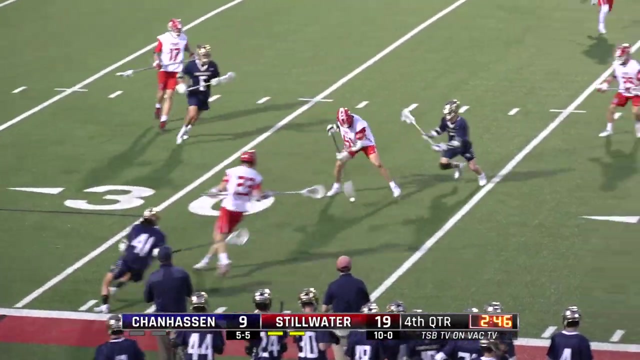 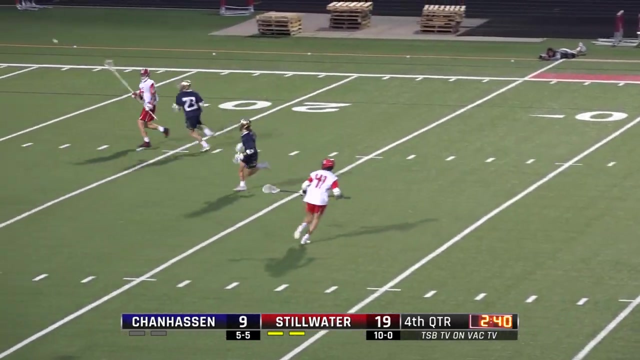 that one player down. that doesn't leave you with much a season-high for Dewey and that will put him at 15 goals for the year. you give him credit. he did everything he could. it just wasn't enough against this Stillwater offense that has caused so many fits over the years, over the 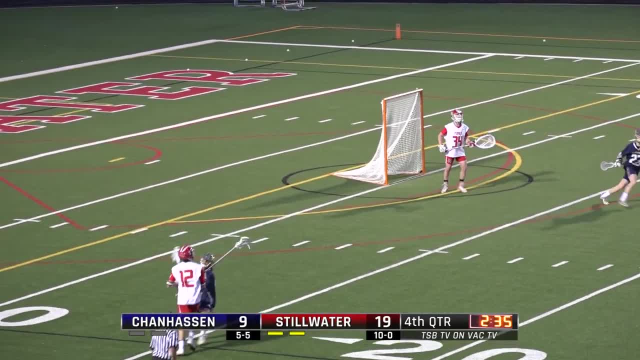 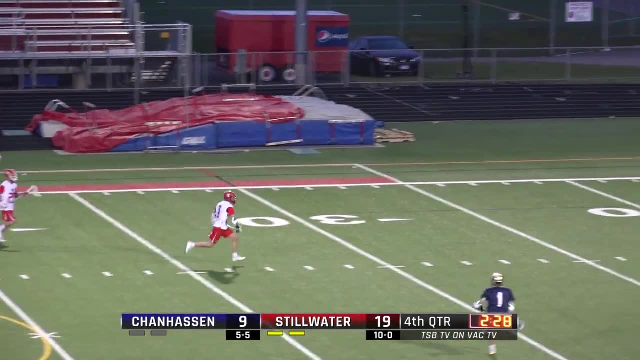 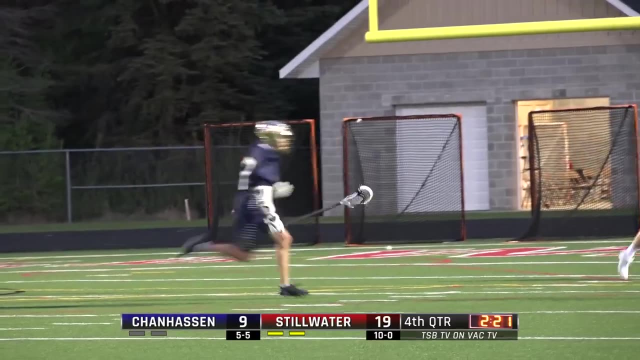 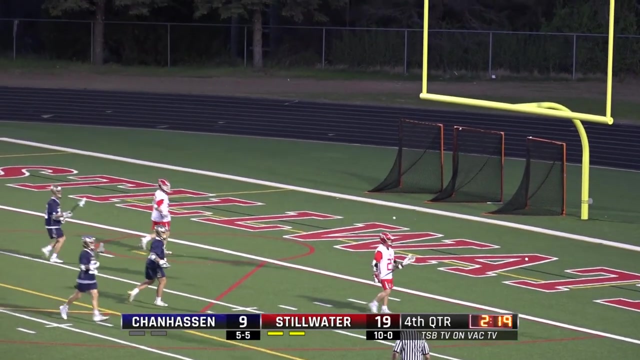 season. well, they have over the years. they won 13 games last year. this was not a fluke and they're gonna get it. oh, if clay batterton doesn't try to go behind the shoulder or whatever he did, if he doesn't back that, I like that, I think. 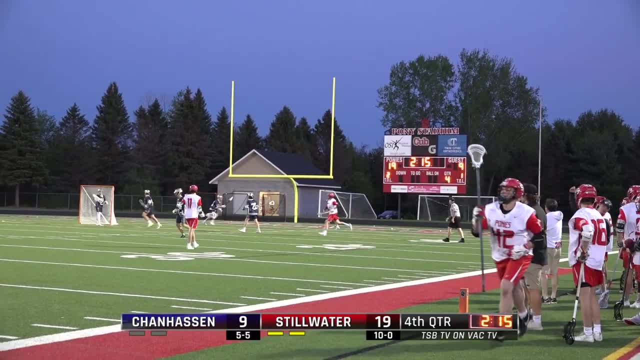 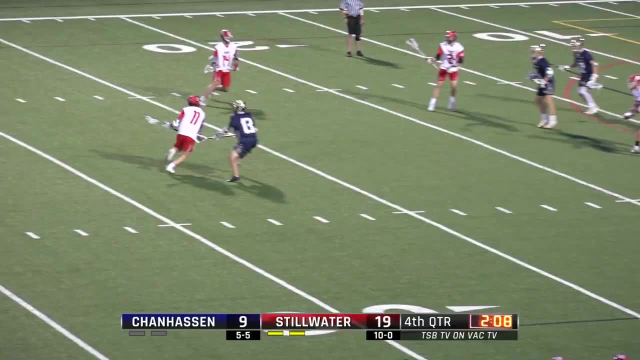 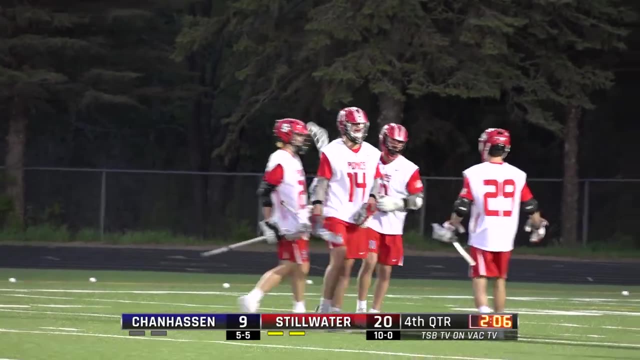 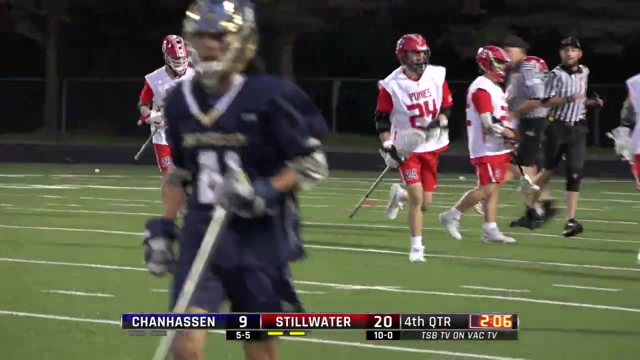 that would have been the 20th goal, but it's still Stillwater ball. yes, they're hungry for one. more. day has turned tonight and they get it. Logan B gives Stillwater their first 20 goal game of the season and for Logan B's that is his. 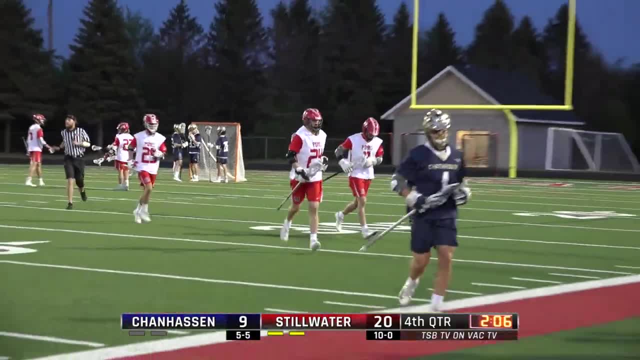 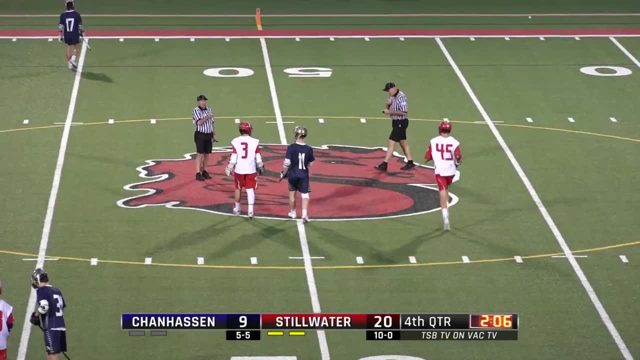 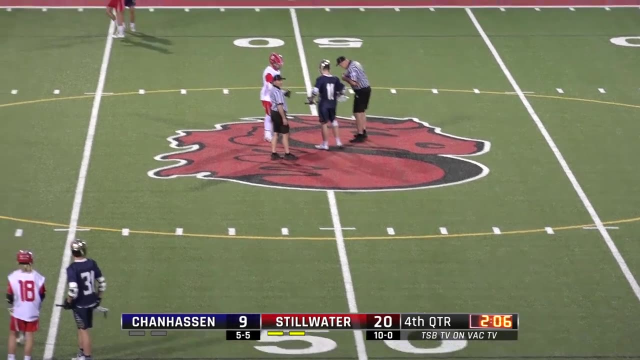 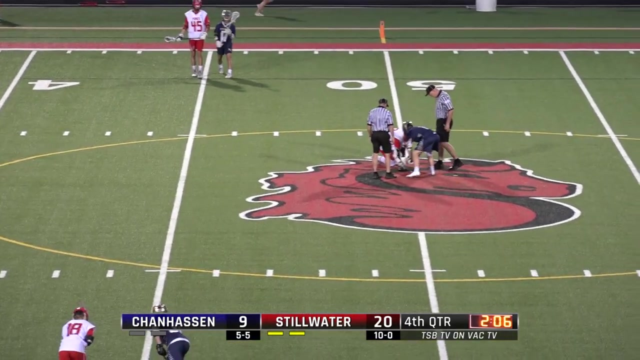 second goal of the year. seven goals for the ponies in the fourth quarter and Theo Robinson gets on the board with the assist. well, that's fun to see some of those deep reserves. yeah, it's like watching a football or basketball game when the outcome is decided by the end, you know well. into the fourth. 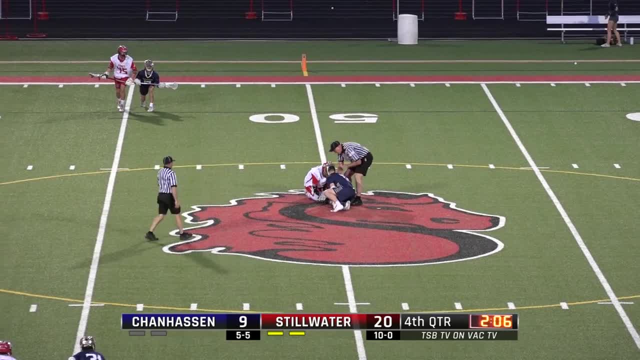 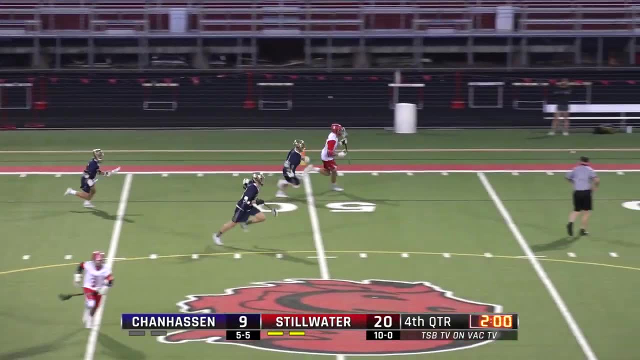 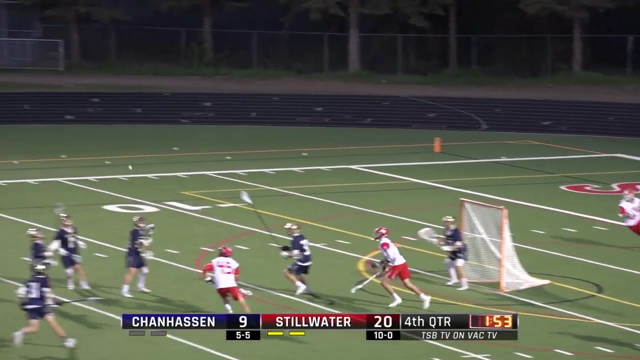 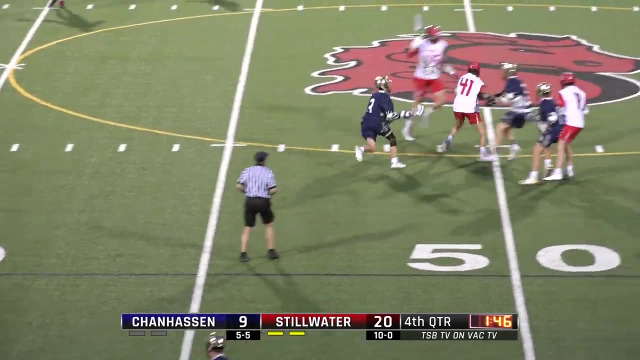 quarter, second half. whatever timing system is used, it's always fun to see some of those guys that will take over the reins in the upcoming seasons and get some action. they want more. Robert, I don't know what your athletic experience is, but I have to imagine for Logan B's and 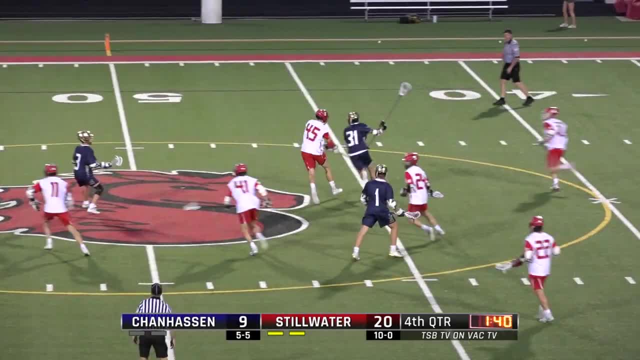 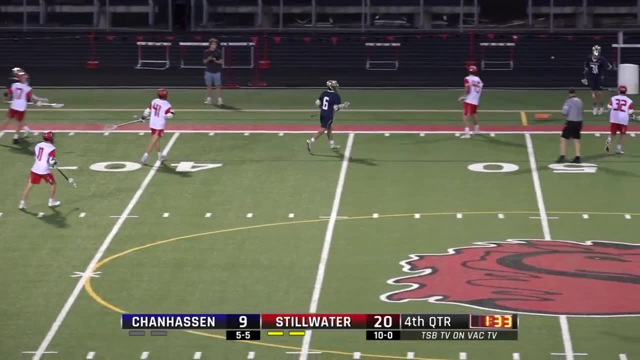 for that team. it's always cool to see one of those guys that scraps just as hard as the big guns. he doesn't get the playing time, but to get a goal in varsity play when you don't get many chances to play, that's always a good. 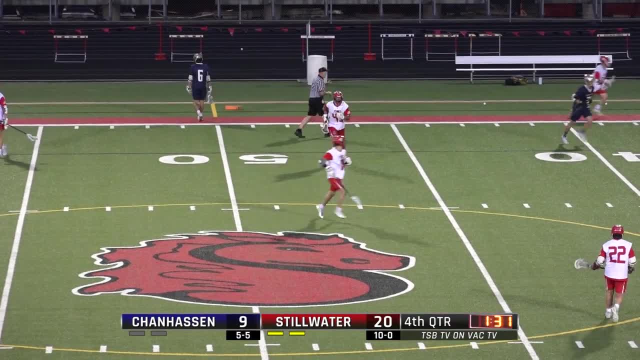 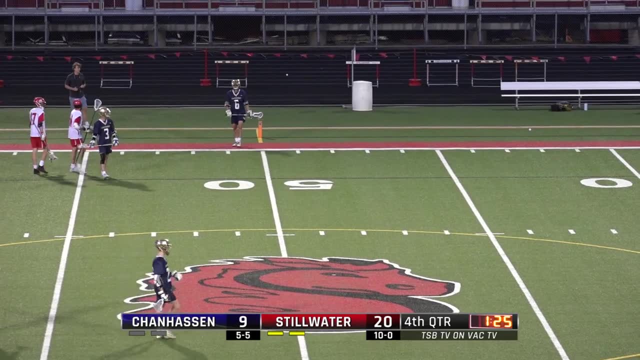 feeling, Mike. I wasn't ever one of the top players in the team, so when I got some, when I made a big play boy, I really made my season and for some of these guys they're good. you're right, Mike, they're kind of unsung heroes, some of the guys. 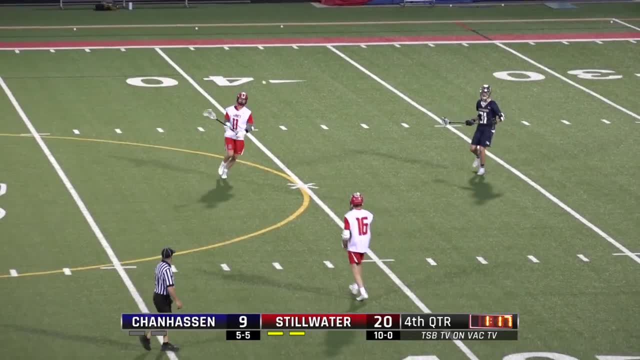 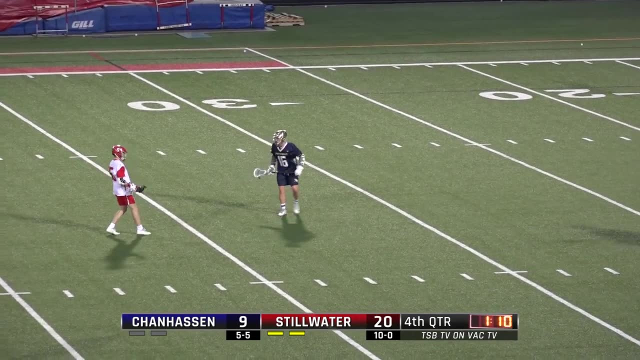 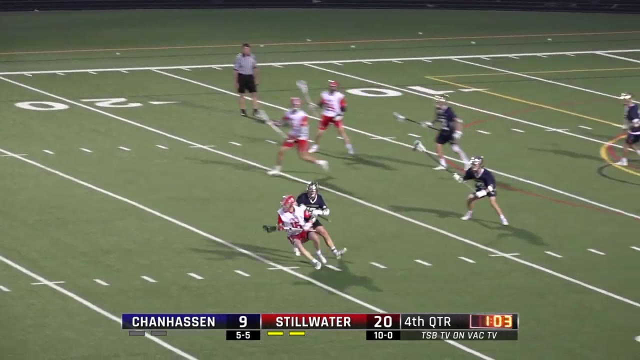 in the team don't get, don't see the ball much. but but the way that they cover the offense so that they don't have to scrum for the ball says all says a lot about them. Mark stopell, it's a good feeling. break ball last feint. 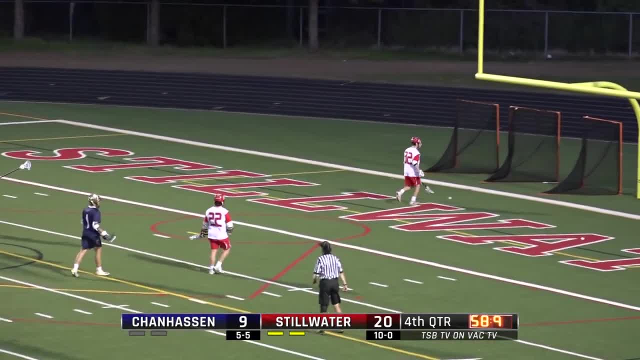 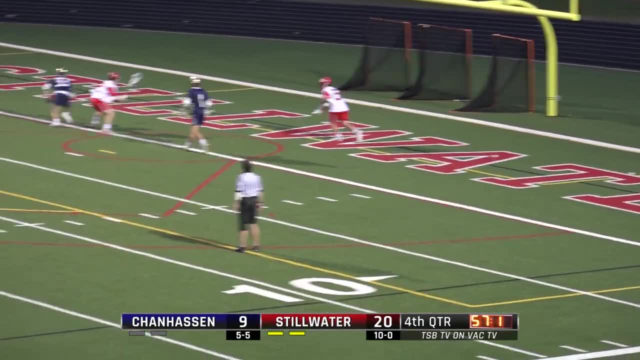 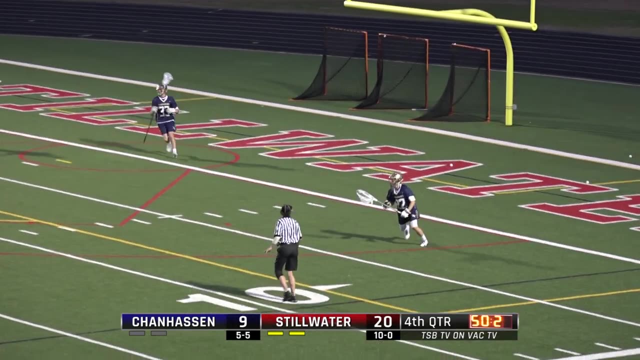 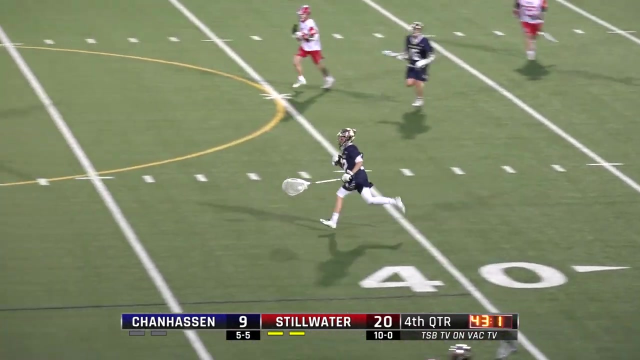 just over a minute to go, am I? Nelson summery would sure like to get on the board with his friends here. goal-wise, yes summary. he's been on the board a lot for assist tonight, but you know if he doesn't score, so what? your summary and Evan's and are similar in 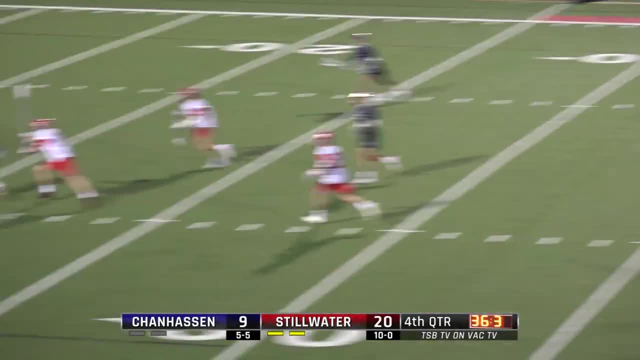 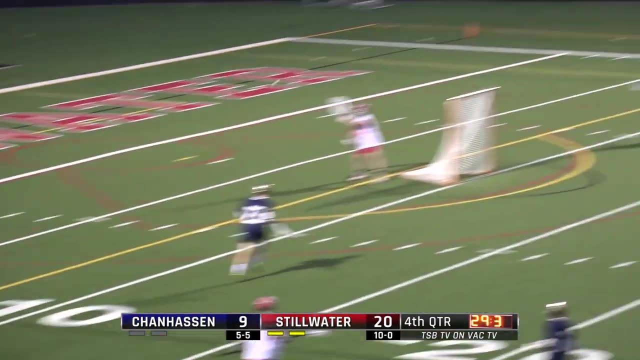 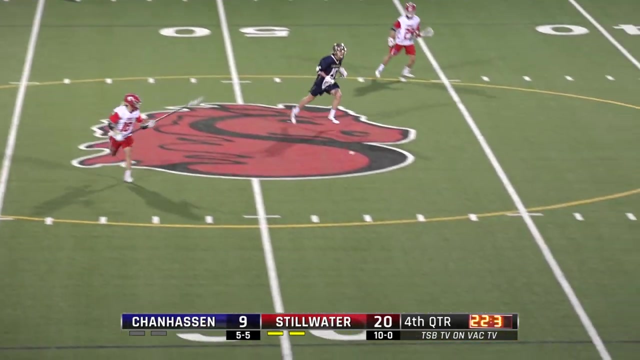 out, It looks like Stillwater will finish at 20 for the night because Chanhassen has the ball here. That was a goalie that came all the way up. That was Rathy Yeah to try to score a goal on our goal. You know well, you've given up 20.. It's like hey, might as well If Gunnar Arendt the 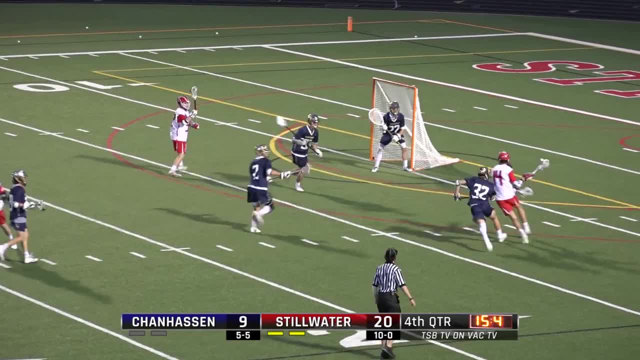 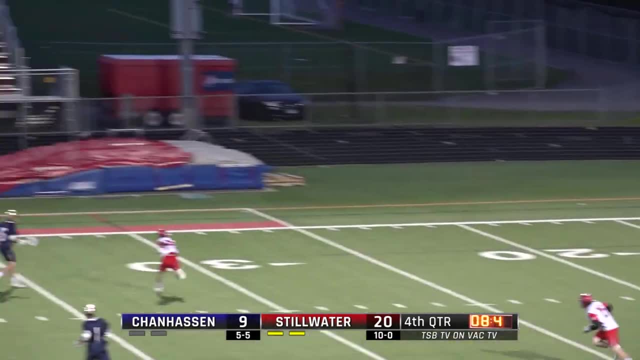 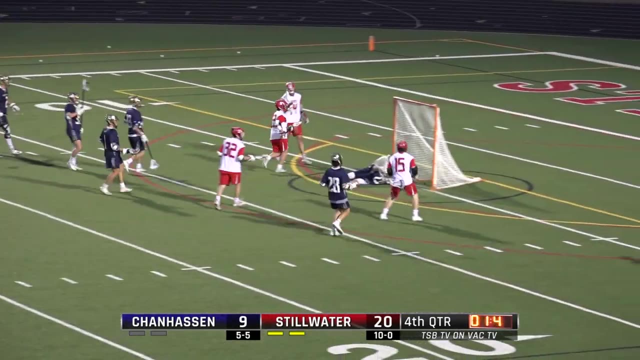 Stillwater goalie can get his first one of the year and Rathy does get back in the net in time, Jeff is saying gives new meaning to the term pull the goaltender. Well, in hockey if you pull it, the goalie can't come out. And just before time expires Stillwater will get 21.. And that 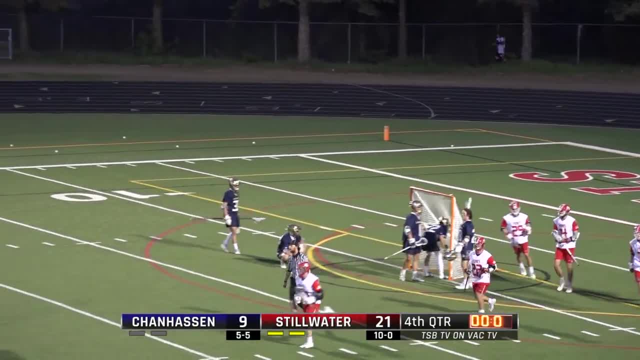 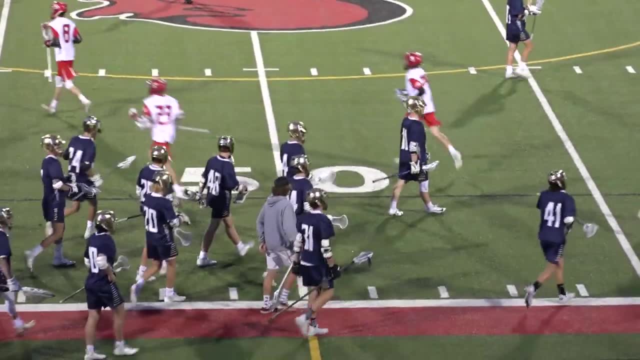 will be Theodore Robinson. Theodore Robinson who scores, And my score sheet only goes to 20, so Theodore Robinson just broke it And they're going to let time expire because the goal is inconsequential. So Theodore Robinson gets a goal, It will count. 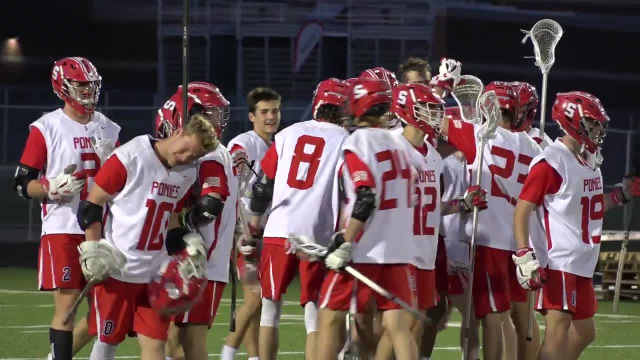 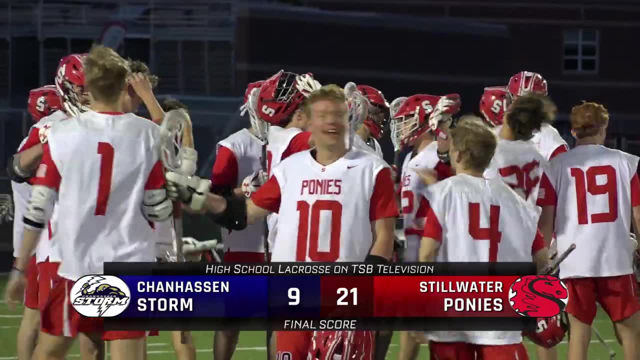 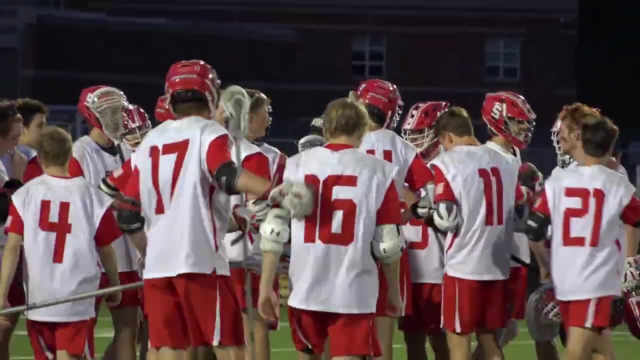 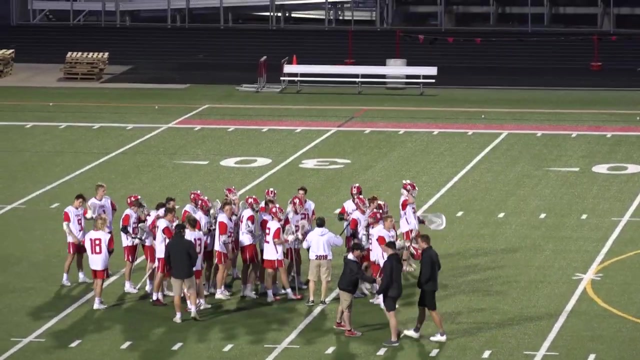 And for Theodore Robinson and Nick Dario gets the assist. So Theodore Robinson ends the game with what I believe is his fifth goal of the year. Robert, 21-9 win for the Ponies. That second half was something to behold. Another display of mastery by the Ponies. 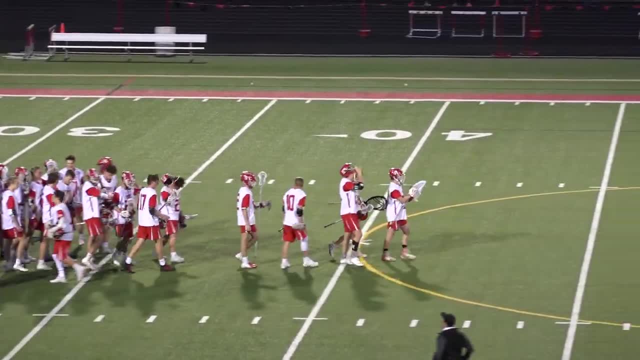 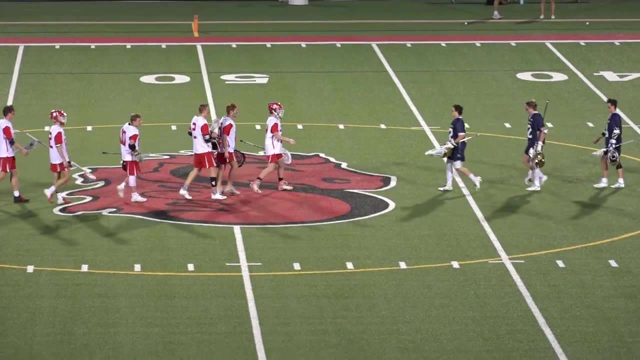 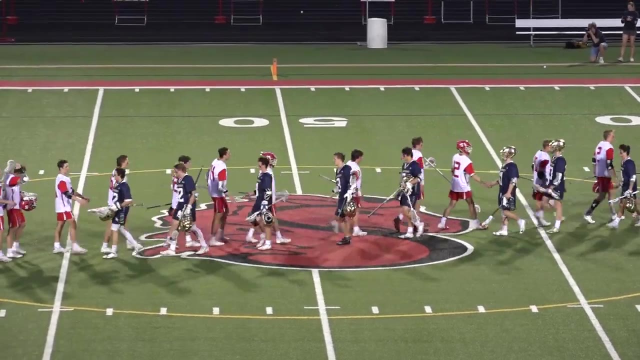 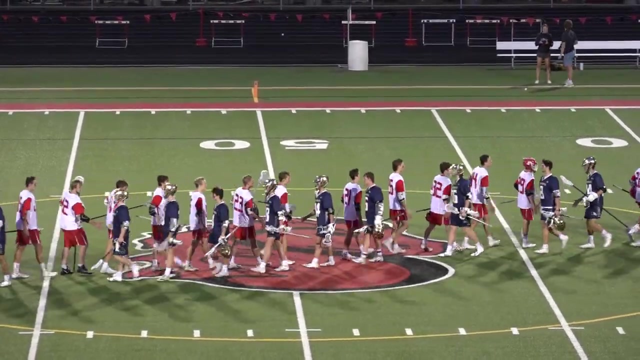 showing that not only can they shut another team down, but if they, If the other team relaxes at all, they're going to make it painful. A 12-3 scoring advantage in the second half, 12-3. And yeah, that's all I got to say. 12-3 edge in the second half. But let's recap the scoring and 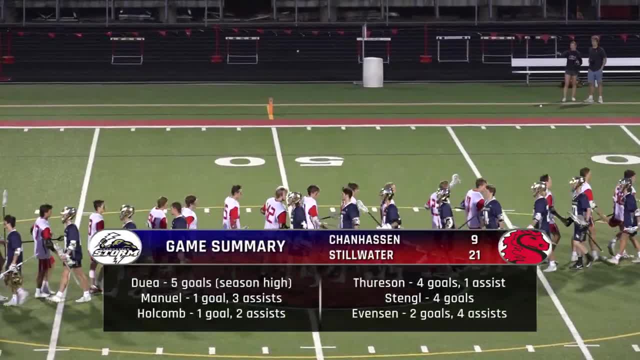 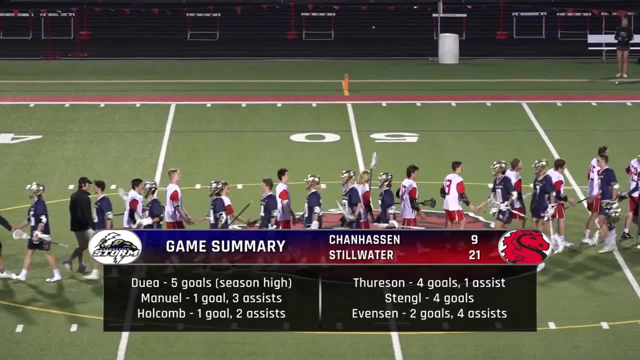 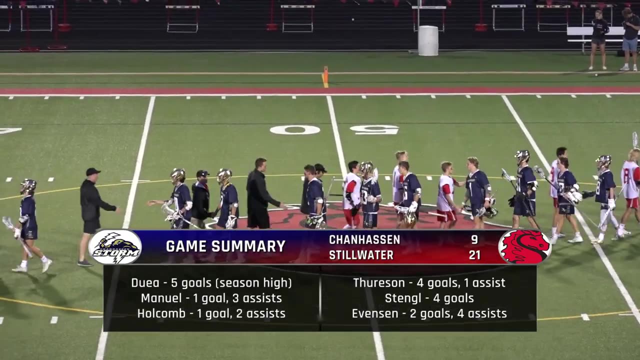 say happy birthday to Coburn Van Dyne, who is the face-off specialist. Four players with four goals, It's a win tunnel, Don't worry, Nobody's angry. Joe Stengel with four goals, Cody Berger with four goals And Ty Thurston with four goals to lead the Ponies. Blake Evanson with a pair. Quinton White: 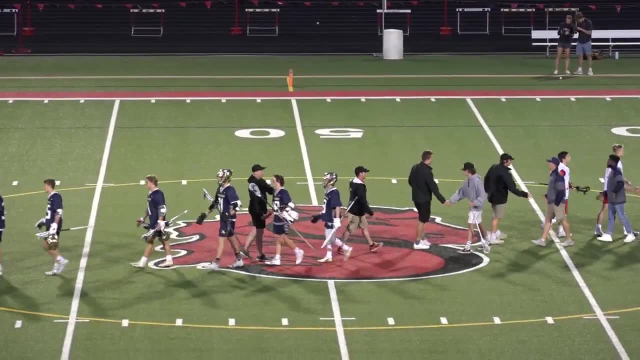 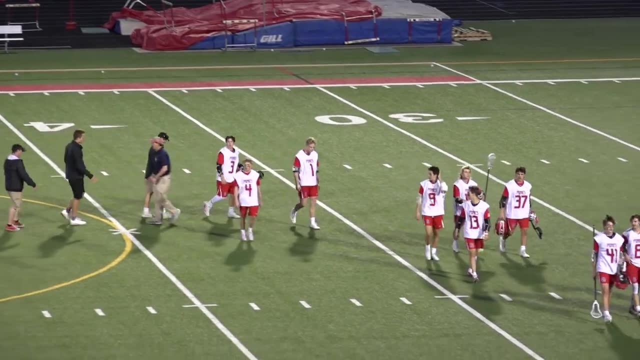 with a pair And Justin Siegfried scored his first goal of the year on the first assist from Gunnar Ahrens And Ben Carl got a couple as well. Four assists from Nelson Summary And Evanson had three assists. So you know, no goals for Summary, but a big point night And it was a big point night for.